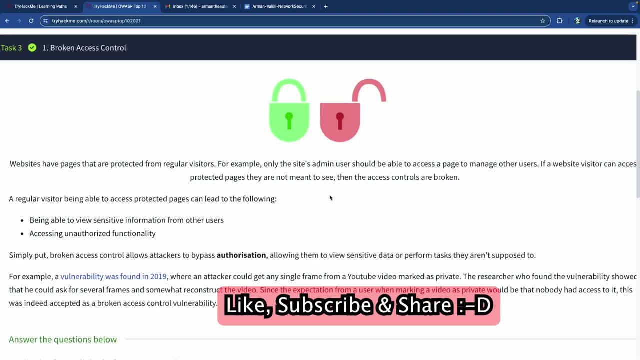 is that the pages or parts of your web application that should be accessed only by admins, for example, shouldn't be accessed by any other users. They shouldn't be accessed by the public. These specific pages, if they have access to the public or other users, they shouldn't be accessed by 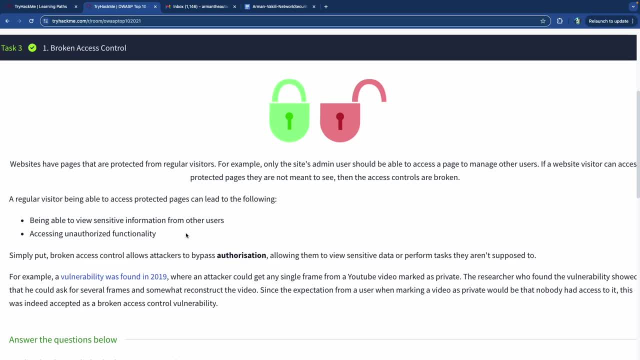 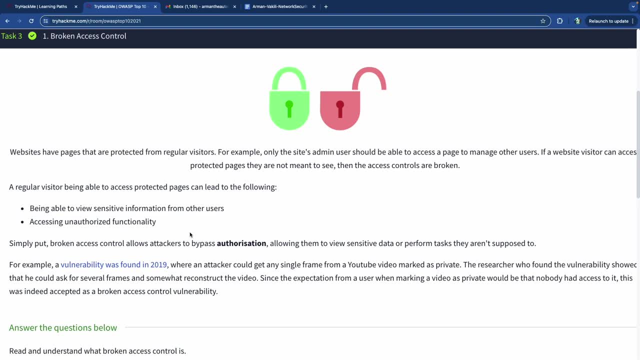 users. That means that the access control for that page is broken And this is the top vulnerability. in the last OWASP top 10 list that was dropped out, It was in 2021.. This was the top vulnerability, meaning most applications, most websites and all these different things. 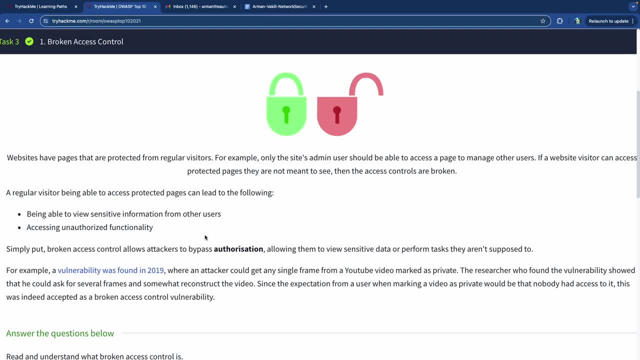 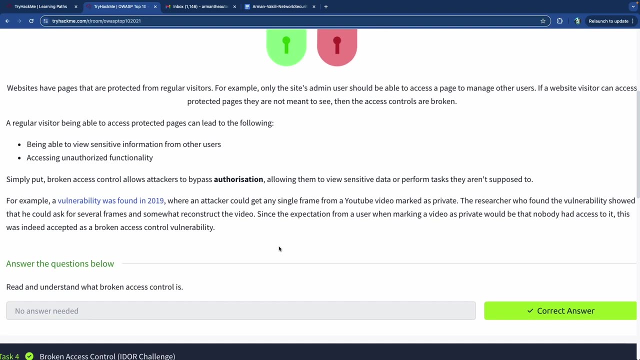 had web pages that were available to non-privileged users that should not have been available. So, simply put, broken access control allows attackers to bypass authorization, allowing them to view sensitive data or perform tasks that they're not supposed to, because those pages were not blocked. 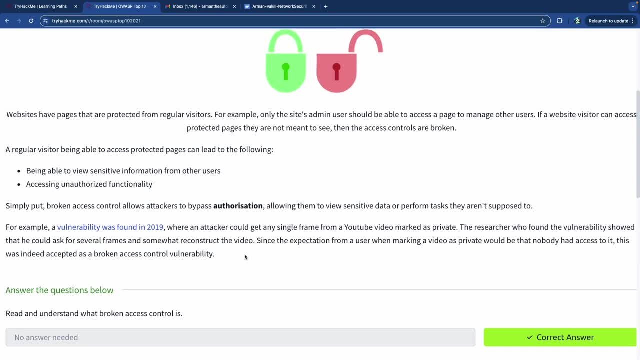 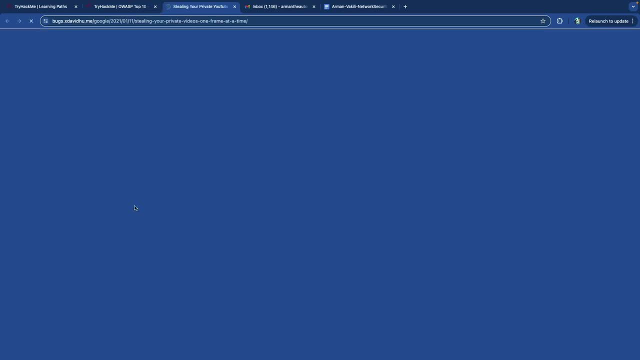 off or they were not secure. So that is the main vulnerability that has happened And there was an example here that was in 2019.. There was a vulnerability that was found And this is it. If you wanted to go check it out, you can Google this: stealing your private YouTube videos. one. 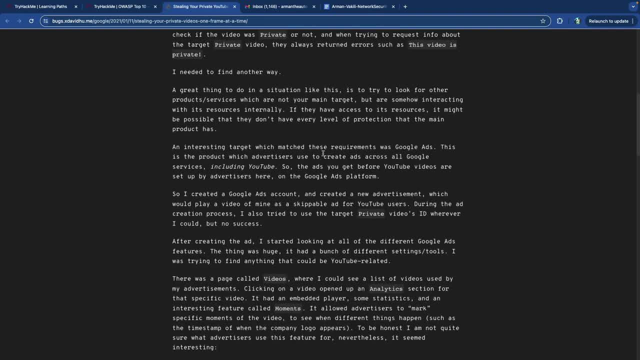 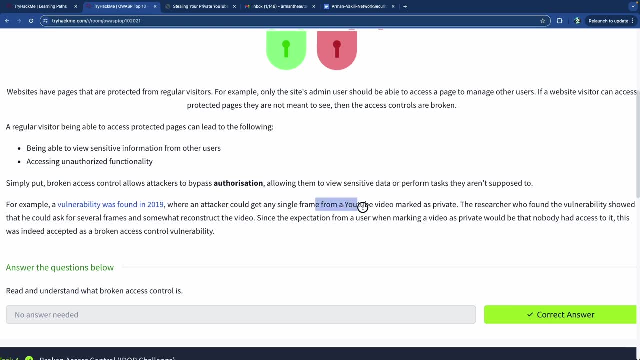 frame at a time. You can go and check this out And literally you could just search for that, stealing your private videos one frame at a time. But the attacker could get a single frame from a YouTube video marked as private And then the. 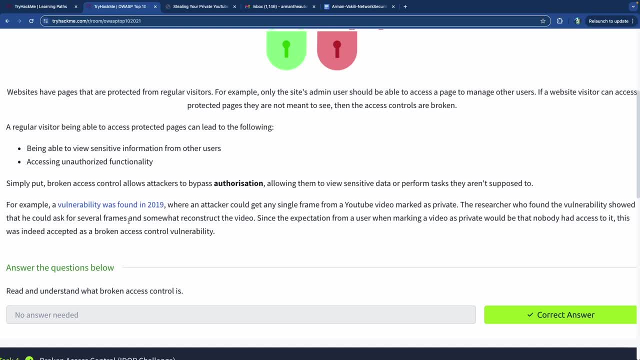 vulnerability that he could ask for several frames and somewhat reconstruct the video And since the expectation from a user when making videos private would be that nobody has access to it, this was indeed accepted as a broken access control vulnerability. And this is on YouTube of. 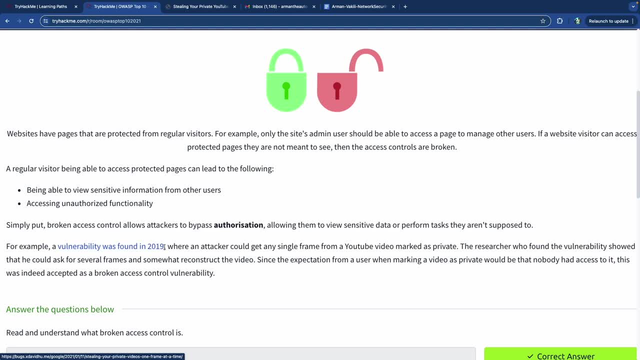 all places. So you got to understand that Google backs YouTube. It's a gigantic business And it's relatively recent. It was just five years ago, 2009.. And it's a huge business. And it's a huge business. It was back in 2019.. It was five years ago, Holy cow, But it was just five years ago that. 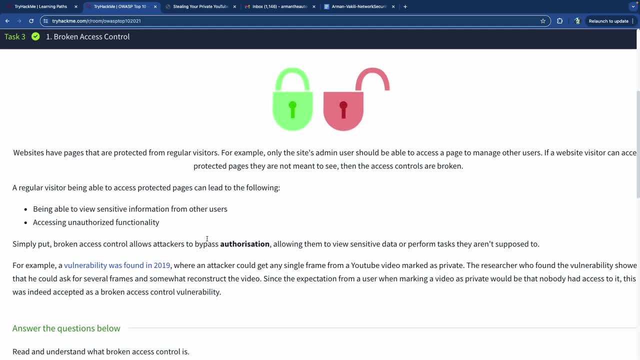 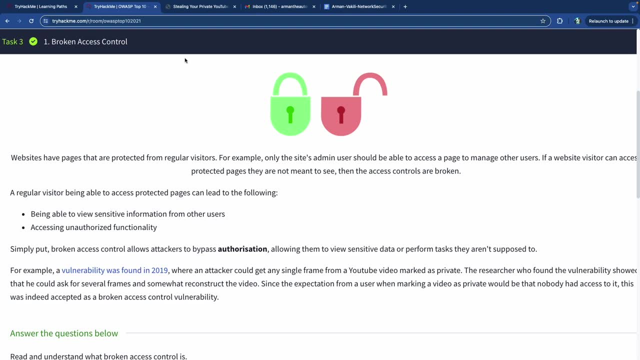 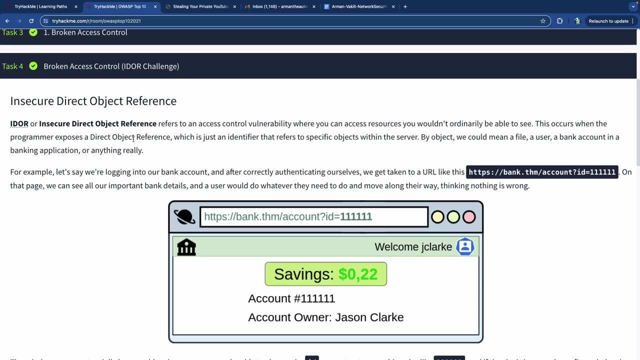 this thing happened, So it's. it could happen to anybody, even the biggest name in the game, And if that's the case, that means that you're also vulnerable to it too. So let's actually look at an E-door challenge, which is the insecure object reference challenge. So let's go check that out. 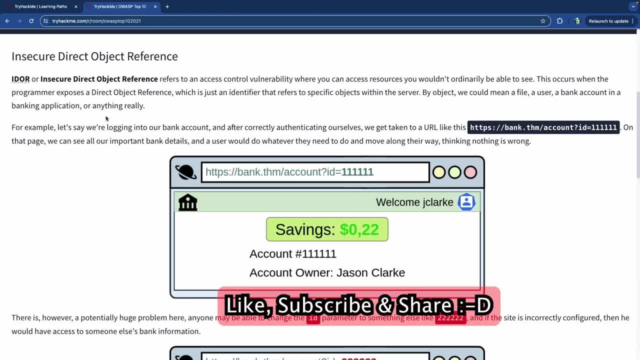 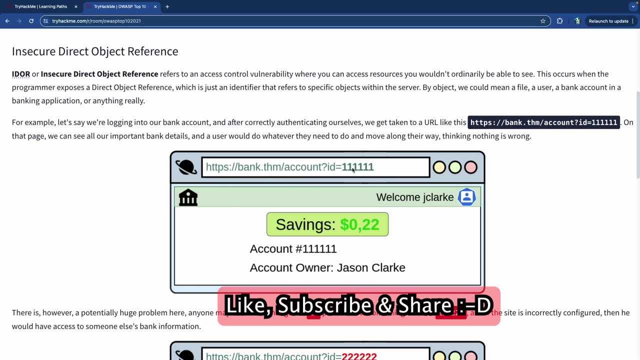 and see what we can exploit here. An insecure direct object reference is essentially something that is available to on a site that you can access. So, for example, in this case it's the ID here that we see and you shouldn't be able to number one. you shouldn't be able to. 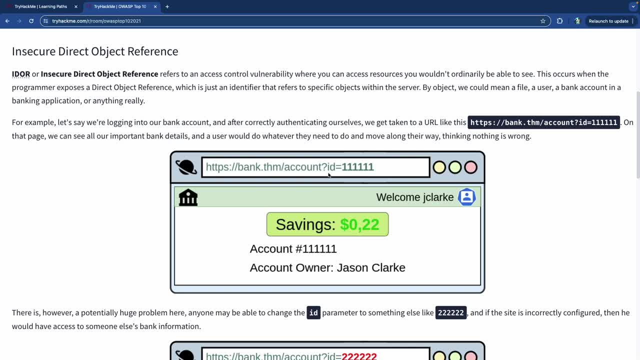 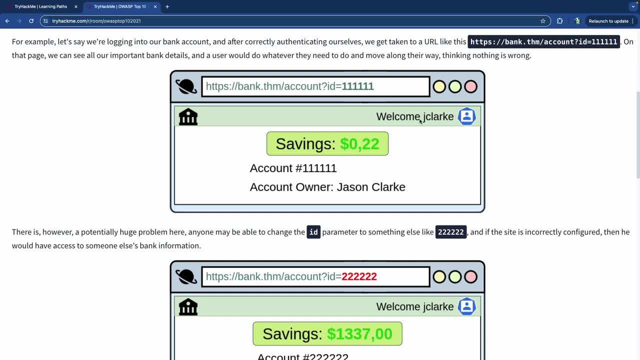 see it. So this link is a bad link. But then the second part that's like really crazy is that you shouldn't be able to edit this. So in this example, the person that you know landed on their account is Jay Clark and their ID is 11, 11,, 11.. And then they changed their ID to 22, 22,. 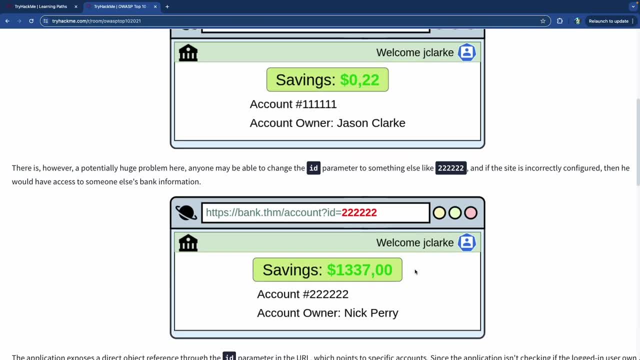 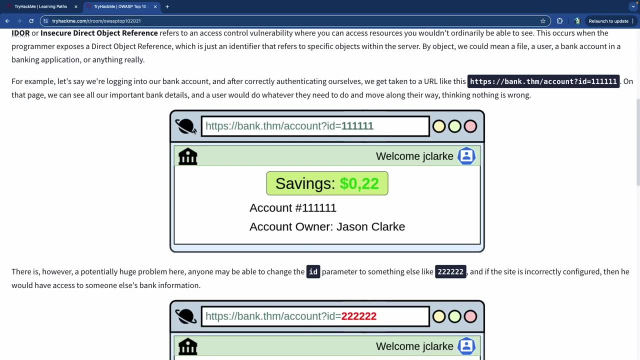 22. And they got access to Nick Perry's uh account information while they're still logged in as Jay Clark over here. So this is called an E-door vulnerability, meaning that the the insecure direct object reference is something that is inside of the link that you. 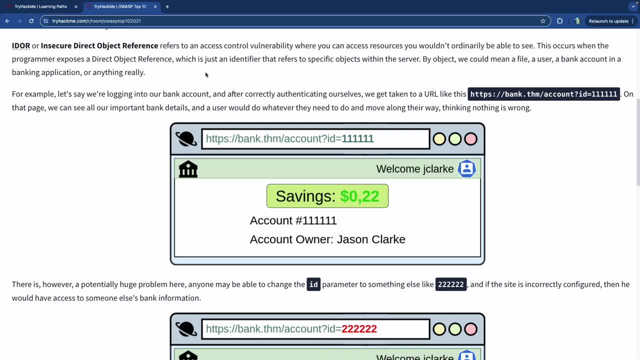 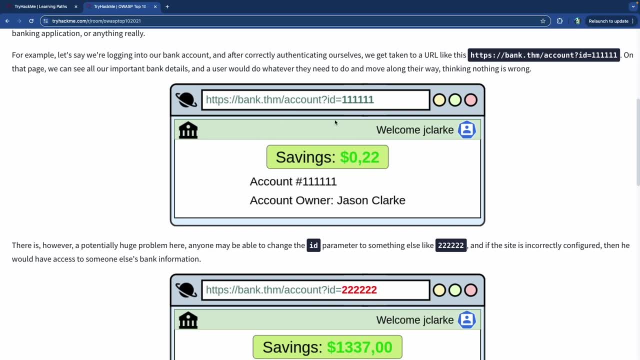 shouldn't be able to get access to. And then when? uh, you can change anything about that link and sometimes even things within the webpage. you can change certain things just about the link or the webpage and it gives you access to certain pages and certain information, and even certain. 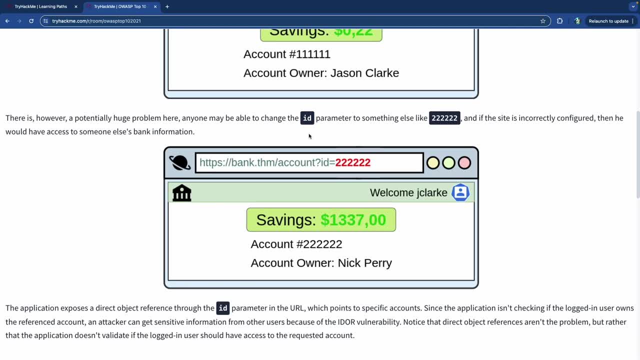 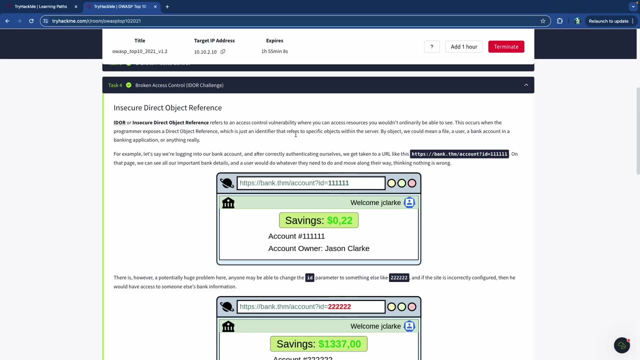 versions And those things should not be available to you. They should not be possible. So that is one of the most basic and, honestly, very common uh forms of uh, uh broken access control that can happen. So what we're going to do is we're going to actually go to the website that I had. 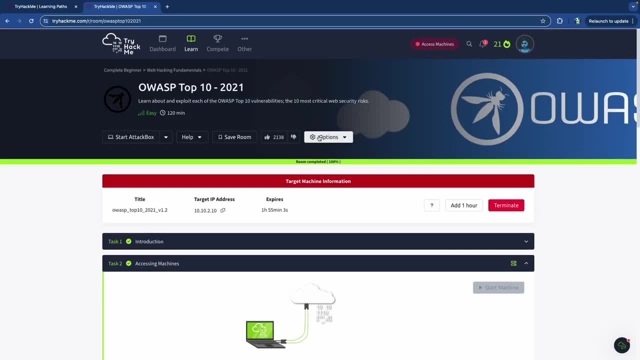 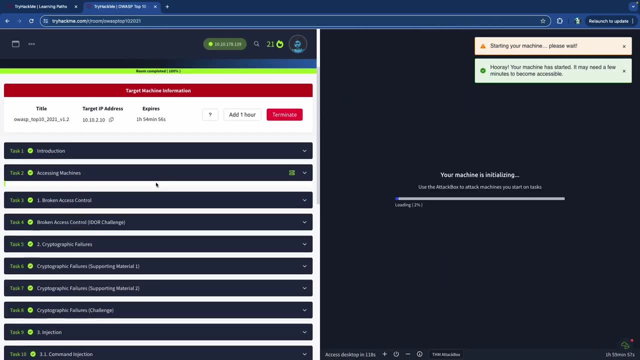 to launch. here There was a machine, a virtual machine, that I was supposed to launch. We're going to actually go to that virtual machine through the attack box that we have here And then from there we're going to go through. uh. 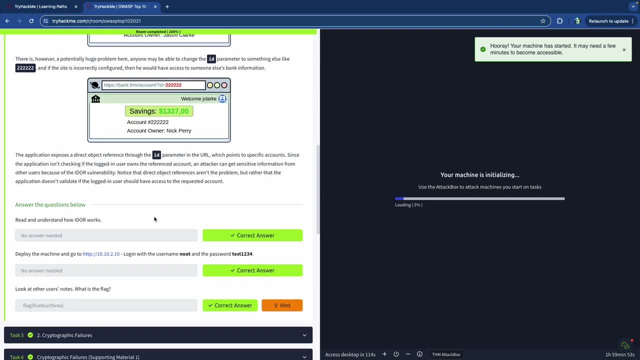 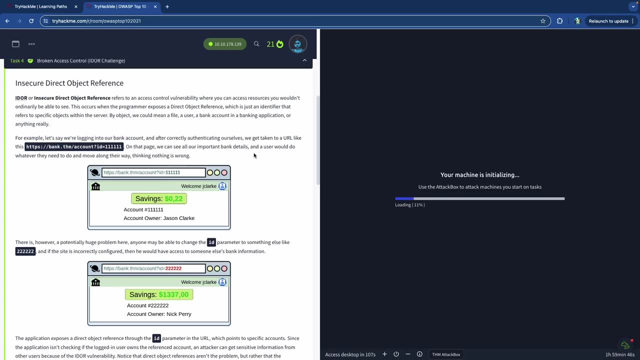 the just some of the webpages that are there and try to find this flag. that's available at the bottom right here. So it's going to be in the user's notes. So I am going to wait for this thing to load real quick And then we're actually going to run that. All right, here we go, We are. 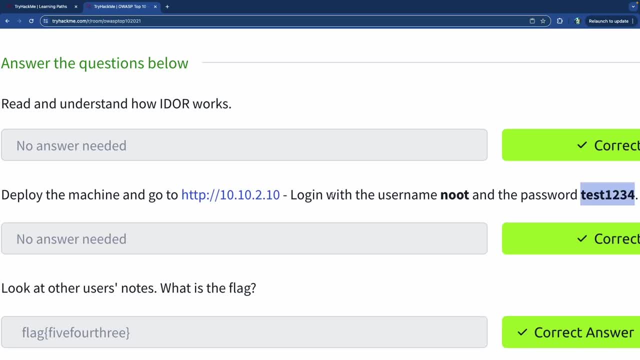 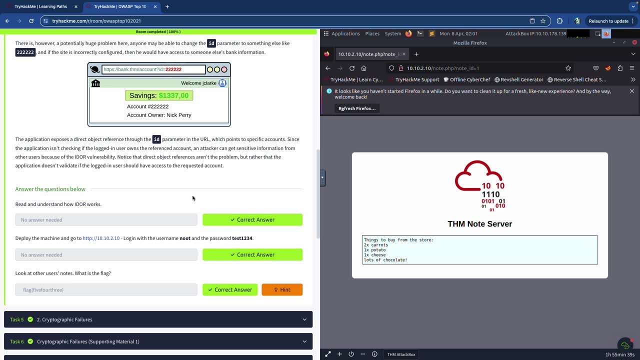 logged in. I logged in with the newt and test one, two, three, four. username password- This is the link that I'm on. Uh, when you launch a virtual machine through try hack me, they give you an IP address and then you can either connect to it via VPN from your own machine or from the. 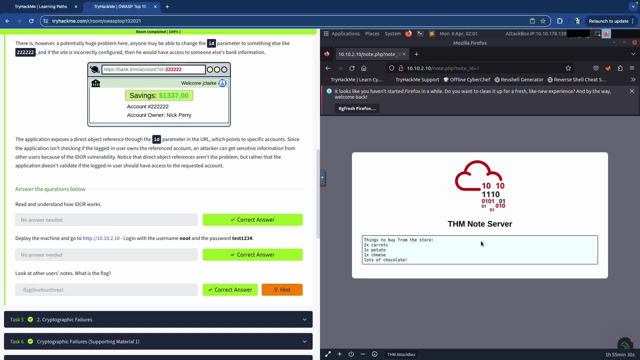 browser, just use the attack box, And so when you log in and when you land on the homepage, this is what it looks like: You have uh notes, uh, you know things to buy from the store, yada, yada, yada, And then we have the URL, which is the important part, right here. So, as we noticed, 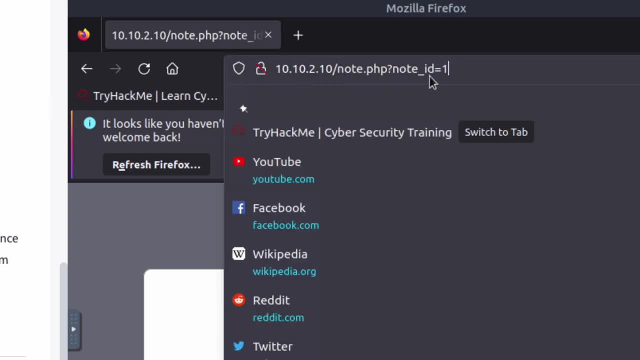 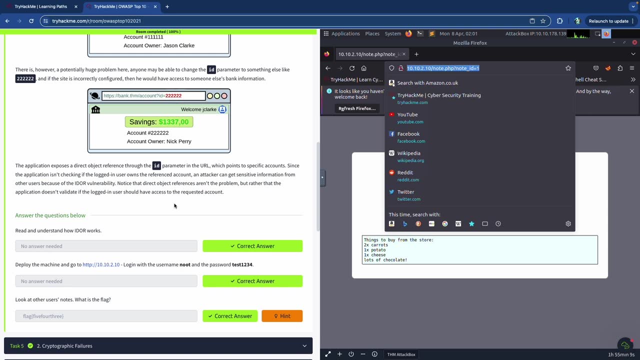 uh, in the previous example or in the documentation of this, the URL can be changed right, So if I go from one to two to three to four, whatever it is, I should be able to find other users, uh, and notes information And so. 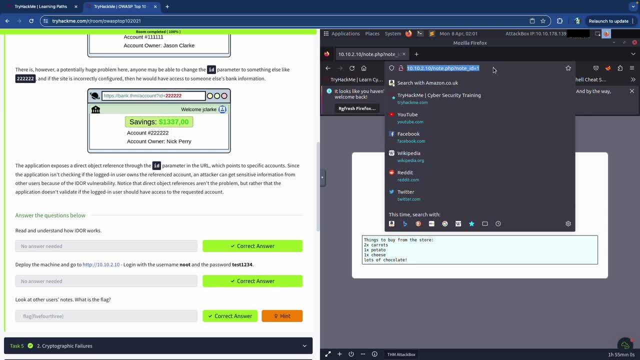 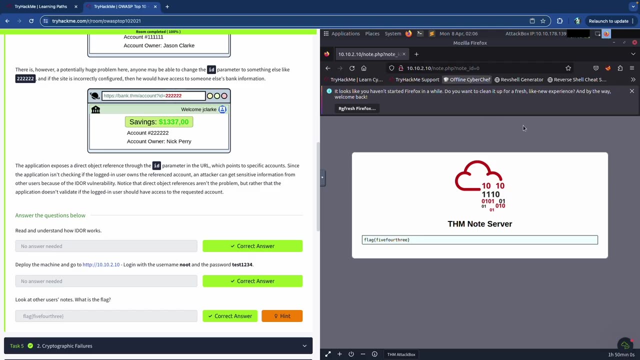 uh, that's literally what I'm gonna do. I'm just gonna, uh, you know, go through, cycle through all the different numbers, the ID numbers, and then see which user will actually have a flag note for me to check. So let's run it and see what we can find here. Okay, here we go. So it was actually. 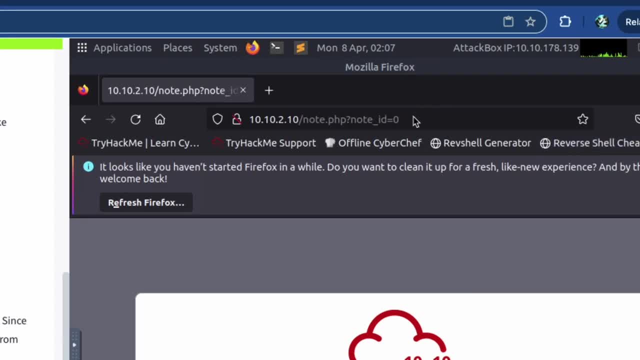 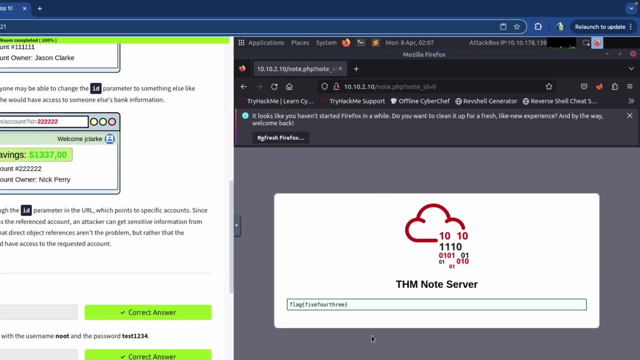 on ID zero. So I went from one and, uh, I went all the way up. when I got to, when I got to five, it gave me a hint and it said, uh, you know, maybe they start less than one, or whatever the hint was. And then it said: 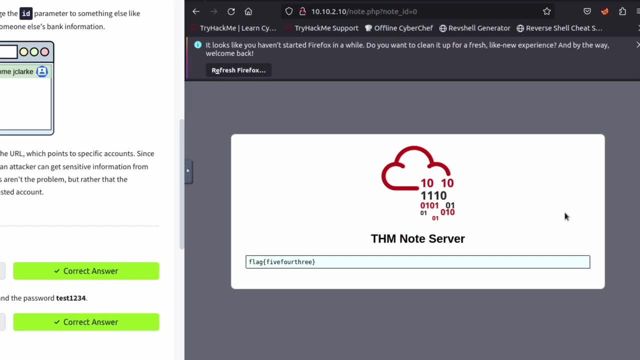 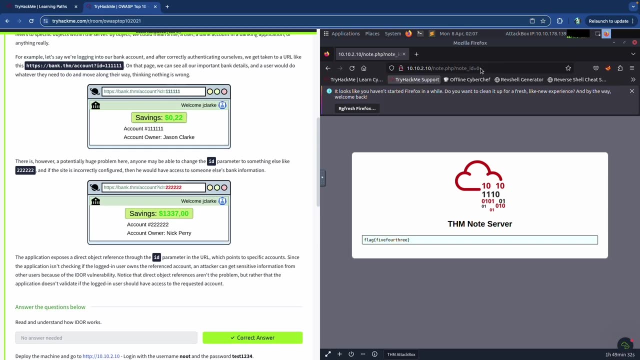 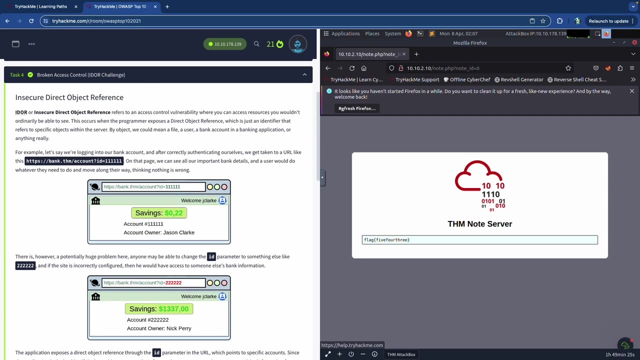 try going less than one, And so I went to zero, and here is our flag. But basically the whole idea is we just cycle through all of the IDs and then we found, uh, the information that we needed And that's pretty much it. So that's what broken access control means: You get to access pages. 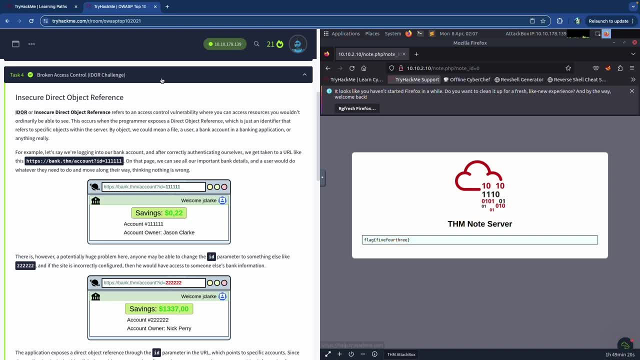 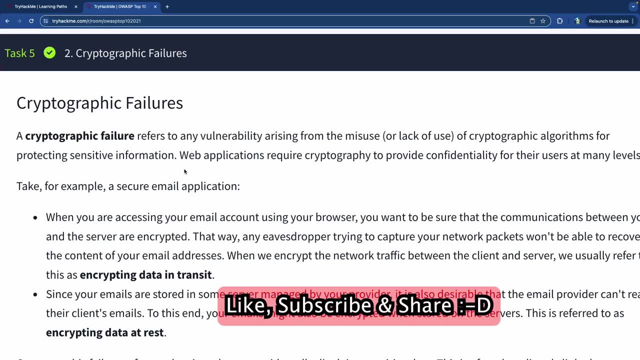 that you're not supposed to access, And that's that all, literally all that means? Uh, let's talk about cryptographic failures. Cryptography is essentially encrypting data. Uh, we did a whole video on this and you can go check that out. Um, when you encrypt data, 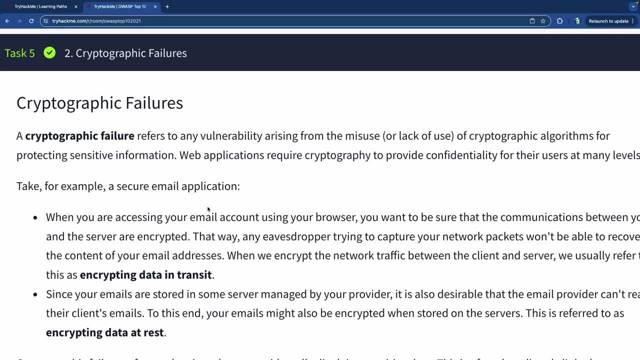 that means you are taking it from clear text which is like this and you're just turning it into a bunch of- uh- jargon, essentially just a bunch of numbers and letters and symbols and things like that. And so you've now encrypted the data and you can either encrypt data in transit. 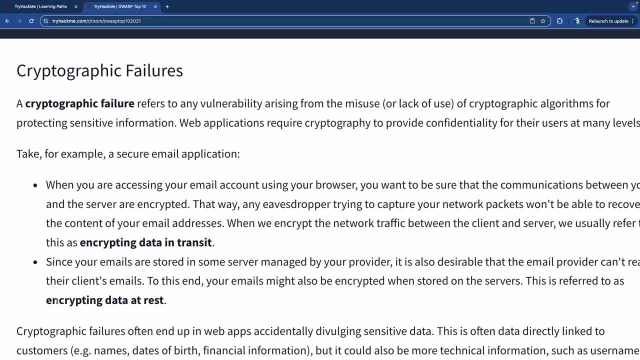 which means while it's being transferred from one place, Another, or you can encrypt data at rest, meaning where it's sitting in a place and then nobody's- uh, you know it's not moving anywhere, but it can be accessed. You can go get that data that. 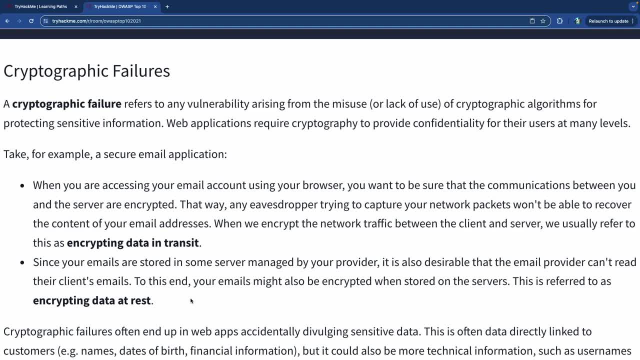 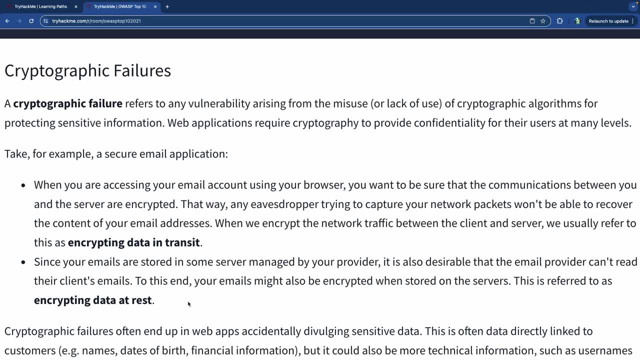 it's sitting in rest somewhere, resting somewhere? Uh, either of those things are very, very important. So you have to encrypt your data, and the the more complex algorithm that you use to encrypt your data, the better off you'll be. Now what happens is sometimes the encryption is weak. 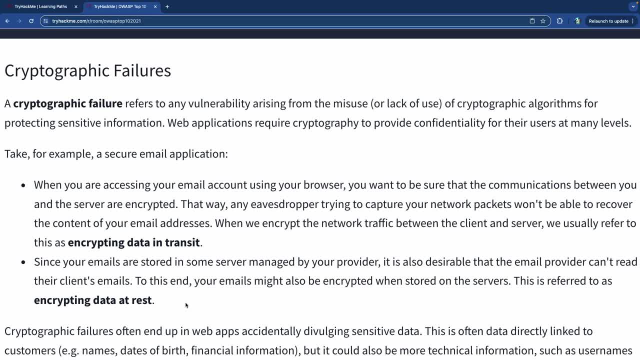 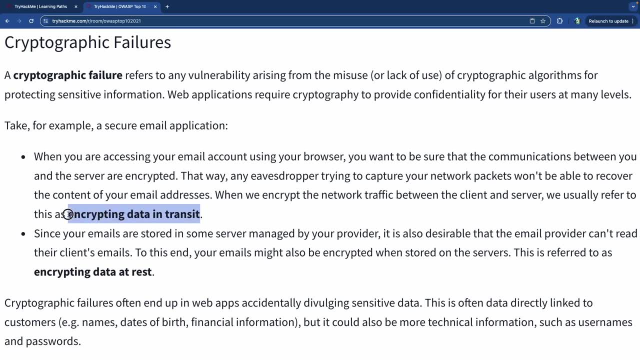 and people can go and decrypt it easily. or sometimes it's not even encrypted to begin with, right? So if it's weakly encrypted or it's not encrypted at all while it's in transit, somebody which is considered an eavesdropper, And then the attack name right there is called. 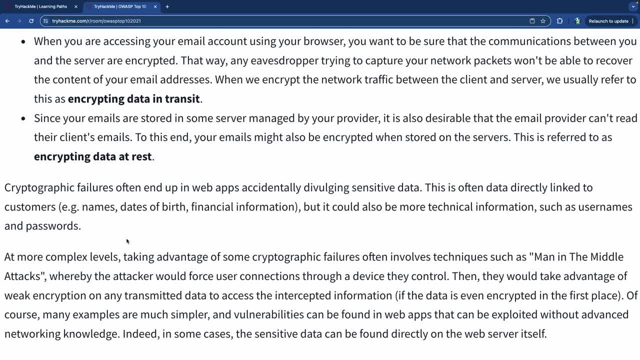 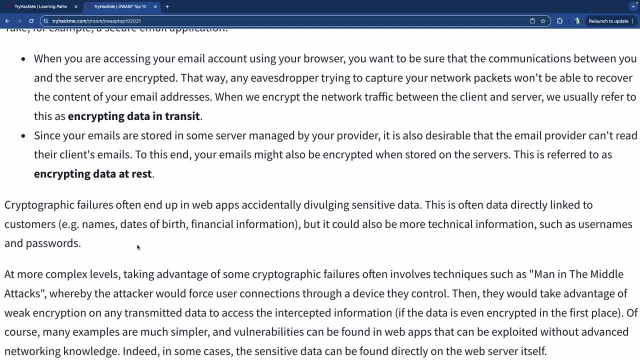 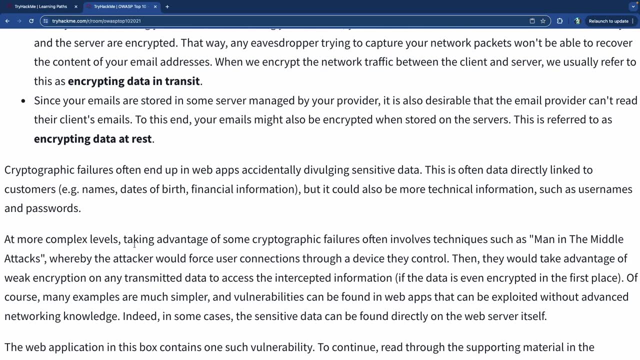 the man in the middle attack, meaning that somebody stands in the middle of the, the load, the source point and then the end point, And then that person is now able to get the data while it's being transferred in transit. And that is a big attack. It's something that actually happens all the time And, uh, it's one. 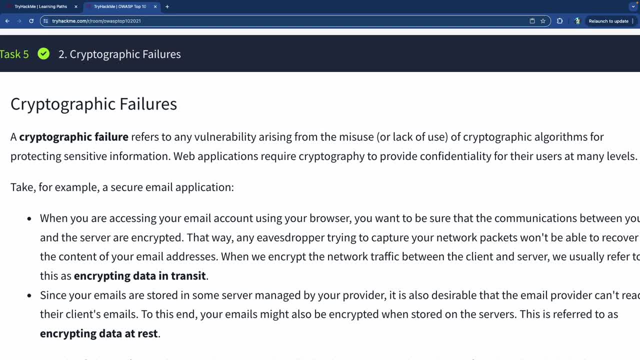 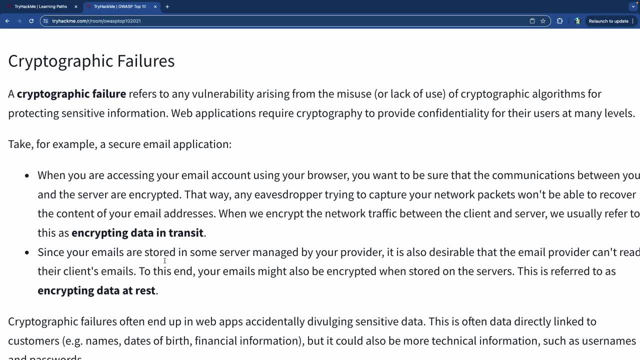 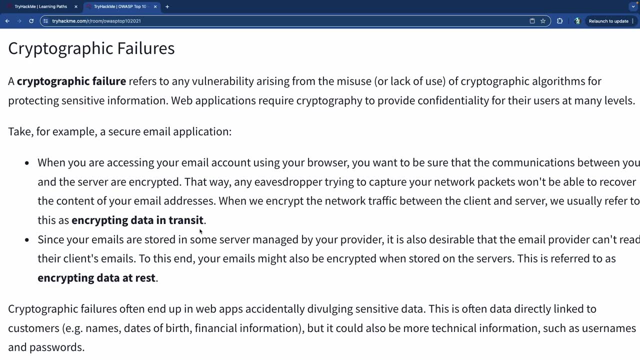 of the, again one of the more common uh web application vulnerabilities. That's why it's number two in the top 10.. So non-encryption of data is a big deal. Uh, if you use ports that are not secure or encrypted, you are leaving yourself vulnerable If you use weak encryption. 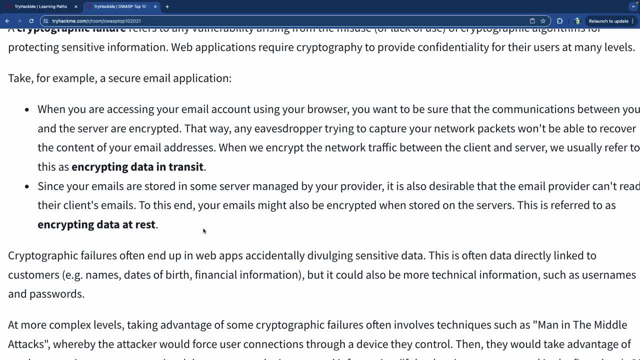 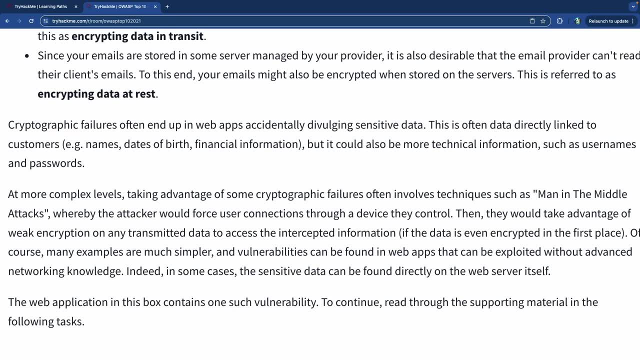 you're leaving yourself vulnerable. uh, encryption, uh, algorithms have evolved throughout time, And the very first one was MD five, And as time went by, it became more and more secure. And so, if you use a weak one, which is the MD five or the MD one, 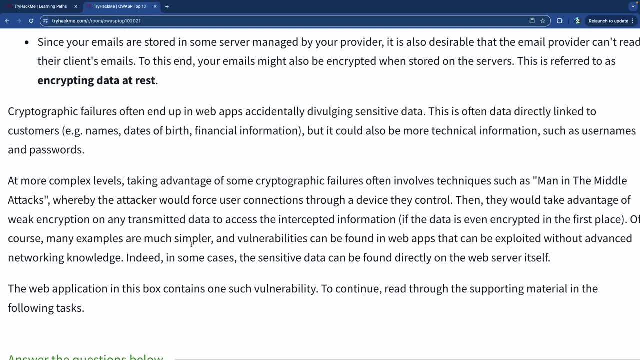 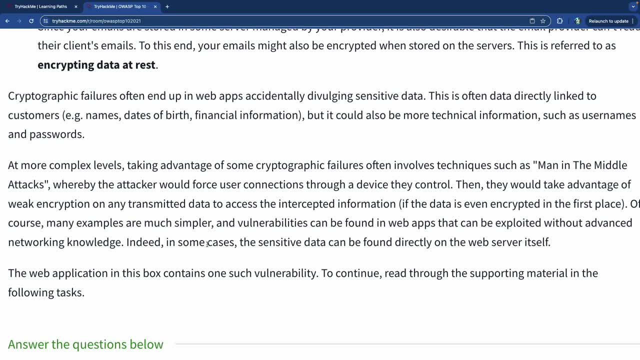 let's say, if you use something like that to encrypt your data, you're just asking for people to decrypt your stuff and and break into your- uh, not just your- your data sets, wherever they're sitting, but log in as your username and do all that jazz that they can finally do. So it is very. 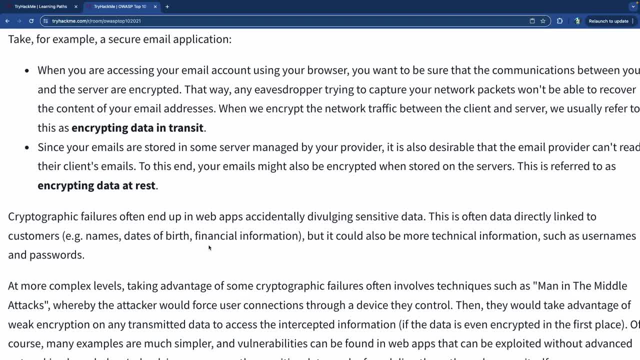 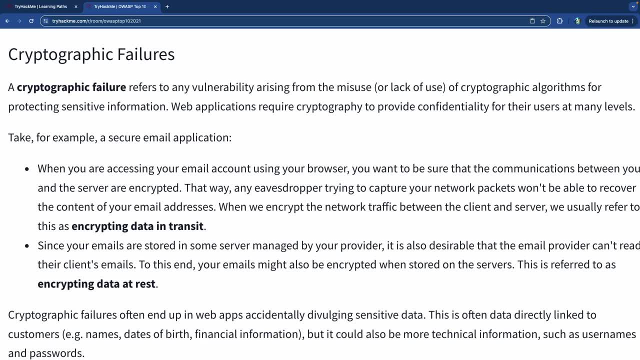 important to make sure that your stuff is encrypted and, uh, cryptography, cryptography, cryptography, cryptography is the concept of encryption of data, So if there's a cryptographic failure, that means it was either not encrypted in the first place or there was a really weak. 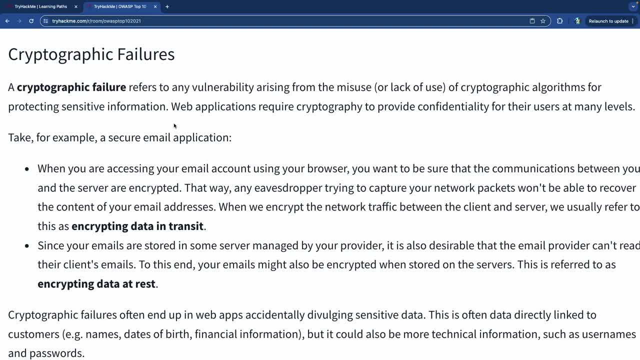 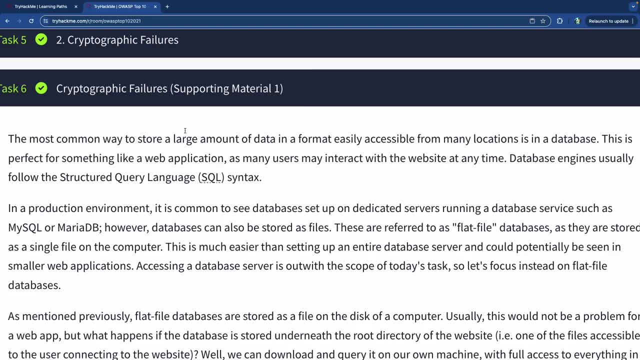 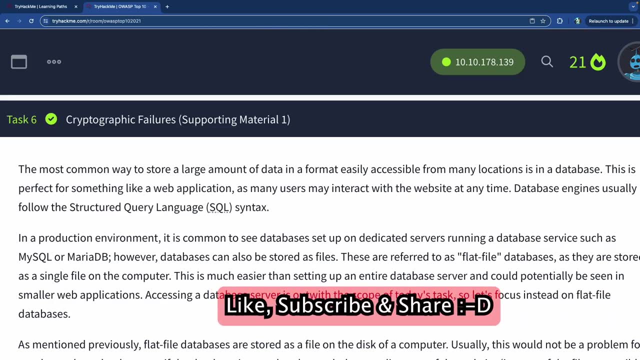 encryption that was used to go ahead and encrypt that data. So let's talk about, or let's actually go ahead and use some supporting material to actually look at some cases, some real life cases of how cryptography can end up hurting somebody. All right, we have two supporting 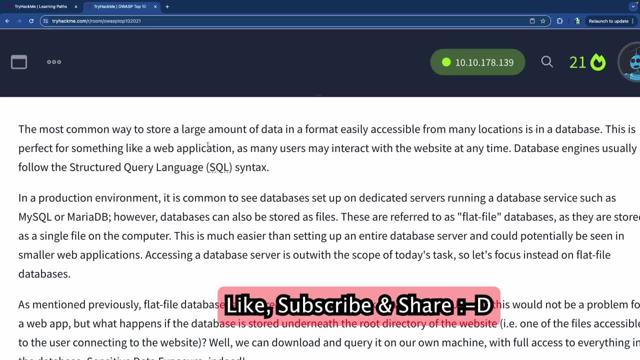 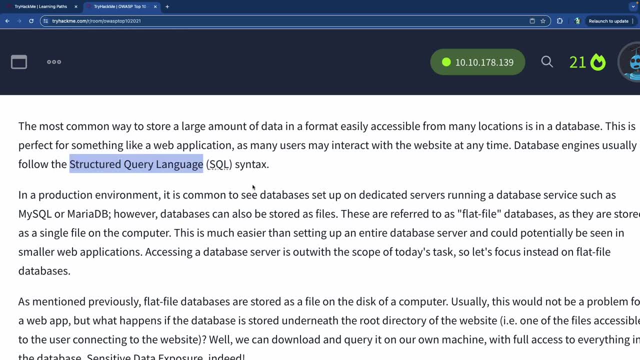 material sections for our cryptography uh exercise, And so the first one just teaches us a little bit about the structured query query language uh, which is called SQL. and SQL is essentially a database language, So it's really easy to store a bunch of data you know large. 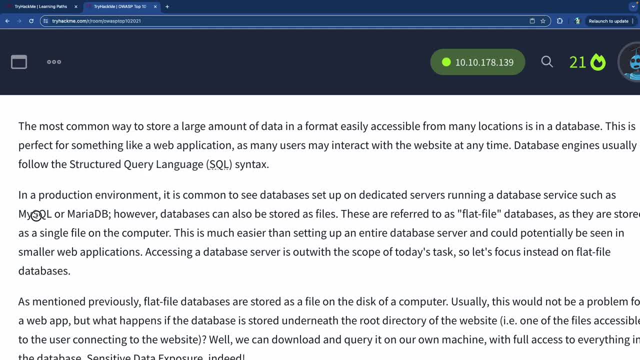 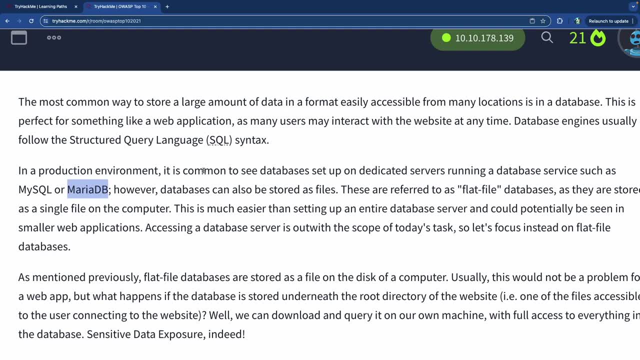 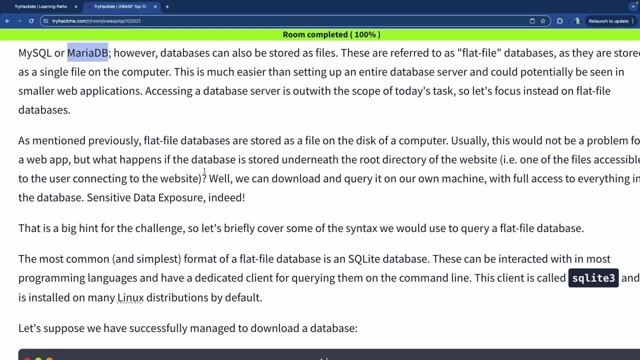 large databases inside of a language like this- And it could be my SQL Maria DB, A lot of these things use use the SQL uh syntax or type of language, And so once you understand the general concept of how SQL works, you can essentially parse through large data sets and find the type of data that you need. 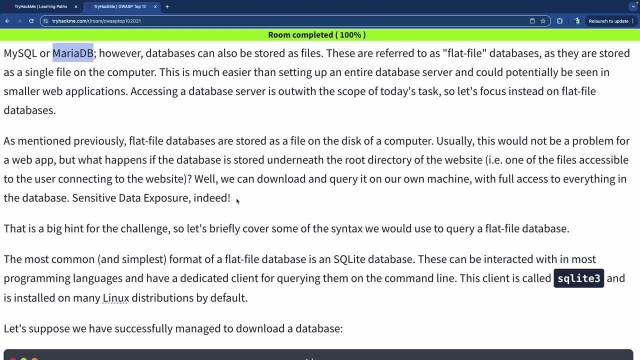 And this is done very frequently for a lot of just normal business activity. But if it's not properly secured, then as a hacker, as an attacker, somebody can go and, you know, parse through that data and find really really sensitive. 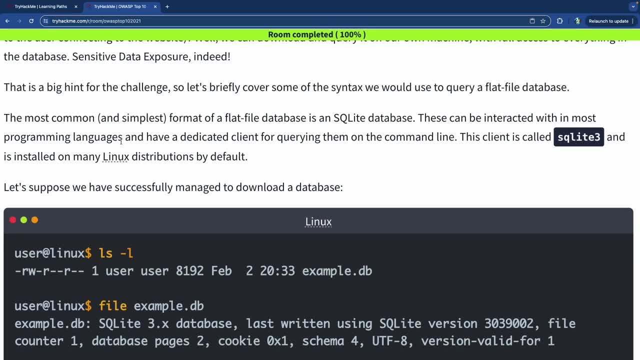 information. So, uh, an example of this would be what we're going to be doing just, or what we're looking at right here. So there's something called SQ light three, which is basically a client that makes it very easy for you to use the command line to parse through databases And, in this particular, 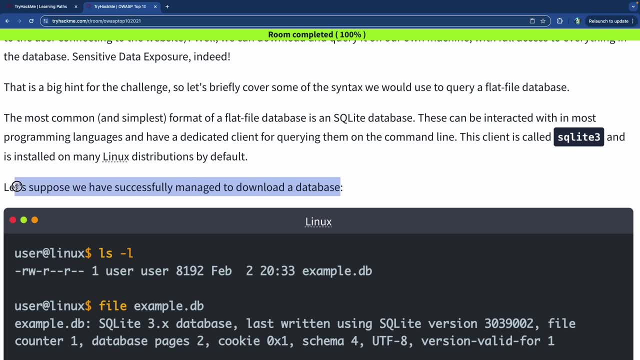 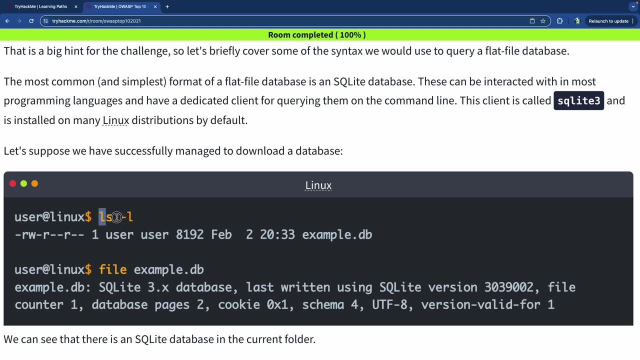 case you know, we've uh downloaded a database. So we have some kind of database file that we were able to download and it usually ends with dot DB And so if uh LS, I mean I'm not going to go. 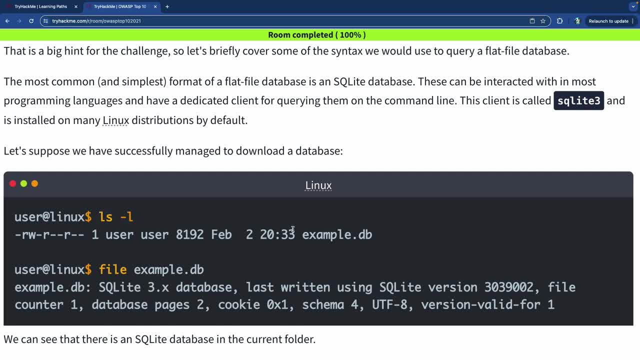 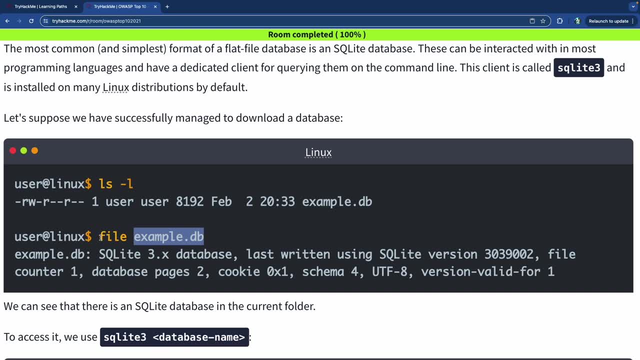 through basic Linux commands here. but uh, I'm going to be doing a little bit of a little bit of Linux commands here. but running an ls command they found that there was a database file and so then used file example db just to see what kind of file it is. so when you use that file it shows. 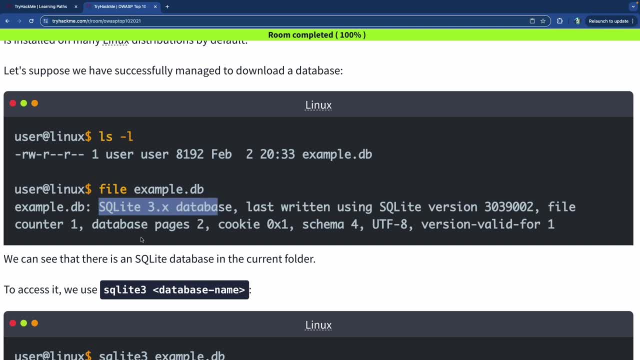 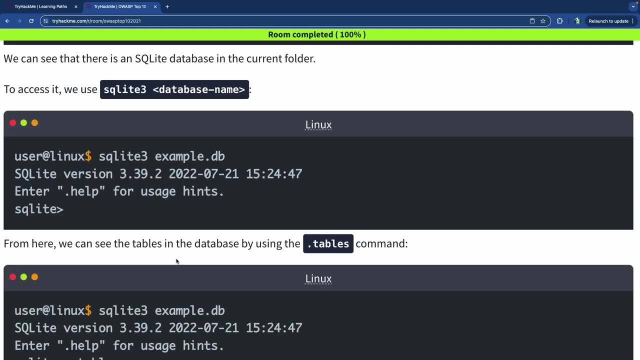 you what kind of file you're dealing with and it says sqlite 3.0, such and such, and so, since it's an sqlite database, you can just use sqlite as the command, including the database name, to be able to get some information. and so when you do sqlite 3 and then use the database name, it actually changes. 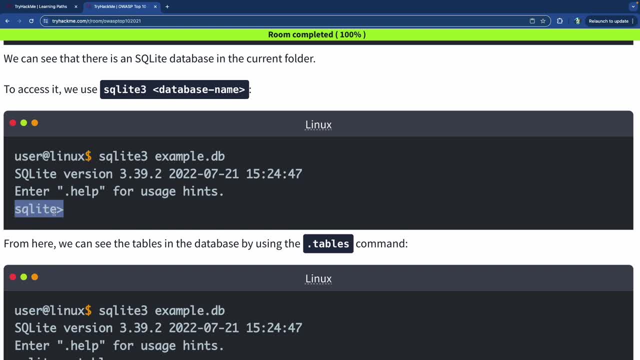 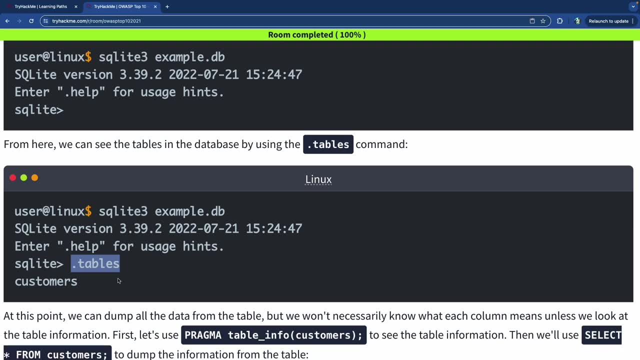 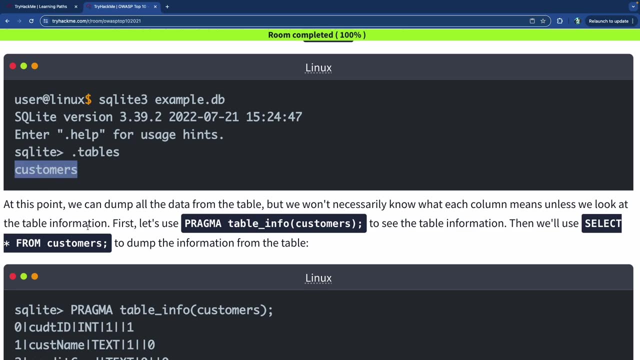 your command line from your user to the sqlite command and then from there you can start doing some really interesting things. so if you just do dot tables, it'll show you where all the tables exist inside of that database. so in our example database there is a table called customers and 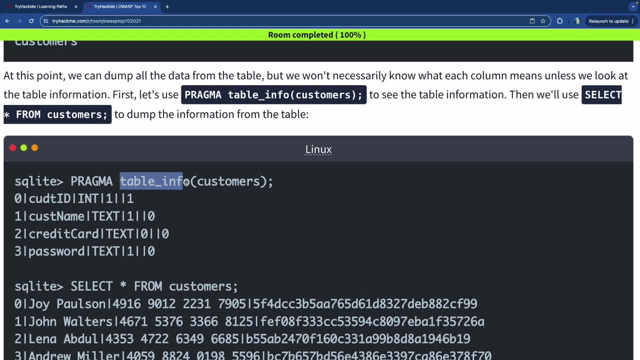 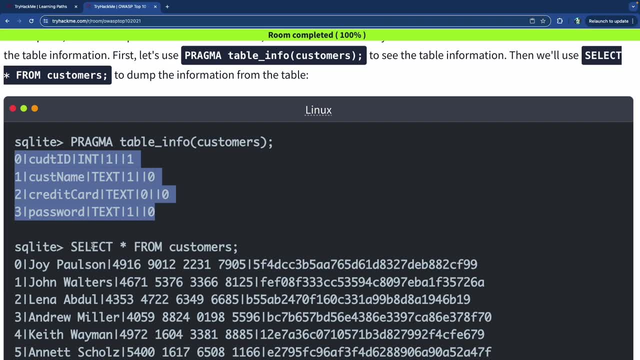 then from there you can do a pragma table- info customers- and it gives you the breakdown of the columns that are inside of this table and in this case we see that table 0, which is the very first column, is the customer ID. then you have the customer name, the credit card information of the customer and the password hash of the customer. 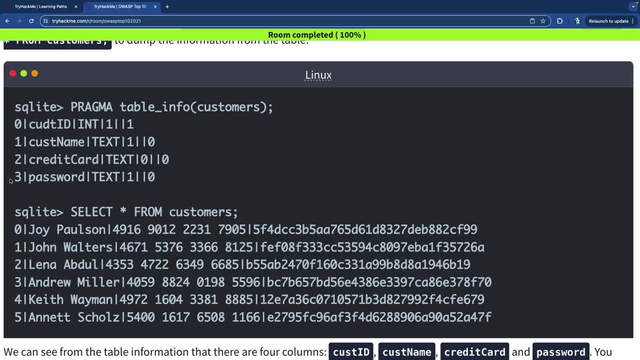 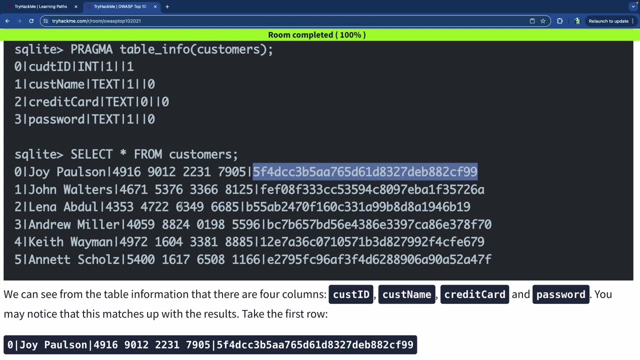 so when we're looking at this, you know column 0 is the ID, so 0, 1, 2, 3, etc. column D: their name is joy Paulson and enjoy Paulson's credit card information is this, and then their password, hash, is this. so, having all of this information, you can now do some. you know, nifty little. 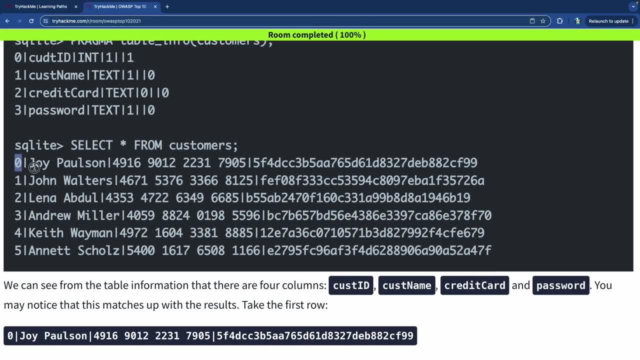 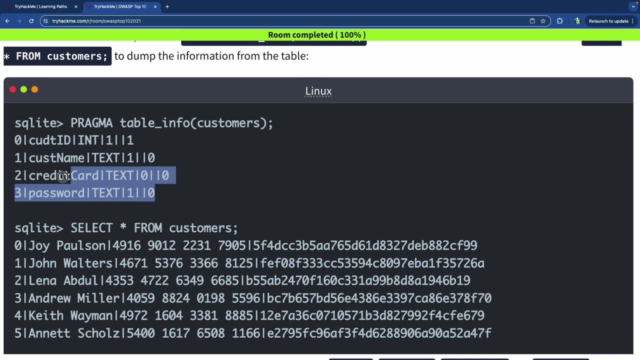 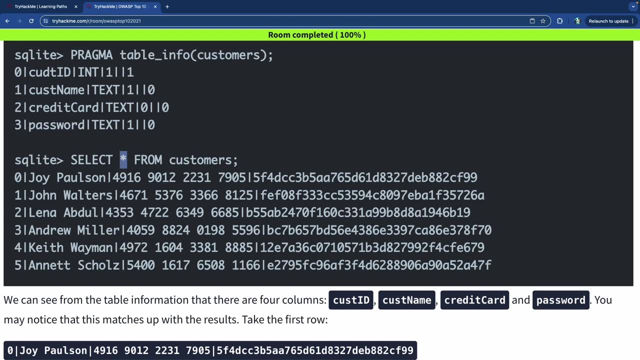 hacks here against any of these users here, and all it took is for us to first run the pragma table info command on the customers. we got the different information of the table columns and then we run the select everything. so asterisk stands for everything. it's a wild card character. so you want. 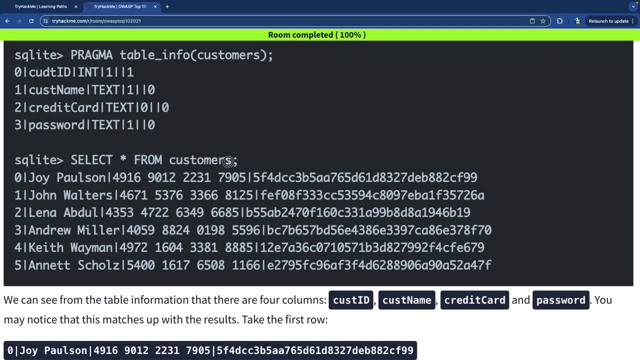 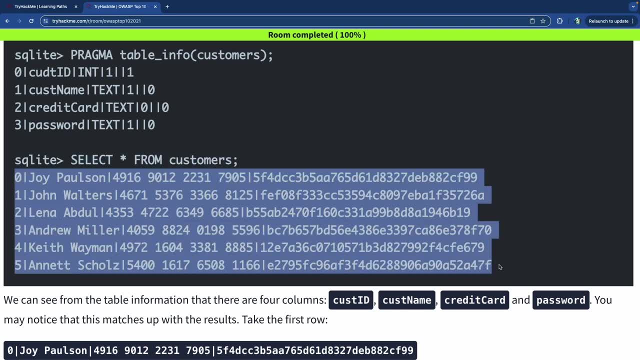 to select everything from customers, right, a very, very basic SQL command, and so you want to do everything from that table. and it gives you a very, very basic sql command. and so you want to do everything from that table and it gives you all the information that is inside of the customers table and just like that, you have all. 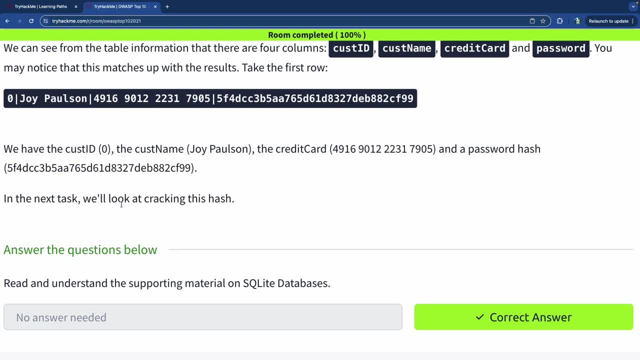 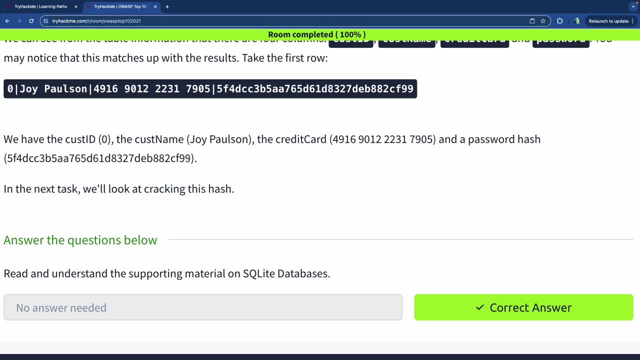 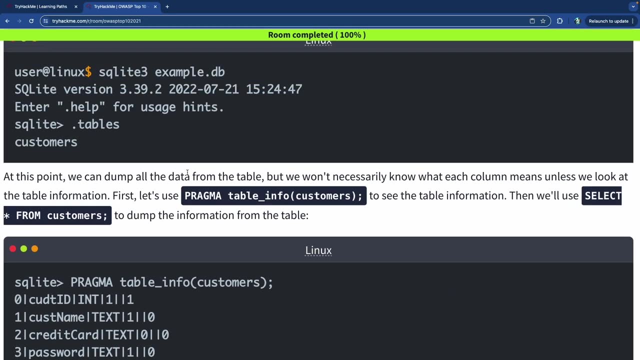 that information and now you can do again some really interesting little hacks. so for this case, we're going to be using some kind of a hash cracker to be able to crash or crack Joy Paulson's hash and then probably log in as Joy Paulson and get some other sensitive data. so 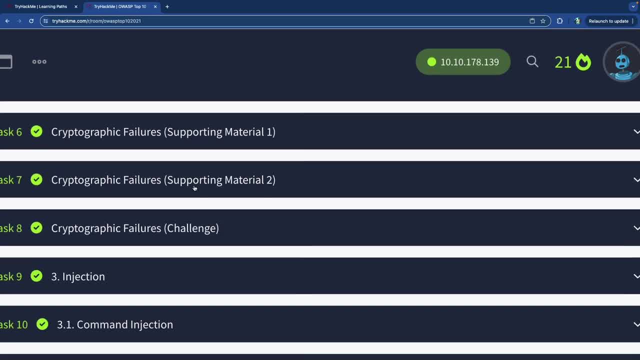 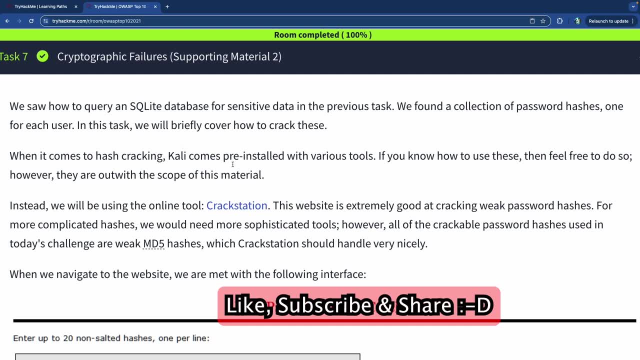 that was the first set of supporting material and we're going to get the second set of supporting, which is basically going to show us how to crack that hash, and the tool that we're using in this case to crack the hash is a website called crackstation, which is absolutely amazing. it's. 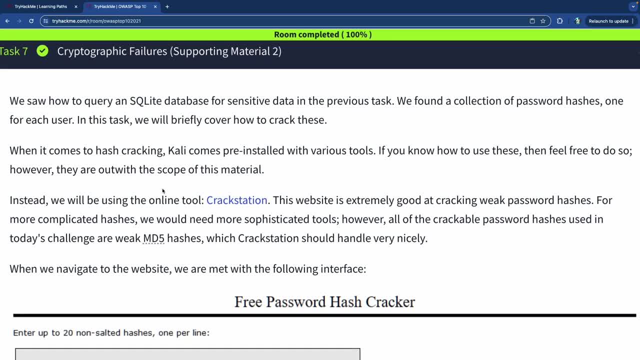 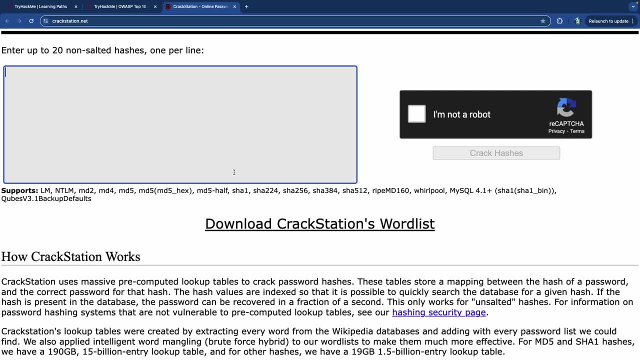 super, super easy to use, and it's kind of scary how easy it is to use. you don't need to know any command line or anything like that, you just need somebody's hash. and so if you go to crackstation at the bottom right here or in the middle of the page, it shows you all of the different. 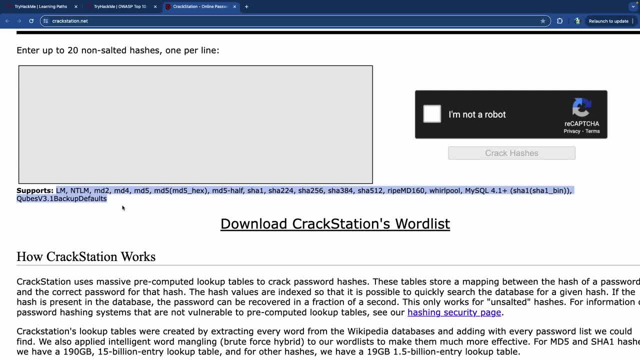 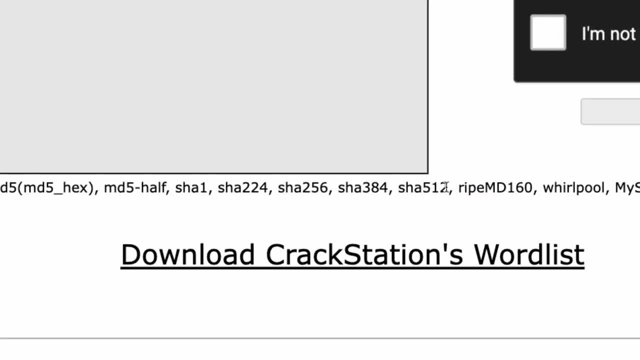 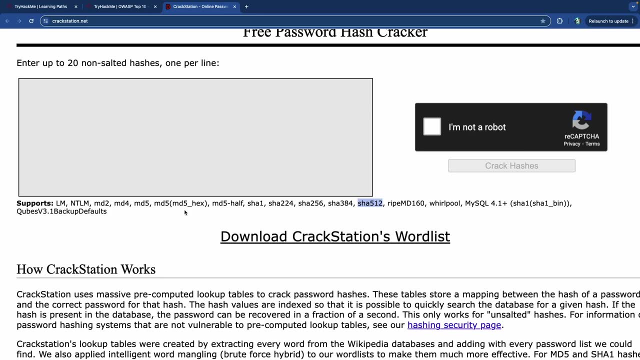 encryption algorithms that it supports, that it can decrypt for you and some of these things right here are very, very secure. so a shot. 512 encryption algorithm is a very, very strong algorithm. but what's important to understand here is if you have a weak password, that password is 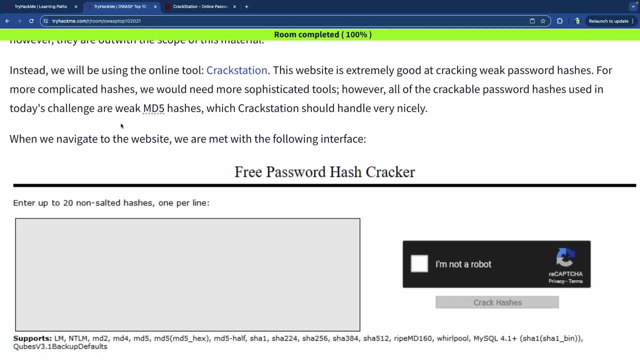 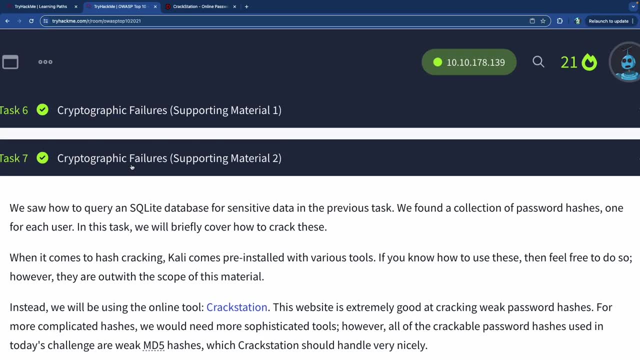 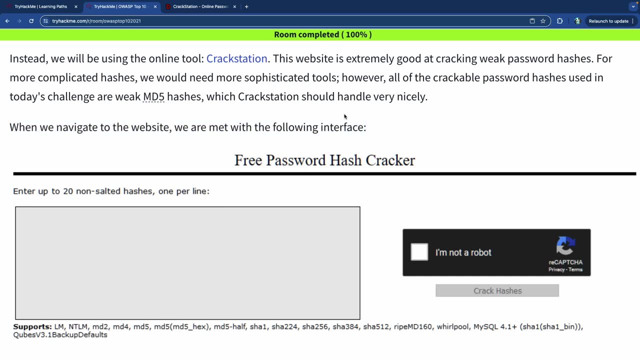 most likely stored inside something called a rainbow table, and a rainbow table is essentially a list very similar to, uh, uh, you know the, the sql database type of a list, where you have on the on one column you have the password hash, on the other column you have the clear text word associated with that hash. what we need to 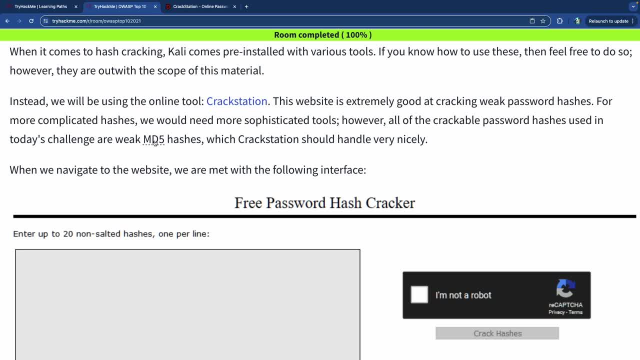 understand is that you can't decrypt a hash by itself. so unless you have a database of stored passwords, for example the rock you password list, which is 15 million passwords stored inside of this text file that's available for free- that you can't decrypt a hash by itself. so unless you have a database of stored passwords, for example, 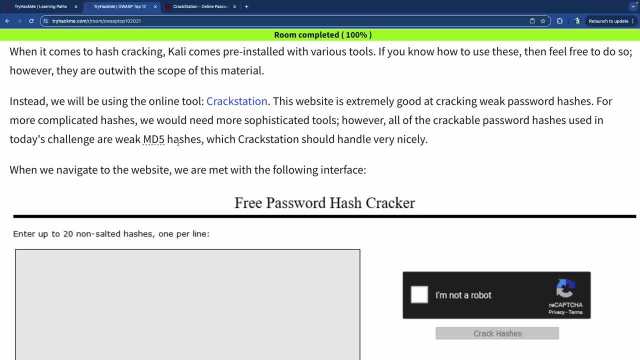 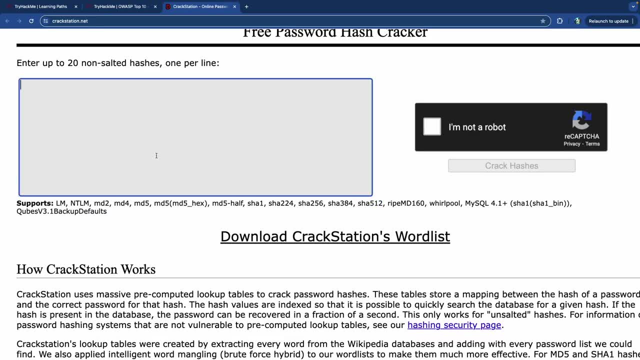 anybody can get, and unless you have something like that, you can't just go and decrypt a hash. the way that crackstation works is that they already have a large database of password hashes that have been stored, and they also have the clear text version of that password hash. so 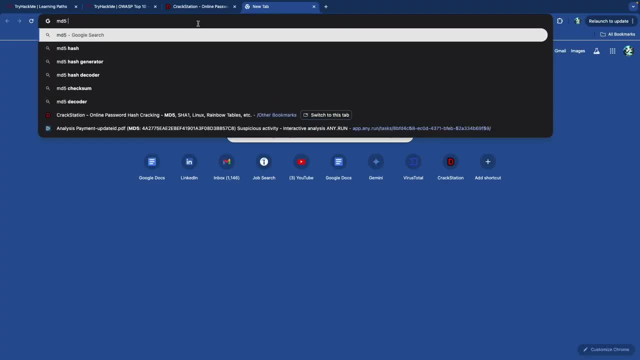 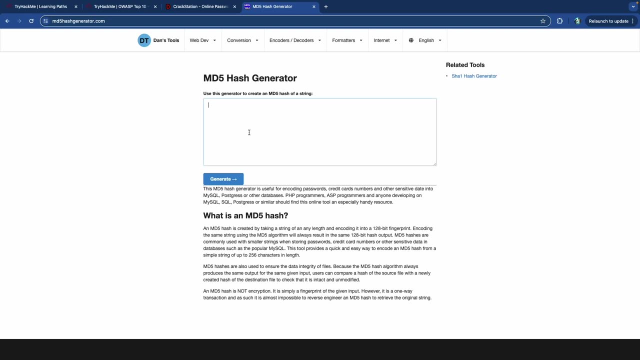 for example, we're going to do a md5 hash generator and i'm just going to show you what this looks like. if you wanted to just create a weak password versus a strong password, so if i use the word password as my password, okay, and i generate that, then it gives. 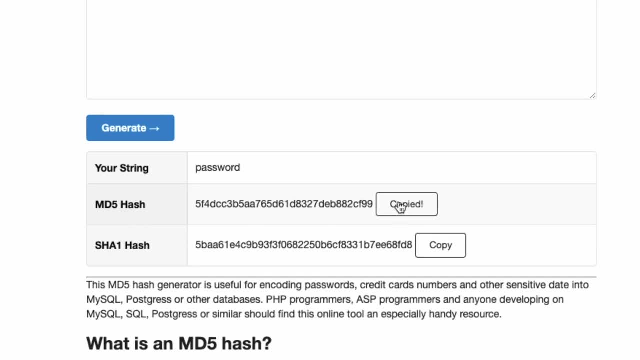 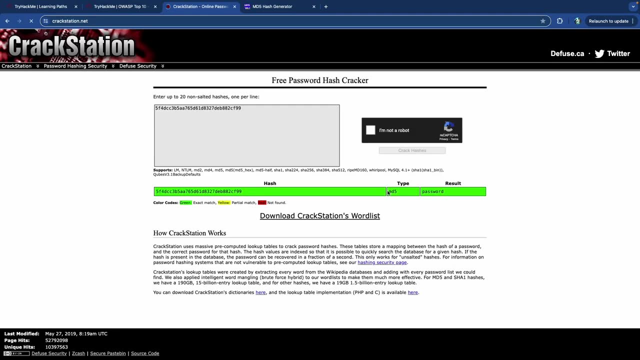 me my md5 as well as my sha1 hash for this. so if i go and copy this and i put this inside of crackstation and then i crack this, it's going to give me the word, because for the word password the hash value is always going to be the same. so whatever the hash value is for a certain phrase, 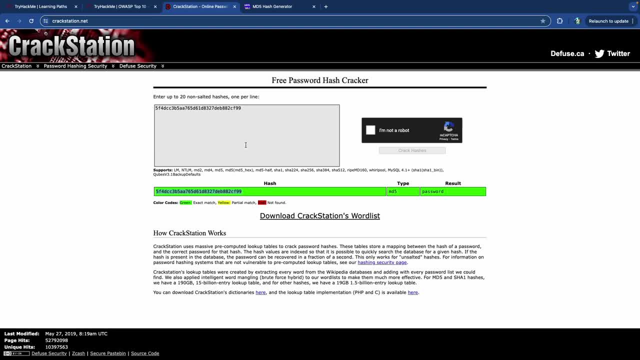 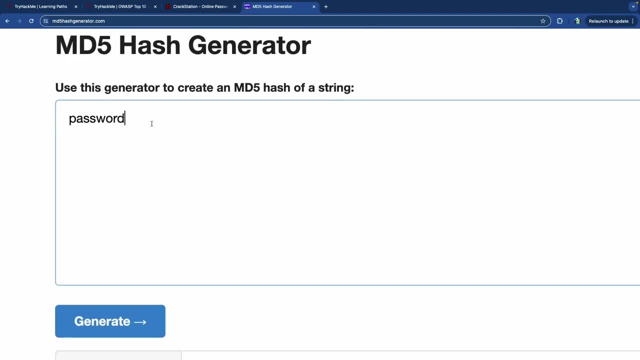 it's never going to change, no matter where you go. so that hash value is always going to be the same. so the hash value is already stored inside of crackstation. so no big deal, right? and if i change this by literally one letter? so even if i, if i don't even change it by a letter, if i just change, 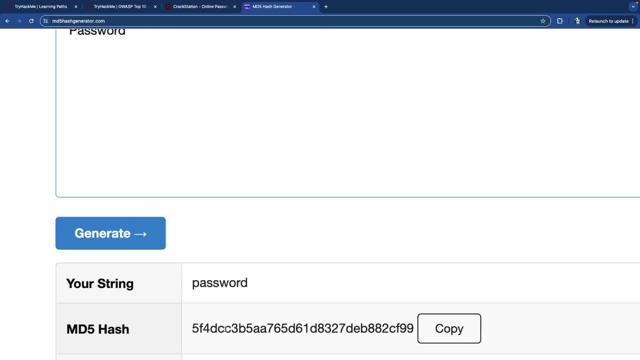 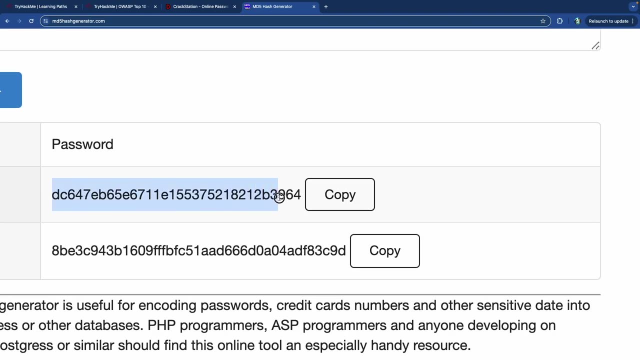 the first letter into a capital p and i do generate hash. so pay attention to this hash right here. we do generate hash and then the hash value completely changes. it's no longer the same hash. and all we did was we just changed the first letter of this thing, and so if i copy this again, 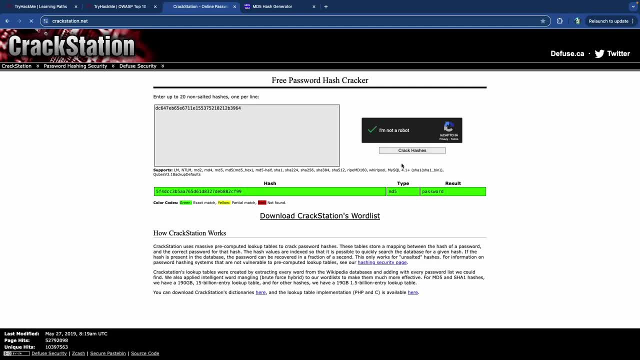 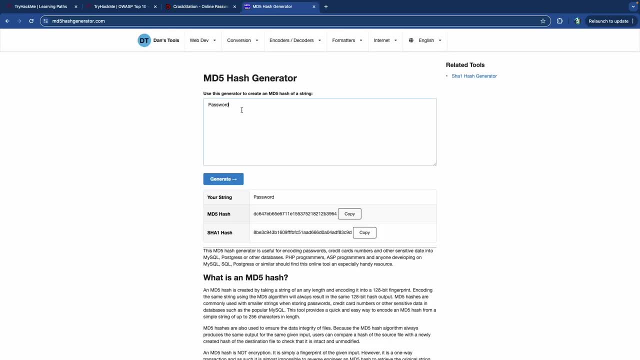 and if i go here and i paste it in here and run the crack hash, it's going to show me the the clear text password, because password with a capital p is still a very weak password and it goes for any variation of this. if you use dollar signs instead of s's, if 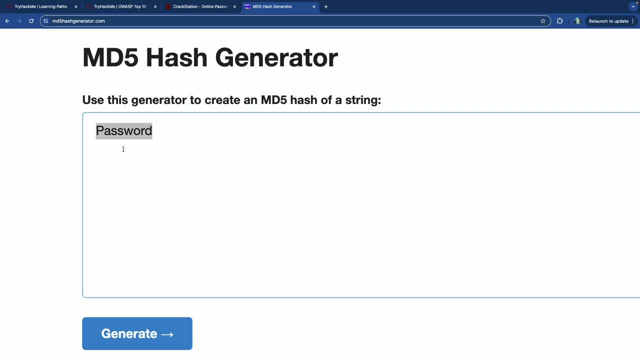 you use a zero instead of an o. all of those things are all stored inside of the rainbow table of a website like crackstation. now, if i use this as an example, so let's do this- is a strong password: one, two, three, four, five, six, seven, eight, nine, and then we'll do this. so let's say this is my. 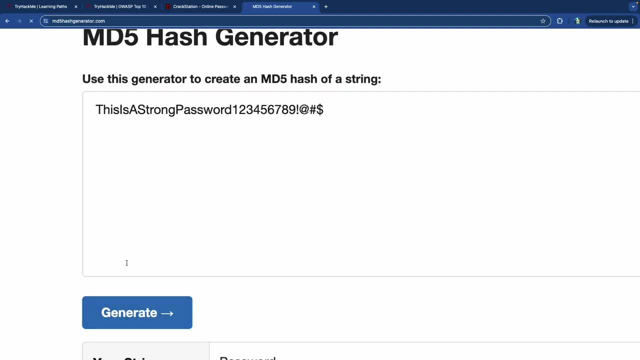 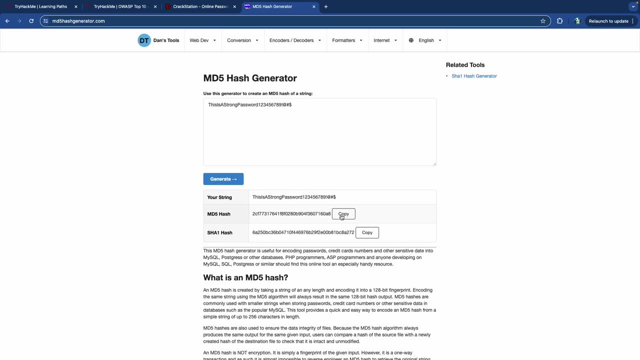 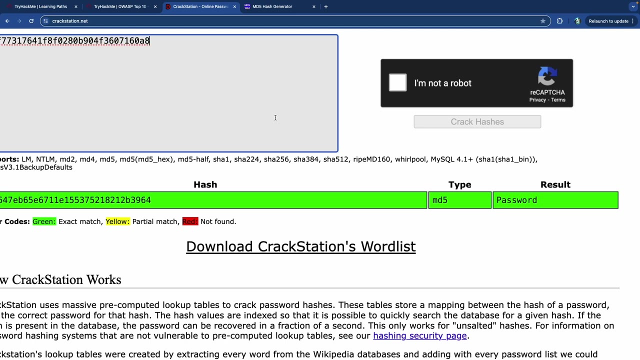 password right, crazy long password and it should not be stored anywhere inside of crackstation. so if i go ahead and take the hash value for this, so let me copy this real quick- so if i take the hash value for this and then come to crackstation, i should get an error message. so hopefully, 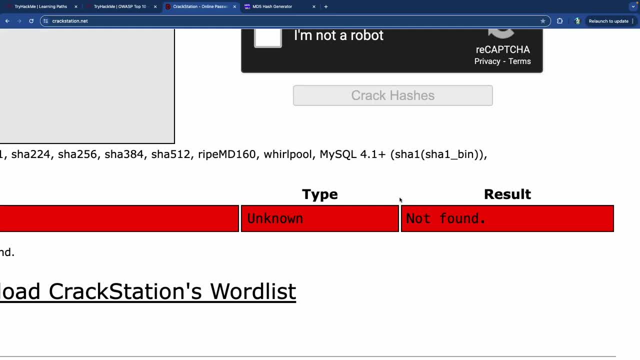 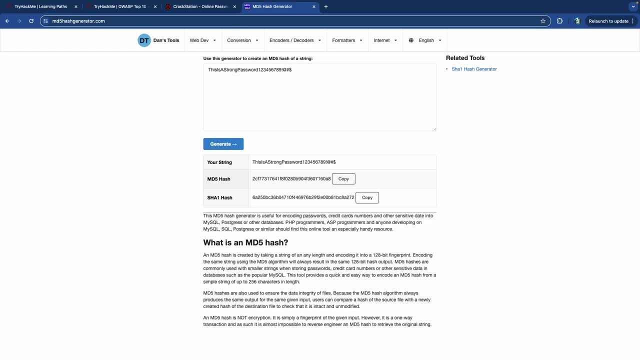 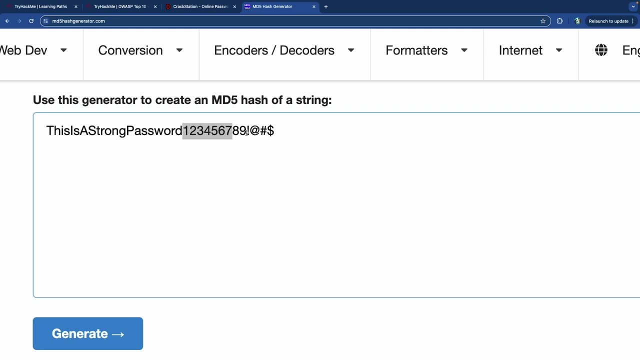 nobody has ever used that password. yeah, so now you get an error message because within their database, within their rainbow table, there is no previous password that's been stored. that is this long ass. you know. every first letter has been capitalized. there's a bunch of numbers in it, there's some special characters in it. so this super long password no longer. it doesn't. 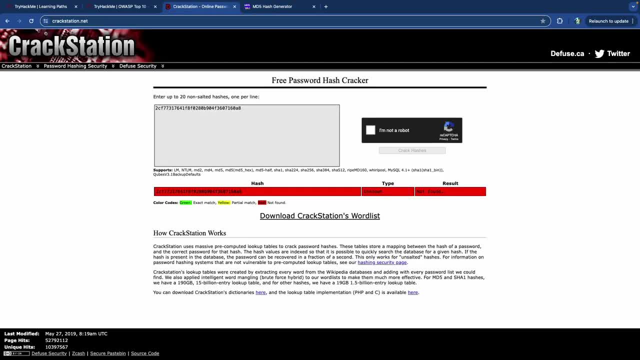 exist in any password dictionary online. so therefore, crackstation can't find it for us- and this is how important a website like crackstation is- and knowing how to use it, so they're not going to decrypt the hash value for you. what they're doing is they're comparing against the data set. 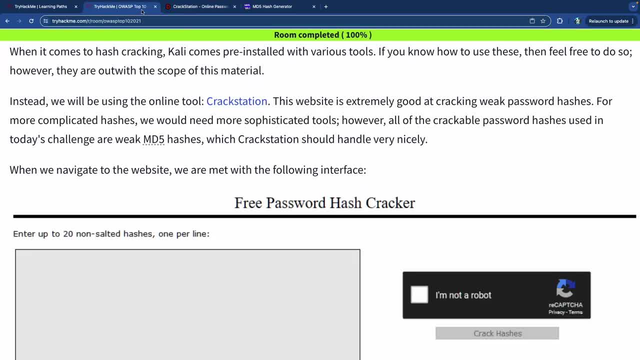 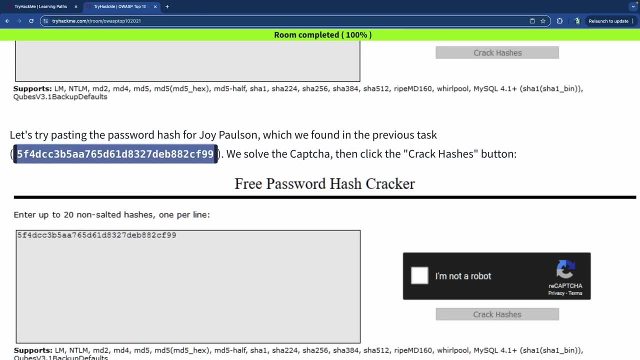 that they already have to see whether or not that password already exists in their data set, and then, if it does, they show you the result of it. so that's how crackstation works. so now what we're going to do is we're going to decrypt this specific password. 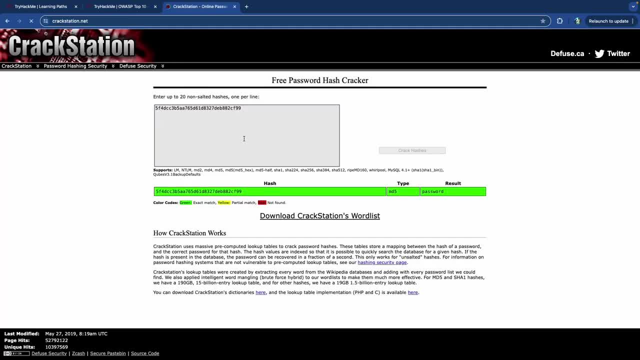 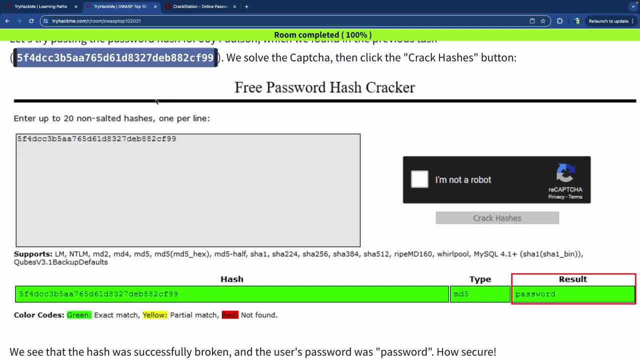 hash that they gave us the same way that we just did right here, and then we're going to look at it and so that it's literally actually the password that we used before, so it's the word password has been saved over there as a password here, so you can. this is how you use crackstation. now there's. 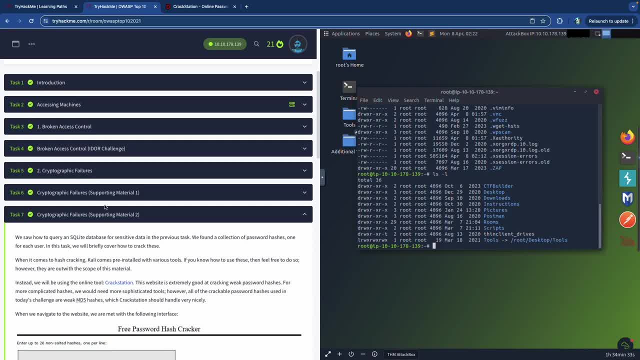 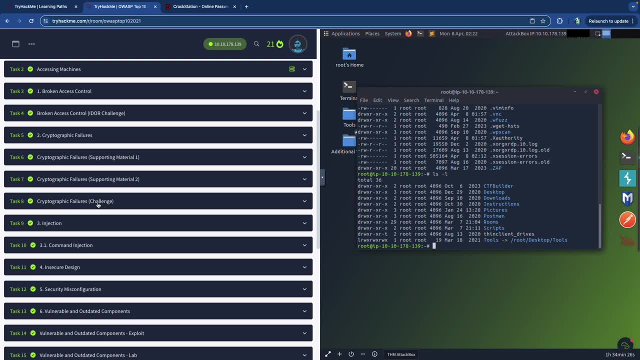 a bunch of different command line tools that you can also use to decrypt hashes or decode hashes, I guess we can say- and something like John the Ripper or hash cat or cane enabled. there's a lot of different tools. Hydra, all these things. there's a lot of different. 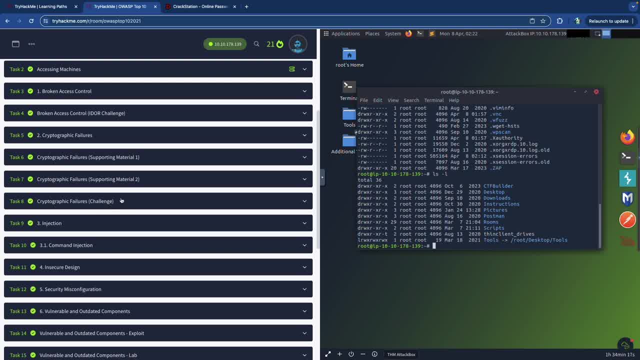 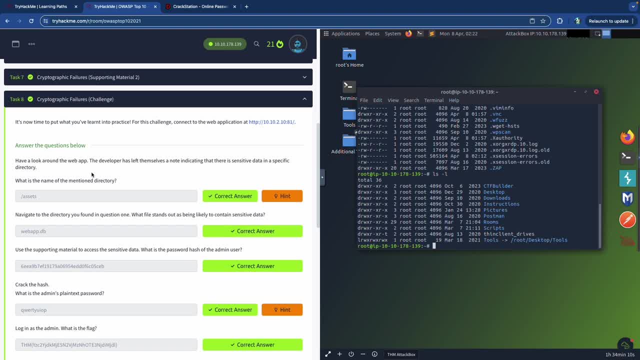 stuff that you can use to decode or decrypt a hash value. so that's the supporting Mary, the supporting material. two for cryptographic failure. so now what we're going to do is we're actually going to go through a challenge and we're going to find some of the hash values that we can use and decrypt in. 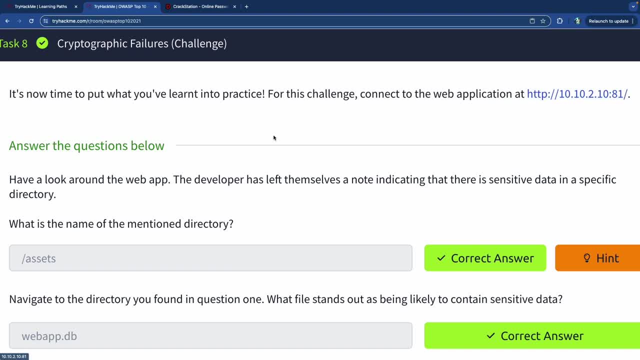 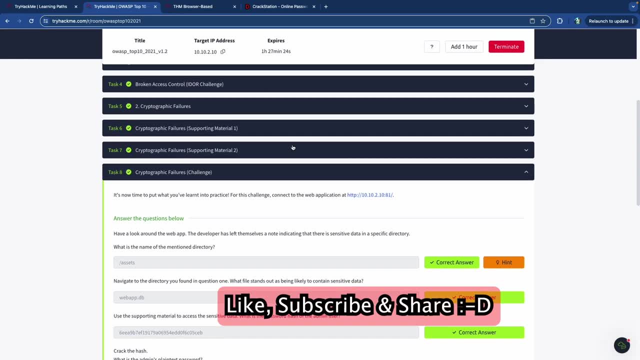 a particular case when it's attached to this specific website right here. so let's go check that out and have some fun with that. all right, I am now on this link right here, the 1010. I just opened it up in a new window just to make it a little bit easier for us to analyze, and it says: 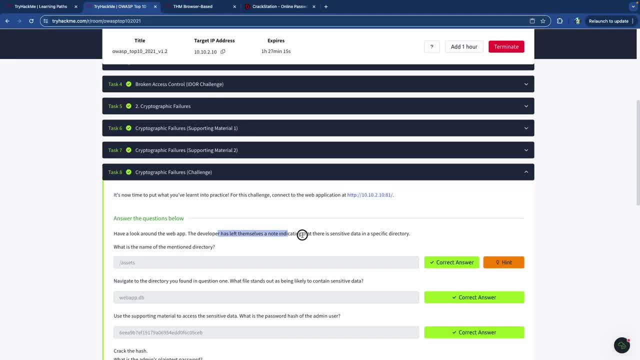 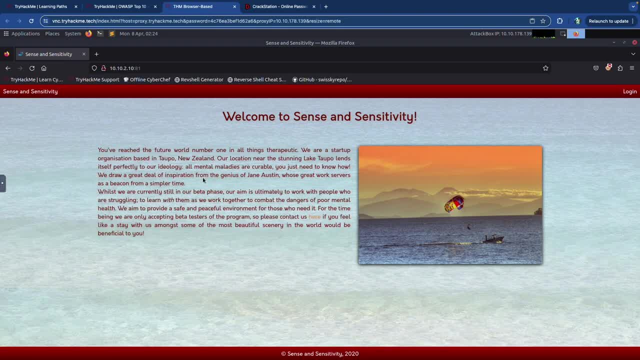 right here in the question one, it says that the developer has left themselves a note indicating that there's sensitive data somewhere. so in order to be able to look at the developer's notes, we literally are going to just look at the source code of the page and through all the browsers you can do this if you just right click on the page as part of the 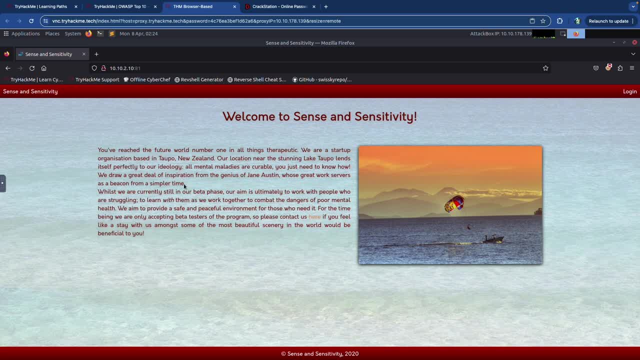 right click menu, the little thing that pops up. it shows you an option called inspect or view source, something similar to those lines. it just depends on which browser that you're using, that the, the text or the command for that is going to change, but essentially it's along those lines where you. 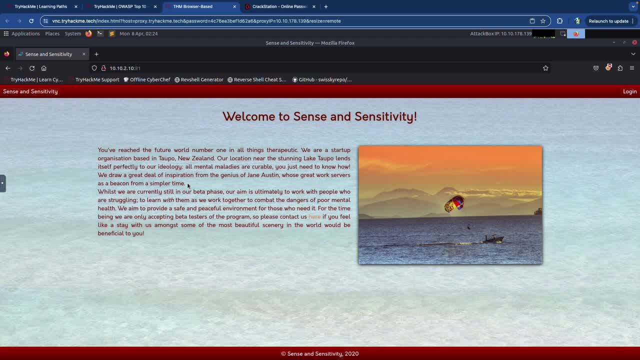 can either inspect the source code of the page or you can view the source- something along those lines- and then, once you do, you'll be able to see what is the actual source code of the page and then, within the source code of the page, you can see what the developer has. 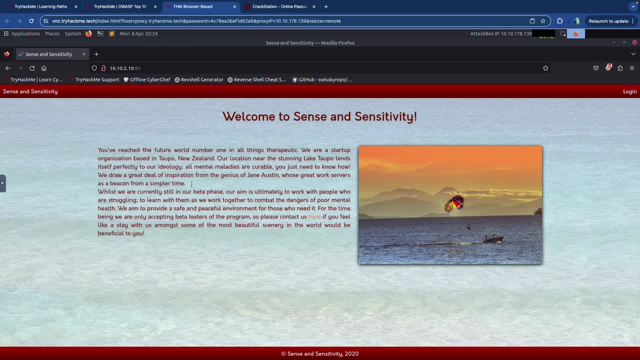 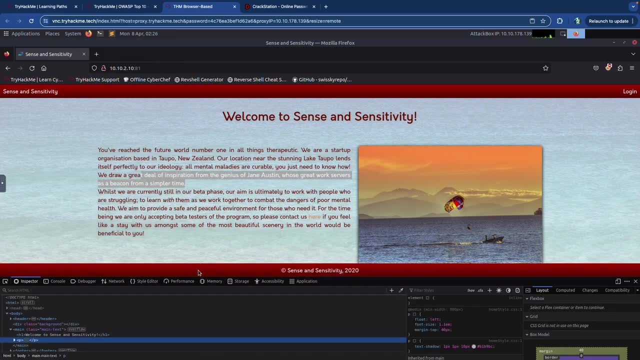 left for themselves as any kind of a note. so we're going to do that here and then from there we're going to try to find the developer's notes. all right, and this is what it looks like. so I'm on Mozilla and when I did the right click, it gave me an option called inspect, and that's what it does. 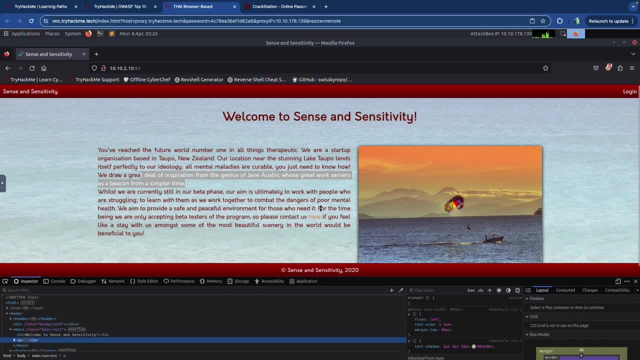 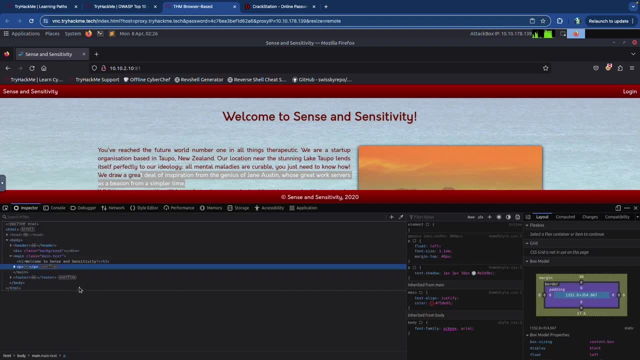 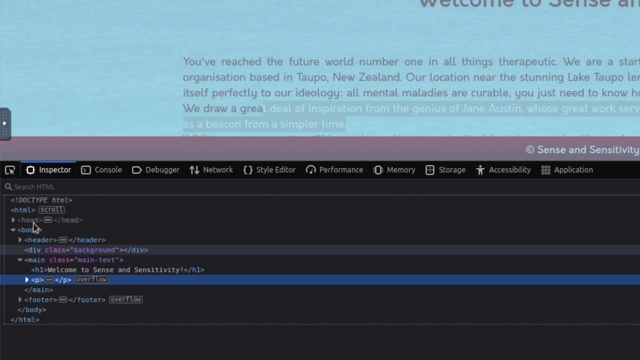 it shows you basically, literally, the source code of the page, and now we want to scan this source code that's at the bottom right here to try to find the information that the developer has left for themselves. so let's see what we can find inside of this source code here, all right right off the bat, inside the header. 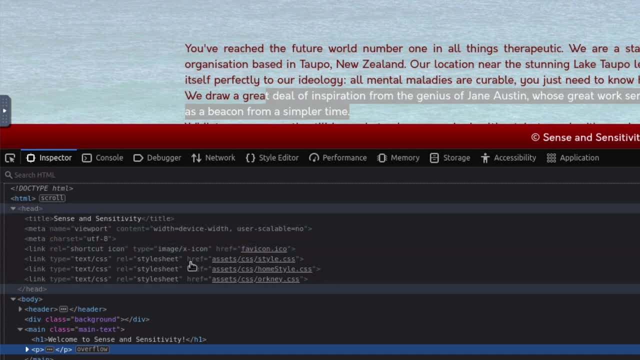 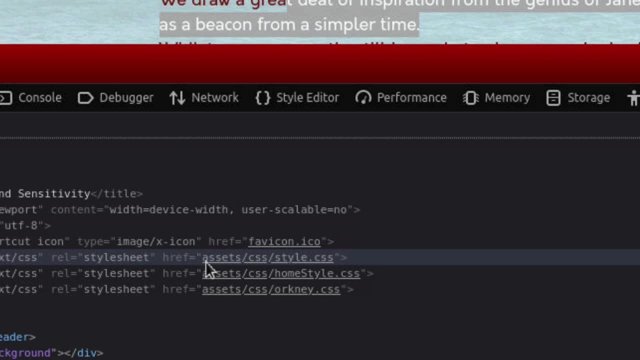 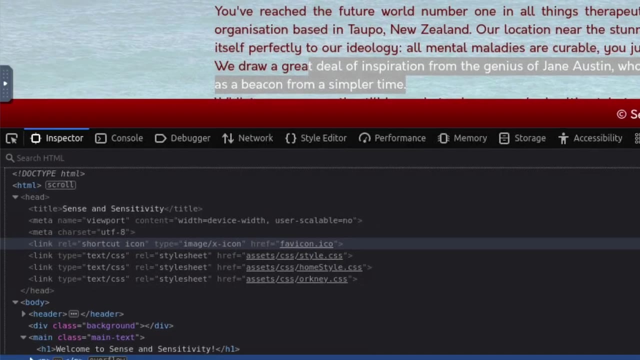 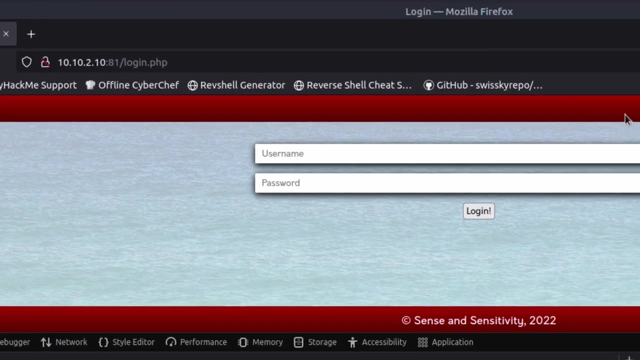 information or inside the head part of the code. there is just something that seems a little bit interesting is the assets folder, so href equals assets style CSS, home style CSS, so assets, just from here. it just stands out. let's see what else we can find here real quick. all right, so it wasn't on the home page, but when I go to login I just 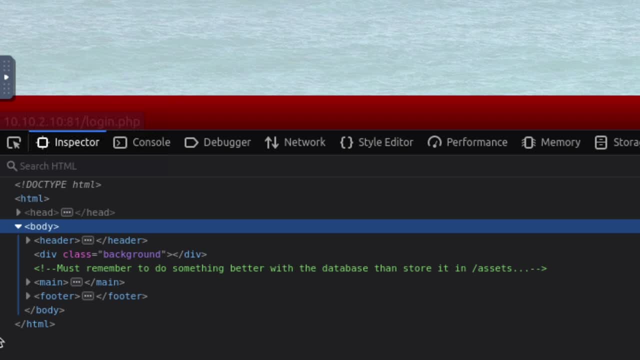 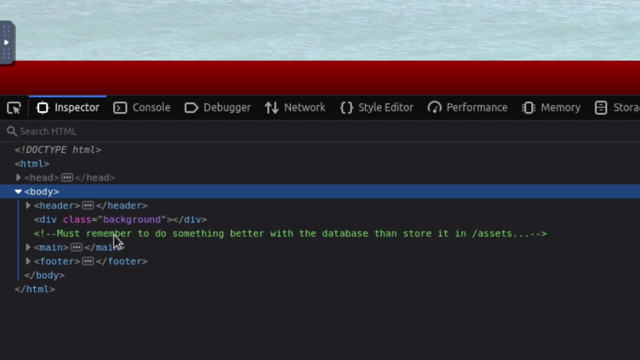 literally click the login button at the top right here. there is a note right here by the developer and it's been commented out so you don't actually see it on the web page itself. but it says: must remember to do something better with the database than store it in assets. so the database 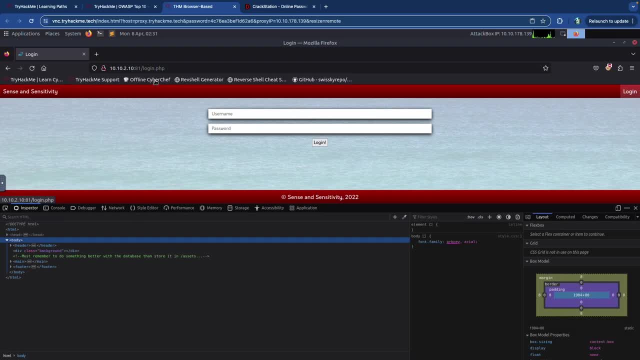 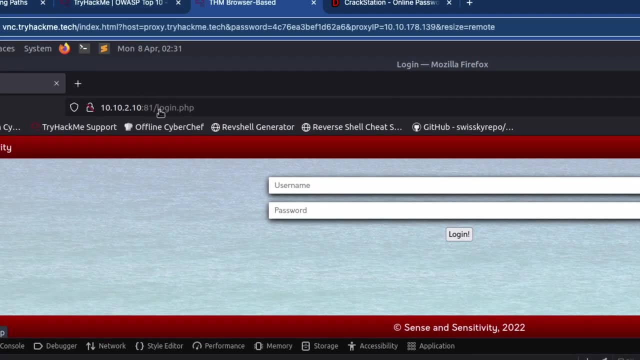 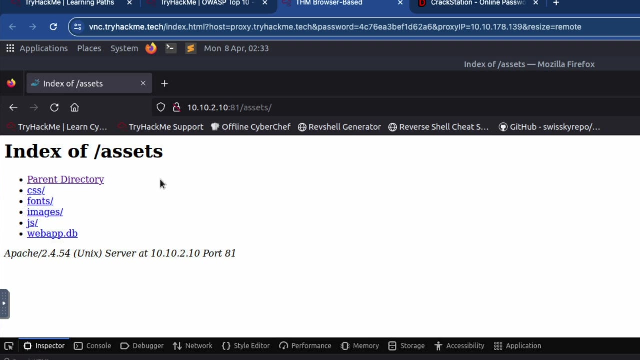 is stored in assetsphp or assets forward slash. so, uh, now what we're going to do is we're going to go inside of the assets directory, inside of this web page, and see what we can find in there, and here we go. so we are now in the assets directory and there's a little DB file. there's a database. 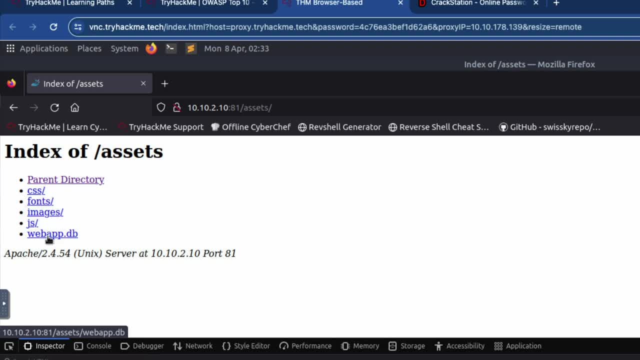 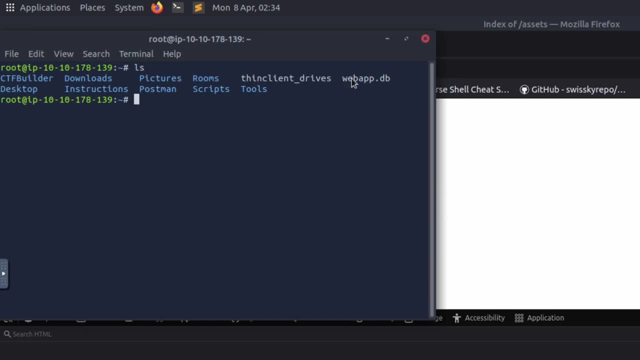 file here that I am going to click on and see what I can find in there. all right, when we click on that link, it downloads the file for us, the webappdb file. so what we're going to do in this case? we're going to literally do the same thing. 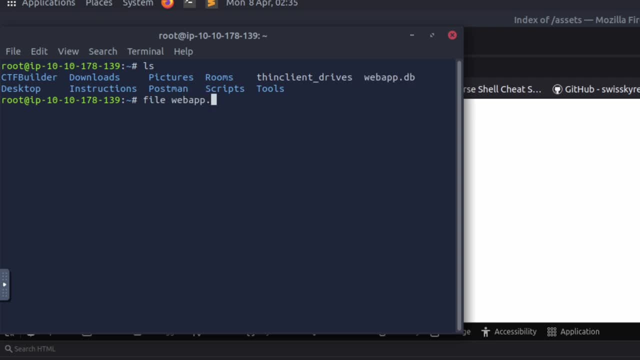 that they showed us in the exercise. first we're going to do filewebappdb to see what kind of file that we're dealing with, and it says that it's an sqlite3, something, something database file. so then I'm going to do sqlite3 and then I'm going to do webappdb. 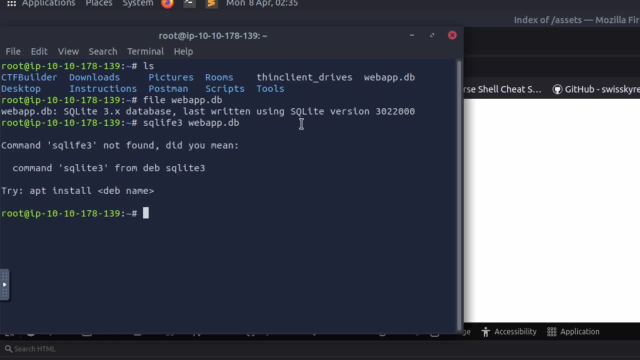 and it's going to open. oops, I did sqlife. there's no such thing as sqlife. so sqlite3, webappdb, and then it's going to go into sqlite for me. so now what I need to do is I need to run that same. 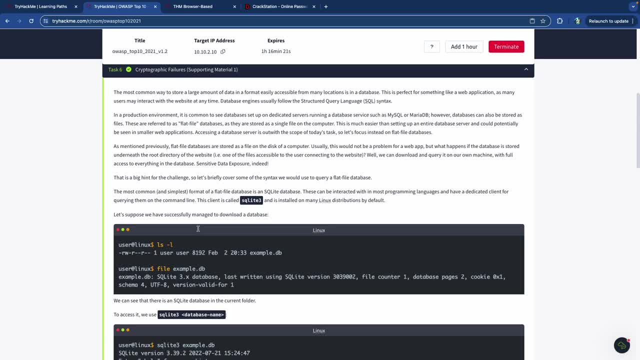 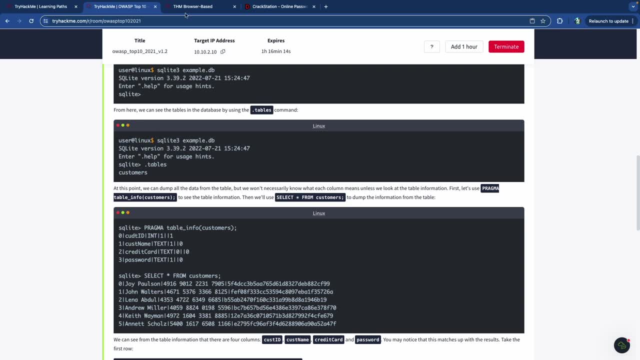 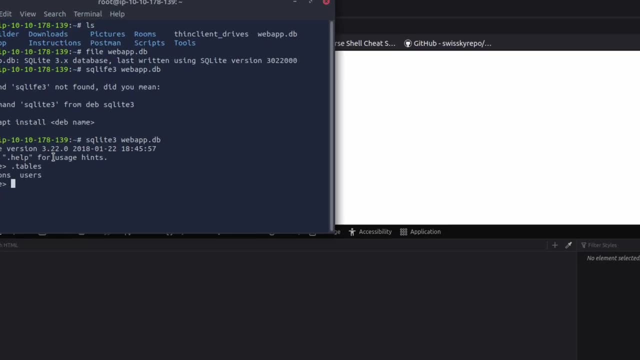 command that we had earlier, which I think it was like pragma or something like that. what is it called? yeah, pragma, pragma, actually. first we're going to do dot tables. so that's what we're going to do. first, we're going to do dot tables to see what is in, what is inside of this thing, and so we have sessions and we have users, those. 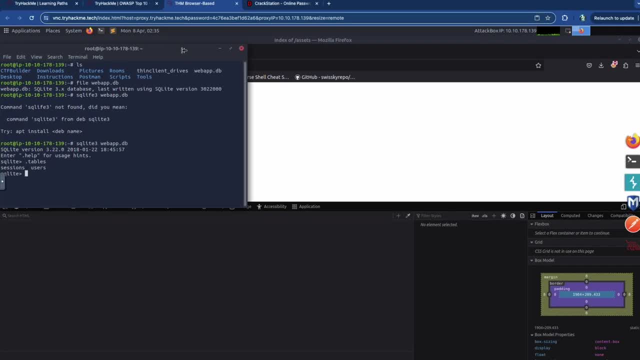 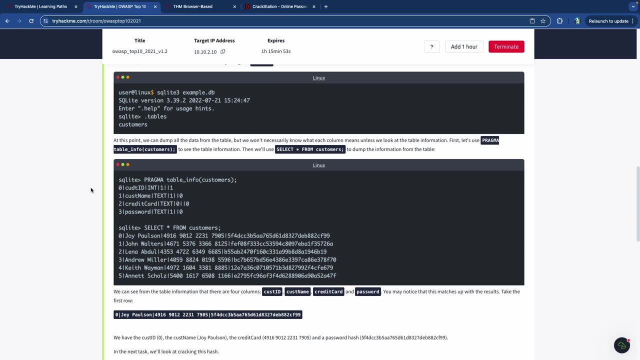 are the two tables that we got in here. let me just bring this to the center of the screen a little bit. so, since we have sessions and we have users, what we really want, based on the questions that they're asking us here, is the information of the admin user. so so far, this is what we got right. so 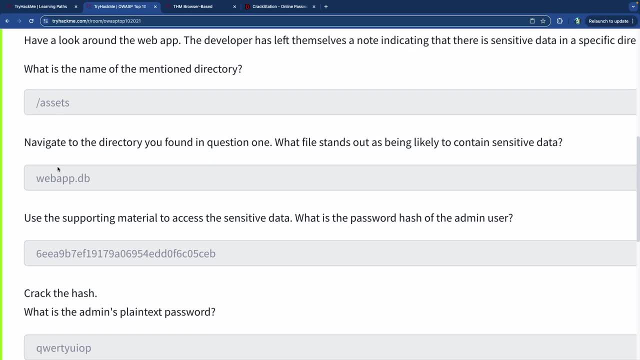 it says: what's the name of the mentioned directory? that's secret, it's assets, what is the file? that's in the database? and then now we need to find this hash value. and of course, you know that that's exactly what I'm about to do. is I'm about to run this pragma code right here, or this pragma command? 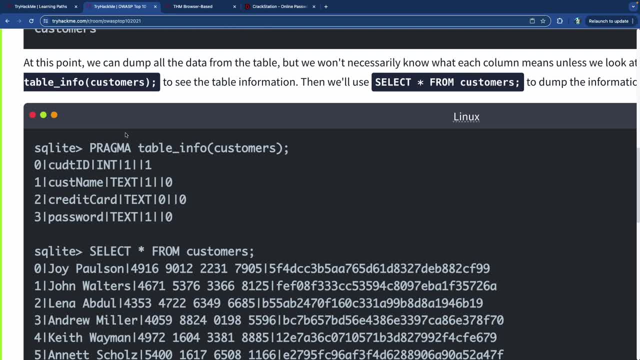 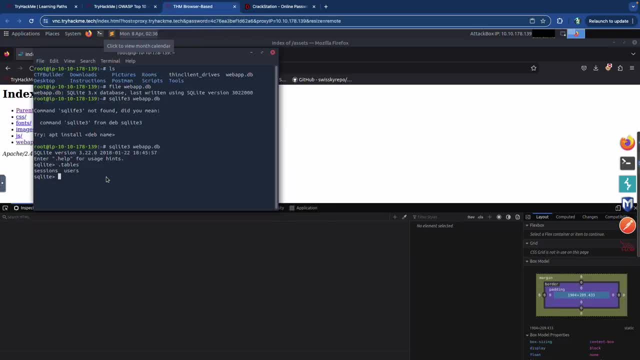 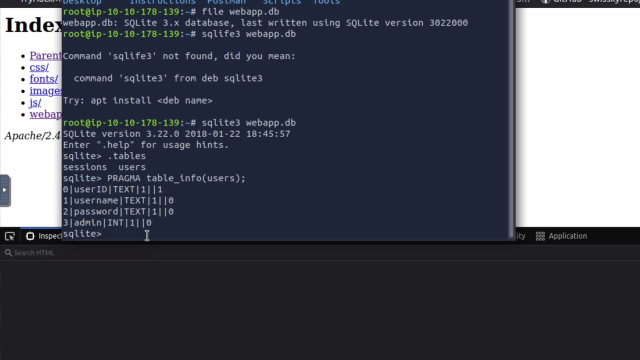 so I have the, the name of the table that I got with dot tables. I'm going to use pragma table information and then get the, the users information of that and then from there we are going to get the info that we need, buddy. so all right, and so these are the columns that we have over here inside of our table users. so we're 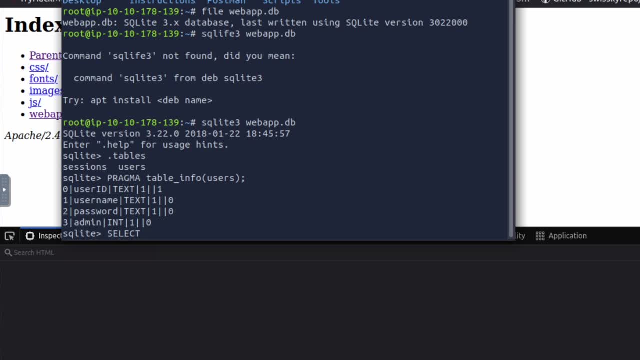 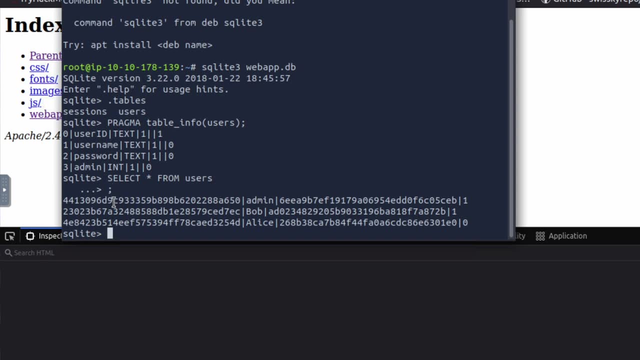 going to run our select everything from users, and there we go. I forgot to put this semicolon at the end of it, so it gave me a new line to finish it, but here it is right. so we have the, the. the column itself is going to have a user ID. 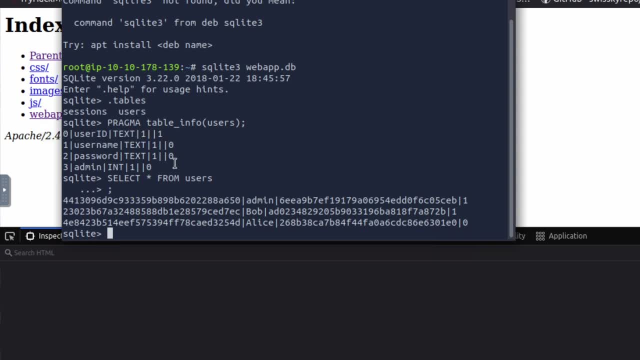 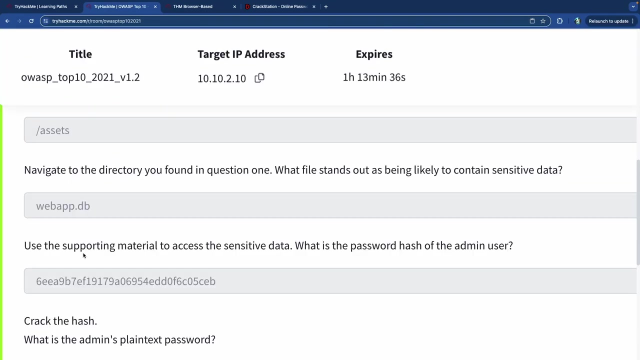 next to it there's going to be some text, and then that's basically it. so you have the, the information right here, you have the user ID and then you got some text and it seems to be that this is the- uh, the, the hash value for the admin user. so let's go and double check that here. and that is indeed. 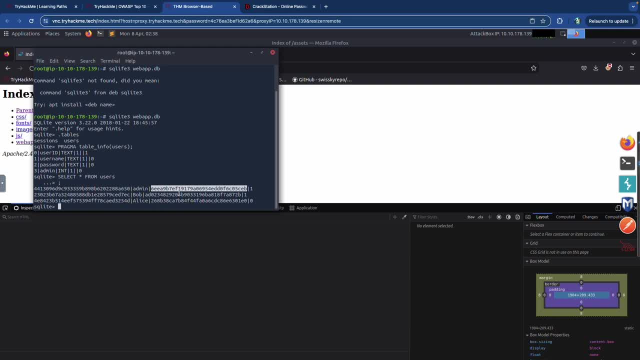 the case, that is the hash value of the admin user. so you know what we're going to do now. so we're going to go ahead and copy this hash value and then from there we're going to go to crack station and crack the darn thing and it seems like it's an 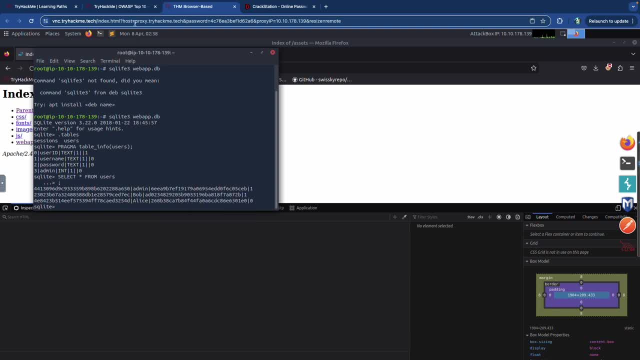 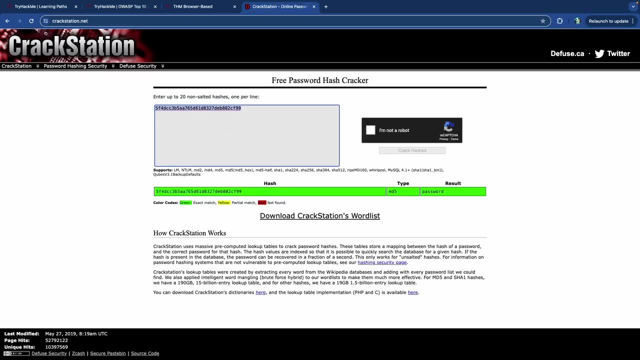 easy one. it's an easy one to crash. so, because of the fact that this is kind of taking uh forever for me to click on it, I'm just going to go and copy it from our answers and we're going to go to crack station, we're going to paste it and we're going to crack this hash and look at that. that is. 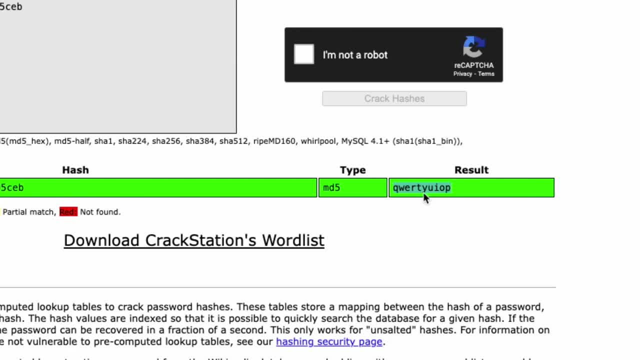 the password of the admin and if you actually look at your keyboard, these are all of the letters that in the top that are in the top row of the keyboard. so it's: it starts with Q and then it just goes q, w, e, r, t, y, qwerty, and then uiop and that's their password, right? so it's not a, it's not any word or anything. 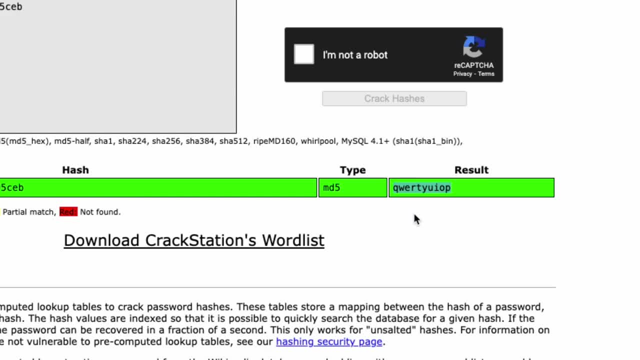 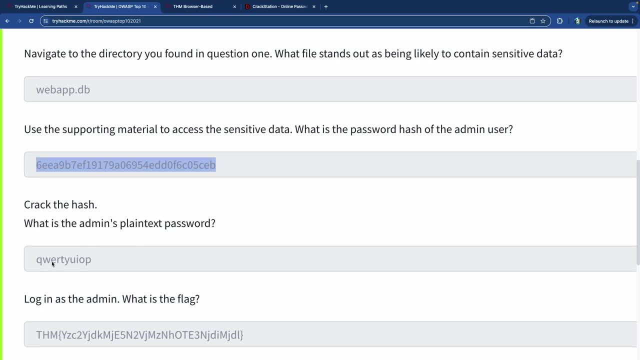 that you would recognize looking at it. but when you see the pattern on the keyboard, you're like, oh, that's, that's a pretty lazy and easy password and just like that, that's the thing. and then so when we crack it, we got qwerty and so now we're going to log in as the admin and we're actually going to get access. 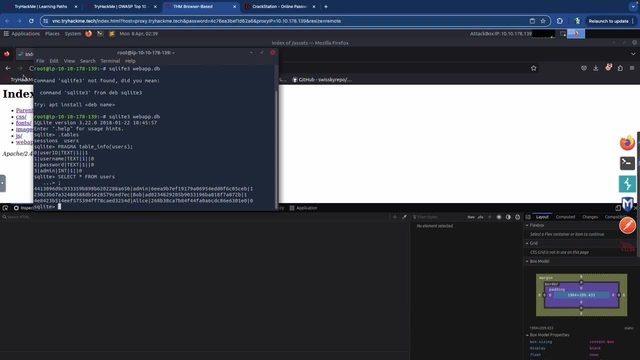 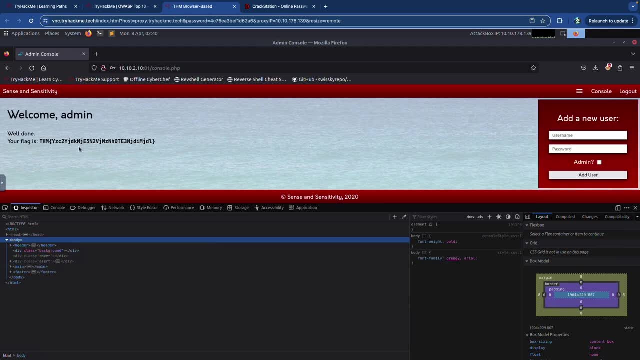 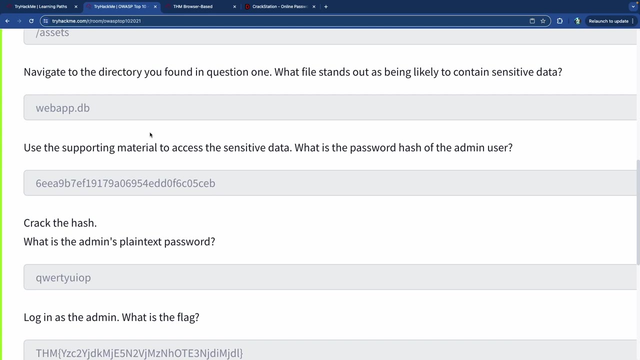 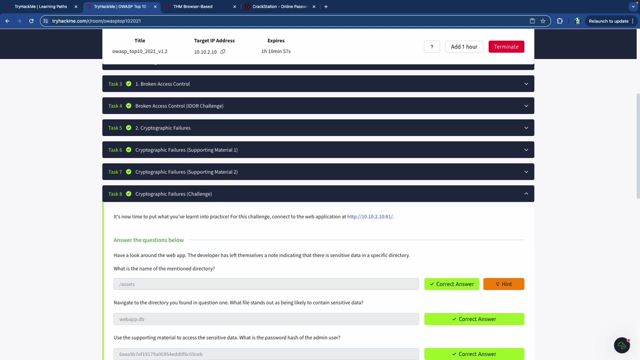 to that information, so easy money. and here we go, there is the flag, just like that, and here's the flag right here. so pretty easy, right, it's not. it's. it's kind of simple, uh, and scary how simple it is to do some of these things and all it takes is for somebody to know a website like crackstation. 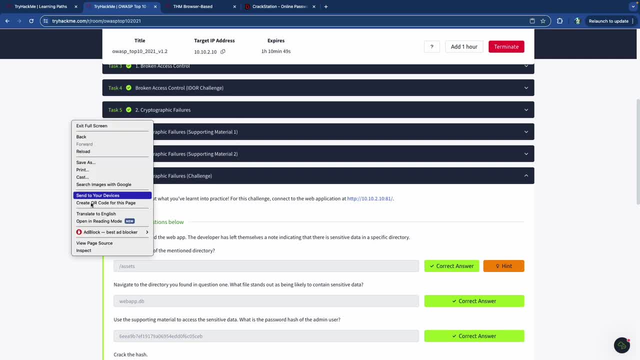 for them to know that they can right click on the web page and go view page source and then get all of the page source data that's on a screen. or do right click on the page and click on inspect and then they get to see all of the data that's on the screen. and if your developer was lazy or 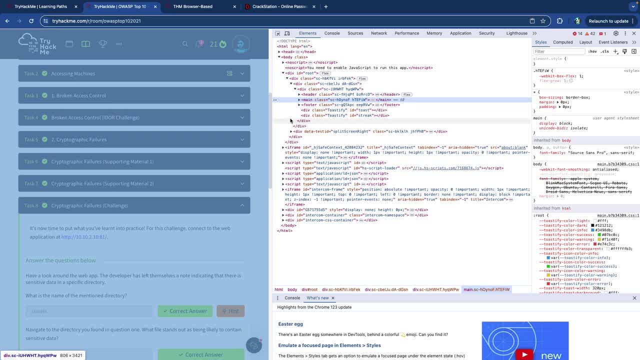 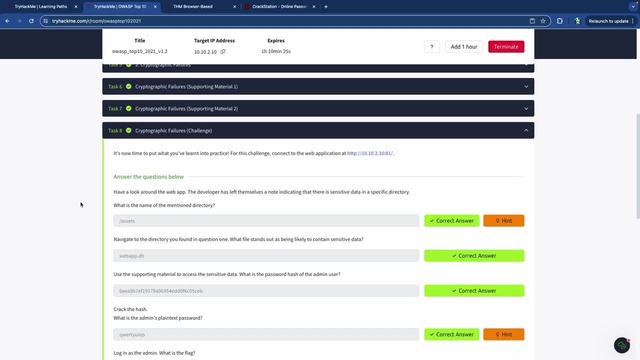 they forgot to delete a comment or something that they left for themselves. that's. all it takes is for somebody to get the information that they should not have access to, and I mean there's a lot of other tools that you can also use to look at the directories that. 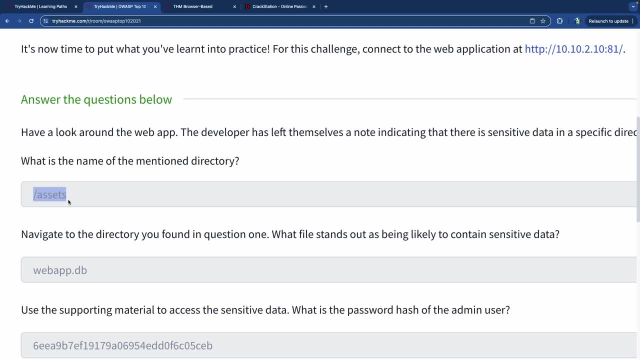 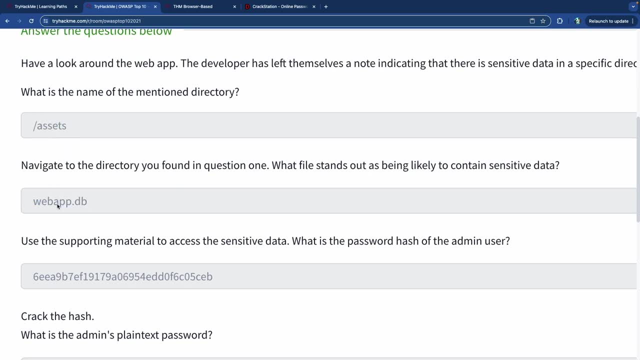 belong to a website, so we could have used nicto, for example, to just scan this website and get the information on the different directories, and then go to that directory and then find this database file. so there's a lot of different ways that you can do this, but this one was a very 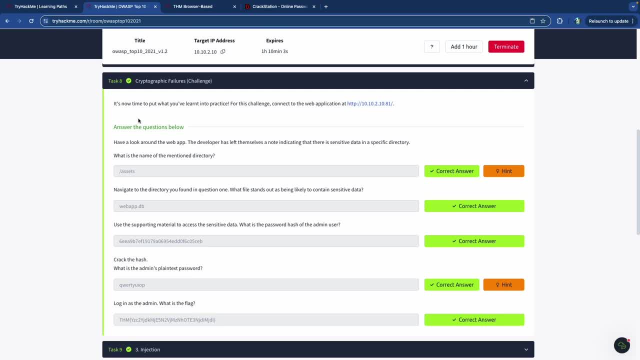 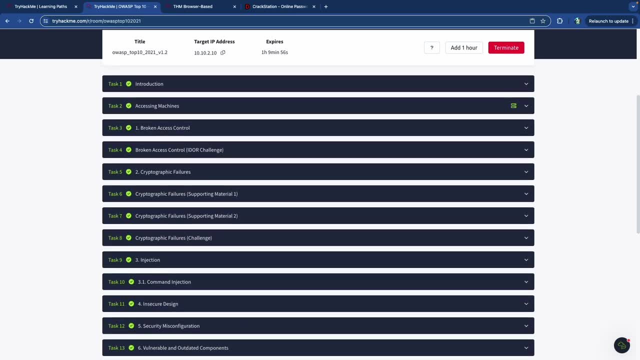 very weak website, obviously, and from there we were able to just do use our browser to go ahead and find some sensitive information. so it's really really crazy how easy it is to do these things and, uh, you know, just bear in mind, as you're doing this for a website or for. 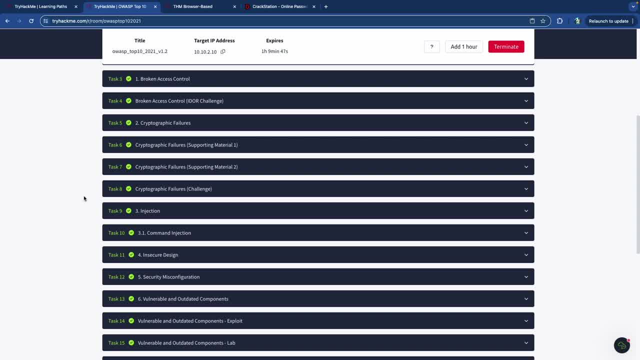 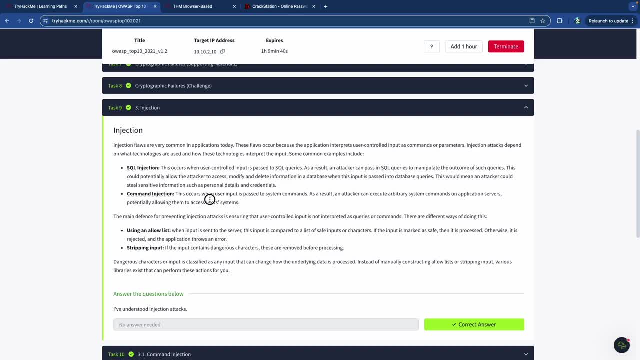 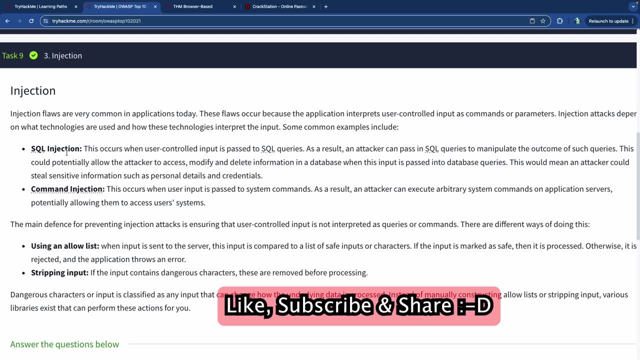 your company, or if you're trying to hack somebody- not not not saying that you should, but if you are. you know it's sometimes it's that easy. so let's look at the injection vulnerability here. all right, injection comes in two big forms. right here you have SQL injection as an. as you already saw, we 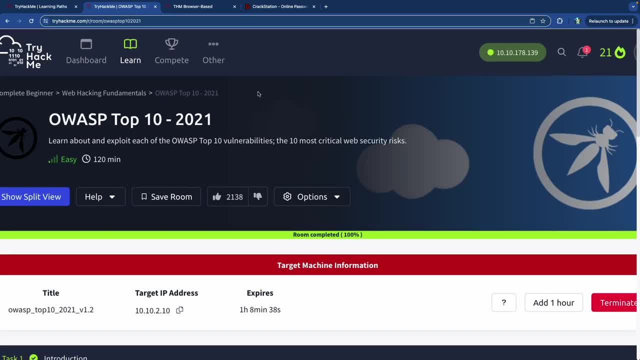 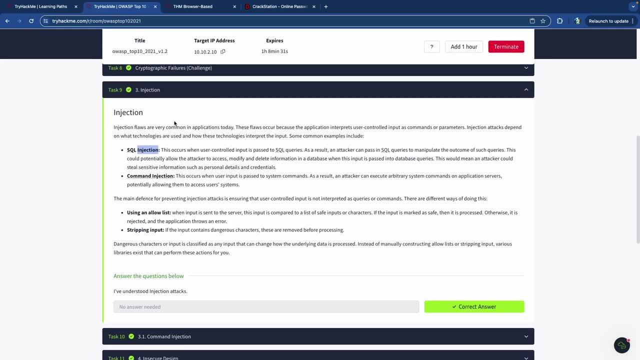 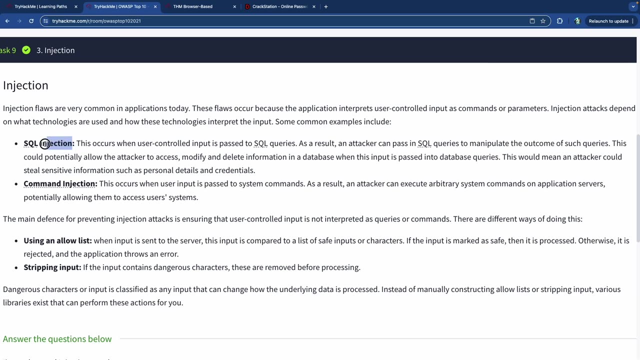 to the fact that you can go to a website that has a search bar or some kind of an input field, and it could even be like the username login field or something like that. but basically a search bar typically works and you go inside that search bar and you inject an SQL command so you say select. 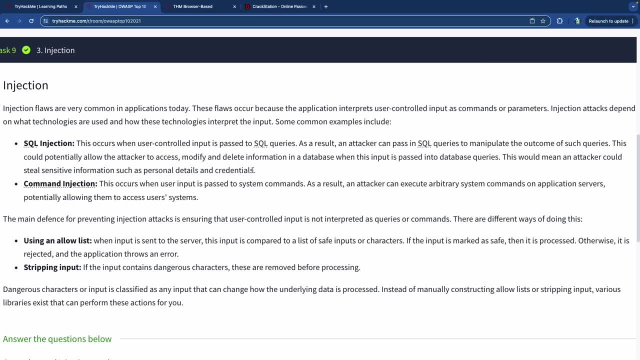 such and such from such and such, and that's a basic SQL command. or you do you do a dot tables command or something, just to see what it go, what actually exists and what kind of table that they're using, anything like that. so that will. if it's a weak website and it hasn't. 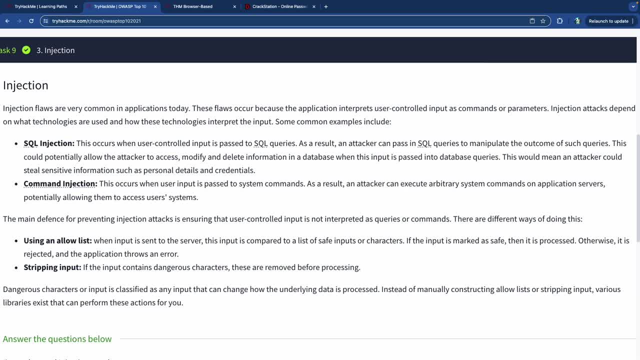 properly been secured. it'll return information to you that you shouldn't have access to, for example, the information inside of their SQL tables. another one is command injection, so you just type in some kind of commands. it could be a um, what is it? it could be a JavaScript command, which is a. 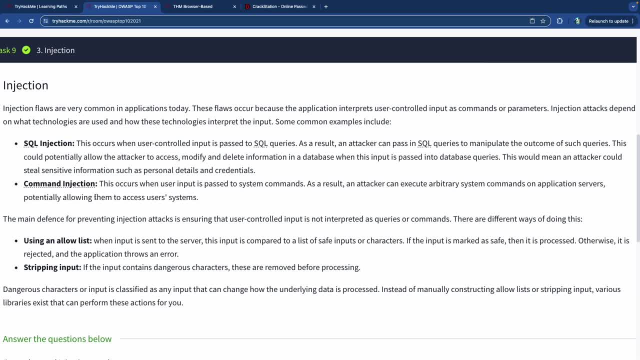 really big deal and it's used very frequently. it could be python, it could be a bunch of different types of command that you should not be able to inject into the website and then, when you do that, it'll return some kind of results. so it's considered. 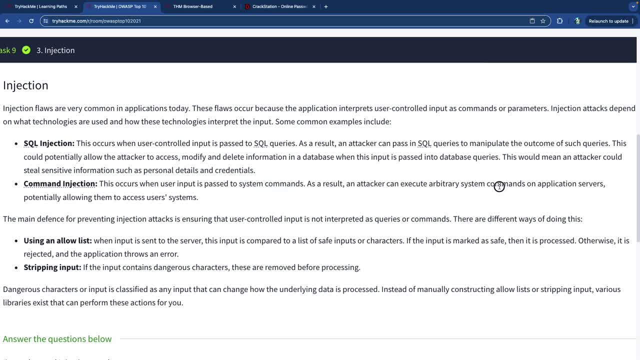 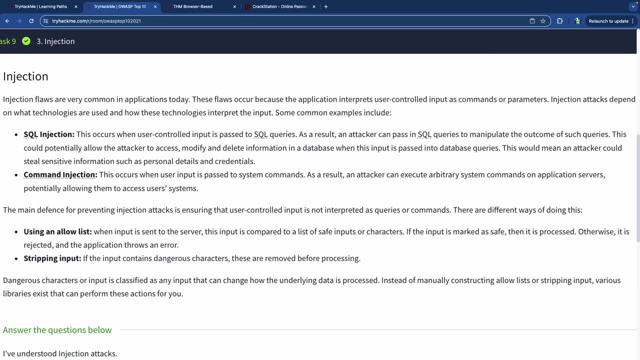 a system command and when you do that, it'll execute some kind of command on the servers and then allowing you to get access to their systems or do some things that you shouldn't be able to do on their system. so one of the easiest ways, or some of the easiest ways, to defend against this. 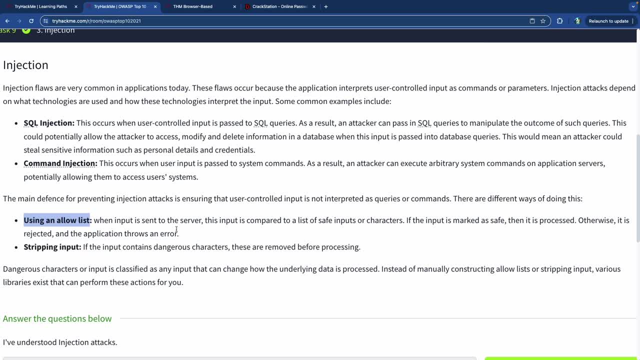 is number one. use an allow list, which means that there's a certain number of inputs that are allowed to be placed into your server and into your search box and all of those data points where you can actually enter information, and anything that's outside of that allow list is automatically just declined and it's rejected. another one is stripping the input. 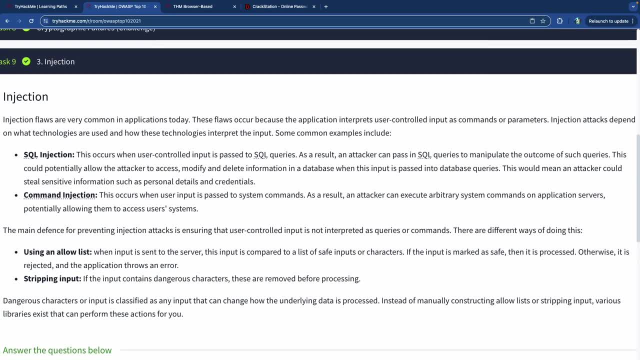 meaning that if somebody puts a asterisk inside when they shouldn't, or if they put any kind of symbol inside where they shouldn't, it automatically strips that input and it doesn't allow it to go through, which means that the full command itself won't be processed. so if you're running a JavaScript, 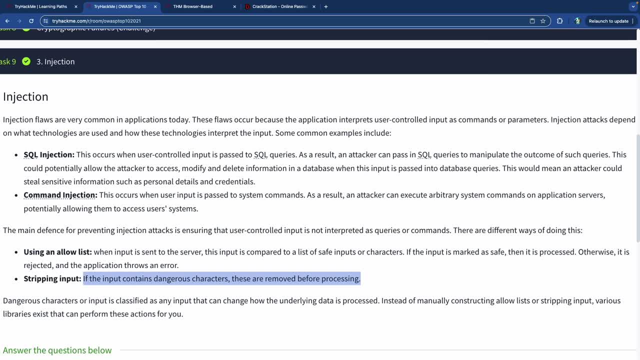 specifically, if you're running any kind of code and you're trying to input that in there, it'll strip that code of all of these malicious input characters and those characters aren't going to be processed. therefore, the command doesn't run and your website is protected, so you can either have 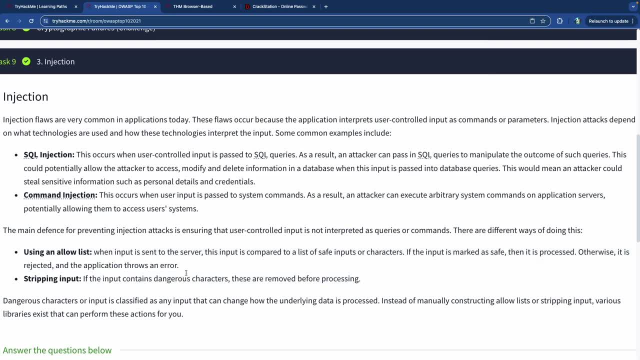 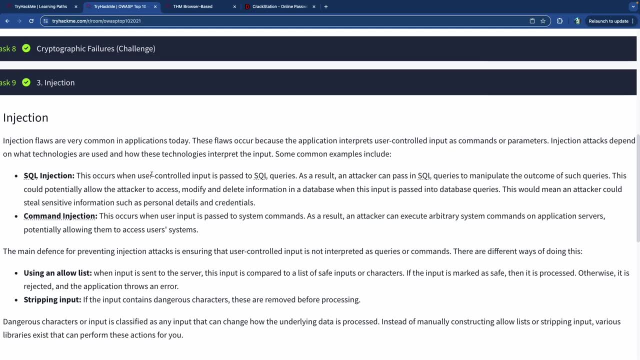 an allow list which can be kind of lengthy, or you can just do a simple stripping of the input so that they can't input any kind of dangerous characters and it won't mess with your website or return any information that it shouldn't or it won't. 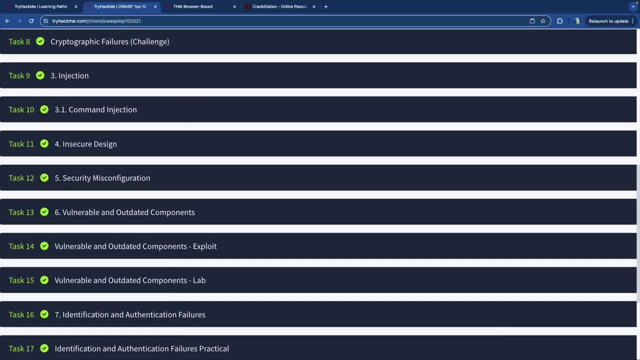 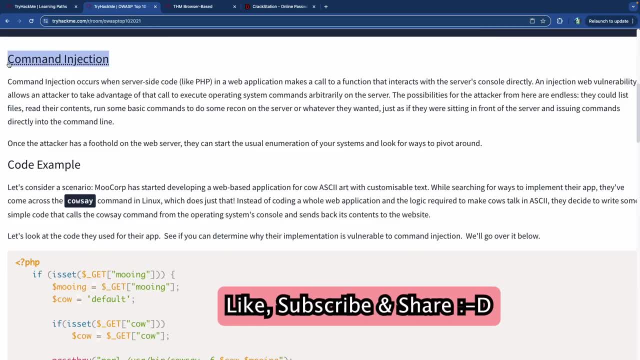 process any commands that it shouldn't. so that is what injection is. so we can now look at command injection and some examples. that goes into it. all right, so we already talked about command injection a little bit and what it actually does. so PHP could be one of the languages that runs on a web. 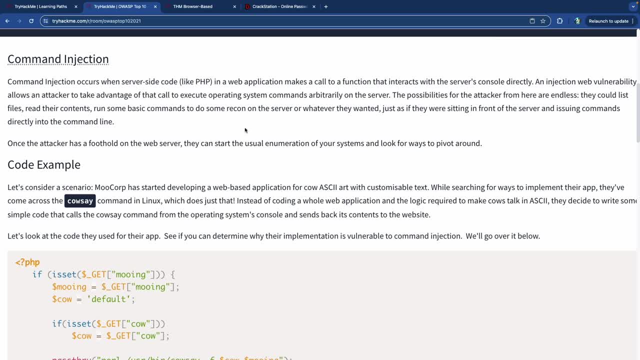 application. there's a lot of web applications that operate based on the PHP language, and so if somebody can get access to some kind of an input area that they shouldn't get access to and run some PHP commands, then they get some information that they shouldn't get access to. so an injection web vulnerability allows us to be able to make. 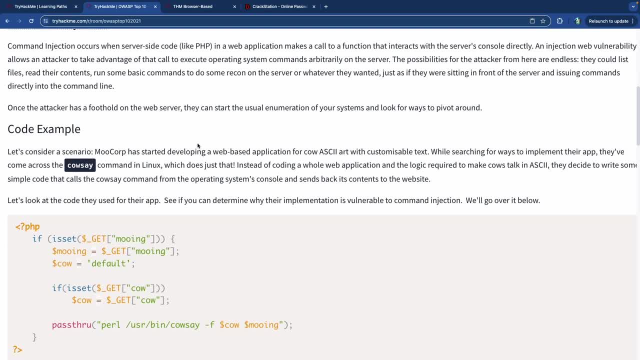 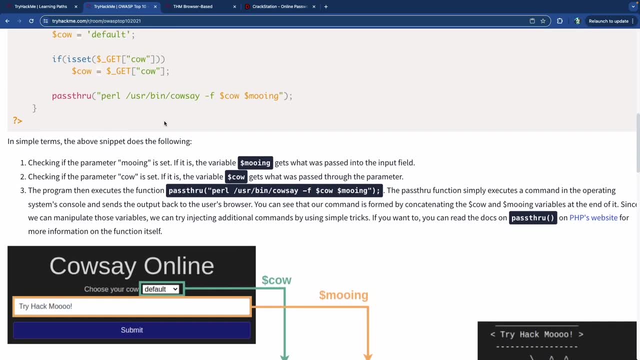 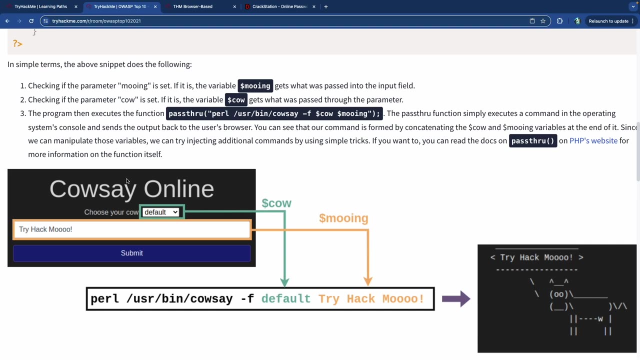 those calls and get those commands executed and get some information out of it. an example for this is the calc command, and it's called the calc online. I think they actually made this specifically to demonstrate this, but there was at one point that people were using it for to run their websites. 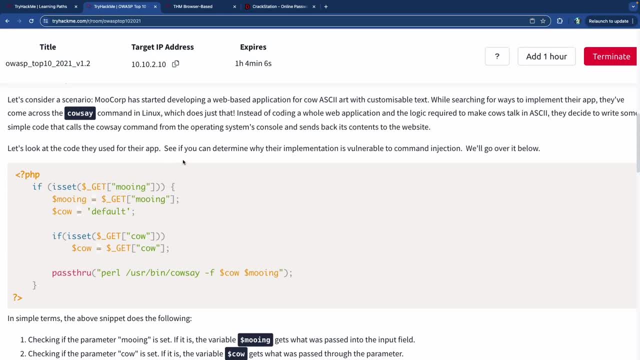 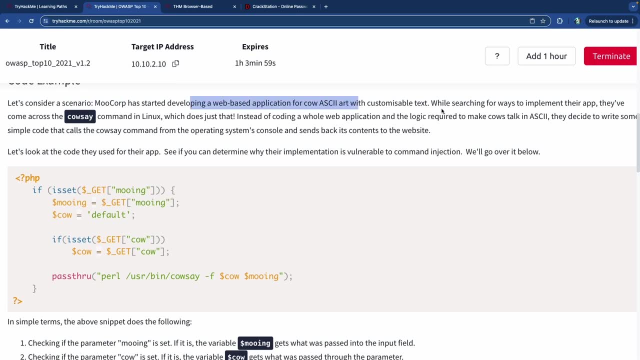 and it kind of turned into a big deal. I I'm not sure on that, you know. so fact check me on that and correct me on that. but moocorp has started developing a web application and while searching for ways to implement their app they come across calc command on Linux which does exactly that. 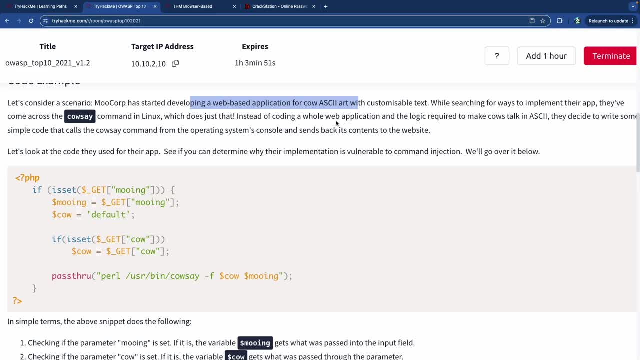 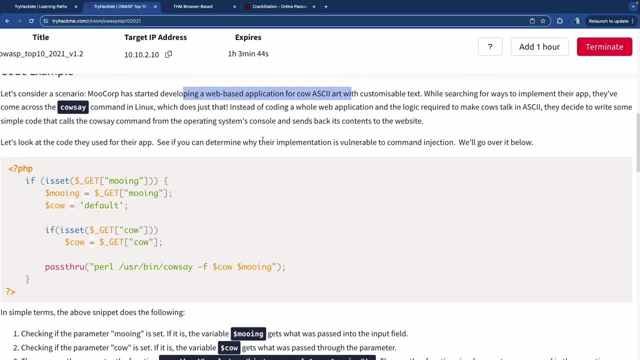 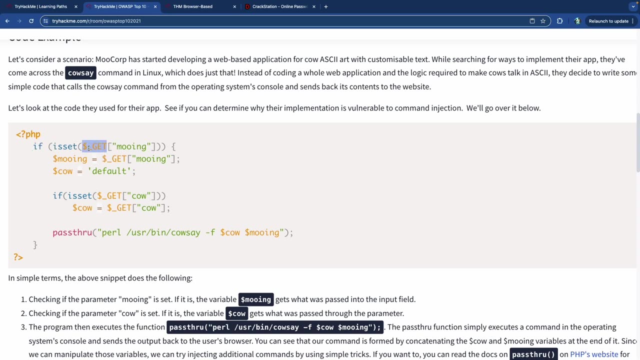 instead of coding a whole web application, they decide to write some simple code that allows the calc command from operating the system console and sends it back, sends the contents back to the website. so if you look at the code, it's like this. so it says: if this thing, the algorithm- uh, not the algorithm, excuse me- the variable get is set to mooing and 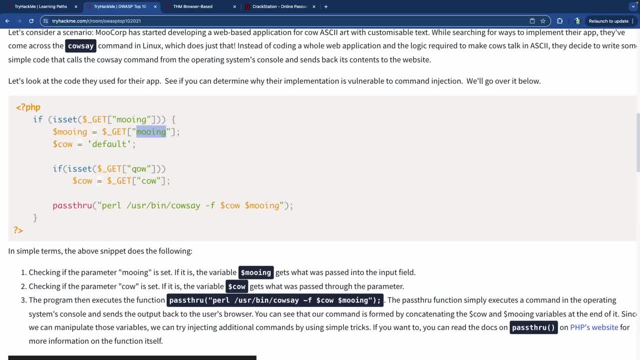 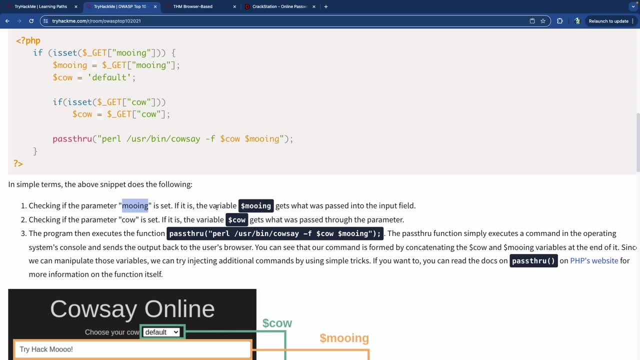 then mooing equals get, mooing count, Etc. so I'm not going to break this down, because they actually explain it over here. so it says: if the parameter mooing is set, then the. uh, if the variable mooing gets what's passed into the input field. so if the parameter mooing is set, so if this is set, then 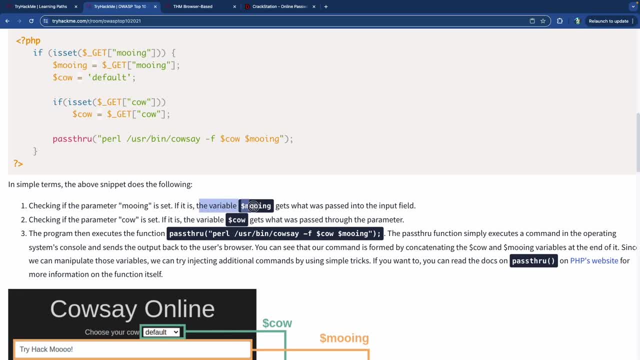 whatever is passed into it. uh, the variable mooing gets whatever is passed inside of that parameter. now, if the parameter cal is set, so if set is if is set cow, so if the parameter cow is set, then the variable cow gets what's passed through the parameter. so then it actually executes the full command. so this is. 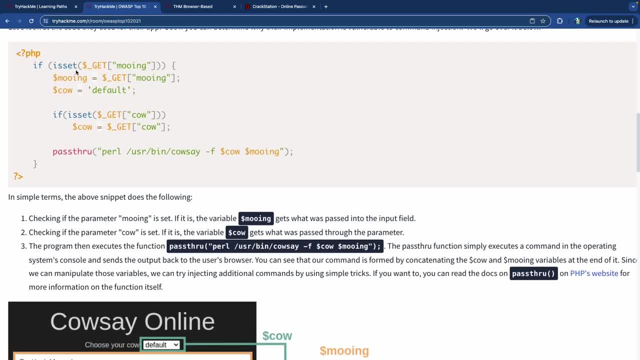 it. so it basically checks two set parameters. so if this is set, and if this is set, in that case we're going to pass through both of those things, both of those variables, cal and mooing, and then we're going to execute it, meaning it's going to be a pearl command that says that uses cal, say binary. 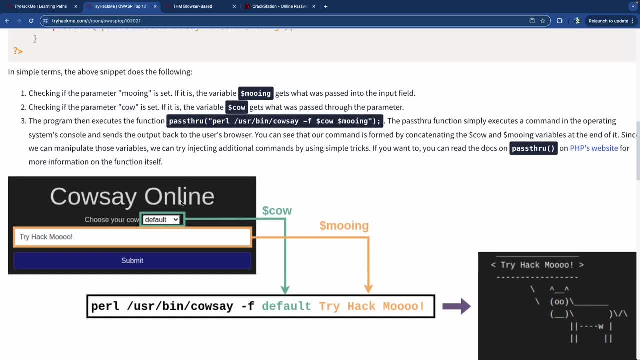 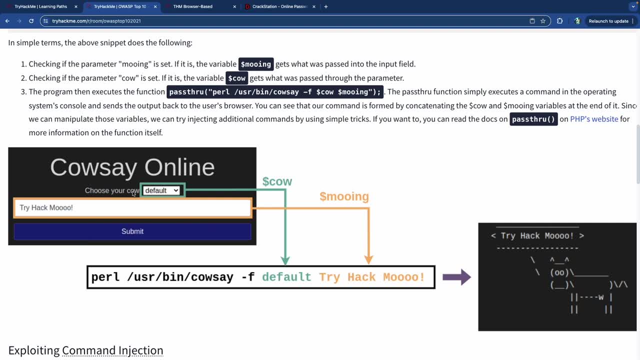 and it executes those things. so when you do that then you get some really interesting results. so in this case, this is our actual search bar and you have your. it says your default cow. so your version of the cow variable is default and the parameter right here, the input right here, goes into the variable mooing. so when you actually press submit here it 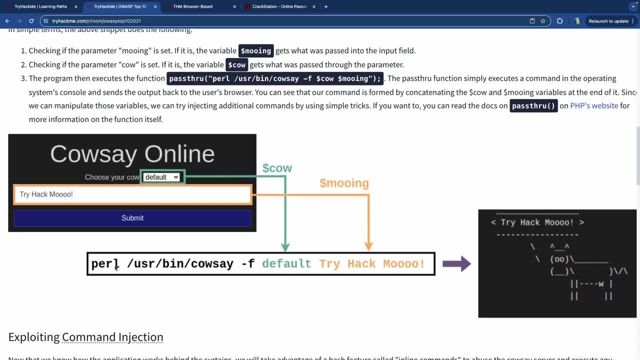 runs this first portion of the command right, so it runs this right here. and then now, whatever is input here is going to be passed due to the cal variable, and whatever is here, it's going to be passed through to the mooing variable. so it said: try hack moo and try hack moves past, and so right. 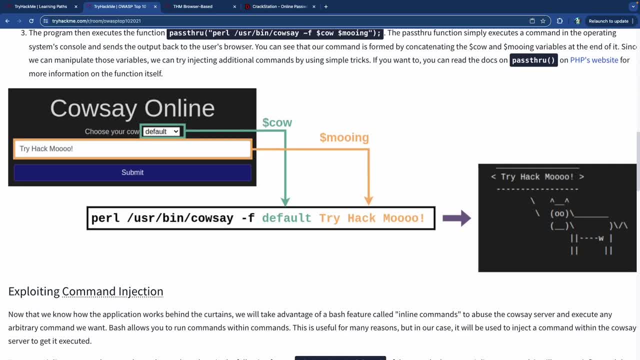 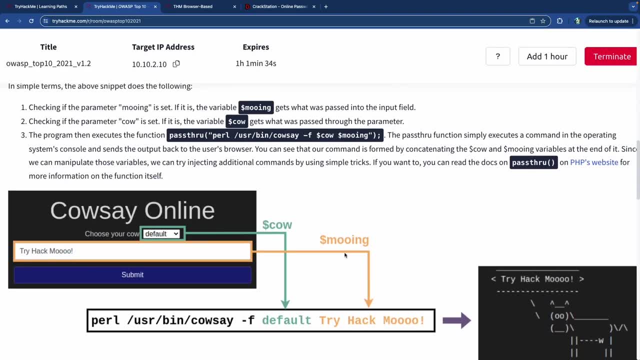 here the cow comes out and says: try, hack moo right. so very, very simple. nothing complicated about it, I mean, unless you don't know anything about code and shit like that. but all you really need to understand is that this thing is connected to the cal variable and this one 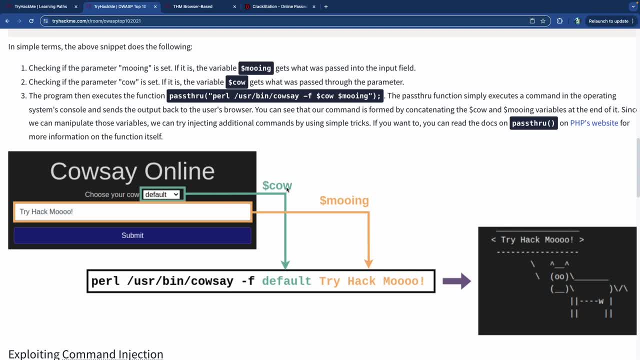 is connected to the mooing variable, and then whatever is chosen here gets passed to that, and whatever is chosen here or whatever is input here typed here, gets past that, and then the result is this little cow is going to say whatever is input here. so now what we can do is we can actually put 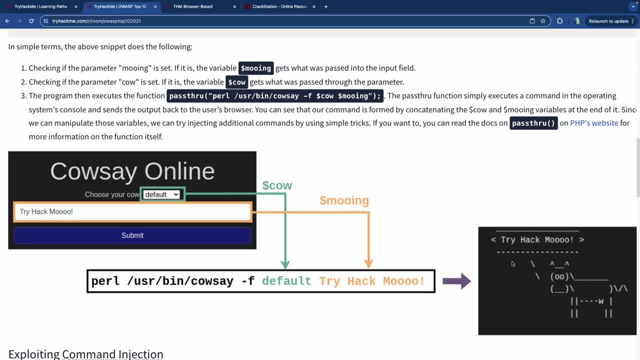 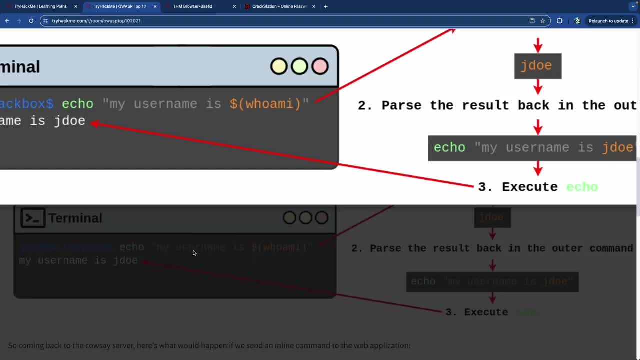 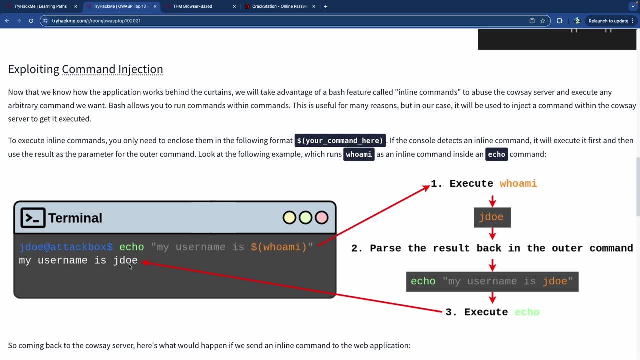 some kind of malicious code in here and this cow is going to. instead of typing out the code, it should give us some kind of a result. so, for example, echo- my username is who am I? my username is jdoe, and this echo command is actually just prints. whatever you 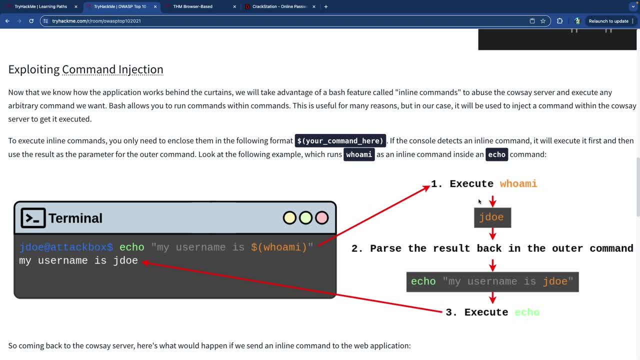 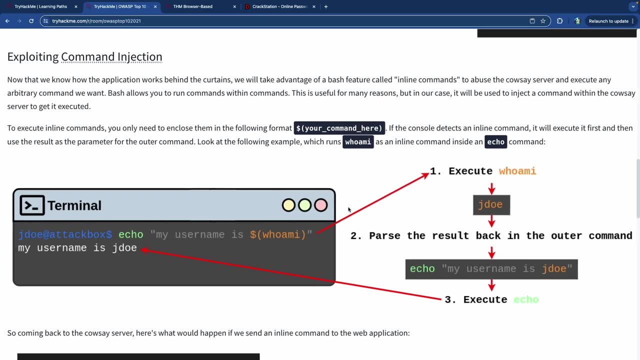 put into here in a string so it says it's executing. who am, I jdoe, parse the result back in the outer command which is going to be executing echo. this is, it's kind of beyond the scope of this. you should have an understanding of PHP. 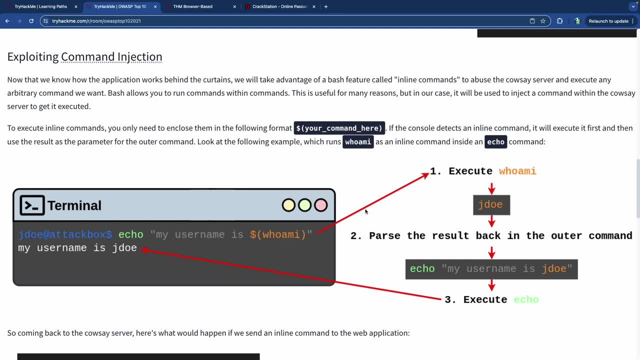 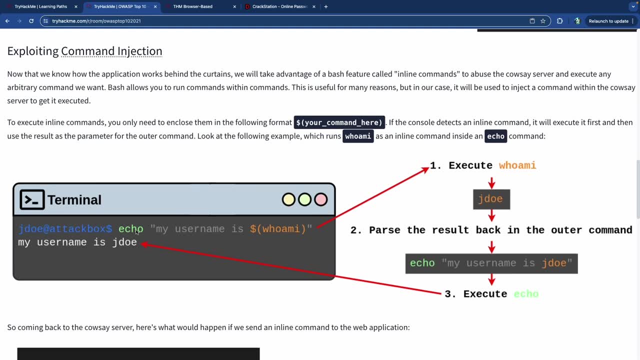 and how this whole thing works. but apart from that, this is really what it does is that if you just type into a terminal some kind of PHP command, so for example echo, and then give it a string value, so everything inside of these quotes is a string, and then we gave it a variable, which is variable. 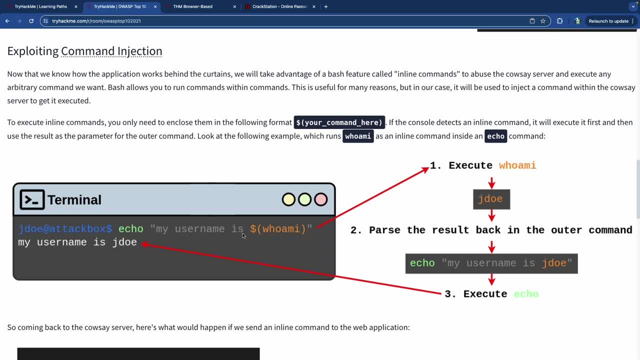 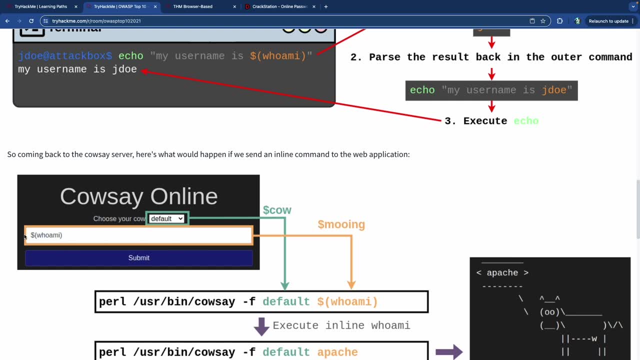 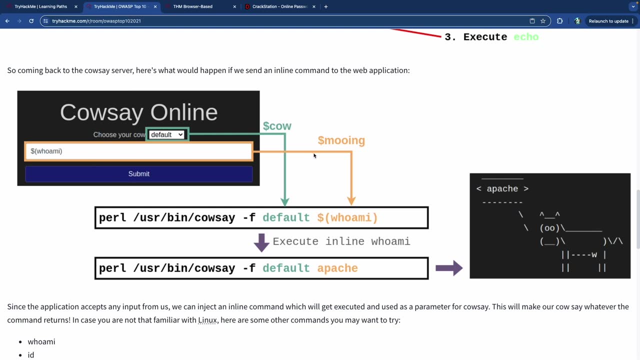 who am I and who am I is a command that you run that gives you the name of the user of that you're using. for example, you run who am I as the variable and it'll give you again. the default is going to be our cow variable and the who am I command is the moving variable and the cow, instead of printing. 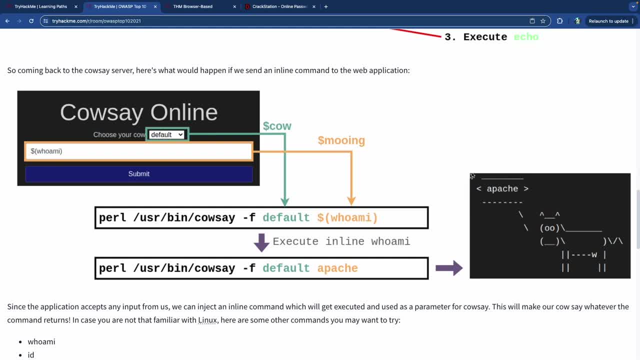 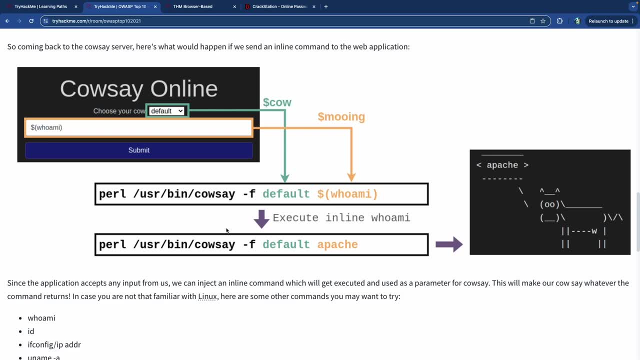 out who am I. it actually gives you the version, or not the version, the username that you're logged into, which is, in this case, a website server, which is Apache, and so it literally runs that for you and it gives that back to you, and so you can run a bunch of different types of. 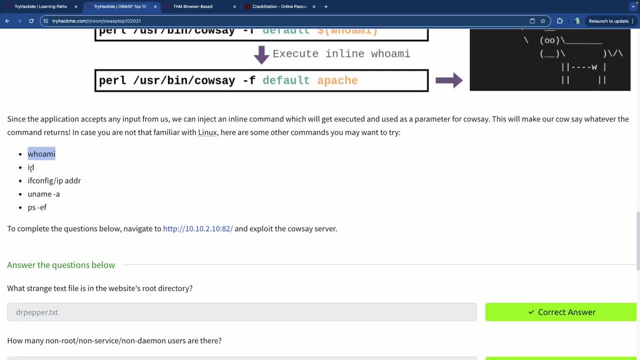 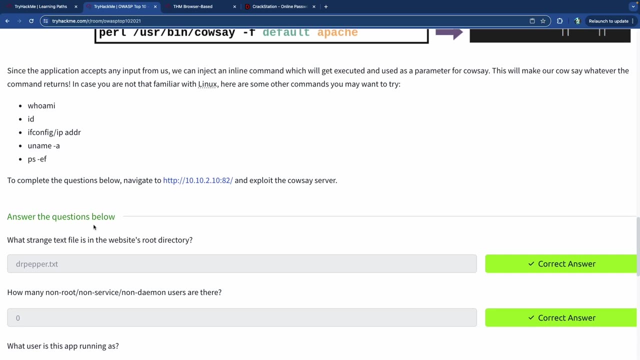 commands in PHP. so you have who am I, ID, IP configuration and the IP address. so this will give you the IP address of the, the web server or the machine you name, a, which gives you the username information of the version of the Apache server that we're on and processes, if you wanted to list. 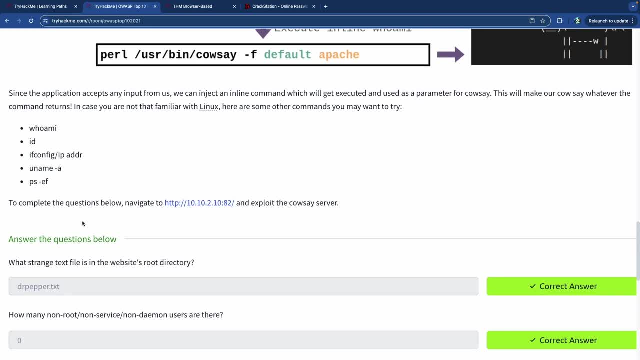 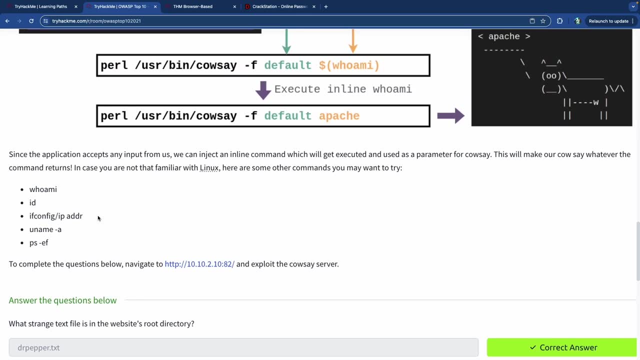 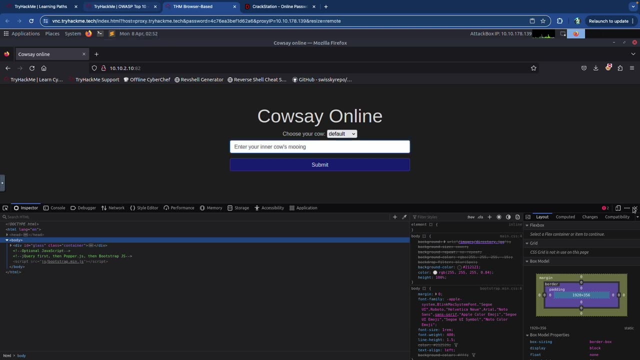 them. so these are some of the things that we're going to be running. so it says what strange text file is in the website's root directory. so what we can do in that case is we can run LS, which is a command to list things. so here we go. this is what we got over here, so I'm going to close this little piece of code at the 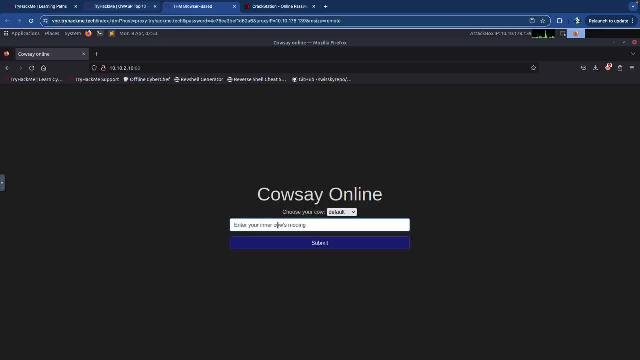 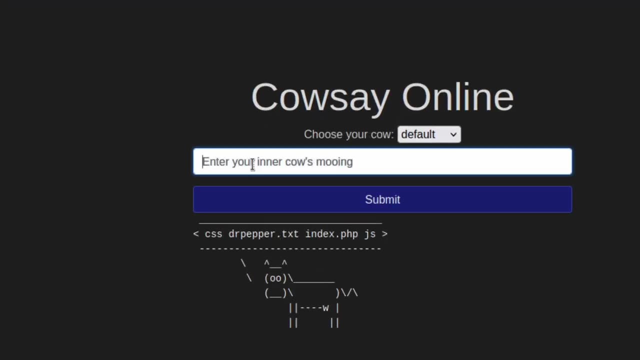 bottom, just to make this a little bit easier to process, and we're going to mess around with some commands here. so let's see what we can get all right, very, very simple. look at that. so I just all I ran was the dollar sign and I think it should show me the commands. there you go, that's the. 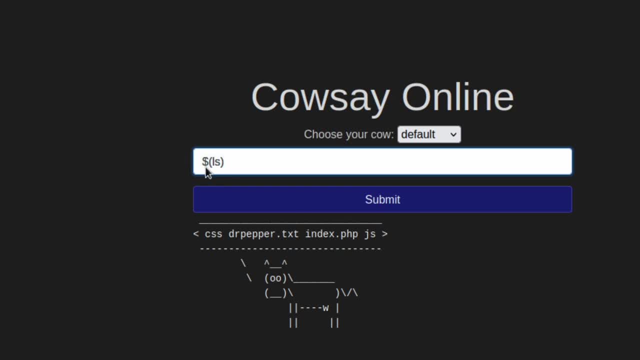 command that I ran. so very, very simple. you just have to put a dollar sign in front of it and then, whatever your command is inside parentheses, and LS is a command to list, and so it gave me the CSS, drpeppertxt, indexphp and JS. those were the stuff that's inside our root folder here and so 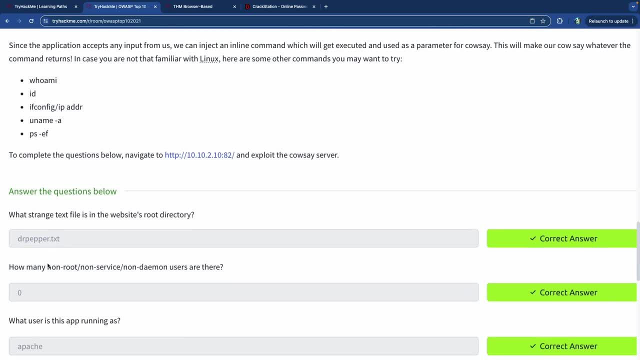 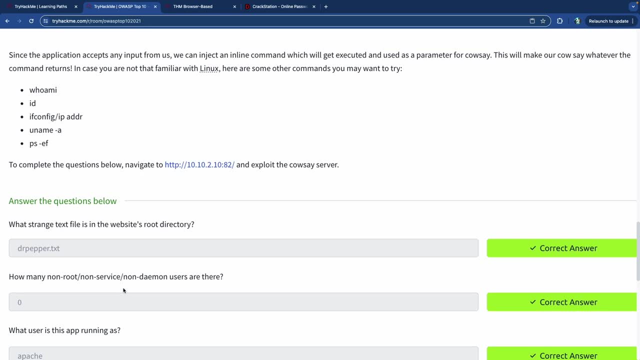 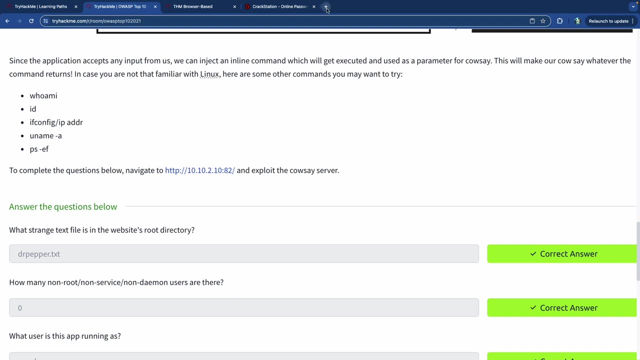 it's asking what is the text file, and so drpeppertxt. now it says how many non-root or non-service, non daemon users are there, and to be able to find that, we would actually have to find the command for it, and I forgot how to do that. so let me, let me check Google real quick. okay, so it's actually. 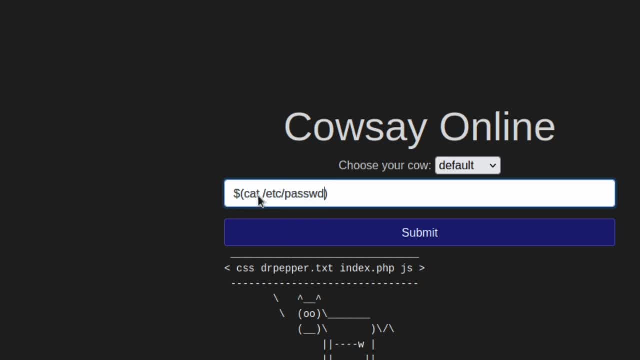 very basic. I thought it was going to be a complicated thing, but we're literally doing a cat, which is can cat and egg, or just print out onto the screen the contents of the etc password file, and the etc password file has a list of all of the users that are assigned to this particular 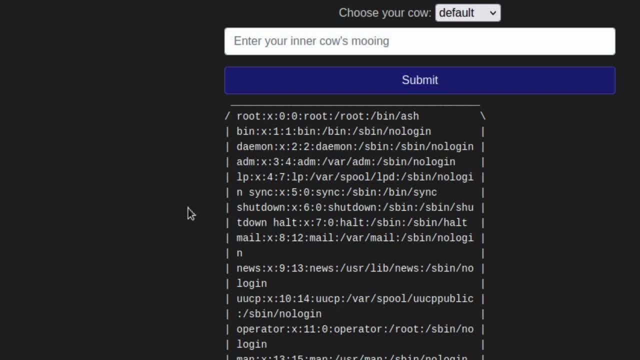 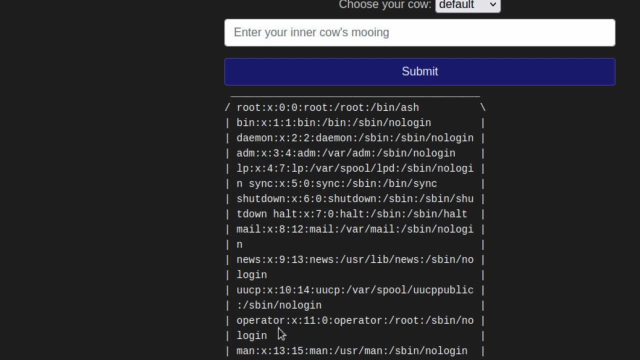 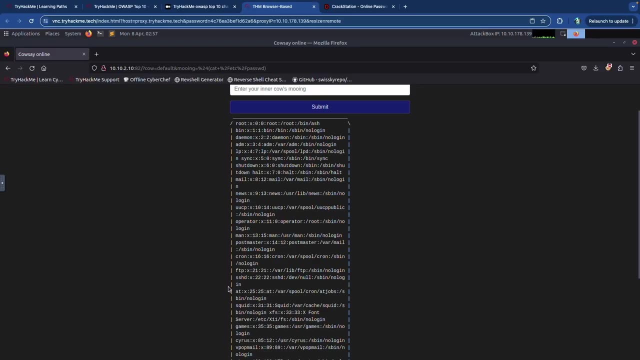 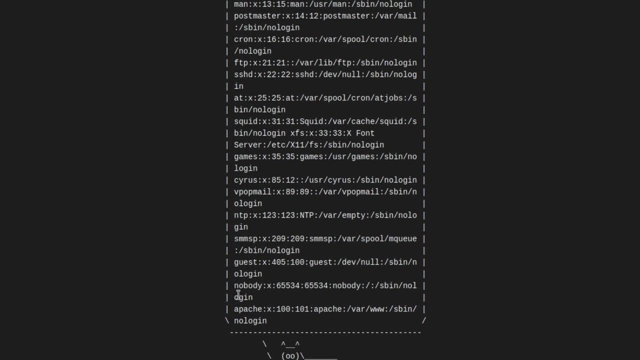 web server and when we run this we should actually get there. we go so we get all the information on it and it gives you all of the, the users in here, and I mean there's a lot of them. and let me see here what do we have that is non-root or non-daemon, non, uh, none, whatever. the other one that was. 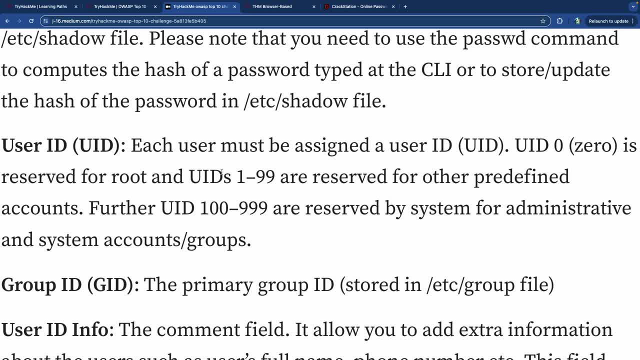 um, so all right. so here is some information that will make this a little bit easier to understand. so the uid0 is reserved for root, anything between 1 to 99 is reserved for other predefined accounts, which are daemon accounts, and everything between 100 to 999 are reserved by the system for administrative and system account groups. so anything essentially. 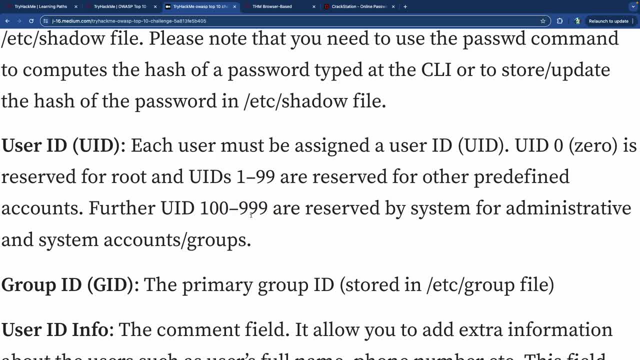 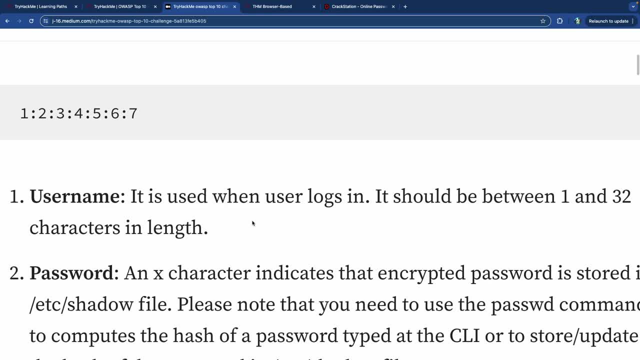 less than a thousand is something that we're looking for, or, excuse me, anything over a thousand is what we're looking for. that would be considered a non-root, non-service or non-daemon account, and this is how it breaks down right here. so if you look at it, you see root and an x, zero, zero. 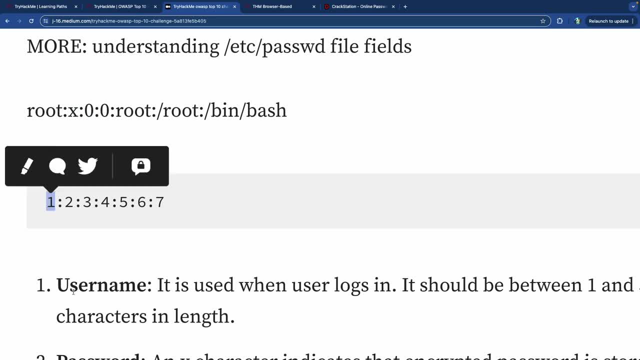 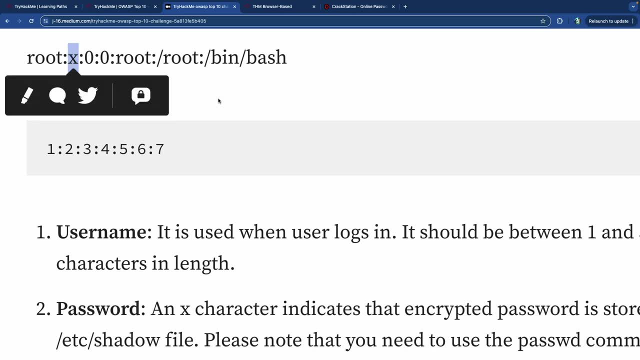 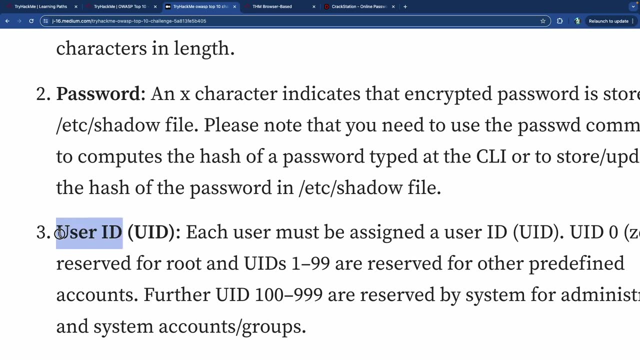 roots. so this would be one, which is the username. two would be the password, which is going to be always an x, because inside of the etc password file we're not going to get any kind of password information. all that stuff is inside the etc Shadow file. and the third piece is the user ID. 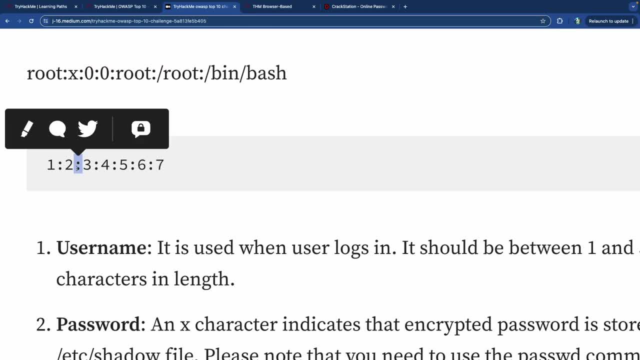 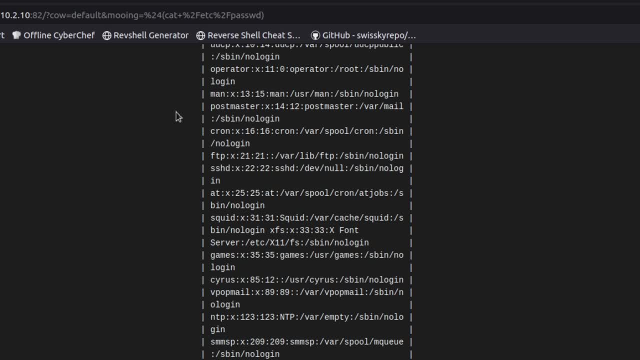 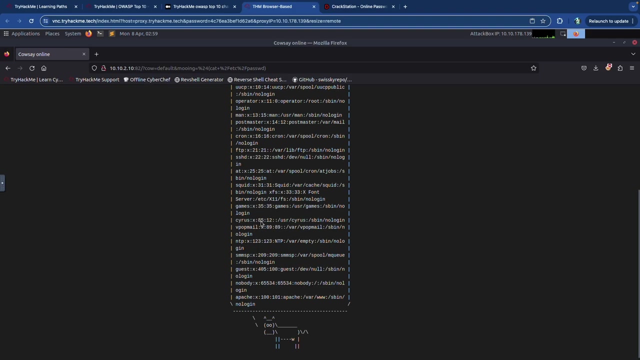 so it's the, it's between the, the second and the third colon is the information that we're looking for. so if we go back over here, we will see that. so you have the user, you have the x for their password and then you have everything between the second and third colon, and there is nothing that is above the number thousand. so 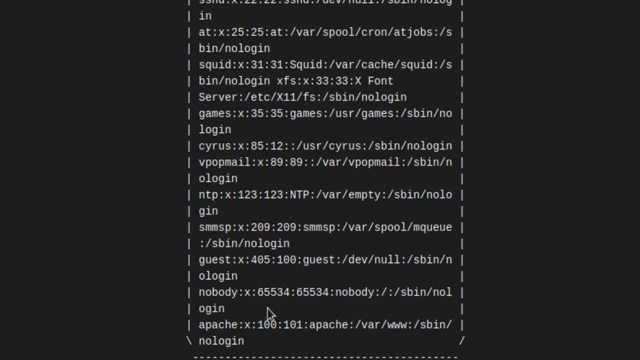 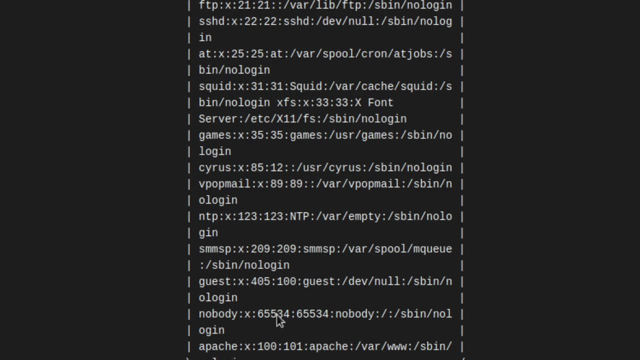 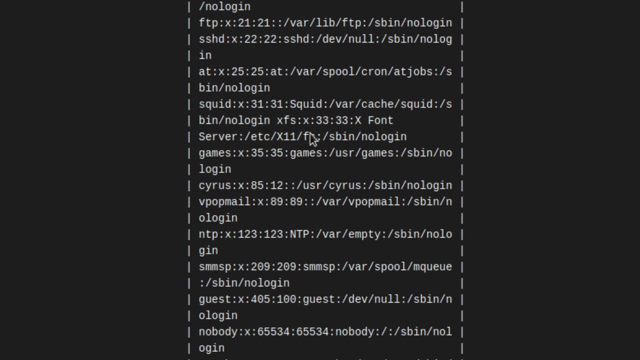 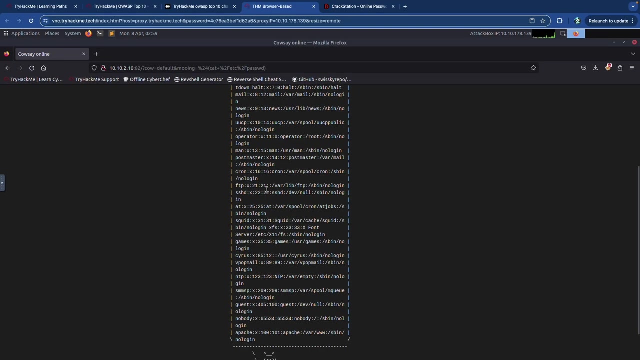 there's literally all of these right here, starting from Apache, and if you go all the way over here, nobody- 65, 534, that is technically. I don't think that even counts. you have 405, 209, 123, 89, 85, 35, uh, the, what is it? you have, uh, 31, 25, 22, 21, so it doesn't look like there's any in here. so if we 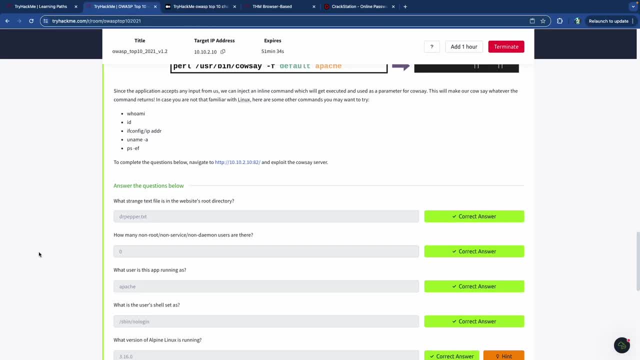 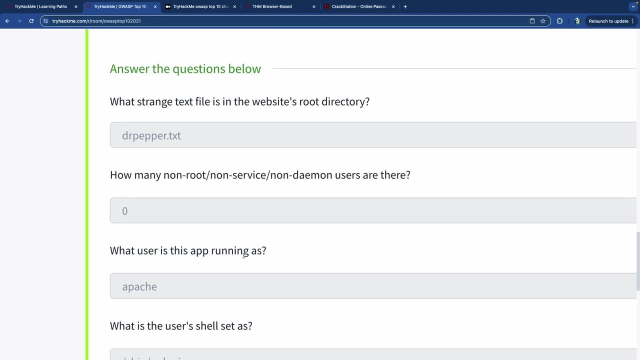 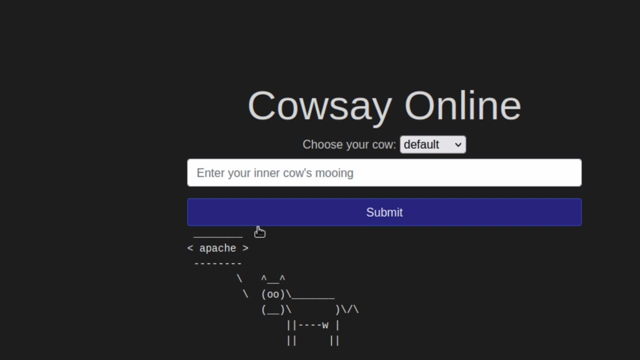 go to our answer here. the answer that we had previously was zero, so that is the correct answer. and so what user is this app running as? so what we want to do is we want to run the who am I command to see what user we're running as. so let's go do that one, and when we run who am? 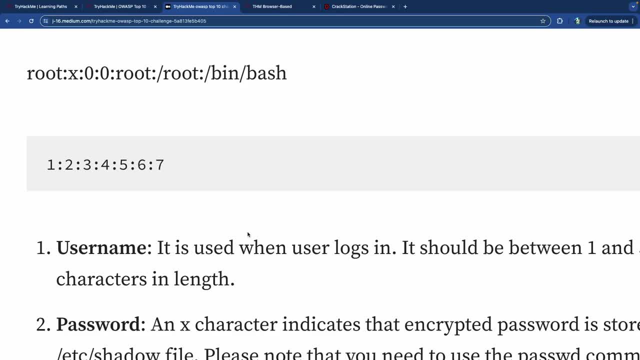 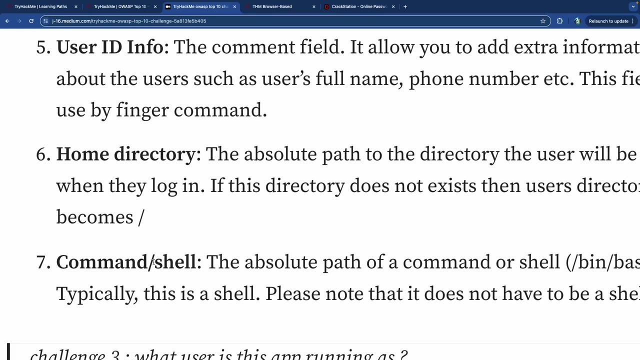 I. it gives us the user Apache, which is the answer to this question right here, and what is the user's shell set as? and so if we go here, right here, where it says bin bash, that's what the very last item on that is, which is their command shell. so when we're looking at it, we're trying to find the very last. 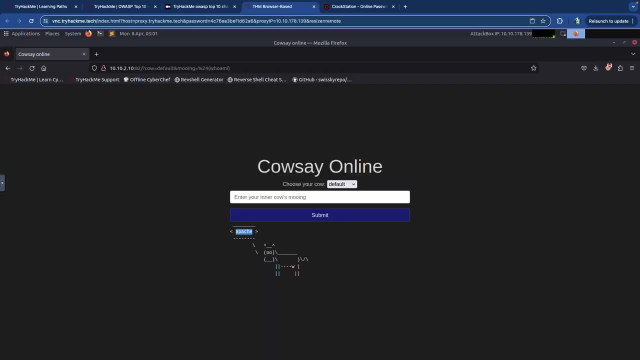 item. so we're going to go back in here and then we're going to run the who am I command one more time. I know we're just going to- not who am I excuse me- the, the, etc. password command and from here we're going to look at the Apache user and then see. 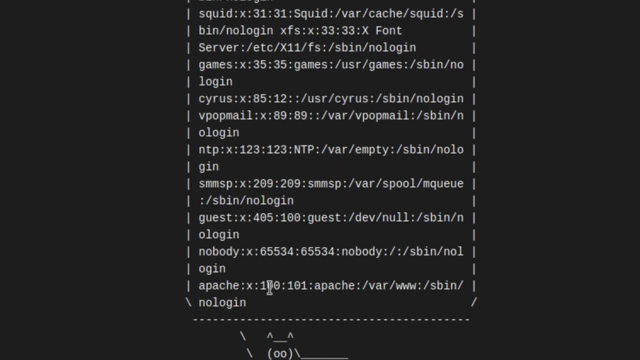 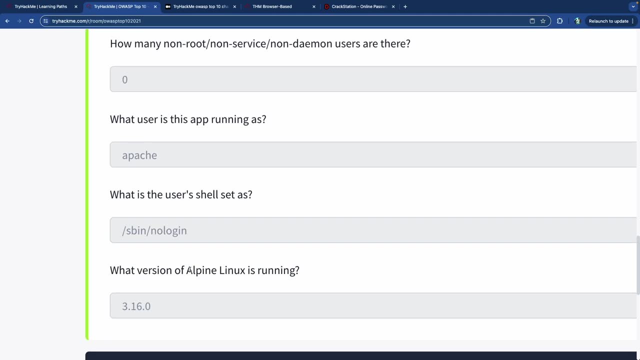 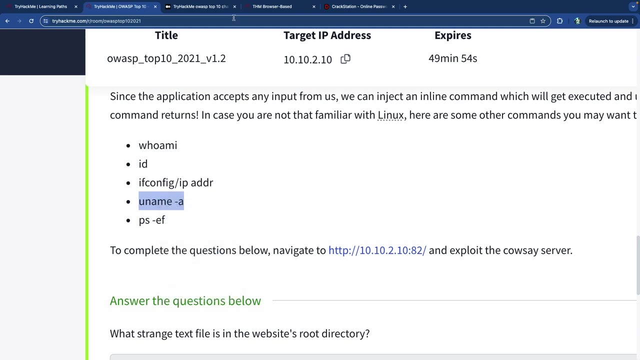 what their shell is set as. and there we go. so we got Apache, their user information, and then sbin: no login is their shell, and so it's been no login. and what version of Alpine Linux is running, and I believe that is the uname a command, so let's go and run that one, all right. when I ran the uname, 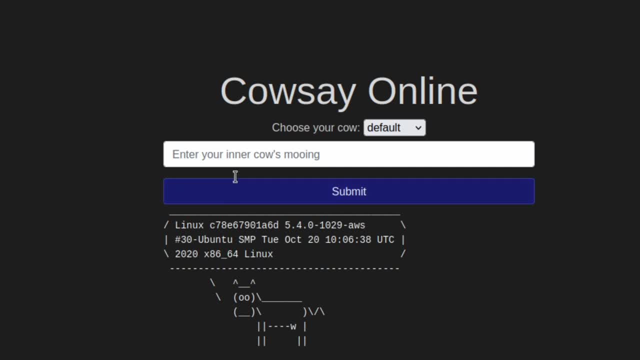 command. it gave me this information, but, uh, the information that we're looking for is actually not in this result. so we're going to run a different search command real quick, and it is uh, this one right here which is lsb, release a. so we're going to run that and that should give us the information that we're looking for. 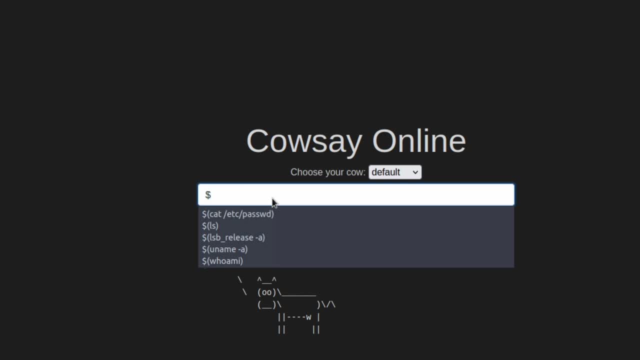 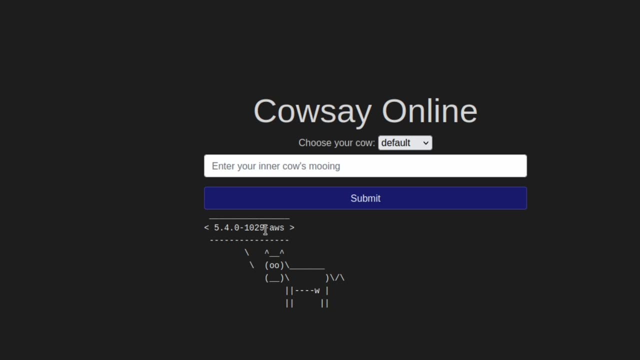 and it is not the case. all right, we're going to test out another one, which is uname R. let's see what this one gives us. so I think, actually, the previous command that we ran was, uh, the right one, the uname a, and it gave us all the information. 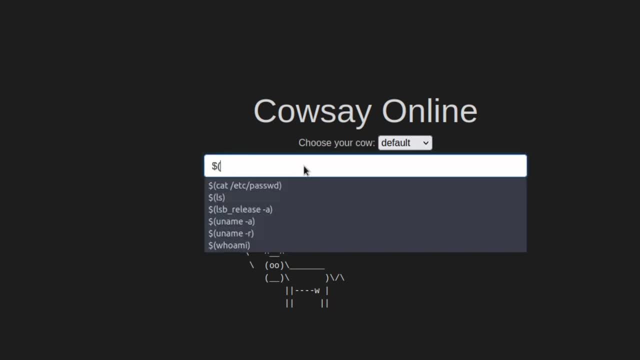 but it was- uh. it's not uh congruent with the very last time that I ran this lap, because when I ran this I actually did it a while ago and I think the information has changed. maybe the server that's been applied to this has changed, so I'm going to run this one other piece right here and see if. 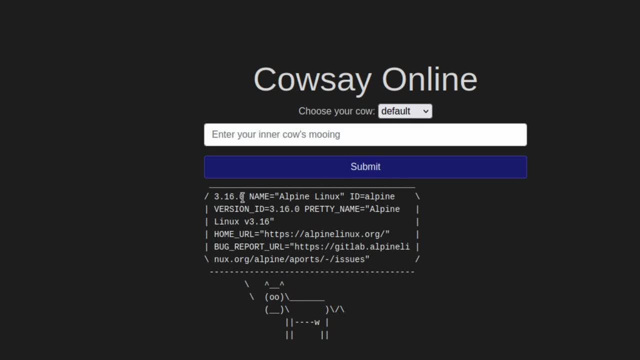 there's any other information that'll come out of this? um, oh no, yeah, there we go. so 3.16.0. name Alpine Linux, so on and so forth, so 3.16.0. so it actually has not changed. it was just different command that we ran and I literally got that command from uh. 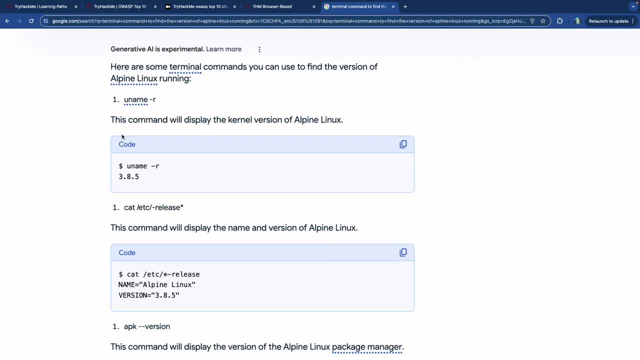 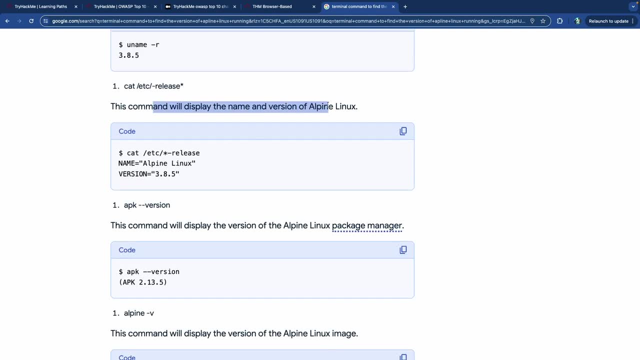 just going to Google and finding a bunch of different terminal commands that will give us the version, so uname. R was the one, the first one that I ran. and then you have cat ETC release. uh, the that'll uh release. that'll give the name and. 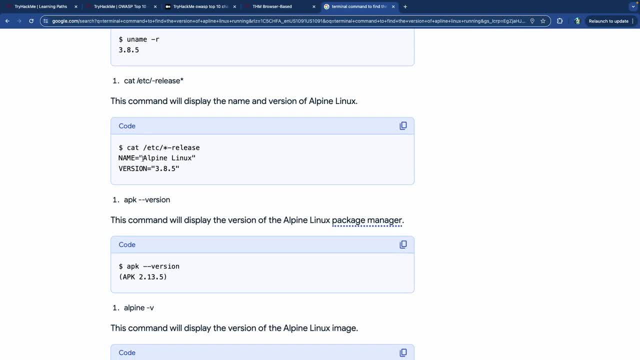 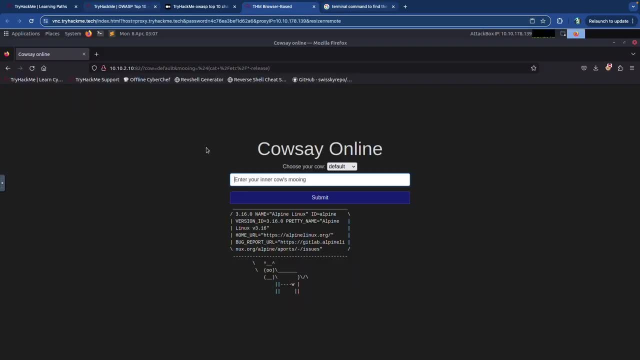 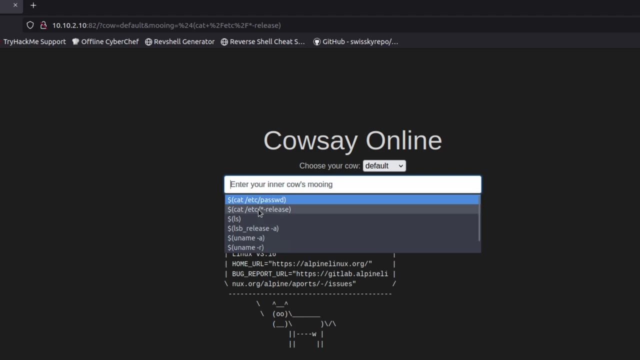 version of the alpine linux that's running on our server and so that is the one that actually worked for us, and it is 3.16.0. that would be the answer. so it's actually the the etc release, uh command that we have here, which is right here. so cat, etc, cat, forward slash, etc, forward slash, asterisk dash. 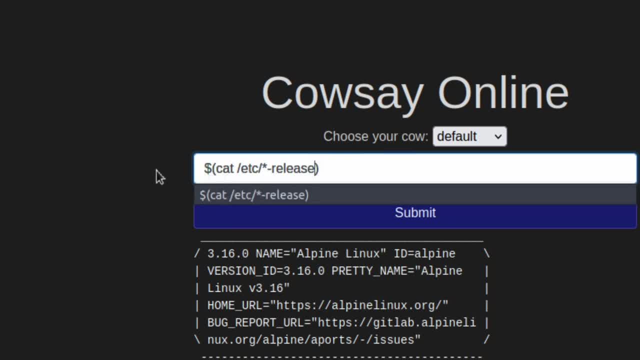 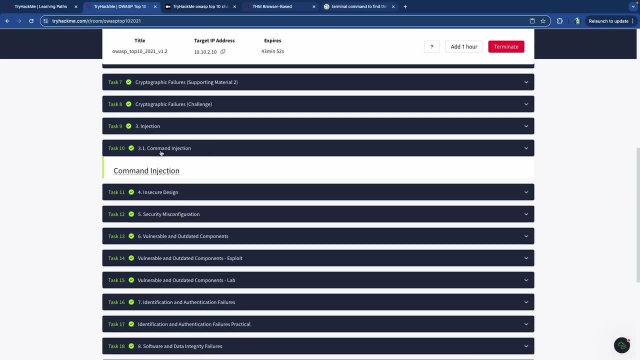 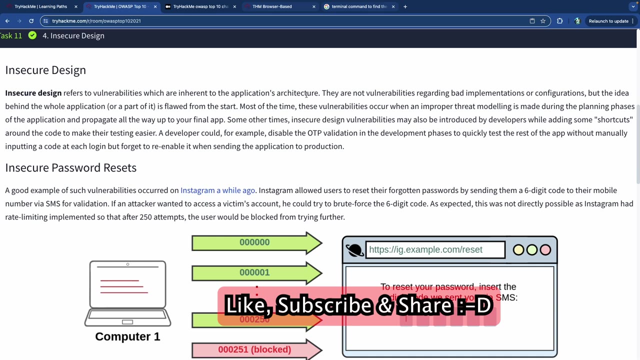 release, and then you put all of that inside of the parentheses and then you get your information like that. so there we go, and that is it for this one for command injection. so let's go look at some insecure design flaws. all right, and secure design has to do with the actual setup of the application. 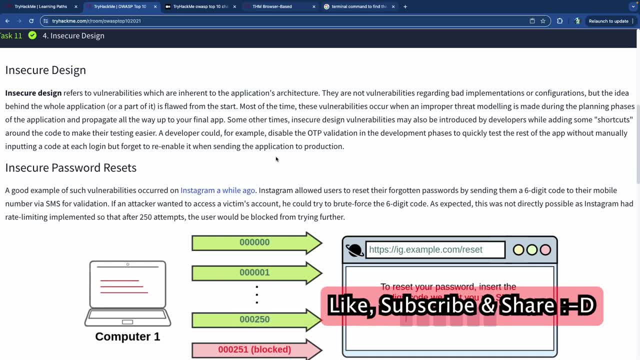 itself. these aren't actual vulnerabilities or anything like that. it's what was done when they were planning to build the application and they took some bad steps in the thread modeling or preparing for the application's design and creation. so it's an actual flaw that was inside. 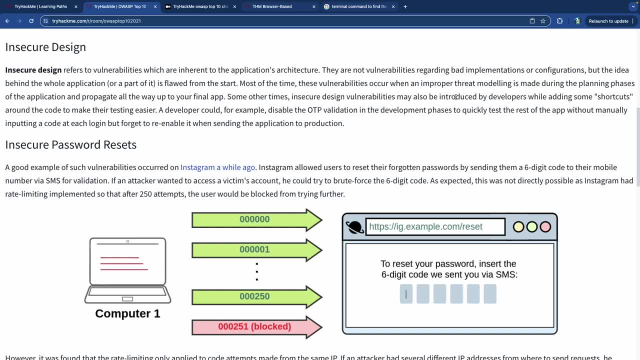 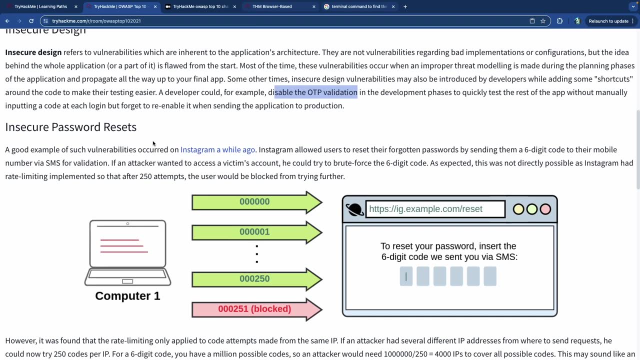 of the design of it, and so your design. vulnerabilities may also be introduced by developers by adding shortcuts around the code to make testing easier, and then they never removed it. so if they disable the one-time password validation in the development phase to quickly test the rest of the app and then not put it back, that's a design flaw and insecure design flaw. so 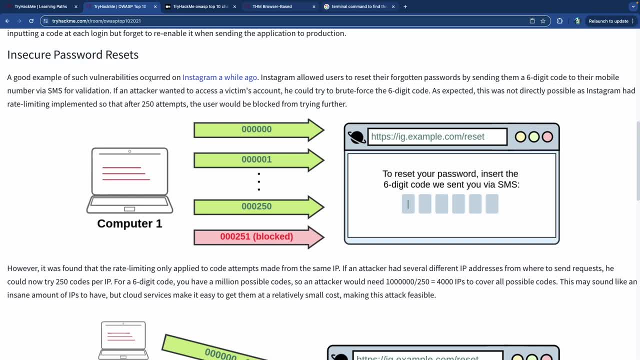 a version of this would be insecure password reset. so this happened on instagram a while ago. they allowed users to reset their forgotten passwords by sending a six-digit code to their mobile device and if the attacker wanted to access their account, they could just brute force the six-digit code, and this wasn't directly possible. 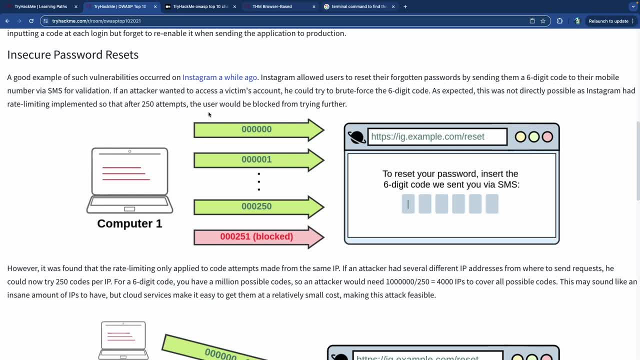 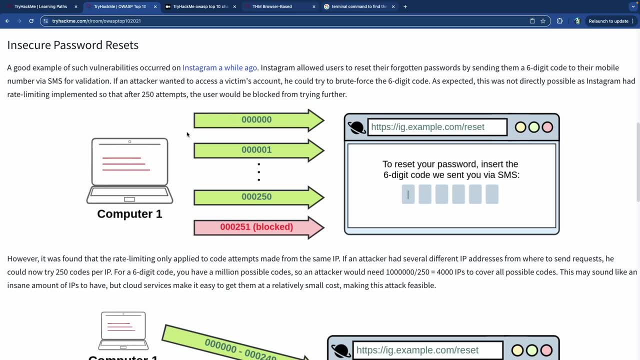 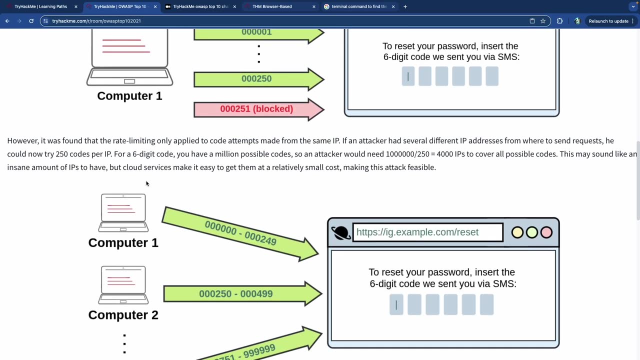 because instagram had rate limiting, meaning after 250 attempts that we just get blocked from doing anything further. that's what rate limiting is, and if it's a six-digit code, there's literally so many different versions. uh, definitely more than 250. i don't know what the number is, but it's definitely more than 250. but they found out. 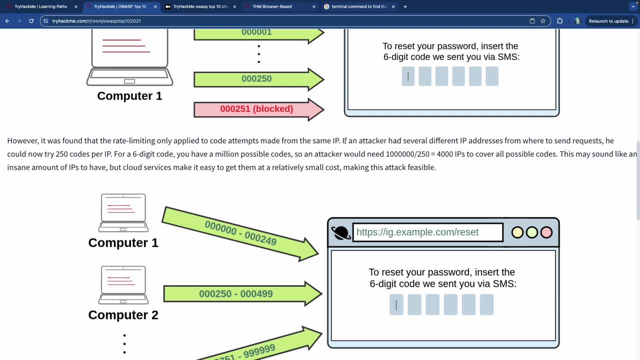 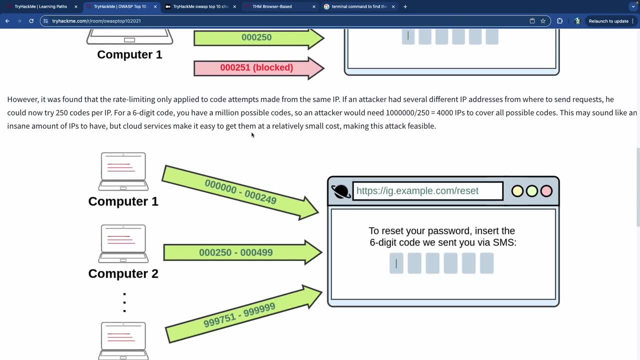 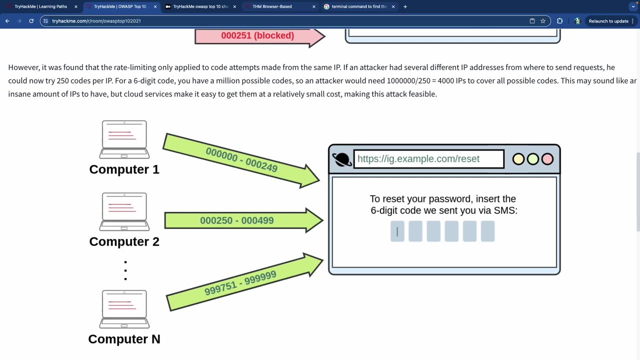 that the rate limiting only applied from the same ip. so if somebody had multiple ip addresses, then they could go up to 250 with one ip, from 250 to 499 with another ip, and then just keep going until they found the actual version of the six-digit code that they needed to be able to get the the. 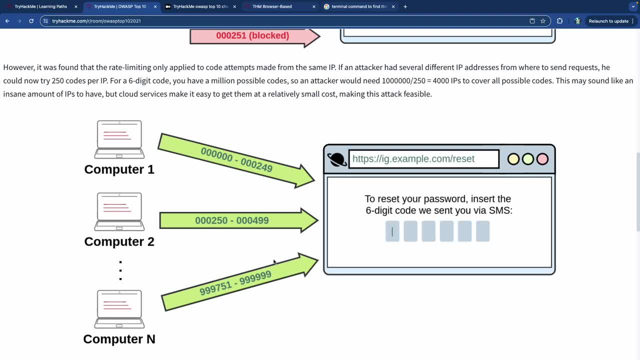 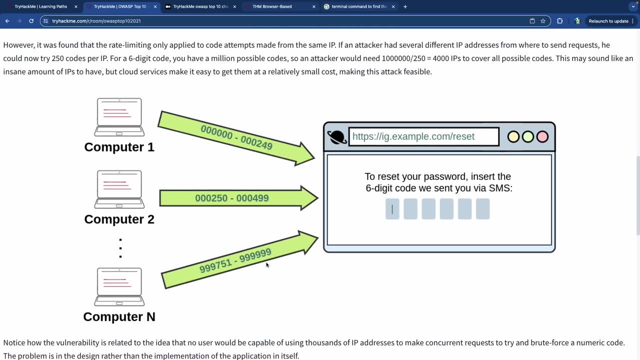 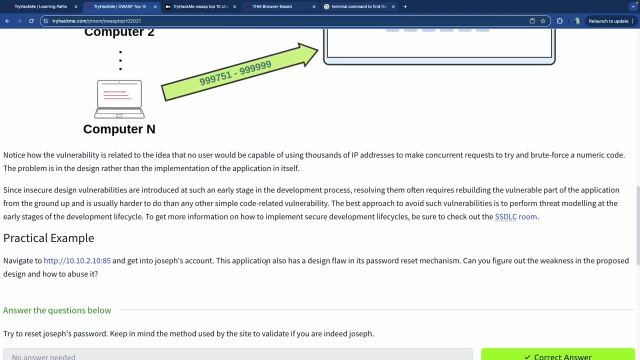 password of the person, so it's kind of a big flaw. uh, it is more of a complex flaw compared to some of the other ones that we noticed, but it is still a pretty big flaw, especially for a website like instagram. so this is one of those things that was a design flaw on on instagram's part, and 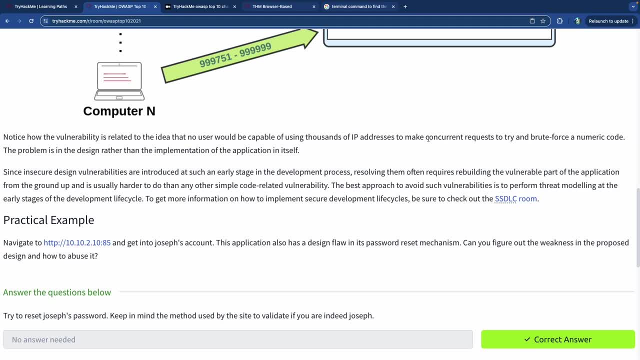 no user would be capable of using thousands of ip addresses to make concurrent requests to try to brute force something. it's in the design rather than the implementation of the application itself. so what we're going to try to do in this case is we're going to go to: 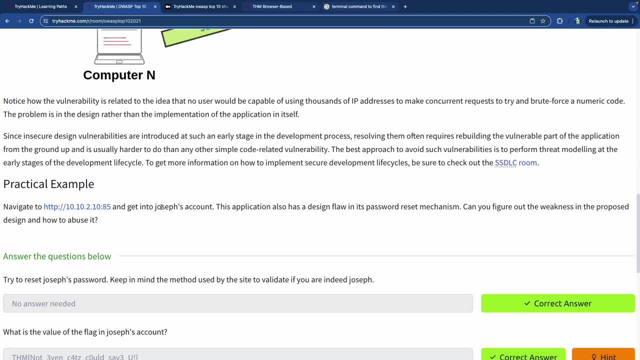 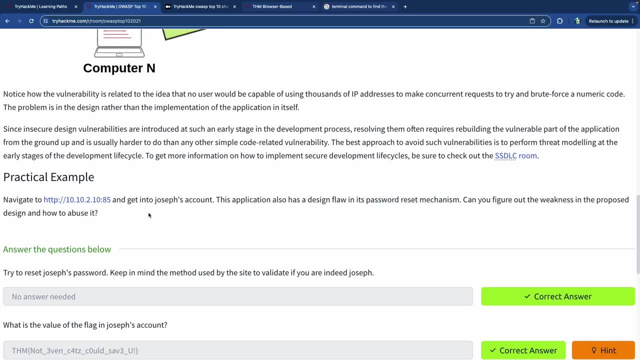 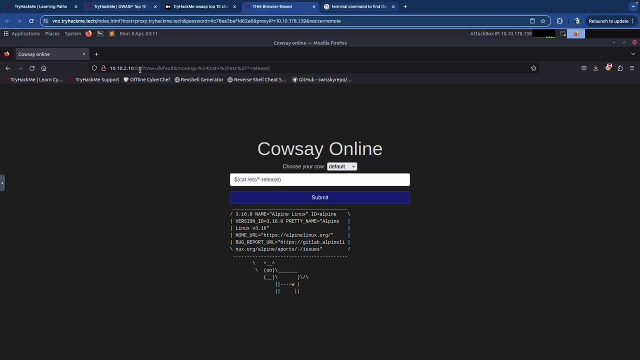 the another version of the website that we've been using and get into joseph's account and then try to find the design flaw in the password reset mechanism and then try to figure out what we can do and abuse it and log in as joseph, and so it's going to be on the port 85 on this website all. 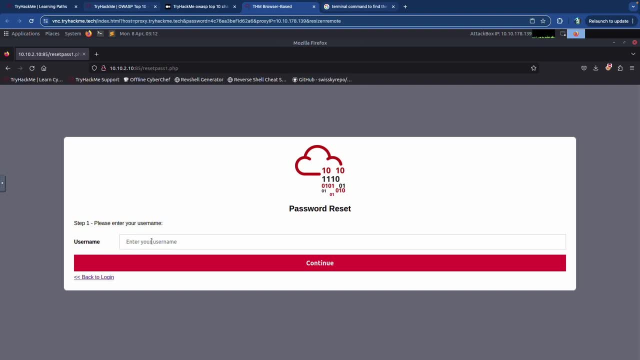 right. so you land on the website. uh, it asks for your username and password. i just clicked on, forgot my password, and what do i need? i just need to use my username, which is joseph in this case, and let's see what the instructions are for us to be able to reset our password as joseph. 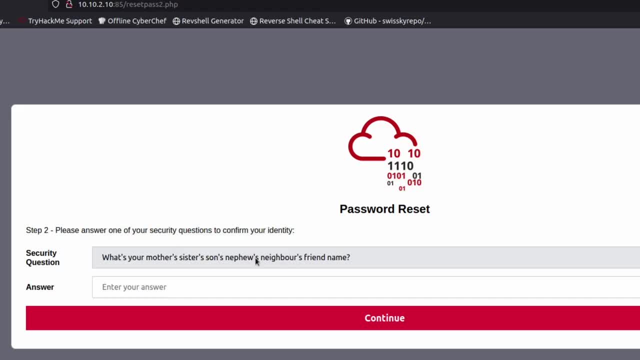 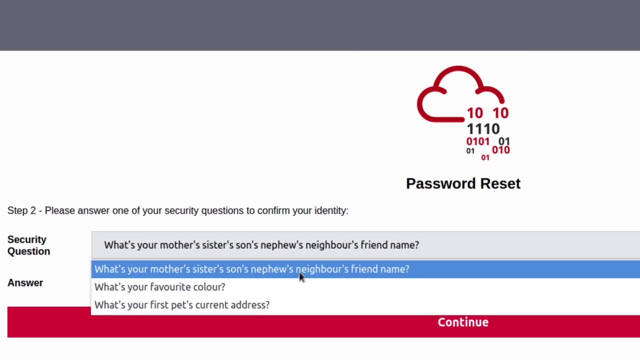 what's your mother's, sister's son, nephew's, neighbor's friend name? so there's a few different security questions that's available for joseph. it could be that one. it could be your favorite color, it could be your first pet's current address, so probably the easiest one would. 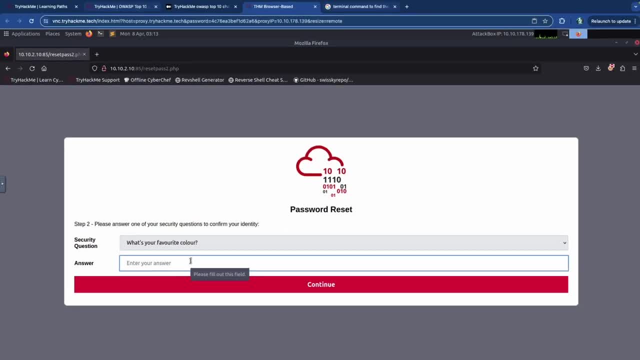 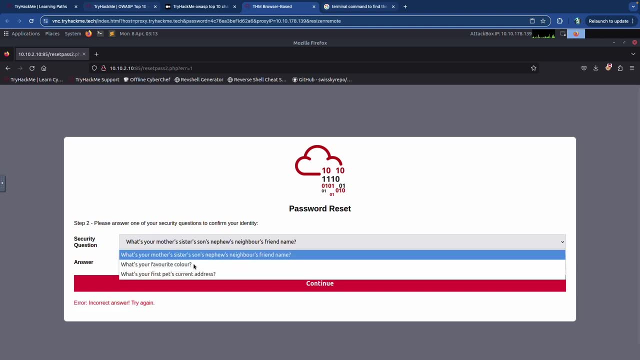 be the favorite color, wasn't your password and you can say, okay, so in this case it's joseph's friend's blood side. well, that's correct. so i'm going to just nesteinize the password first and see where thatgers come from. then i can relook at that same answer and use this. 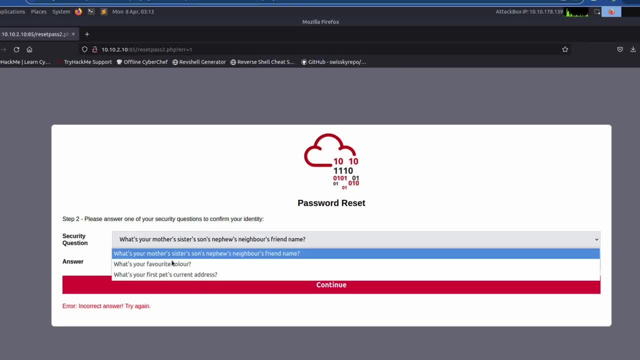 right so that we can reset joseph's password, so that we can relook. but there's a couple of changelins, so let's check this out. so i should be able to think about how to reset password. so i'm going to check. how do i set? 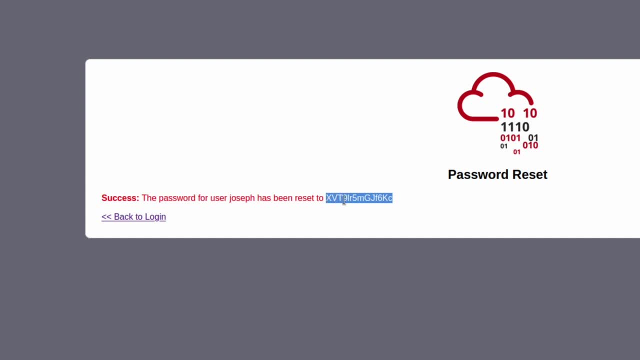 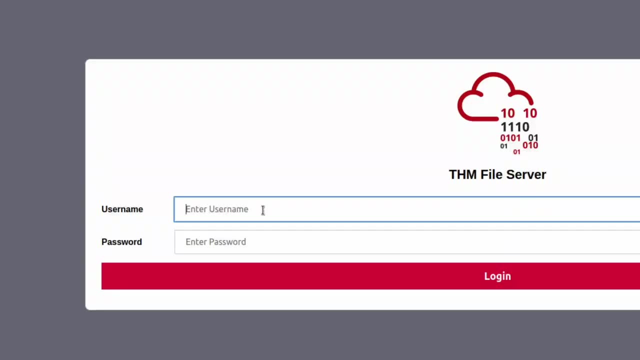 password before i set joseph's password. so what does that tell you? it'll tell you that i've strengthen the login page and we're going to log in as joseph. see how easy that. this is obviously an exaggeration because it's not going to be that simple, but uh, it's just to kind of prove the. 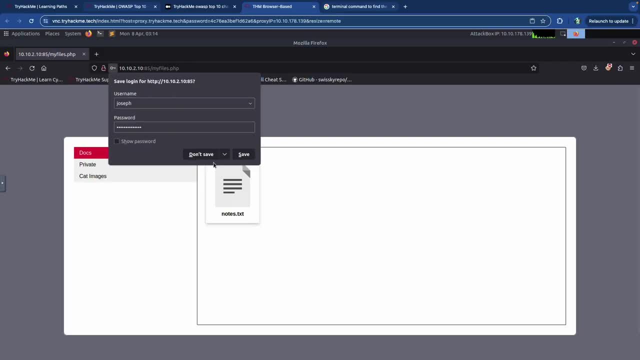 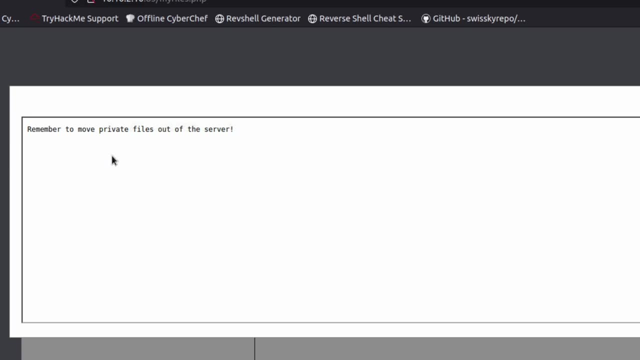 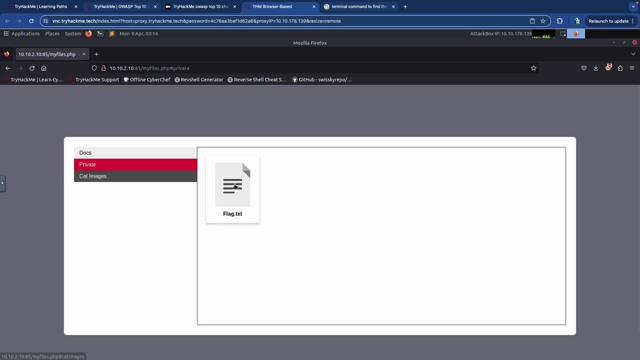 point and drive the point home. and so when we log in as joseph, there's a note here and if i go inside the note it says to move private files out of the server. okay, fine, so it's not his note private, let's go to private and see what we can get here and there you go inside his private. 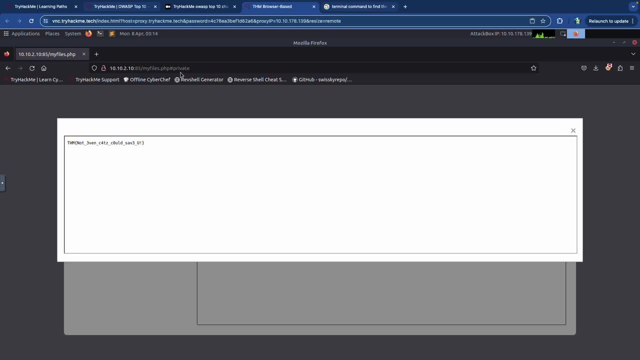 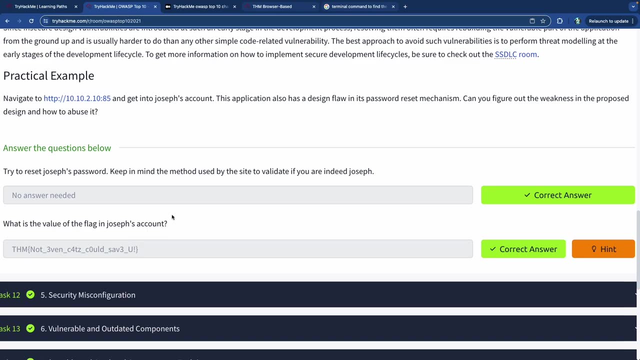 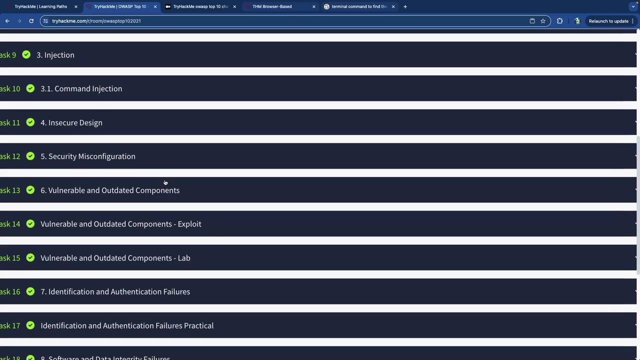 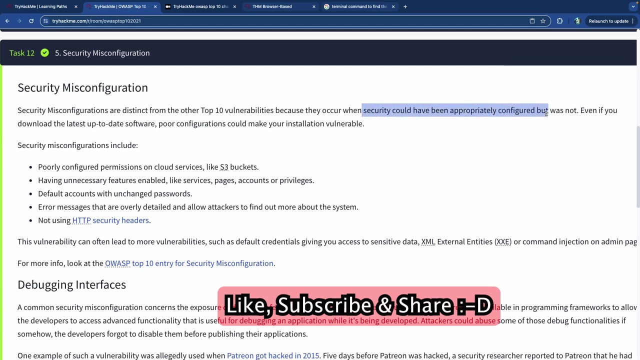 directory, there's the flag and there you go, and that's the flag, right here. not even cats could save you. that's it all right. so now let's go into the next one, which is security misconfigurations. so security misconfigurations, uh, happen when security has not been properly configured. 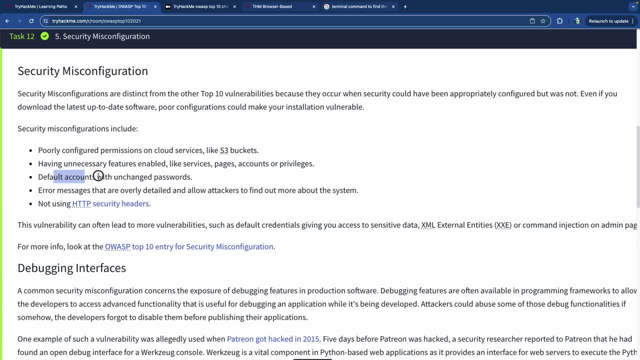 it should have been, but it wasn't. so, for example, it could be a default account that has an unchanged password. usually a system comes with a default account and it has a default password, and if they never change those things, that's a security misconfiguration. if you have a. 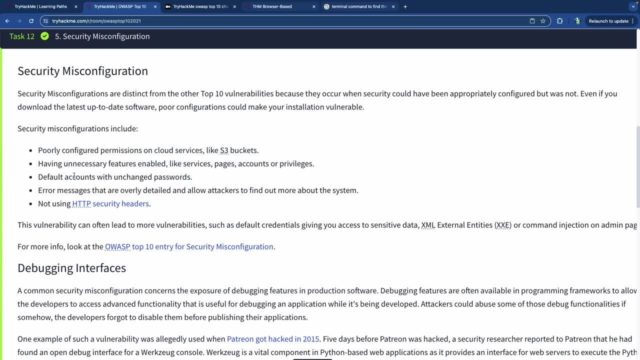 permission on your cloud services like a amazon s3 bucket. that is very, very. it's another security misconfiguration, unnecessary features, error messages that are overly detailed and allow attackers to find out more about the system. so if the error message gives a version of the os that 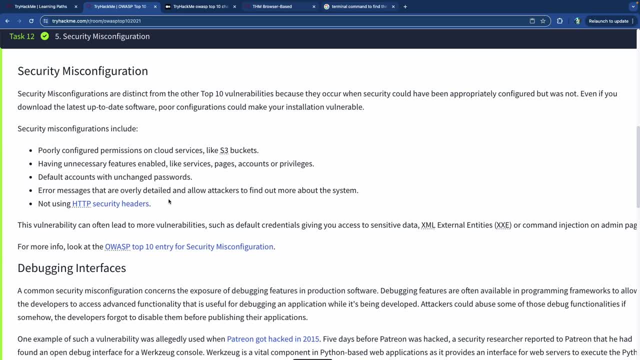 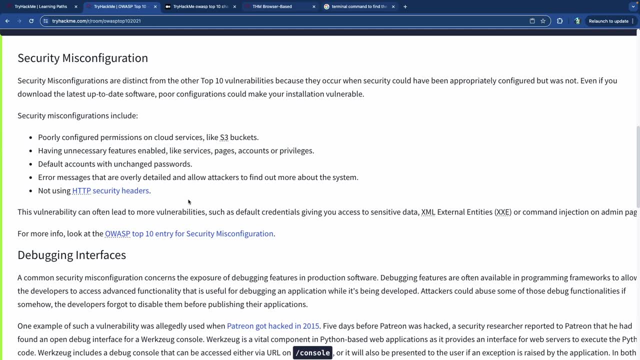 was responded, or it says that you know this command doesn't work, or anything of the sort. instead of just saying incorrect, try again. that could be information that can be exploited not using http security headers. and these are just a few of them so you can actually go to. 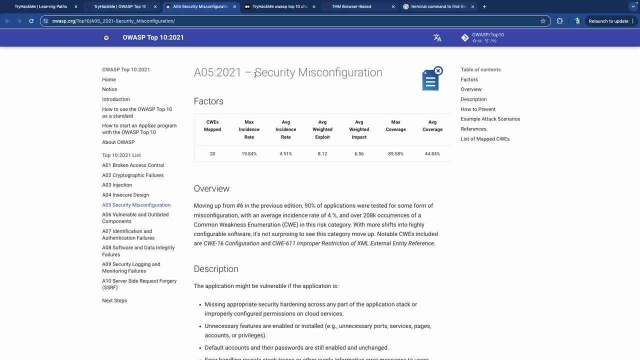 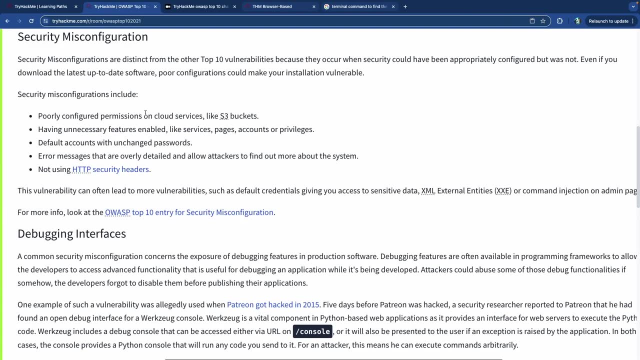 the os top 10 uh website and look at security misconfiguration and then under that, you get to see a lot more results as far as the different things that could uh, that could be used as security misconfiguration. so, uh, something that happened previously to patreon in 2015. 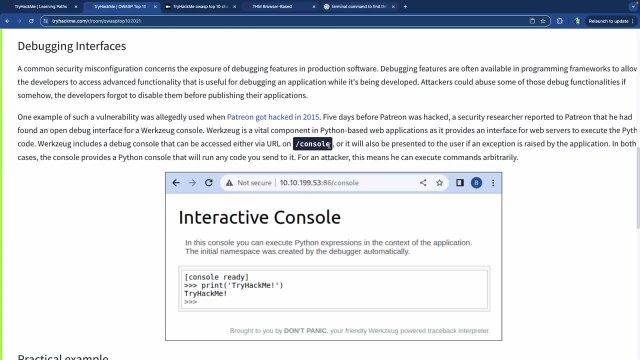 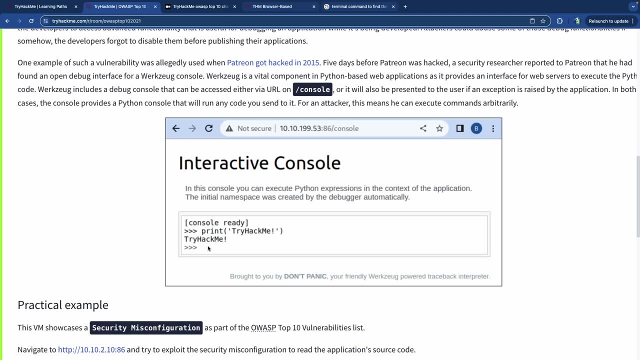 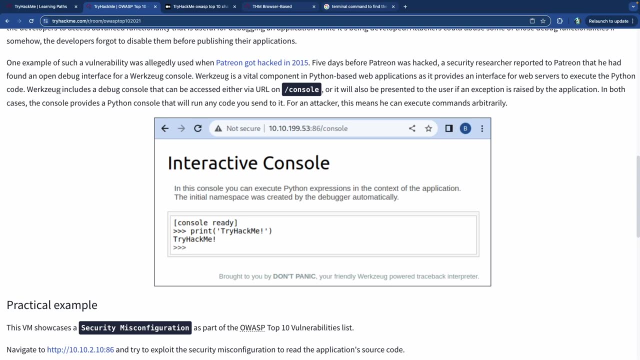 was that there's something called the console, so forward slash console, and it can give you an interactive terminal on the web page that you can print commands into and you can uh actually run those commands, And I think it's called WorkZook or WorkZook, whatever. however you 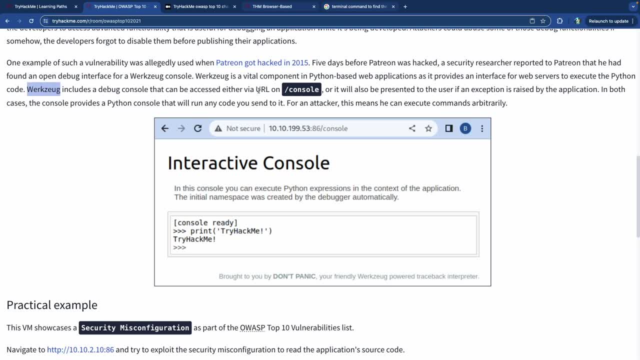 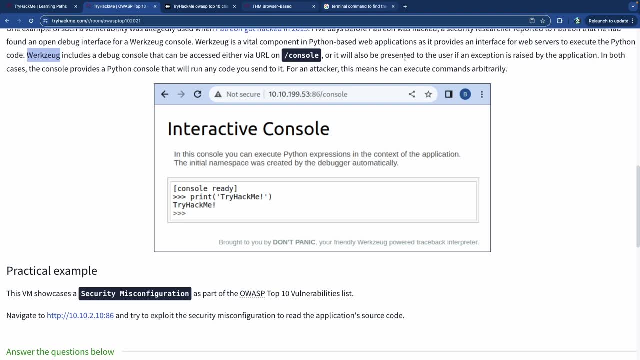 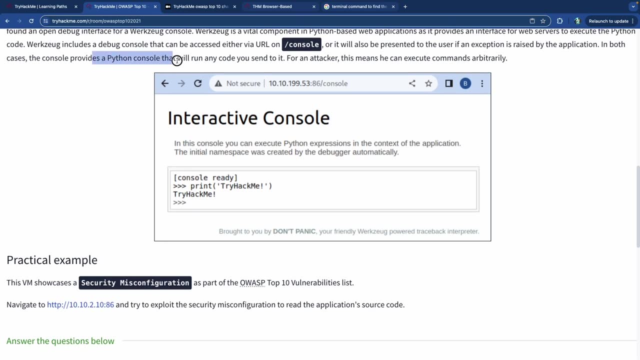 pronounce this- that gives you a console that can be accessed via a URL, And so it can literally be done in a lot of in a few different ways, because it could also be presented to the user if an exception is raised by the application. In both cases, it provides a Python console that can run. 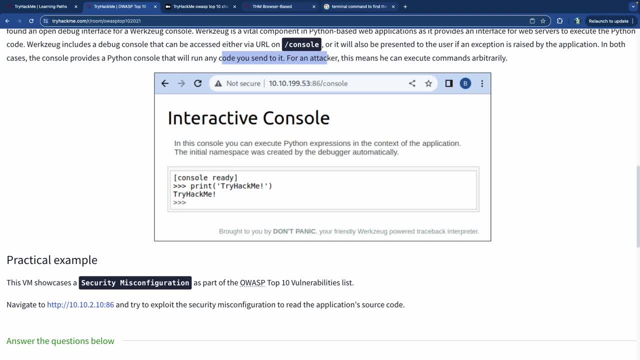 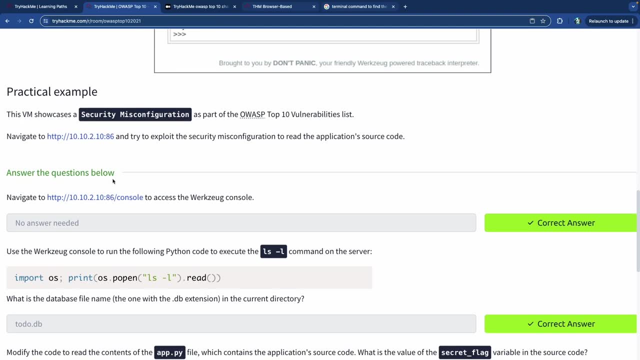 any code that you send to it. So if you know how to use Python, or if you know how to use the internet and Google, then you can try to find a bunch of different commands that you can run. So, for example, if we go to the console that's on our web page, we can run this command right here. 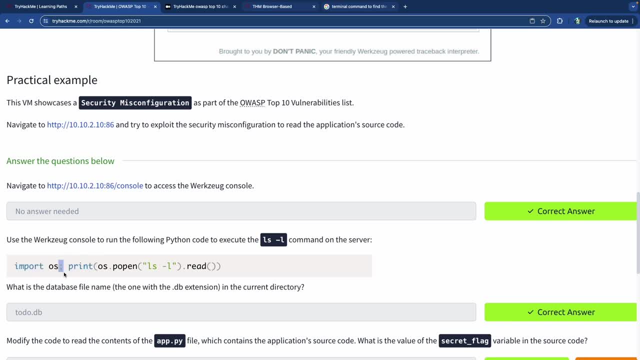 which is importing the OS, and then you do a semicolon and then print onto the screen, which is ospopen, and then this command, and then read it. So that's the command itself. that's being done with Python. So this is actually two commands that's being run. Number one: 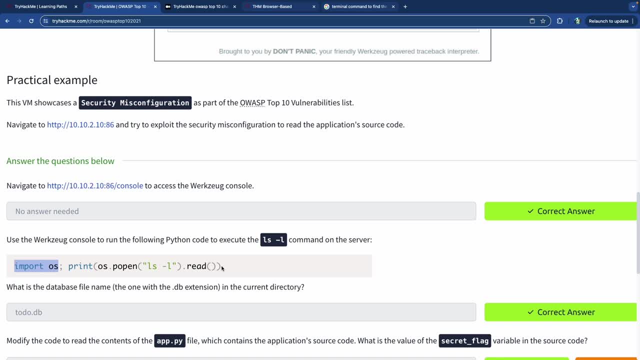 it's importing OS So that you can run OS commands, And then the second one is the command itself. So I'm just going to take this exact same command and I'm going to run it, And in this case it's going to. 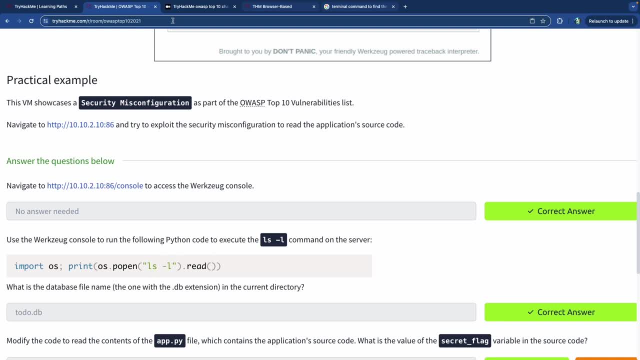 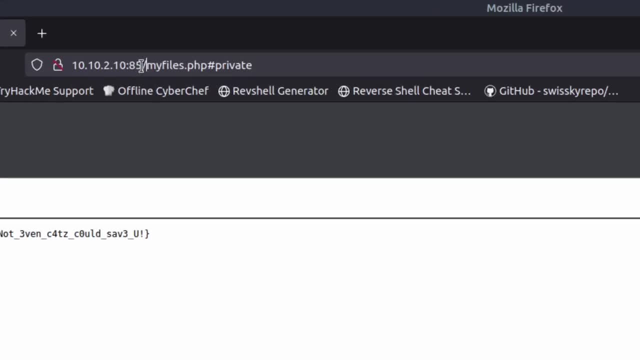 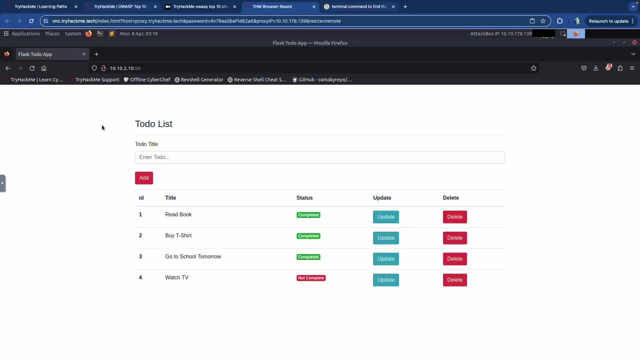 give us an LSL, meaning it's going to list whatever's inside of our our terminal. So let's go into the next port on our website here and run those commands, All right, so this is the, the website itself. nothing exciting to do here. So what we're going to do is we're going to go to 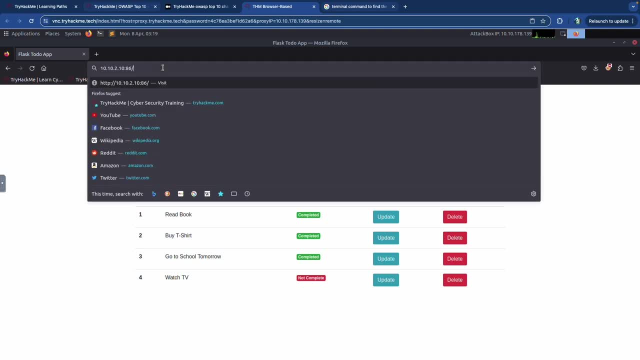 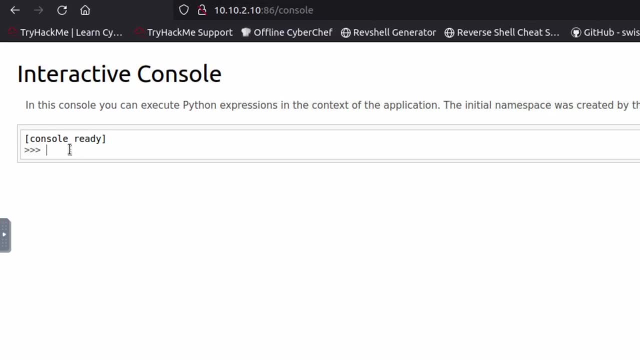 forward slash console, because that's the one that they gave us And let's see what we can do. There you go, We have the interactive console here ready to go, And so I can just drop in import, OS, print the command, and then we're going to run it And there it is. These are the contents. 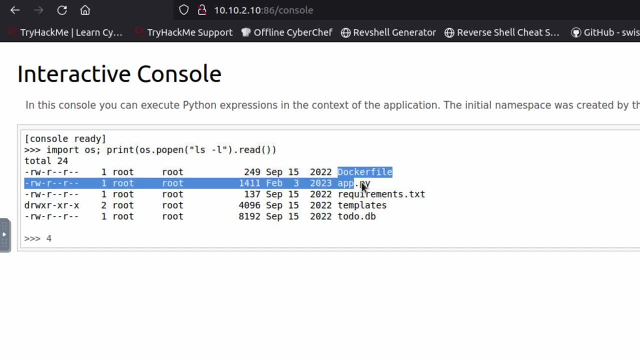 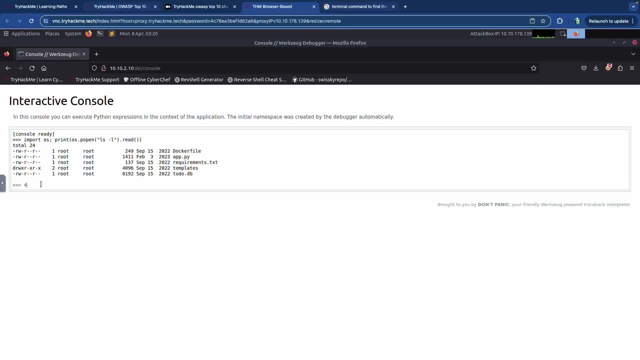 of our command here. So you have apppy, Docker file requirementstxt templates to do dot database. So we have a bunch of things that we can run here. So what is the question it's asking us? It says what's the database file. So to do dot. 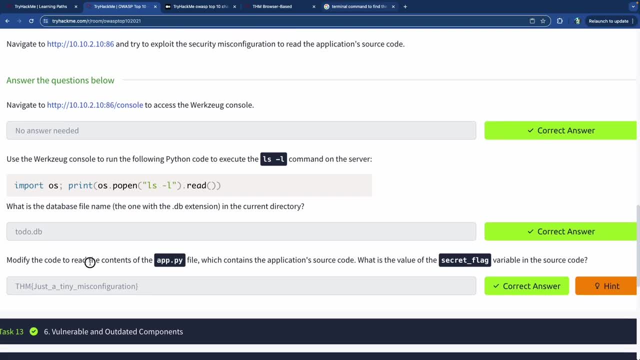 database. that's the question here. And so now it says: modify the code to read the contents of apppy, which contains the application source code. what is the value of the secret flag in the source code? So all we need to do is just read this command right here. So we 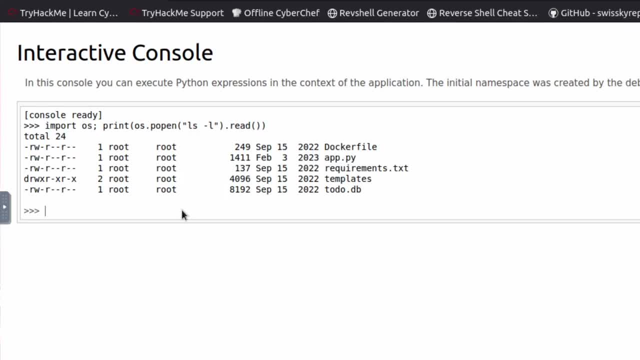 want to read the apppy command. So I'm literally going to do the same thing. I'm going to drop this in here. I'm going to repaste that original command. Oh well, I didn't. I didn't copy it. 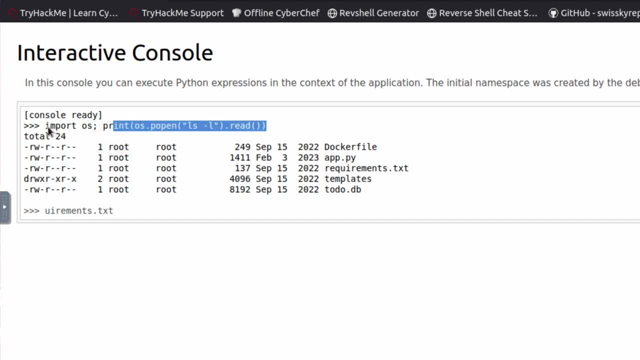 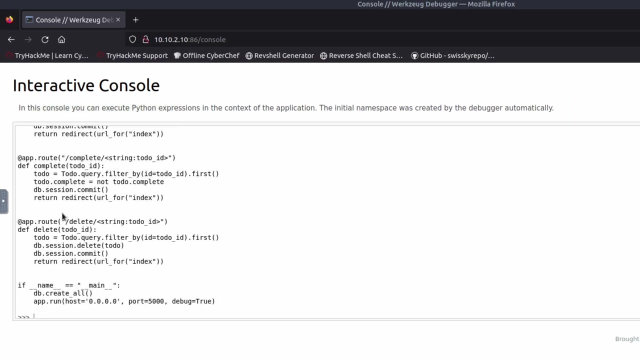 for whatever reason. So we're going to take this command and we're going to repaste this thing, And then it's going to be the cat apppy. That's the command that we actually want to run, And there we go. So these are the contents of the apppy file. So now what we're looking for. 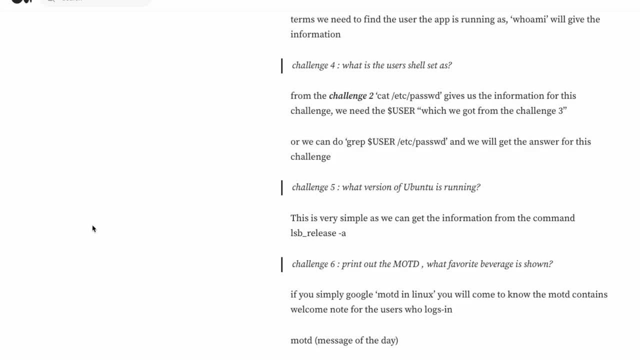 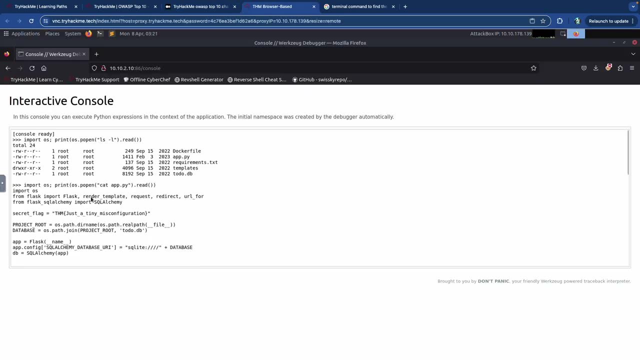 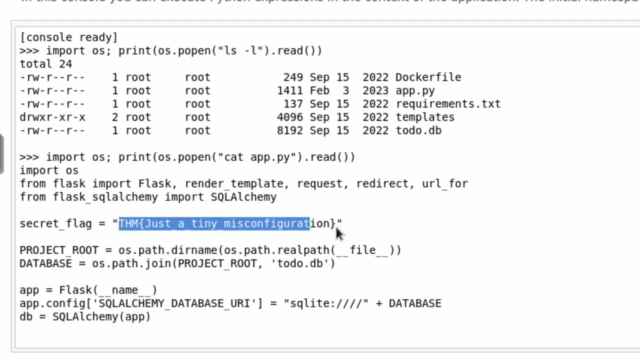 is the variable that? what is the variable called? The variable is secret flag. So we're looking for the secret flag variable on this page. So let's try to. oh, there it is, It's literally right at the top. So, secret flag, thm, yada, yada, yada. tiny misconfiguration, And so we copy this. 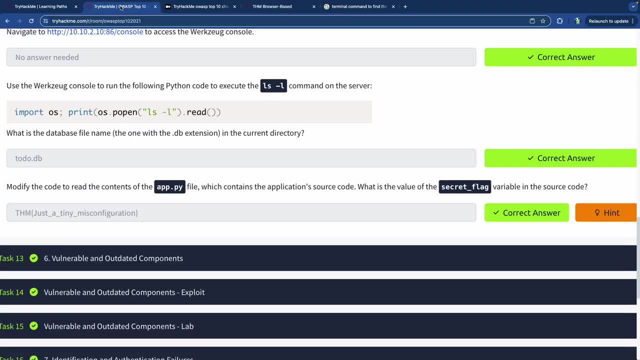 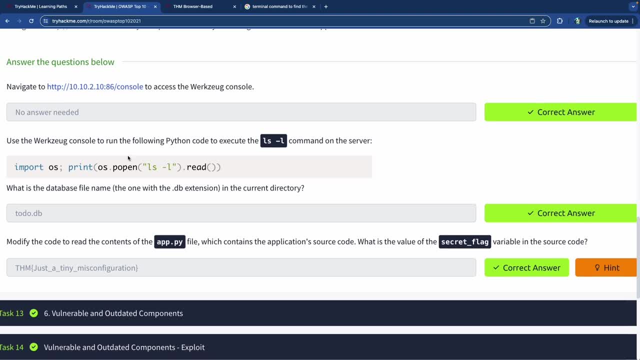 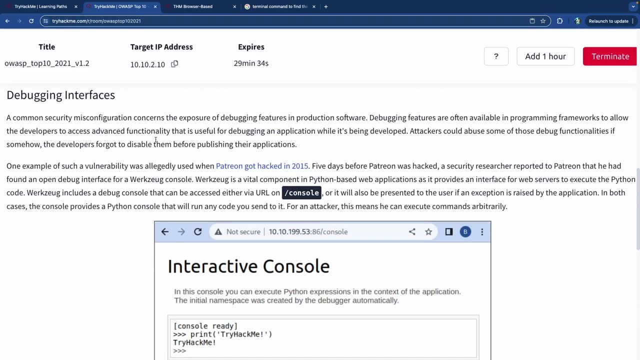 That is our flag, which is just a tiny misconfiguration, So easy, like super freaking easy. But yeah, that's another one. So this is a security misconfiguration that allows for a console to be presented to somebody that has access to that link And then, if you just go to 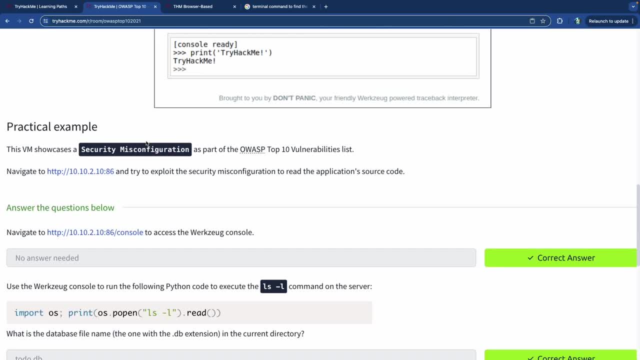 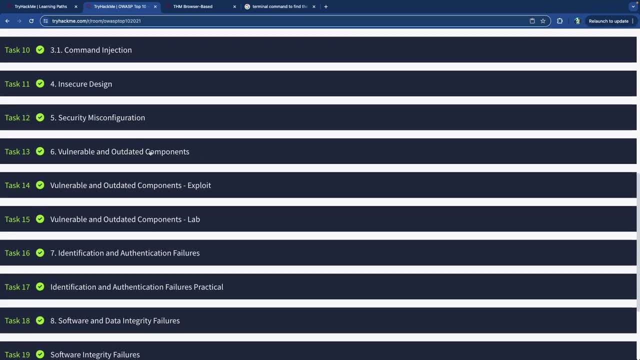 it and you know anything about Python, then you can. you can run your Python command and get information that you shouldn't have access to. So that is security misconfiguration. Let's talk about vulnerable and outdated components, which is I mean this one's. 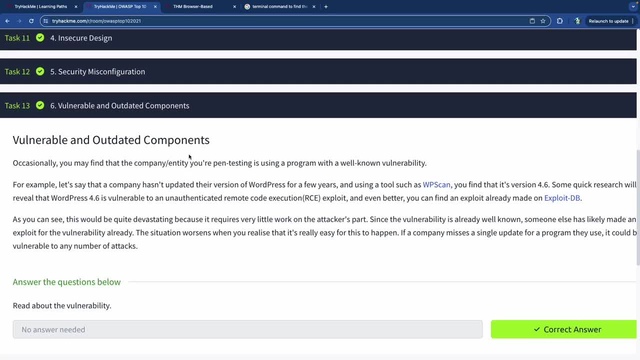 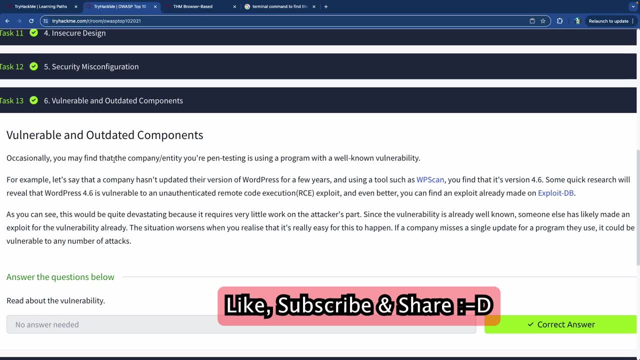 pretty self-explanatory. I feel like we don't even need to do this, but let's just. let's just read through it. Why not? So if your website is outdated, if your computer is outdated, any of those things? obviously? So in this case, we're talking about web applications, So it's it would. 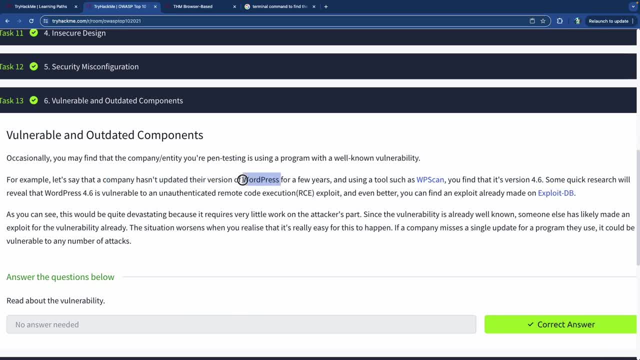 be the website. If they're using WordPress, for example, and if they haven't updated their version of WordPress in a while, you can use something called WP scan, which is a terminal command line for a freaking easy to use and it can give you the version of WordPress. And then, if you look, 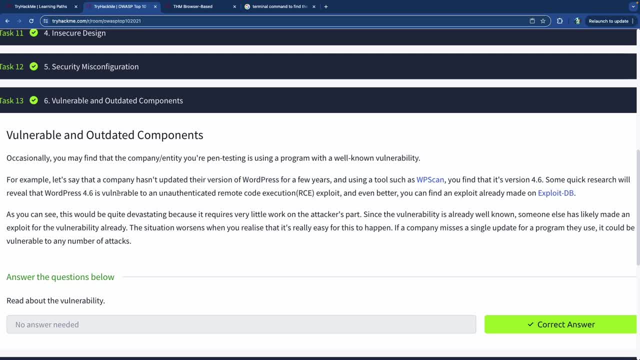 online. you can see that for WordPress 4.6,, for example, there's a vulnerability for remote code execution. And then you can go to exploit database, which is a large database of exploits that are already pre-written, ready for you to use at any point, And then you can just use that exploit. 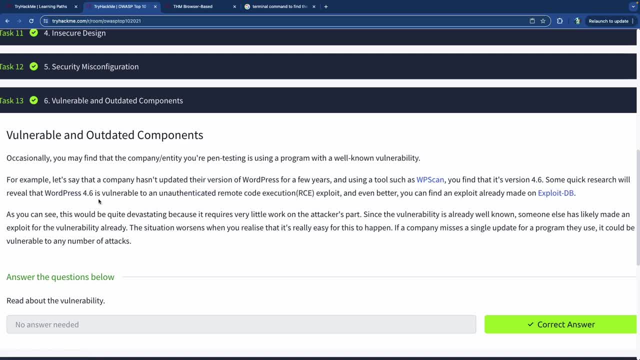 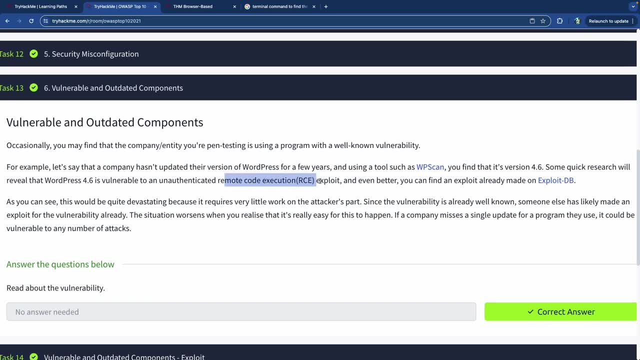 That's been given for WordPress 4.6, and then get into their website right And execute- execute some remote code. This would be very, very bad because it doesn't require any work, very, very little work on the attacker's part, And then they have access to the kingdom. 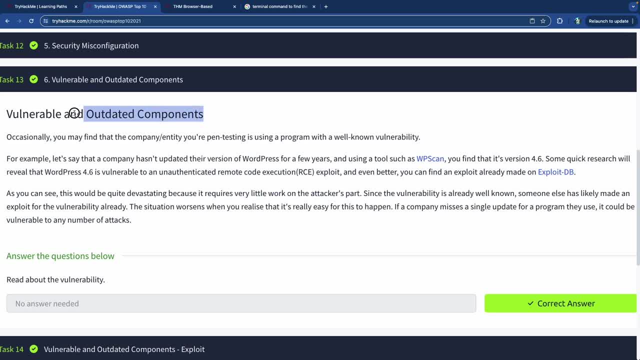 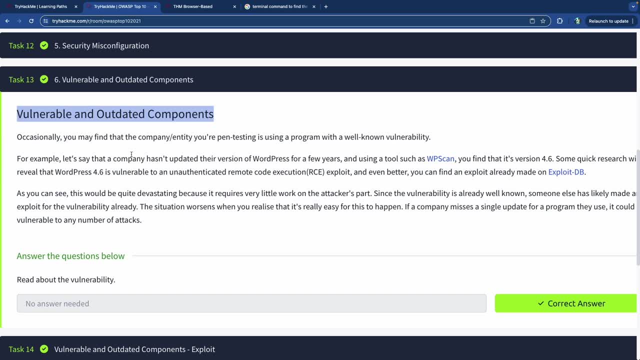 So this is what is horrible about having outdated or vulnerable versions of websites or versions of portals or versions of the. what are they? They called the web builders. right, These are. WordPress is technically a web builder and it's a platform that you can use to build your website, And it's really really common. 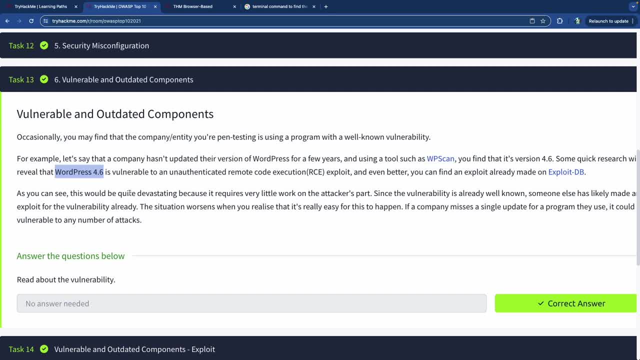 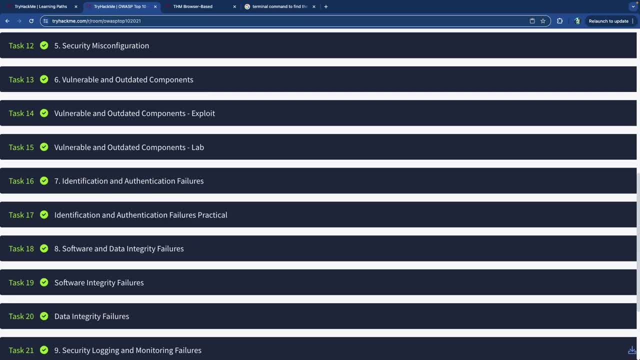 And a lot of people use it. I use it. but if it's an outdated version, if it's an old version of WordPress, that means there's probably a vulnerability that exists, and somebody could just go find that vulnerability really easily. And so you guessed it right. We're about to go and 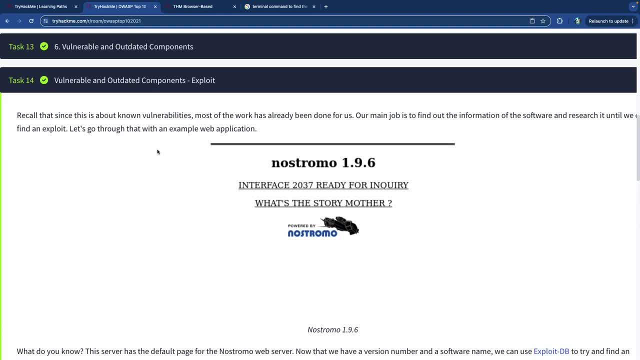 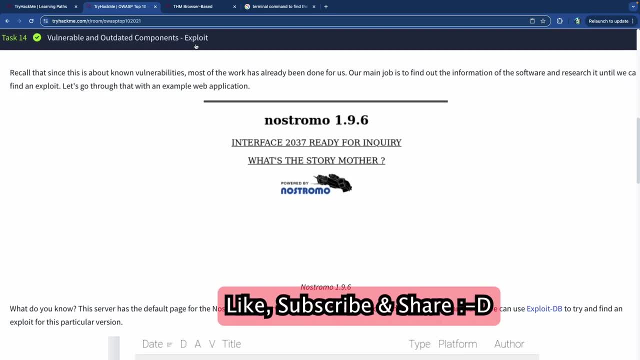 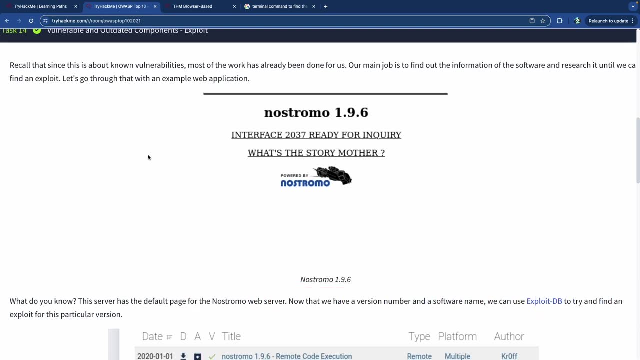 actually find some exploits to be able to run against this website that we got, So let's do that. This is an example exploit. that is for the Nostromo 1.9.6, a web server, And so. on this website's homepage there's the actual version of the web server that they used, And so if you 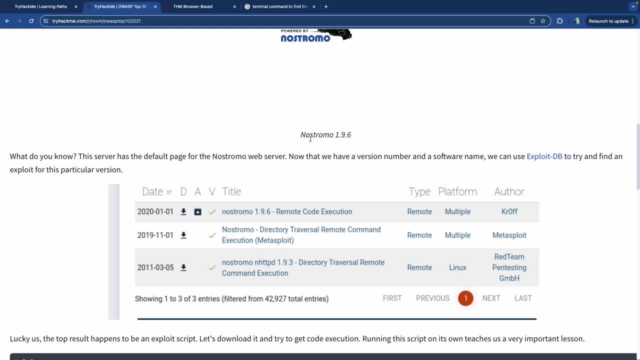 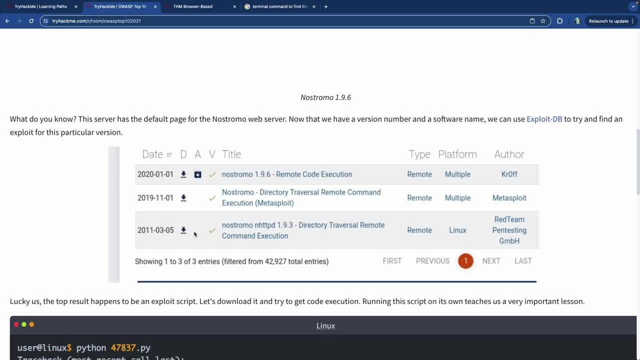 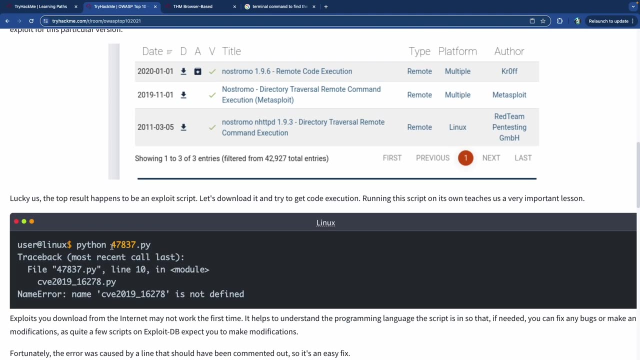 go to exploit database and then just search for Nostromo 1.9.6, then you get a list of a list of exploits that come pretty. they're just built for you And then you can just download any of them and use any of them. So in this particular case it's a Python file And if you run it, 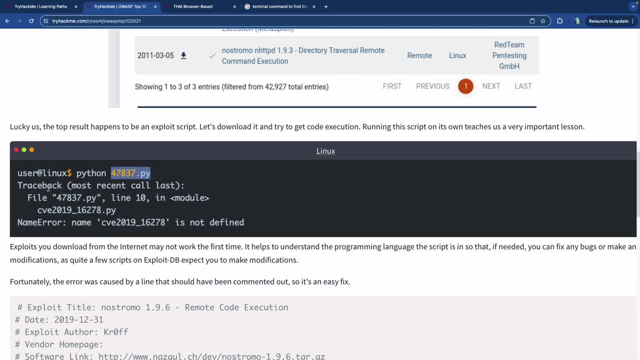 then it gives you certain things. So it says: you know, in this particular case, when they ran it, it gave back an error And it said that the variable right here is not defined. Now, if you know anything there is to know about Python, you can kind of just read through the 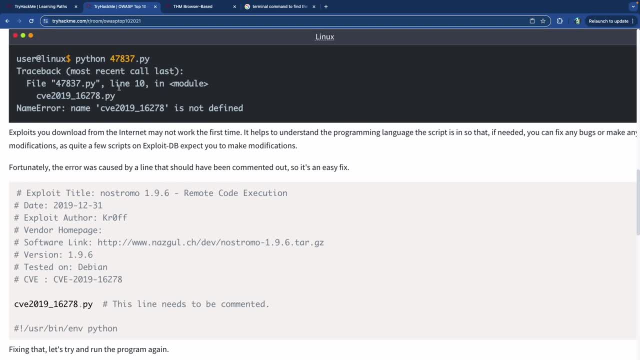 Python code and see what the issue is, And it actually it's nice because it gives you the line of the code that the error happened in. So it says in line 10, there's this thing and it's not defined. And in this case there was a. 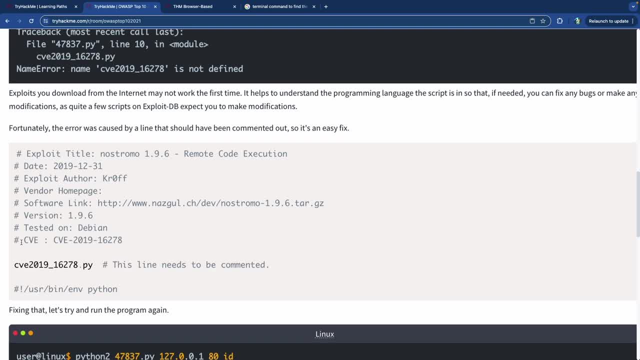 comment right here that says this line needs to be commented, And all you need to do is put a hashtag in front of it and it will comment this out, and it won't. you know, the same error won't be caused anymore, And so when you do that, you run the code again And in this particular case, you also have 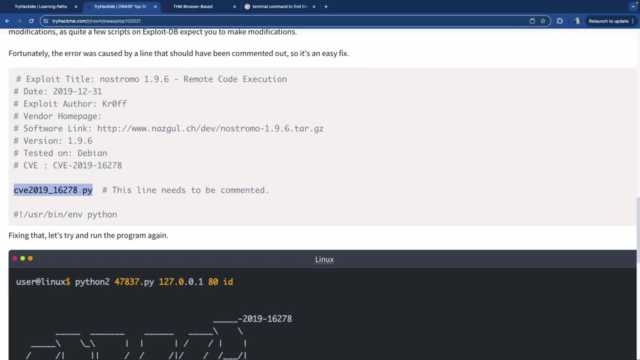 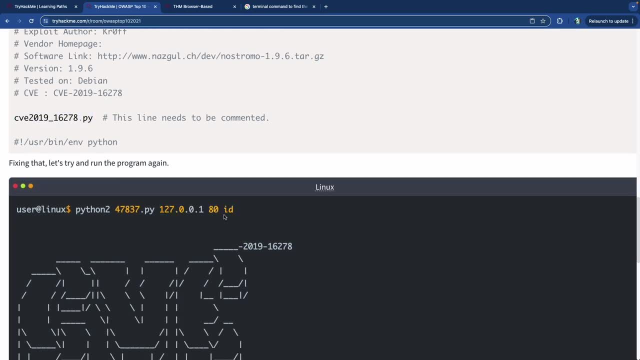 some instructions. I think that told you that you need to potentially use the. oh no, this is just the IP address and the port that you want to do, And then you use the port and IP address that you want to attack and then you just use the ID command. So it's just the terminal command, that's. 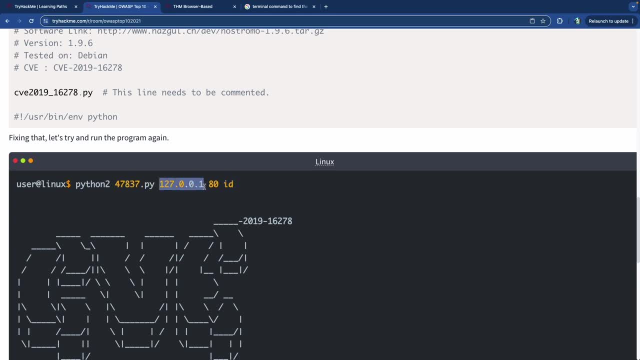 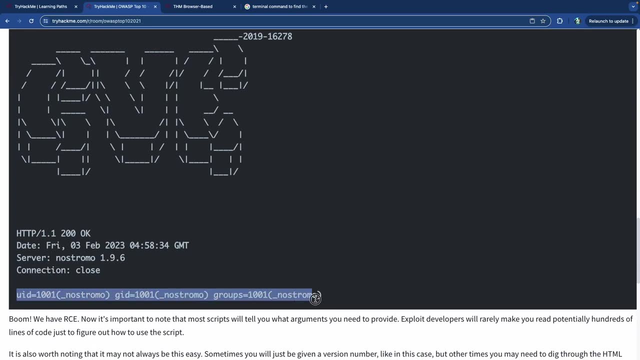 going to run. So you do Python, the file itself, the IP address and the port, and then you do ID and it'll run and it'll give you back the ID, which is, in this case, this information. So now, 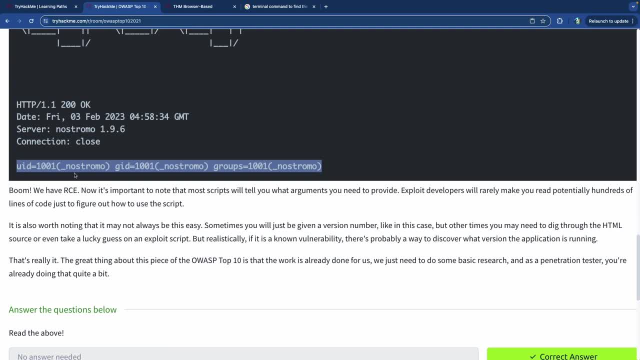 we have remote code execution happening And then if that means, if that ran, that you could probably run any other code As well and you'll probably be met with some kind of a successful output. So most scripts is going to tell you the arguments that you have to provide. They rarely make you read potentially. 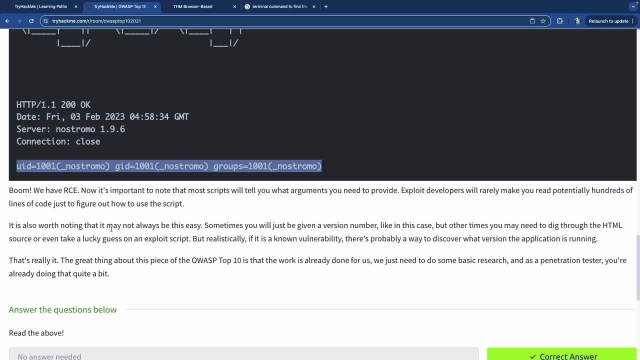 hundreds of lines of code to figure out what you need to do. So that's one of the things that is really nice about a lot of these exploits that have been pre-made by these hackers and left on exploit database for us. So it's scary, Like the more I go through stuff like this, I'm like 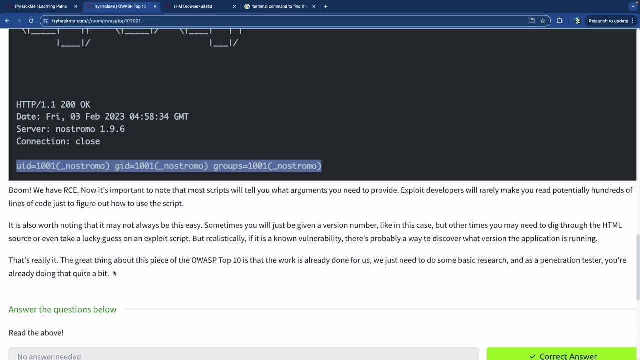 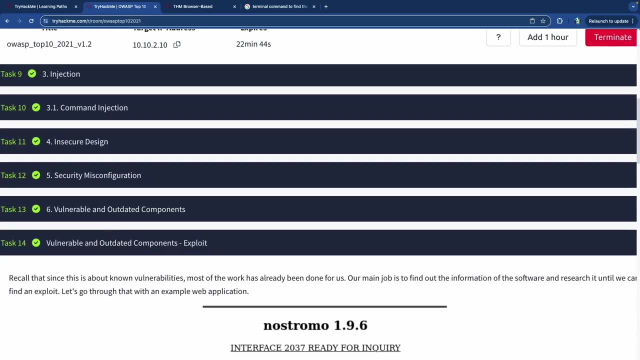 damn dude, I can't believe that it's that easy Sometimes. So, anyways, this is it for this particular exploit example. So now what we're going to do is we're actually going to do a lab on this. We're going to try to find some kind of a 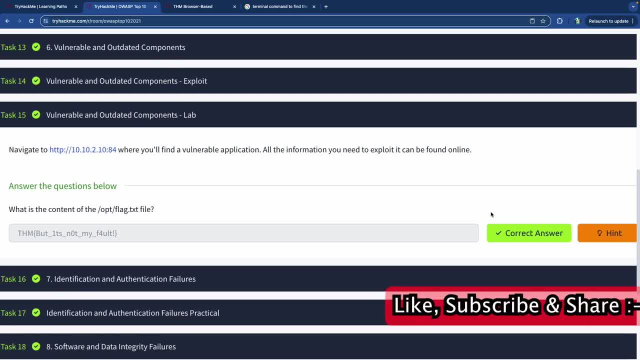 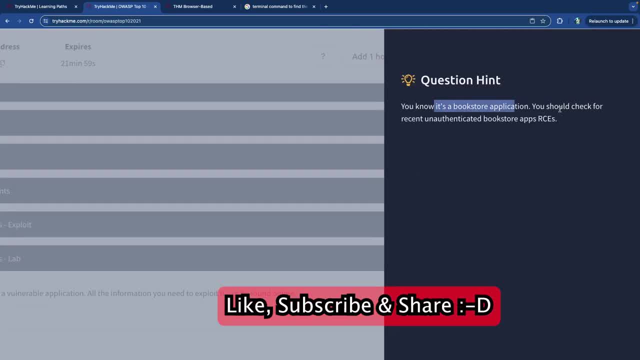 vulnerability exploit for this webpage. All right, so this is it. That's going to be our URL that we're going to go to. There's a hint here: It's a bookstore application. you should check for recent unauthenticated bookstore app remote code execution. So that's what the hands gave us, And 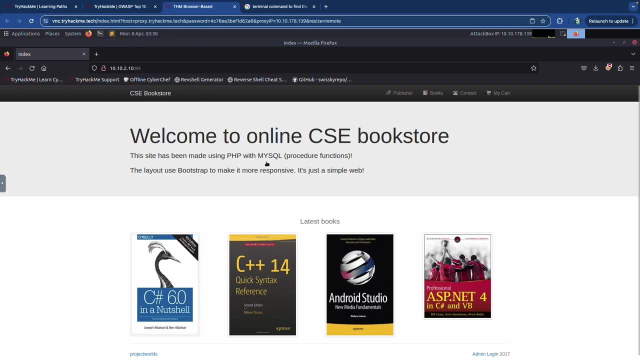 so this is the actual web application It says: it says CSE bookstore, and my PHP, my SQL procedure, functions, so on and so forth. admin login 2017.. So let's click on the admin login at the bottom right here. see what we can find here. 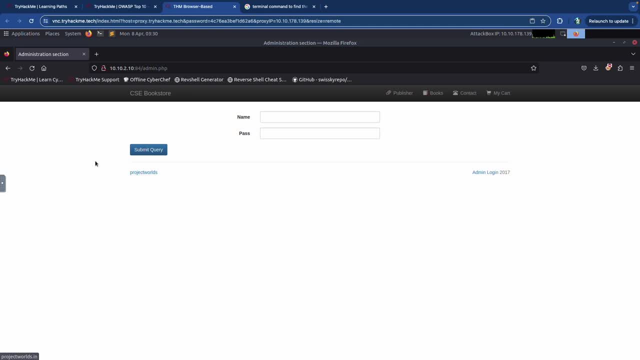 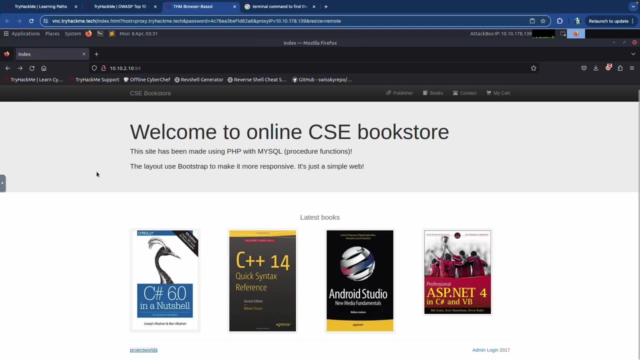 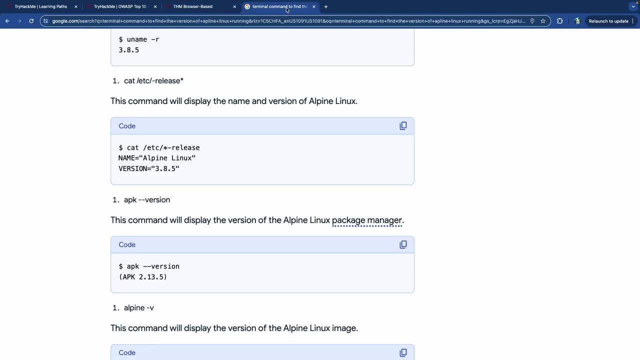 Nothing to see here. Let's see what other information that we can find that might be able to make it easy for us to find an exploit for this. Okay, so there's nothing there. I am going to just run with this And let's go search for CSE bookstore to see what we can find on exploit DB. 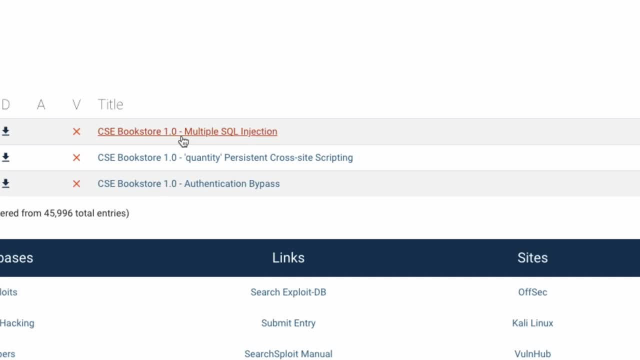 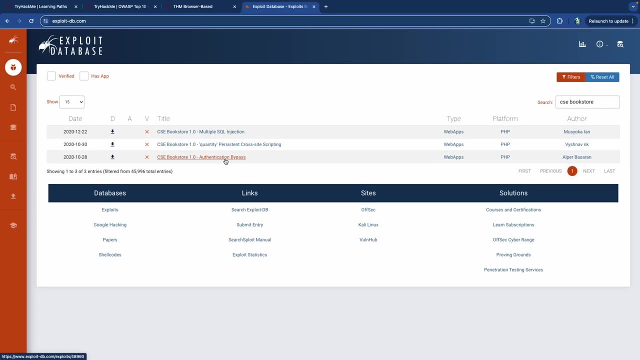 Okay, so there we go. CSE bookstore actually shows up And we have multiple SQL injection, persistent cross site scripting, authentication bypass. These are some of the things that we can do with this, So let's see which one will end up working for us. I think I actually need to do this on the. on the. 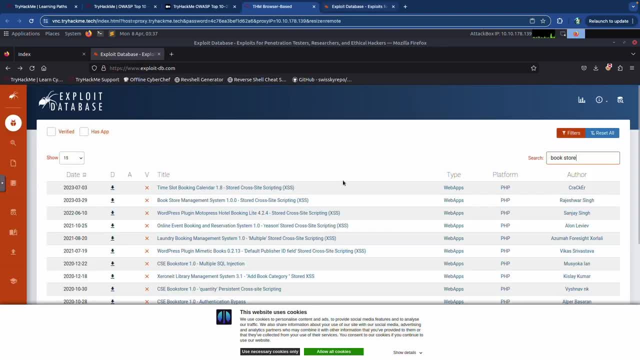 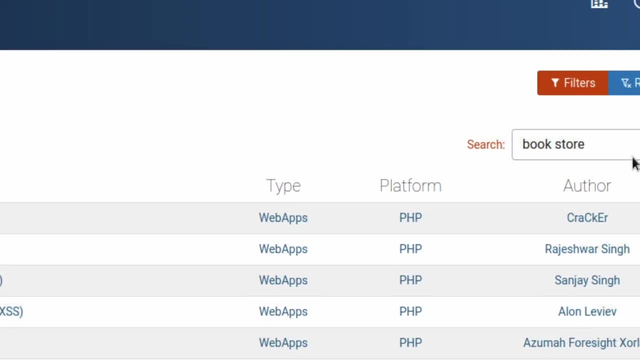 browser of this thing Right here, So let's go here and do it. Alright, this one. actually, I had to do a few different types of searches, So when you do bookstore as one word, you only get four different exploits that show up, And 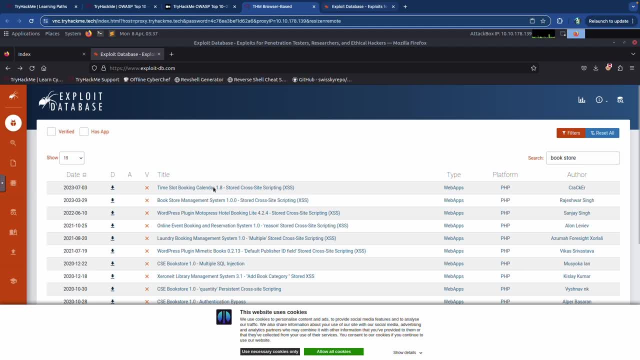 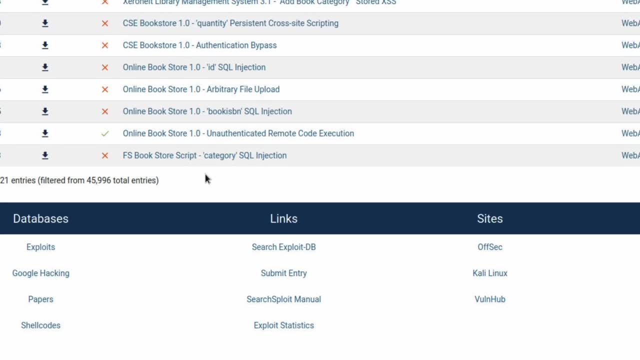 then, when you split it up between, when you turn it into two words, basically, you get a much larger list of exploits that come out. And then there's one in particular that I believe is the one that I used last time, which is this one: it's the only one that has a checkmark next to it, So online. 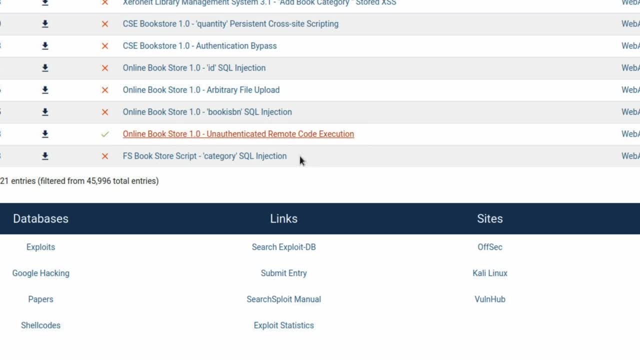 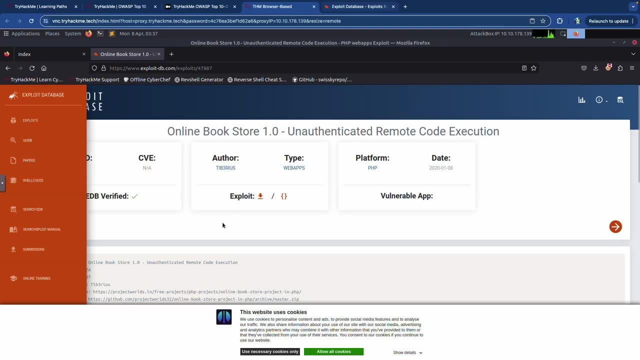 bookstore: unauthenticated remote code execution. And this is the one I believe. Yeah, so this is also the ID 47887.. So this is going to be the one that we're going to use And since I'm already inside this attack box, I'm just going to download it And then from here we're going to modify some of. 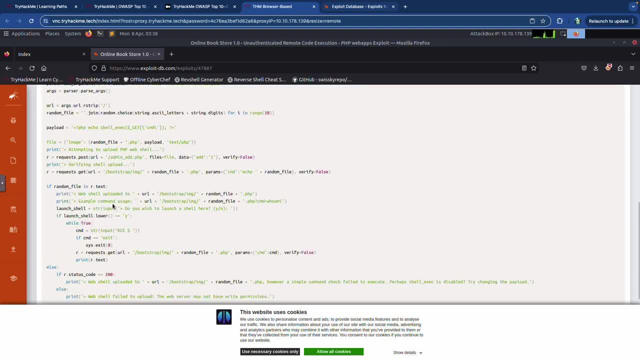 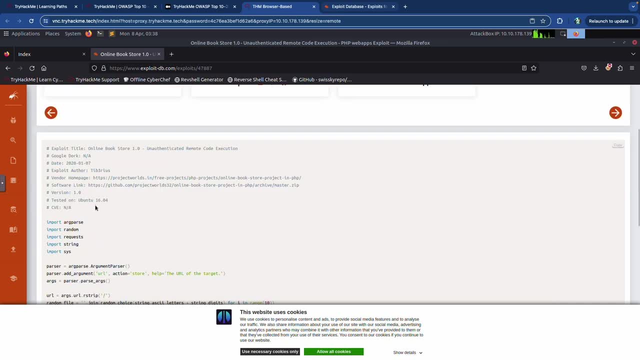 the code And what we're going to do is we're just going to read through the instructions here And I think it should be fine. I don't think there needs to be anything that I need to really modify the code. So we're just going to modify here, But it gives us the comments at the very top, So exploit. 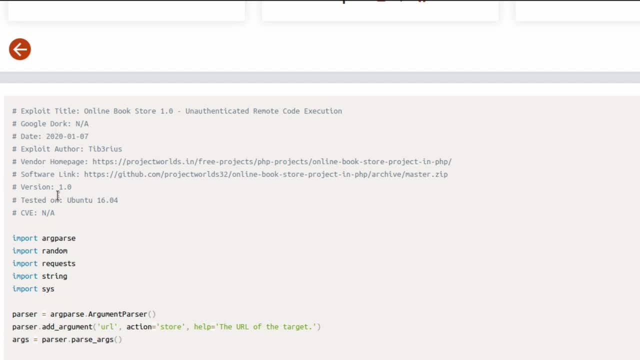 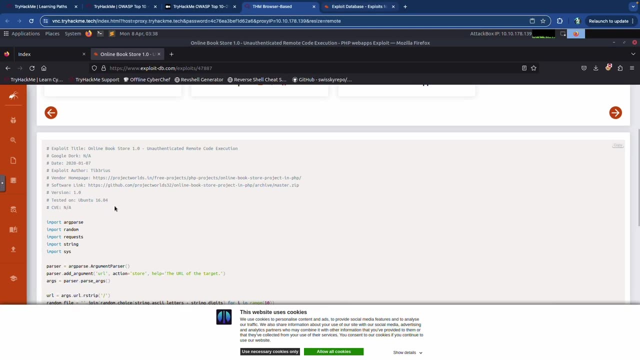 is this Google Doc, not a data vendor homepage. software link, tested CV and a, And that's basically it. There's really nothing else that's been listed here As far as instructions. I'm going to look at the rest of the code to see if there's anything that we need to modify, But I 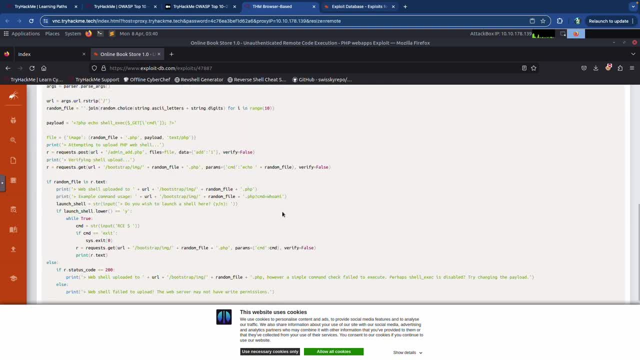 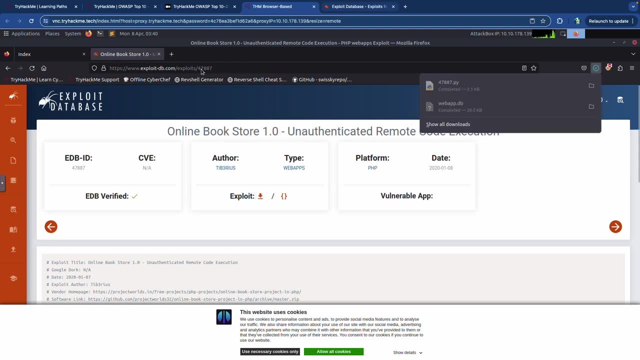 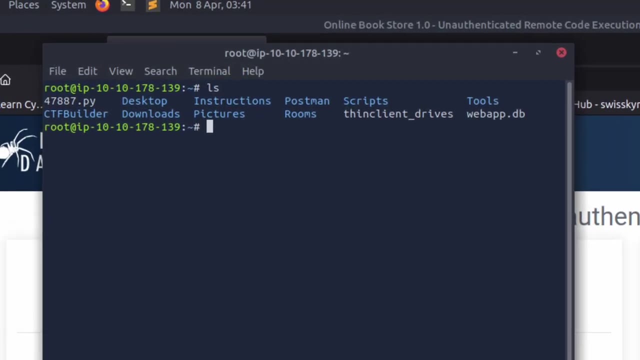 think this is pretty much it, So let's check it out. All right, there were no other comments to check out, So I'm going to download this thing And then we're going to run it in our terminal on the attack box and see what we can get out of here. All right, there is my file 47887.. Right here, This is our. 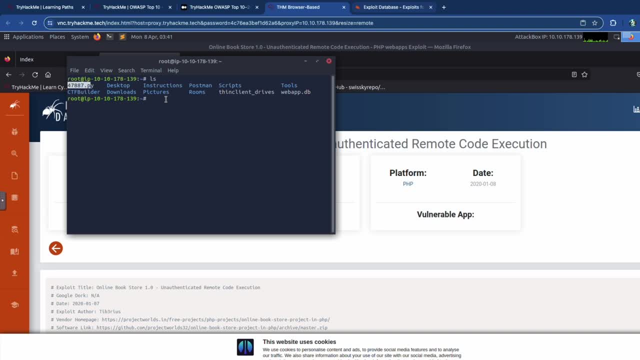 Python file And we do need to provide an argument, which is basically what we want to apply this code to. So I think it's maybe Python three that I got to use- We'll see which one of this- 47887.py. And. 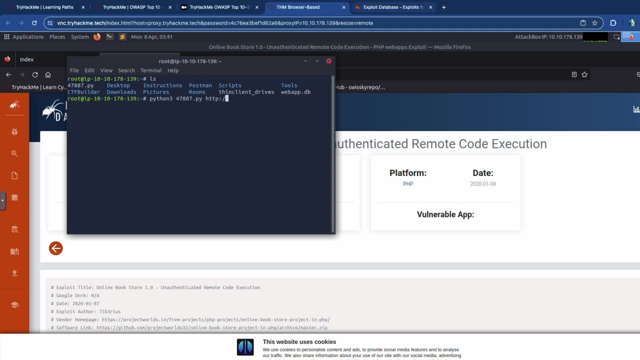 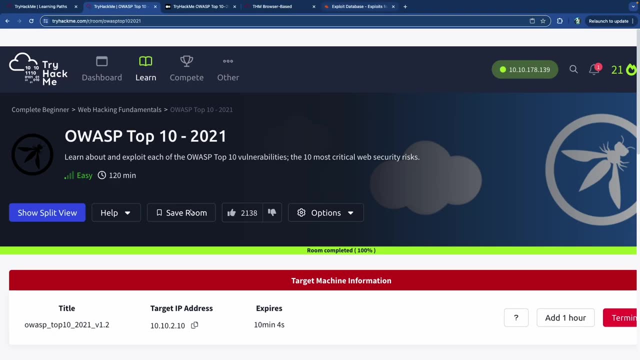 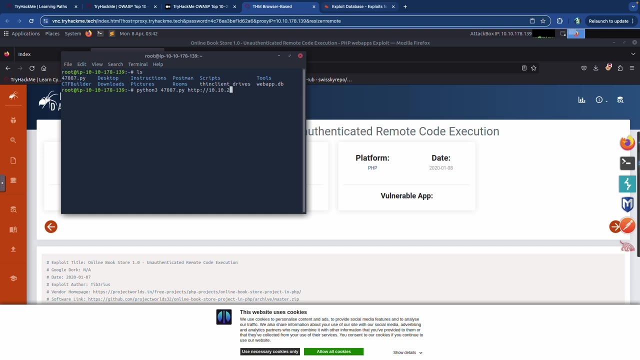 the reason I really want the website that we're trying to hack, which is- let's see what was it- 1010 to 1084.. And let me extend this thing so it doesn't die on me: 1010 to 1084. Okay, cool that. 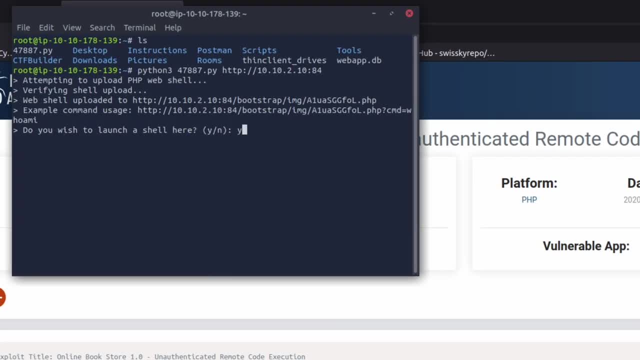 worked, And so it was a. do you want to launch a shell here? And I do want to launch shell? There we go. Our want to launch shell, there we go, rce. so if i do ls, hopefully it'll work. it'll give me something. 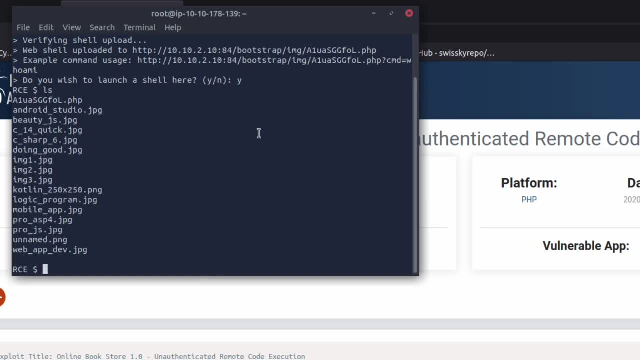 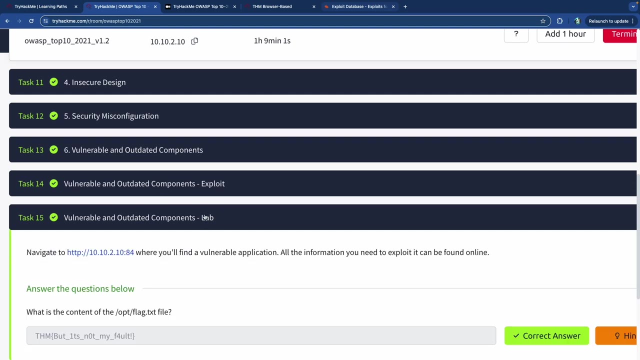 there you go, look at that, so we have all the information and it actually listed everything that we're in. so if i do print working directory, for example, it should tell me where i am, and it is definitely working. so now, what is the question? uh, the question: where is it lab right here? so it. 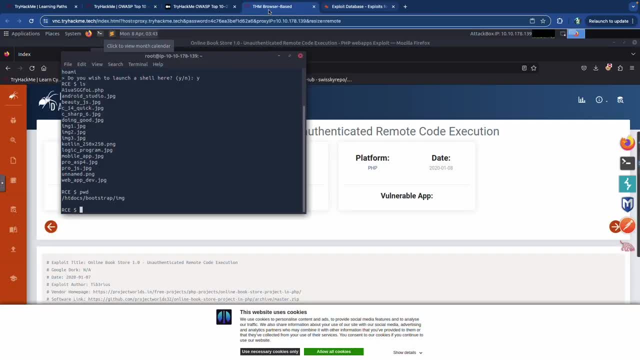 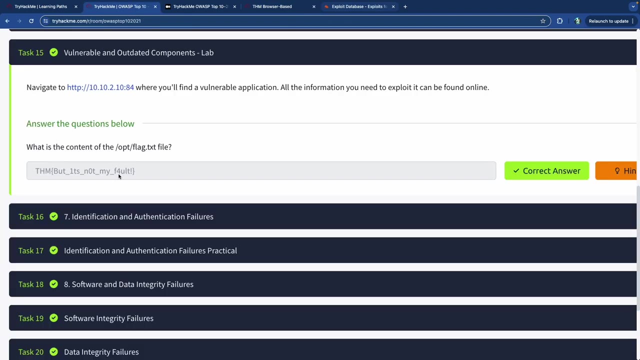 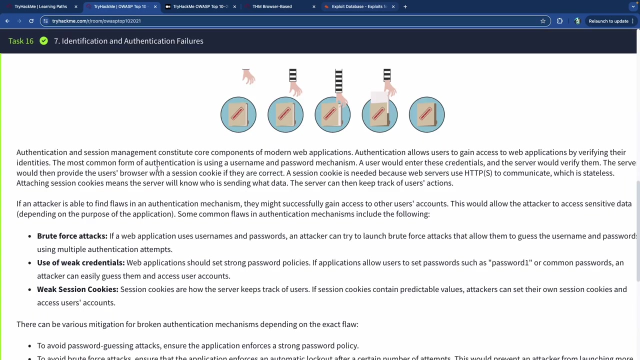 says what is the contents of the opt flag file. so i just really need to do that. so i'm just going to do cat opt flagtxt, and there we go. and there it is thm. but it's not my fault, but it kind of is, though, and there we go. that is it. so let's move on to identification and authentication failures. 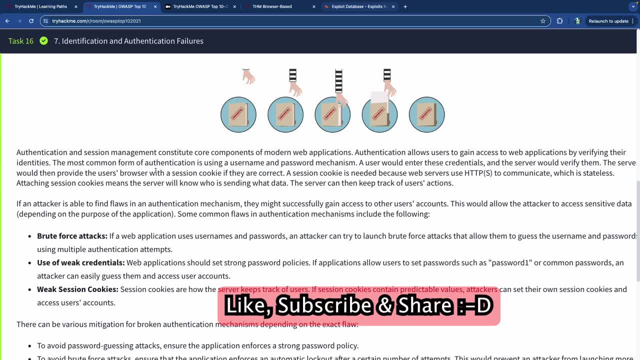 all right, this is actually a big one, and i think it's very, very important, uh, to understand how this whole thing works. so i'll just get right to the beginning of this and then i'll show you how work. So typically, when you log into a website, you provide your username and password, And then 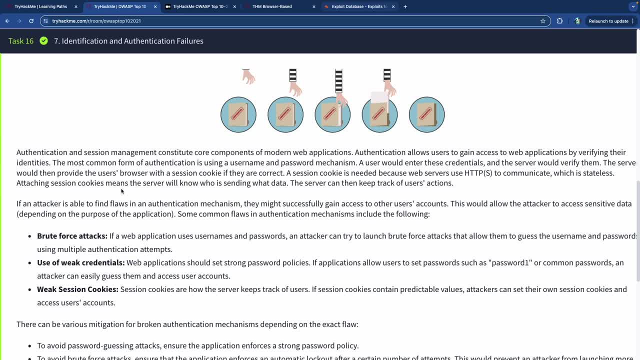 when you log in you can choose save identity right. So when you basically save your credentials into your browser and that way your browser knows that it's you And then the next time that you go to that website it keeps you logged in. So you don't have to re log in every single time And 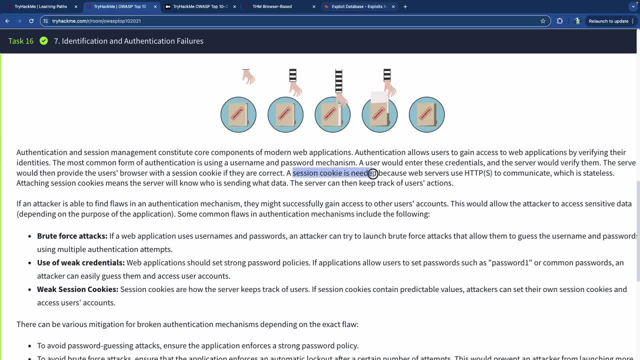 what's generated every time when you do that. it's called a session cookie, So your cookies go into your cache and it gets saved, And then that way you can essentially just revisit that website as many times as you want without having to log back in. And that's, you know, my interaction. 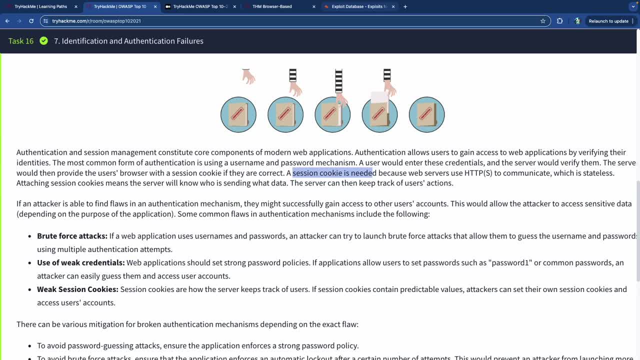 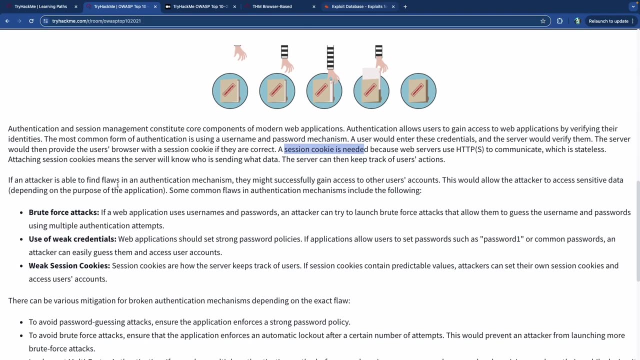 with try hack me right now is just like that right, Every time I go to try hack me I don't have to log back in because it's already remembered me And there's a session cookie that's been attached to my browser on this particular computer. So when that happens you can kind of take 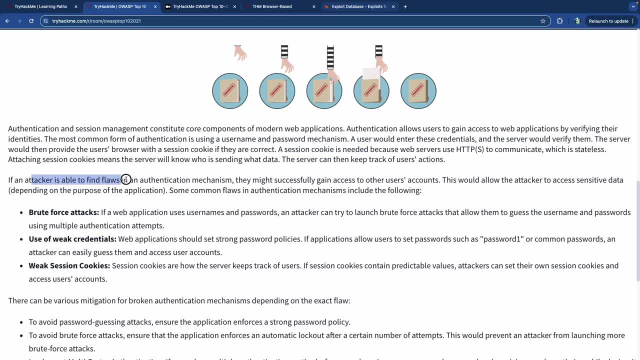 advantage of that vulnerability. So if an attacker is able to find flaws in the mechanism, they might successfully gain access to the other user accounts. this allows them to access sensitive data, And some flaws in authentication include brute force attacks. So if a web application uses username, 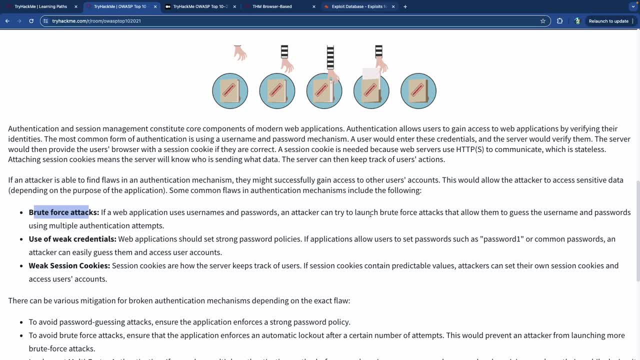 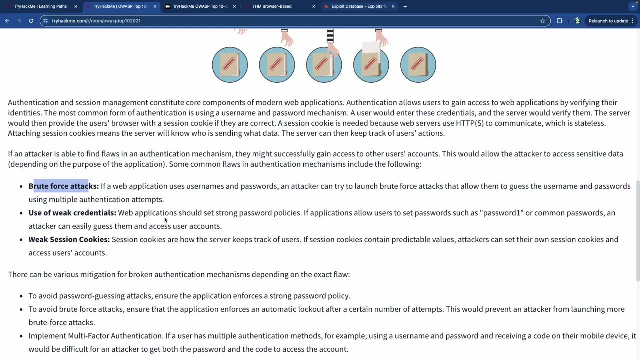 passwords they can weaken. as an attacker, we can try to launch brute force, meaning just try a bunch of different passwords using a dictionary to try to guess the username and password that's associated with it. We credentials, as we already visited crackstation, I mean. 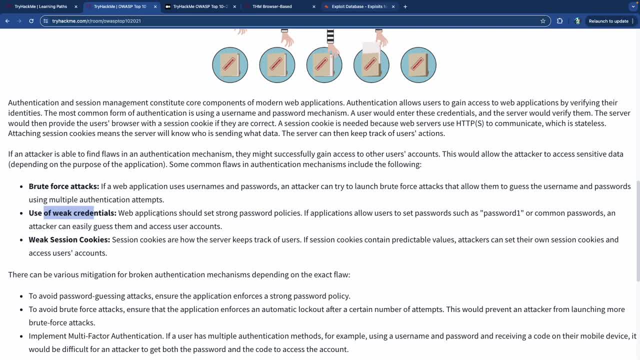 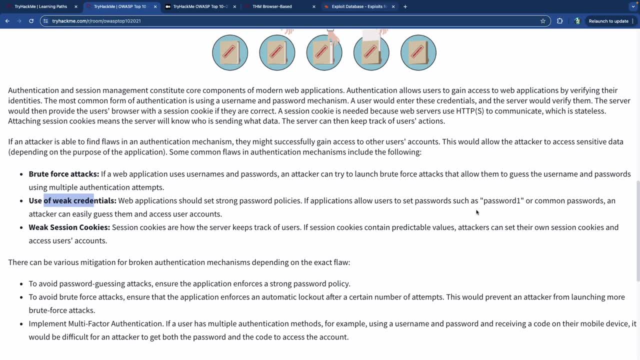 it's pretty easy to crack somebody's password, especially if they're using a weak password, And you just get their hash value and go to a website like crackstation and gives you the password. So, for example, if you use password one or some kind of easy as passwords like that, then that's it. 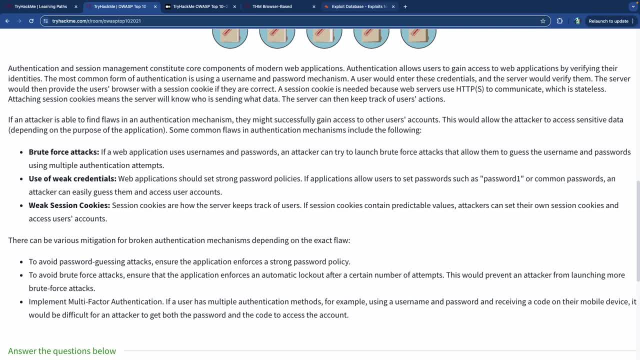 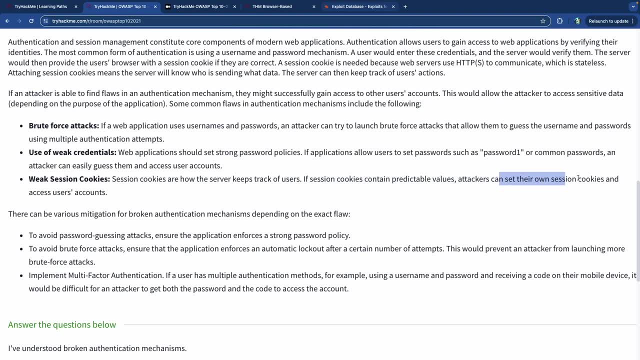 And then there's another one, which is the week session cookie. So session cookies is how the server keeps track of users, And if a session cookie contains predictable values, then we can use our own. we can set our own session cookies and user and access. 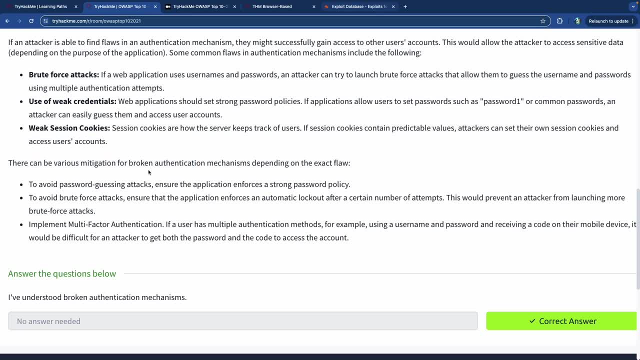 The user's account. So there's a lot of very mitigation efforts for broken authentication And, depending on what that is, you can kind of solve for it. Some of the most basic ones are to avoid password guessing attacks, to make sure that you actually have a really strong password policy. Avoid 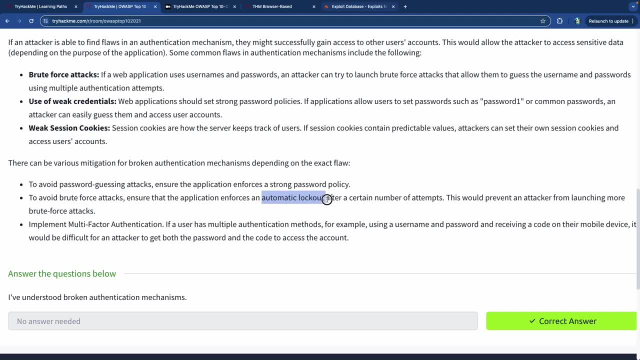 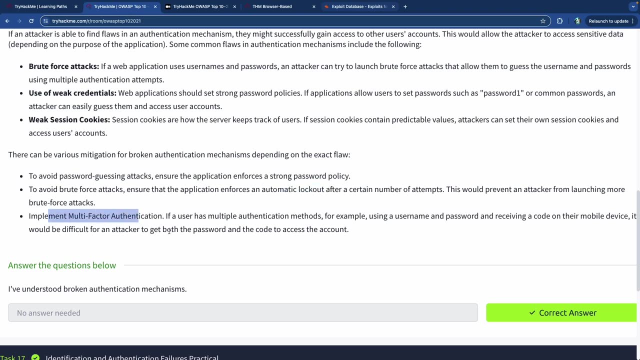 brute force attacks by doing automatic lockout as a policy, so that if somebody has three failed password attempts, then it locks them out And then the attacker can no longer do a brute force attack implementing multi-factor authentication. So if they have their username and password, it asks: okay, we're going to send you a secret code to your email. 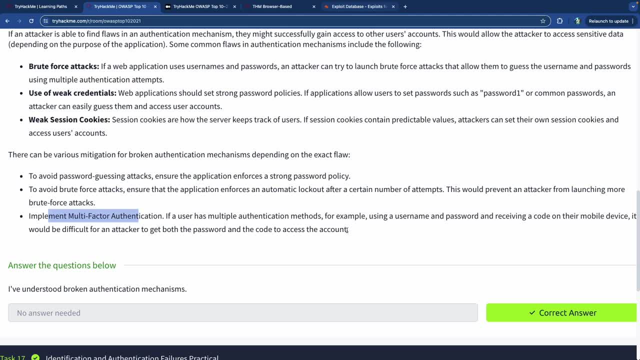 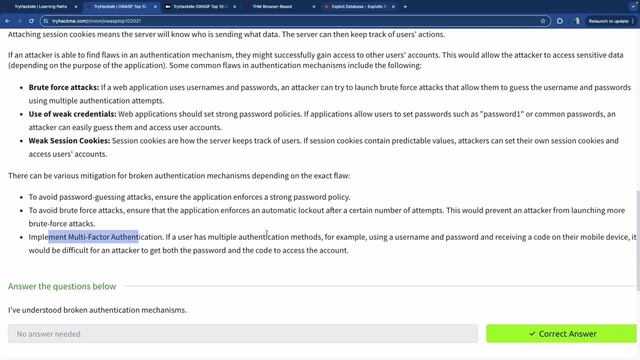 or we're going to send you a secret code to your phone number, or maybe use Google authenticator or some kind of a third party authentication like that to just make sure that these people are actually who they say they are when they try to log into the system. So authentication. 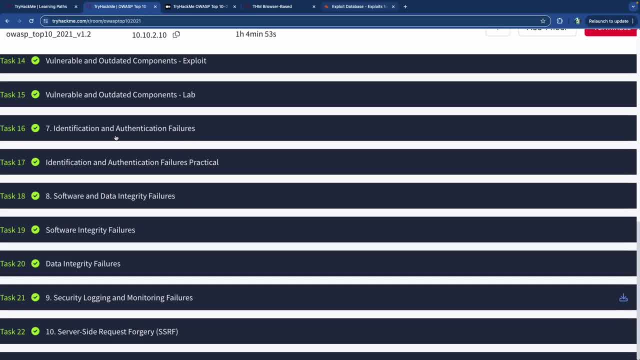 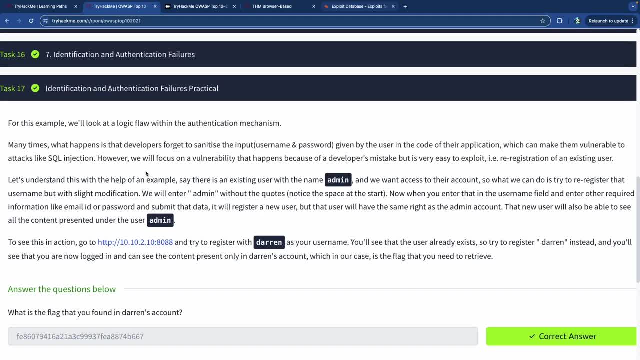 and identification are really important. The number is seven on the list, but it's still super important to be able to mitigate for this and prepare for this. So what we're going to do is we're going to run another exercise and we're going to now try to log in as admin and 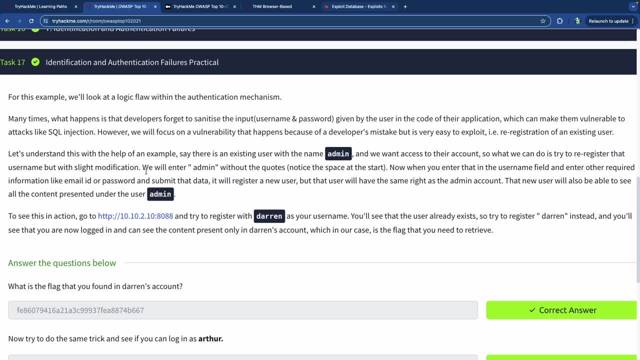 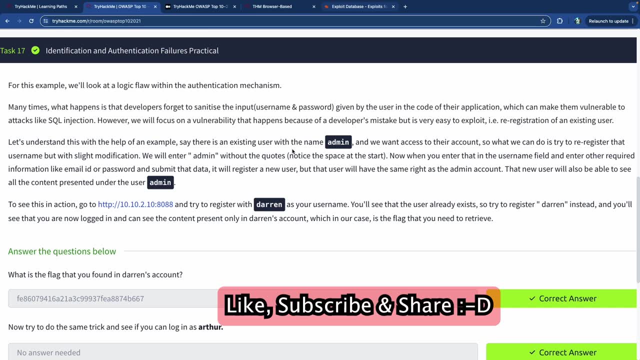 then Darren, to try to get some information from this website. All right, in this practical, we're going to be going to this web server and there's a very interesting concept here. so that you know, obviously there's most likely going to be a user named admin. 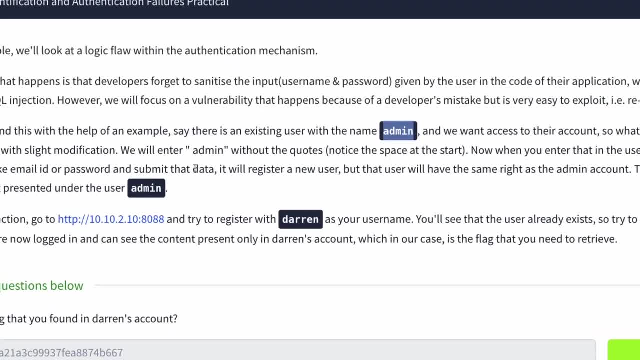 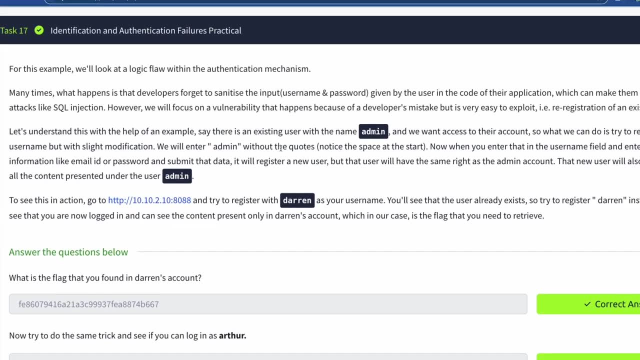 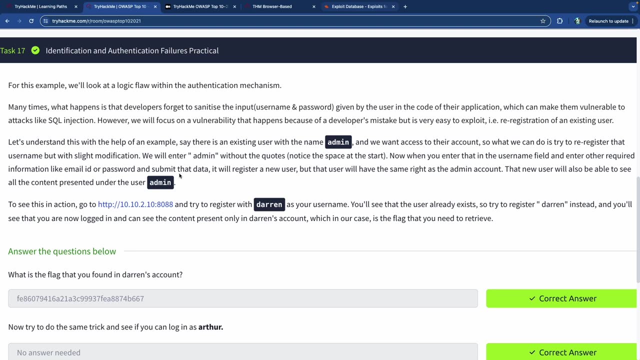 Um, but if it's not configured properly, if the website authentication is not configured properly, if you use admin with a space in the beginning, um, it'll still, uh, register you. But now, because you're registering as a new user, you can assign your own password and then it'll actually. 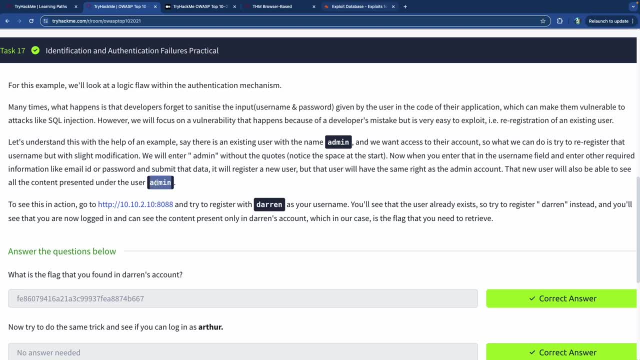 register you as an administrator and give you all the uh access rights of that user, that original admin user. So, to actually see this in action, we're going to do this for the user Darren. So we're going to go to this website. Here we go. 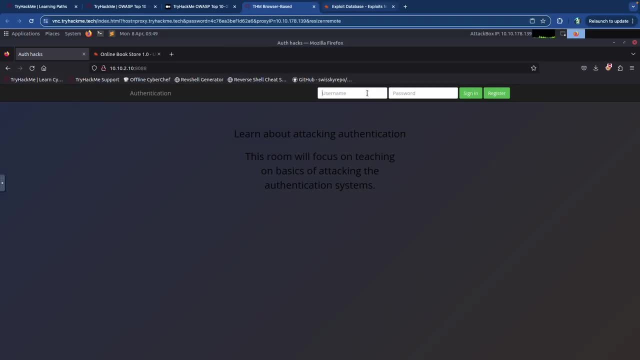 Learn about attacking authentication, yada, yada yada. So we're going to try to log in as Darren and then it's going to allow. it's going to say, no right, Cause you can't do it, Cause- uh, whatever, I'm going to type in password as his password. 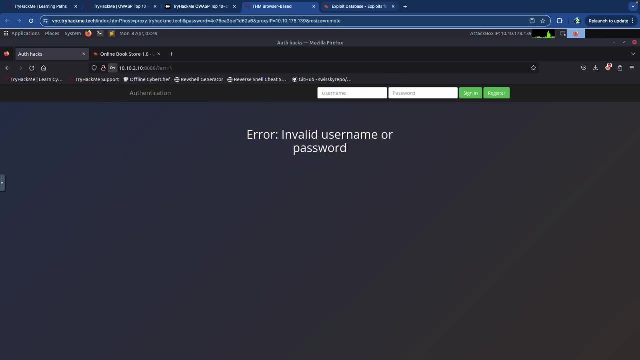 to see if that's his actual password. Watch it be his password. Okay, So invalid username and password. there you go. So that's not good. So I'm going to register now as a new user, but I'm going to do space, Darren, instead of doing, uh, any other thing. So I'm going to do space. 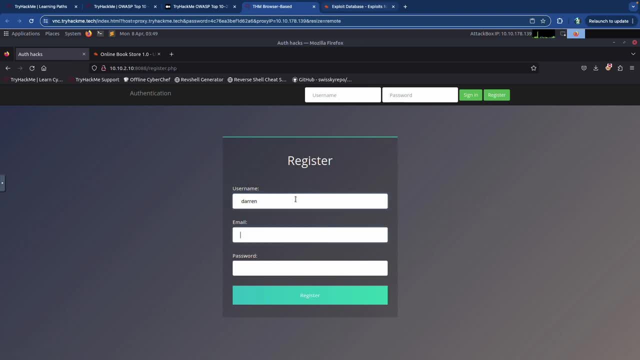 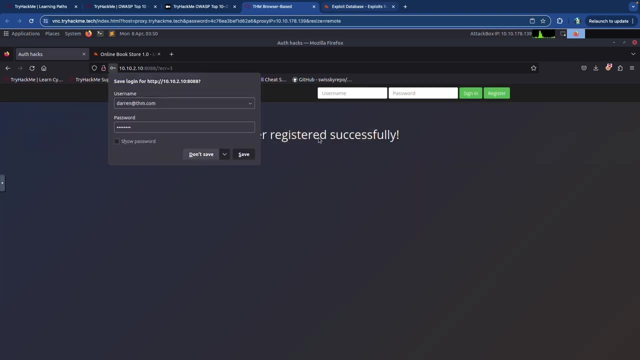 then darren, and then i'm going to use darren at thmcom as the email, and then we're going to do password as our password and we're going to register. and there we go, we have been registered successfully. so now we're going to do darren and do password, and that's going to be. 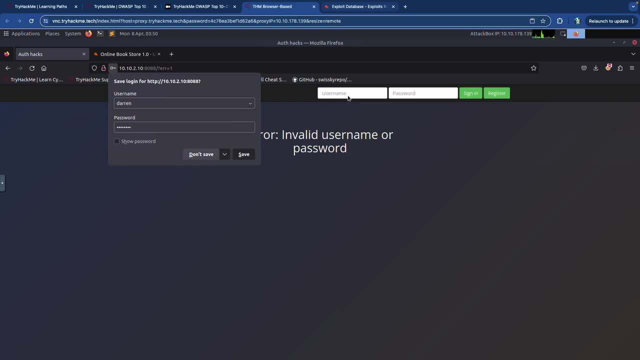 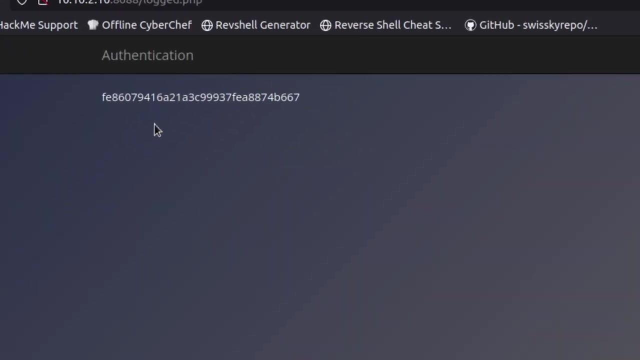 invalid. so what we're going to do again is we're going to do space darren- it sounds like astronaut name space darren, and then password, and log in. and look at that, we are logged in and there is the content that we need for our flag right here. so where's the flag that you found? 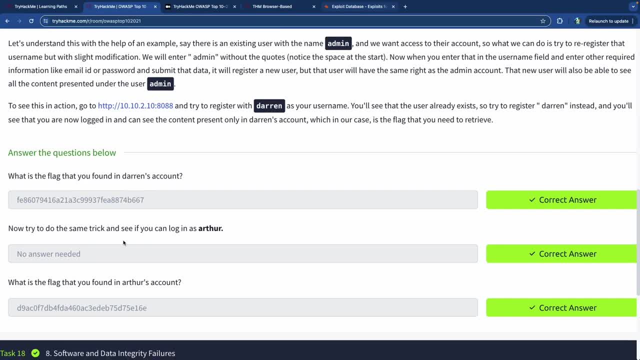 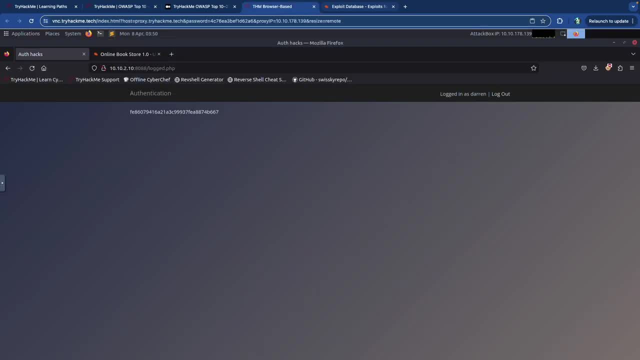 and that's the flag, and so let's try to do it with arthur and same process. so now it's going to be invalid. so what we're going to do again is: we're going to do space, darren, that we know that it's not going to. let us do it, so we're just going to go and log out. i'm just 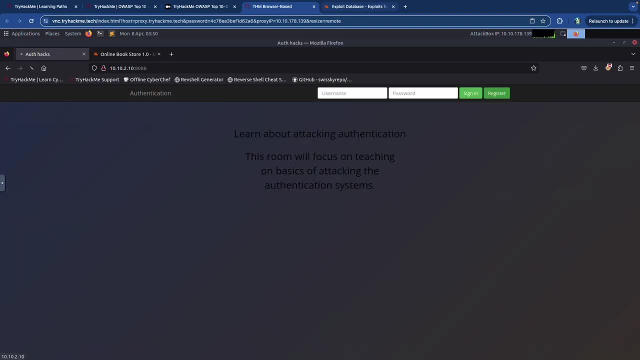 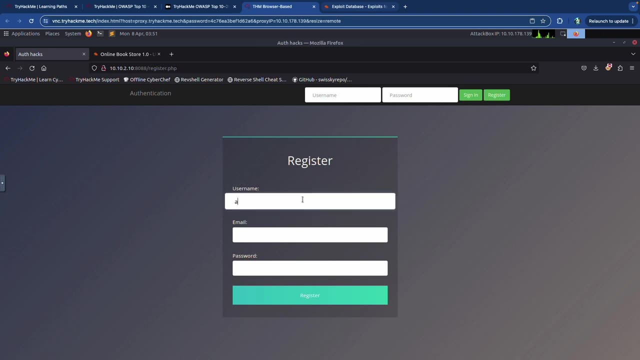 going to register as a new user instead of going back and forth and showing you all that. so i'm going to register here, and then it's going to be space arthur, and then arthur at thmcom, and then password as his password, and there we go. we have been successfully registered. 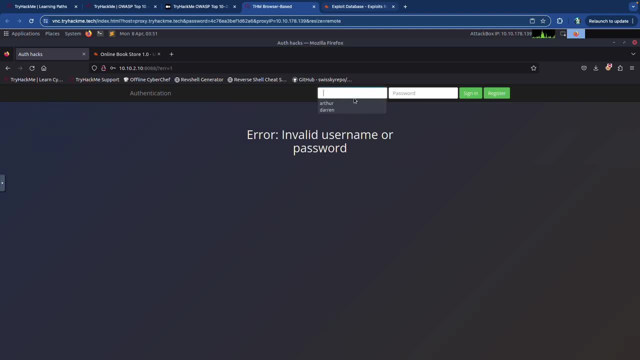 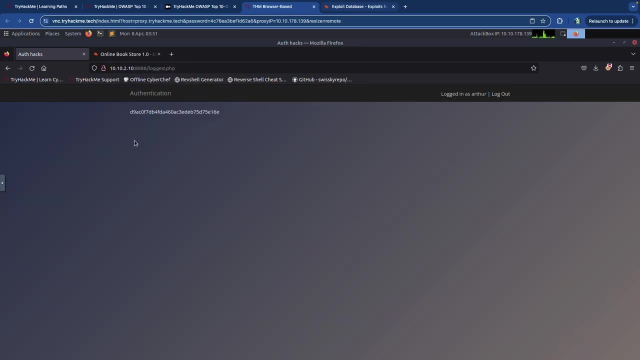 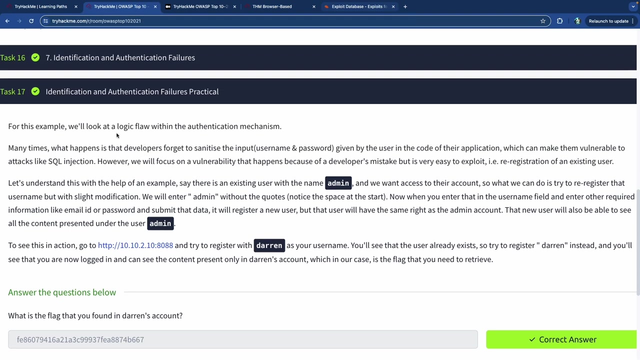 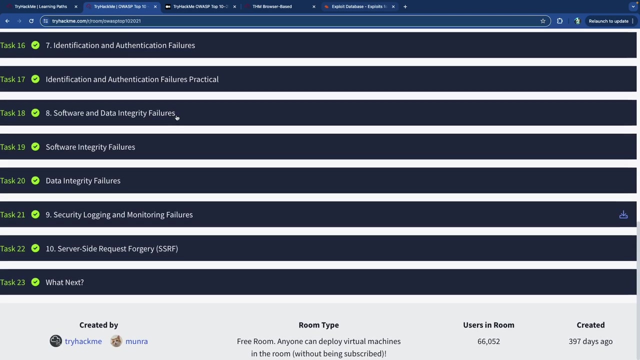 so we're now going to use space arthur and password and there it is so fairly simple to understand and this was just a weak authentication mechanism for that website. so it's kind of crazy, it's it? it seems overly simplistic, but it's very, very crazy how that. 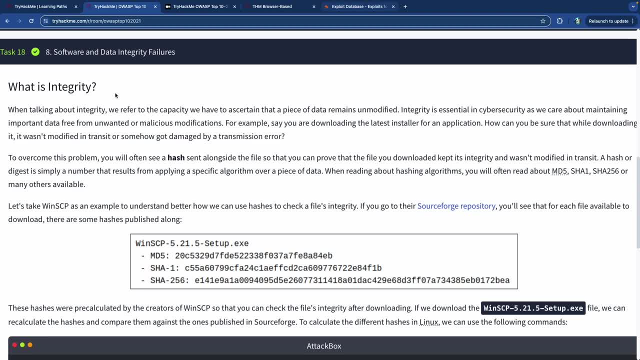 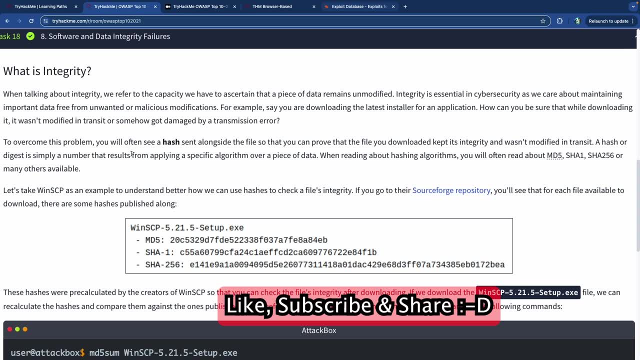 works. so software and password are two different things. so we're going to do space arthur and data integrity failures. so let's check this out. when we refer to integrity in cyber security and data information security, we're making sure that the- whatever the software is or the data is, it's 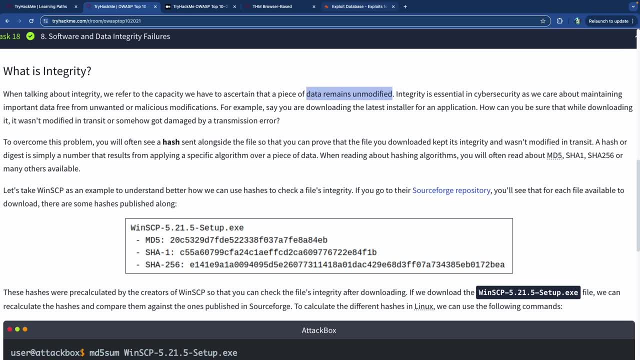 been unmodified, so it hasn't been altered or changed in any way. and the way that we do that is we check the hash value of it. so if you wanted to go to, let's go to cali. so if we go to caliorg for 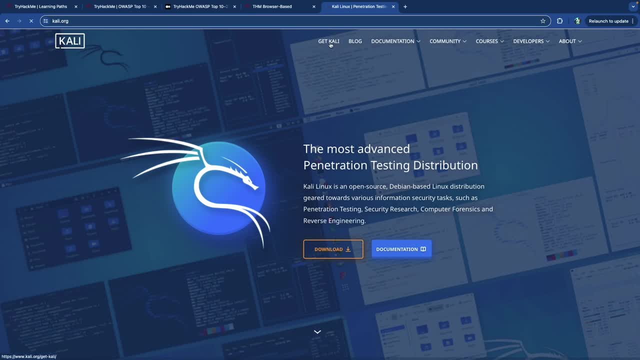 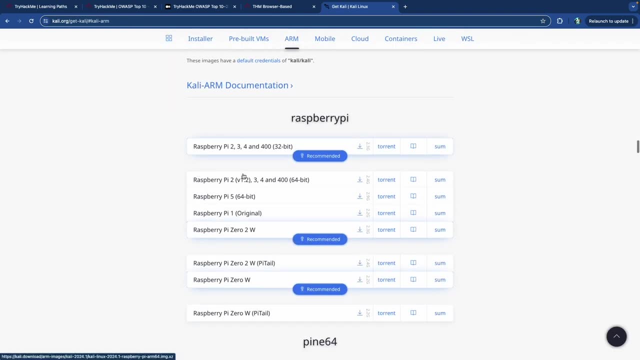 cali linux and then you want to download any of these uh, cali linux versions. so if you go and click on any of these, so i'm going to click on arm and then i go here and i check one of these things and i didn't mean to download it. so let's stop that and let's go here. what i want to do is right. 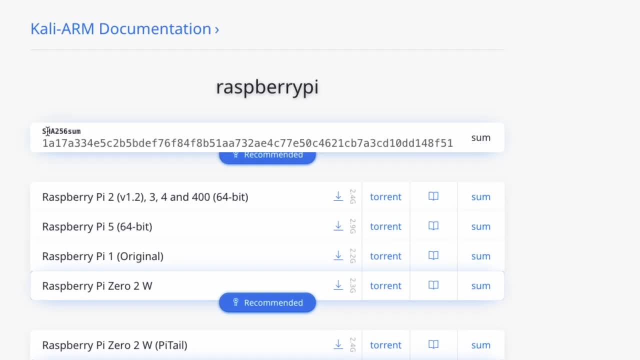 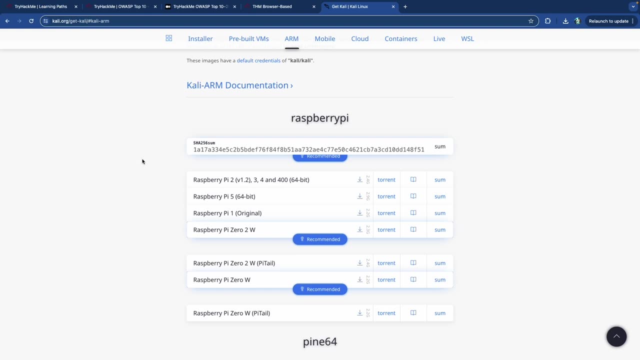 here, so i'm going to click on some. when i click on some, it gives me the sha256 sum. this is the. and if you download this from any other place and you, you know, they say, yeah, this is a cali arm version that you want to download, and you run the sha256 sum to get the hash value of the file. that 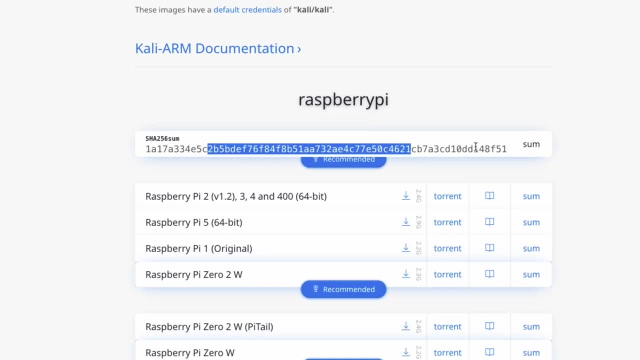 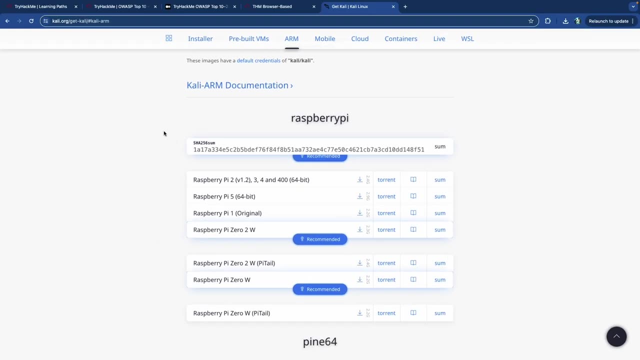 you downloaded. if it's anything other than this hash value, you can be sure that that file has been altered in some way, and this is how you verify the integrity of something that you're downloading. they use this a lot, this concept of the file and data integrity failure. so if you download this from any other place and you 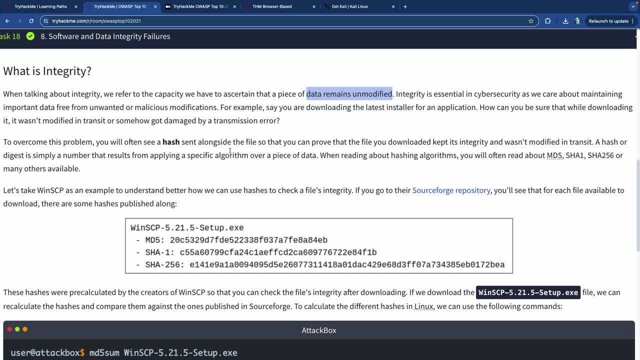 want to get the hash value of the file that you downloaded. this is how you verify the integrity. this is used a lot in forensics. in digital forensics there's something called the chain of custody, and in the chain of custody you start out with getting the copy of the evidence from. 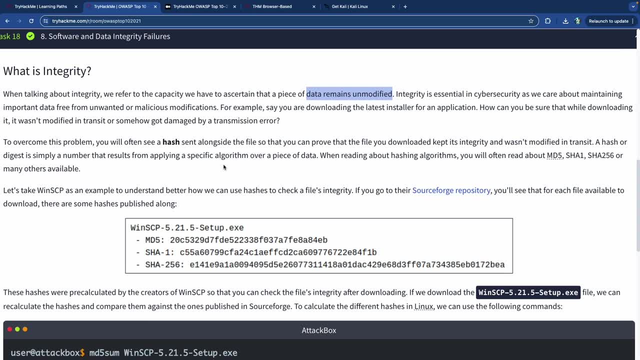 the crime scene and immediately the forensic investigator, the digital forensic investigator, creates a hash value of that disk image that they got and they put that hash value in the- uh, the forms that go along with chain of custody and along that the management of that piece of evidence. if that hash value has changed even by one letter, and i mean 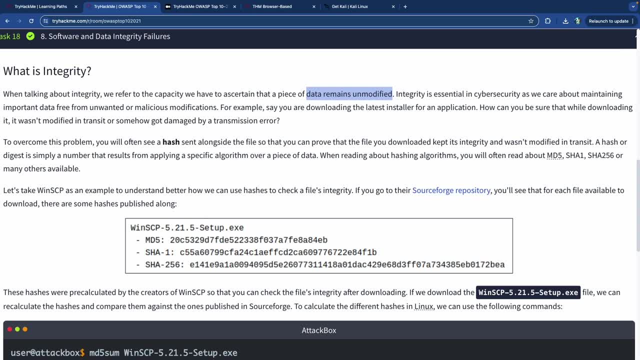 if anything changes, the entire hash value changes, as you saw when we went through the password example at the beginning. so if that hash value has changed from the beginning hash value that means that file has been altered, that is, disk image has been altered. so that's what we 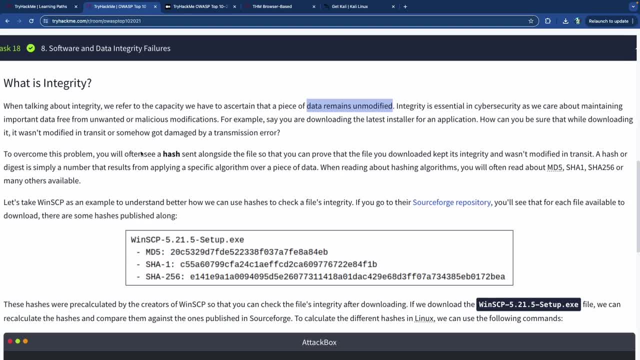 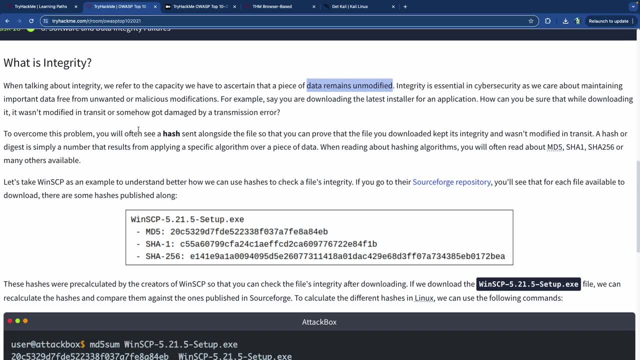 use to verify the integrity of data, and so software and data integrity failures typically are some of the ways in which that hash value can be changed, and so let's look at an example here. with this specific example- i'm going to go to this specific example- that something has been. 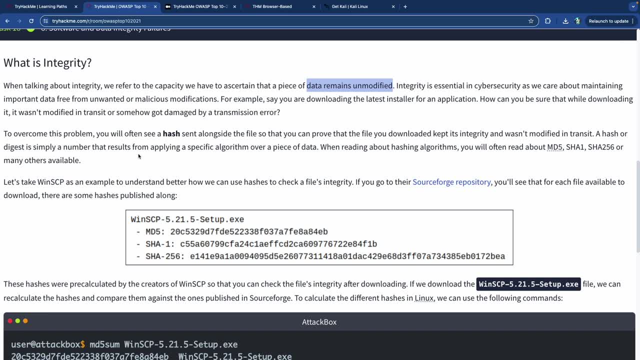 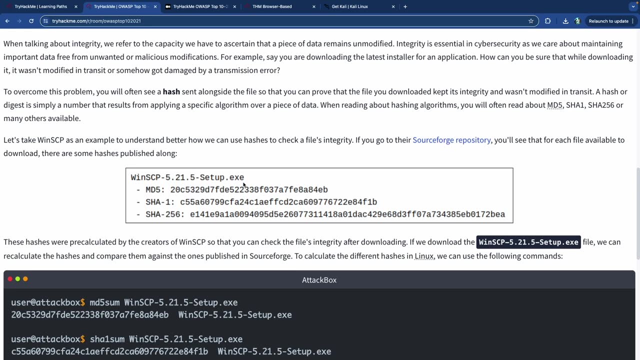 changed inside of the source code of that software or something has been changed by the, the, the macros of the file that you're downloading, or anything along those lines. if it's been altered in any way, then you know that the hash value has been changed and check, and so this was. uh, this is on the source forge repository and you look at it like this: 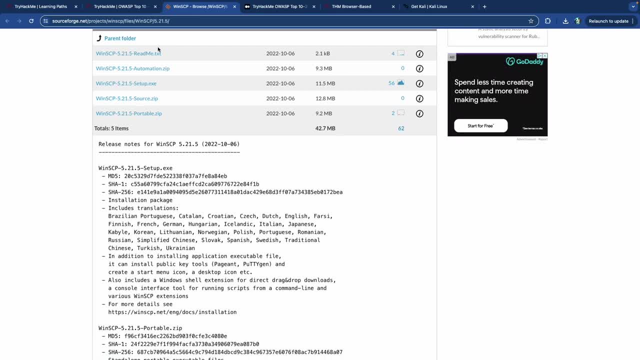 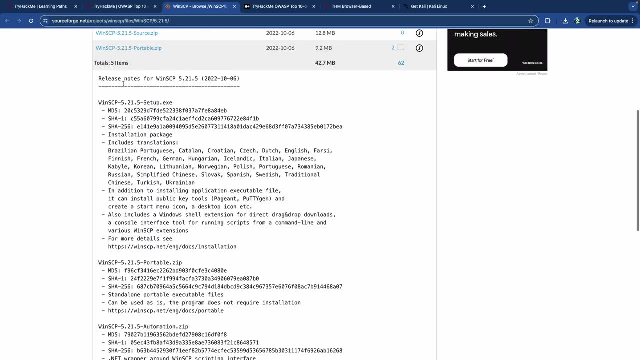 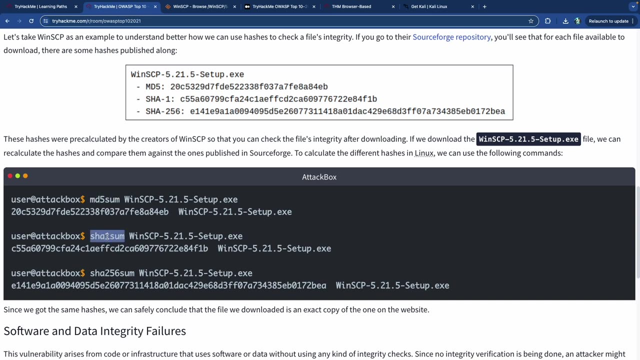 and this is just another version of what we just checked out on kelly linux- that it gives you the hash values right here. so there's the md5 hash value, sha1 and sha256 hash values of this and then from there you get to run: uh, the md5 sum, sha1 sum, sha256, sum against the file that you've. 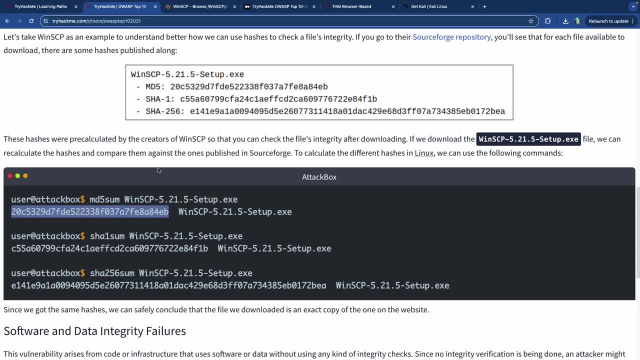 downloaded and it should be the exact same thing that's available on their website. if it's not, that means that you downloaded an altered file and there's something wrong with that file, and you should not open that file, you shouldn't run it, you shouldn't do anything with it, and this is. 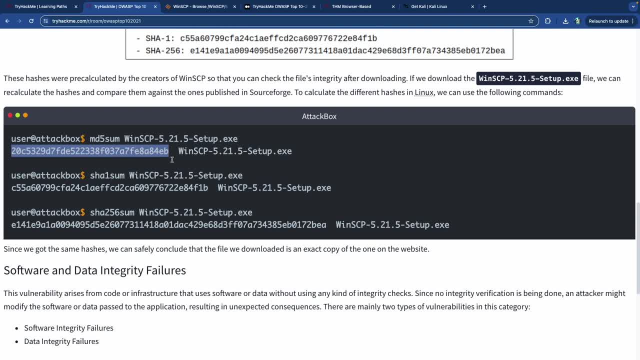 very important to understand that anything that you download if you're not downloading it directly from the website- so if you're not downloading from the microsoft app store, for example, and you're downloading from something separately- you can verify the hash value of the file that you downloaded to make sure. 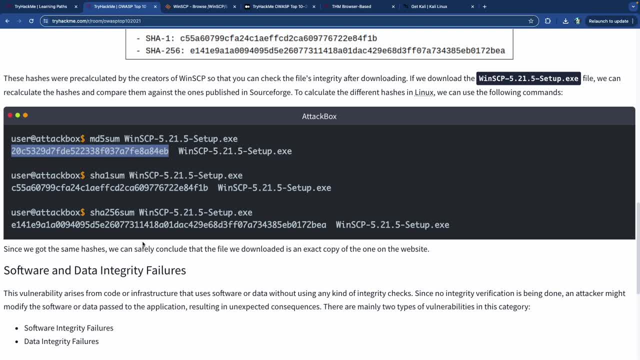 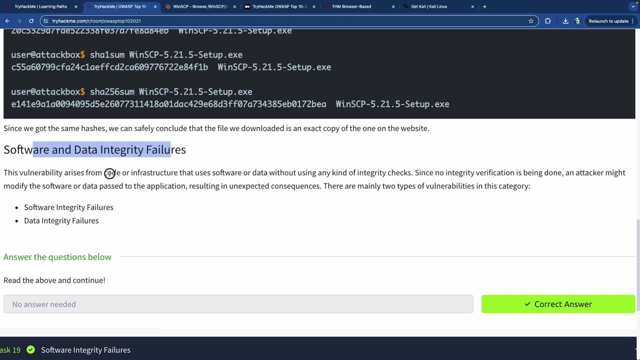 that you actually have the right file. otherwise it's been altered and you should not use it. so software and data integrity failures? uh, they arise from code or infrastructure that uses software data without using any kind of integrity check, and since there's no integrity verification being done, an attacker might modify the software and data pass to the application, resulting in 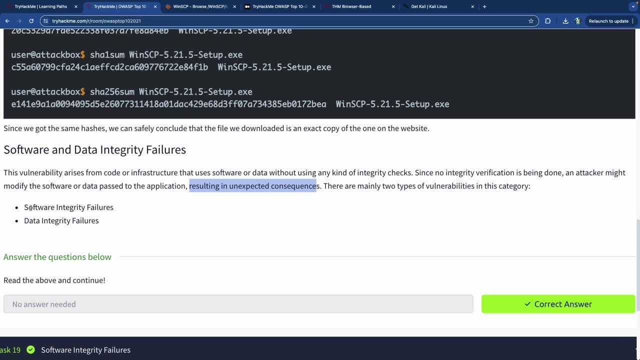 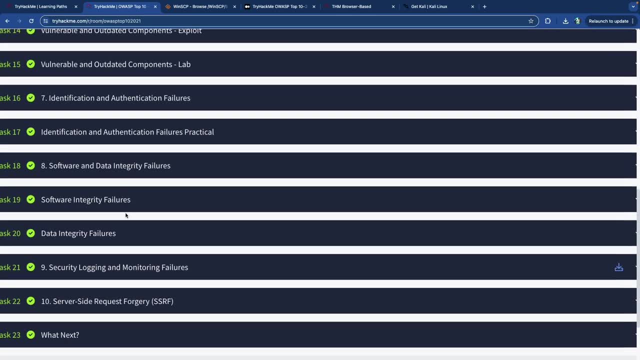 unexpected consequences, and two vulnerabilities are software integrity failures and data integrity failures that are relevant to this. so we are now going to go ahead and run this and we're going to go ahead and run this and we're going to go to look at that in a real life example. so, software integrity failures: suppose you have a website that 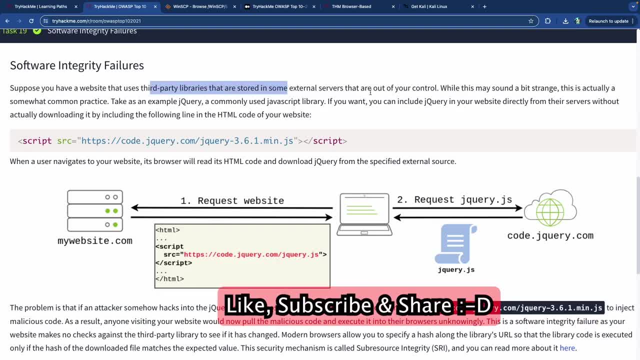 uses third-party libraries that are stored in some external server and they're out of your control. this is actually a common practice, and so we can, example, use jquery, which is a javascript library. if you want to use jquery in your website, you use it without actually downloading it. you use 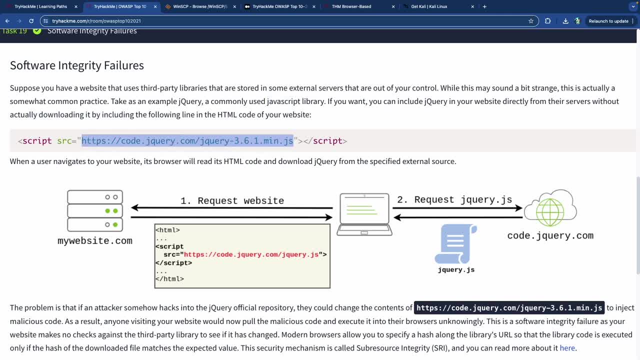 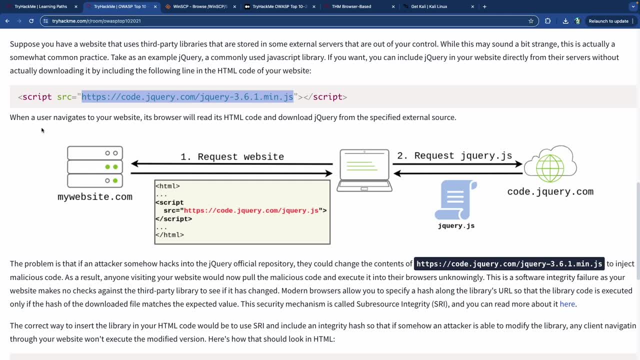 the following command and you use their link for the script right. so you use the link from their actual jquery website to be able to use this right without actually having to download it. when a user navigates to the website, it'll the browser is going to read the html code. 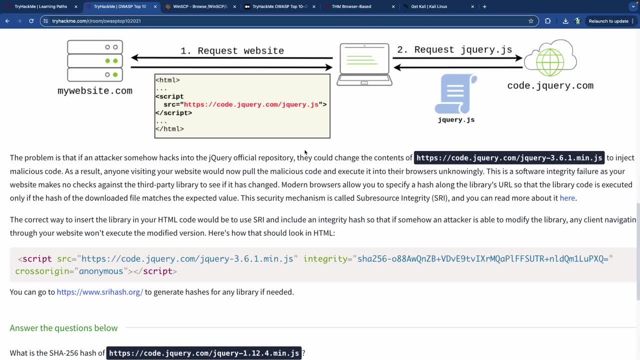 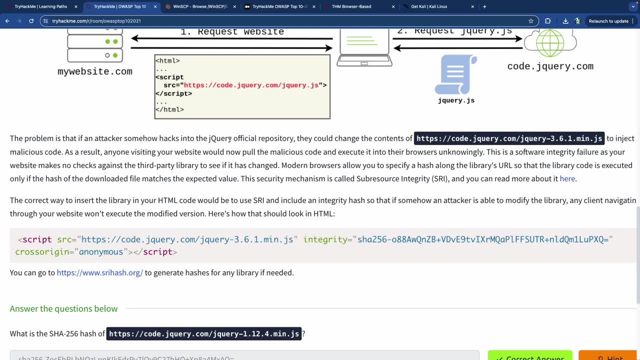 and download jquery and then process everything that you want in your code as if you had downloaded jquery directly to your website. now the problem is this: if an attacker somehow hacks jquery and they change the contents of this endpoint and inject any kind of malicious code, then that puts you at risk as well. 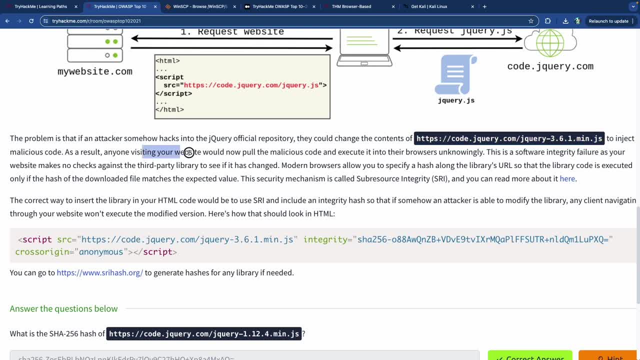 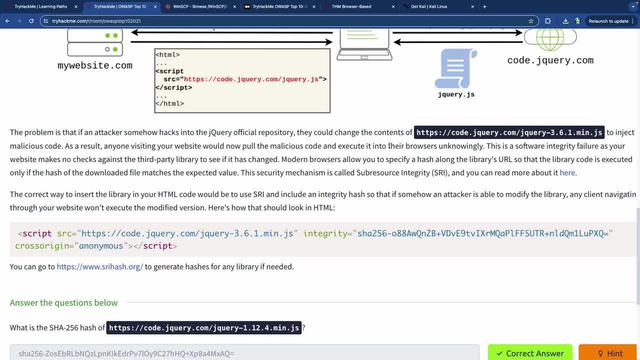 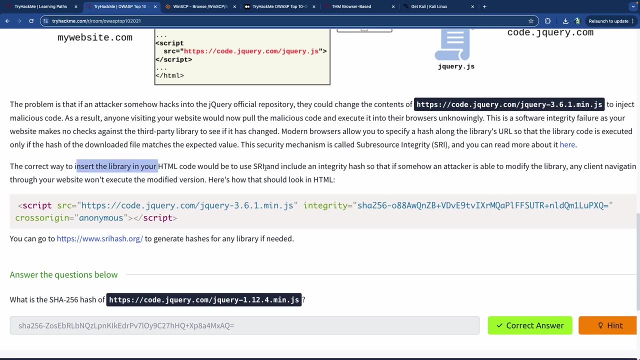 then that puts you at risk as well. so anyone visiting your website could now pull the malicious code executed and without them knowing something's going on on their website. this is an integrity failure on software, and the correct way to insert the library in html code would be to use the sri and include. 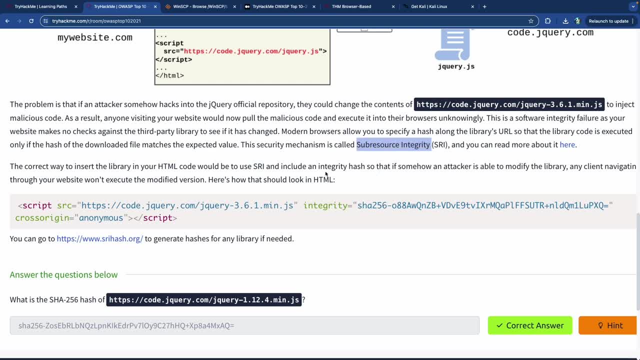 which is the sub resource, integrity, and you can include the integrity's hash value so that somehow the attacker is able to modify the library and store these. but if you don't have it, then this should do that. it's pretty easy and it's very easy to do if you're a developer yourself and you want to run a free. 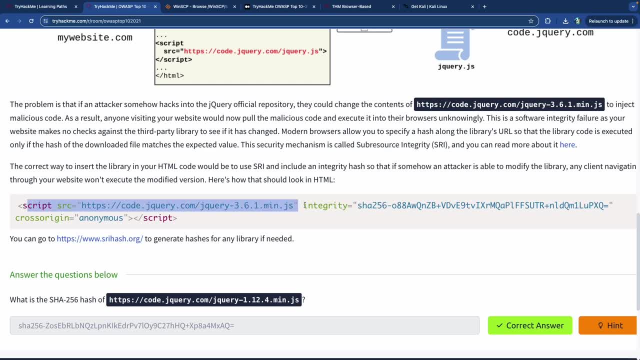 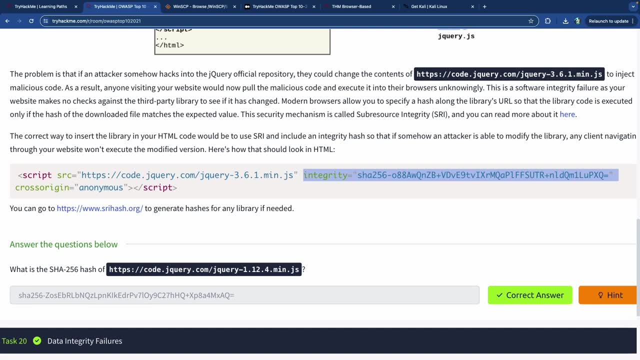 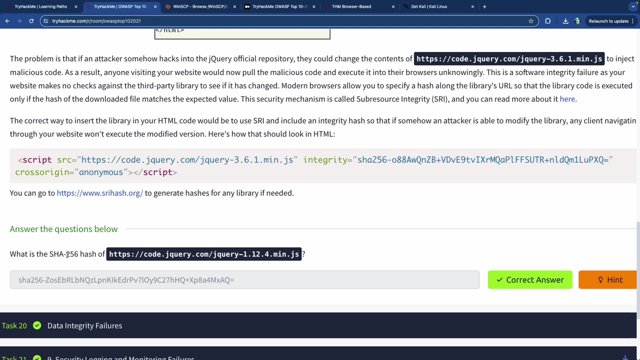 Hershey's library. if you're using any web or any other users site, that as well if you need it. So what we're trying to do in this particular case is get the hash value of this thing- HTTPS code such and such and such- So we can just go and copy. 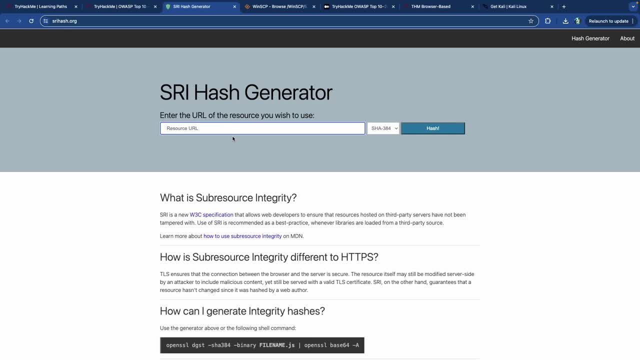 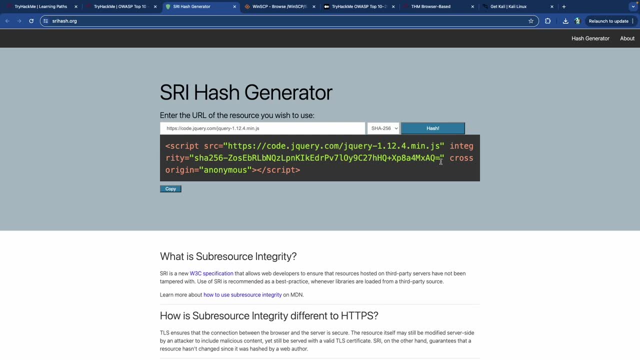 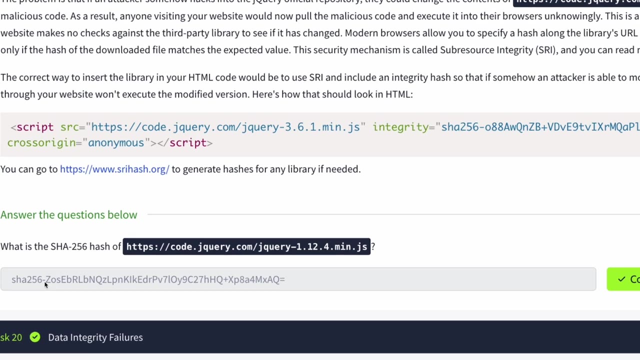 this and go here and then run that URL here and we want the SHA-256.. So we generate that hash and here it is. This is the SHA-256 hash value of this. So if I copy this and come here, this is exactly it. So they actually have the SHA-256 portion at the beginning. 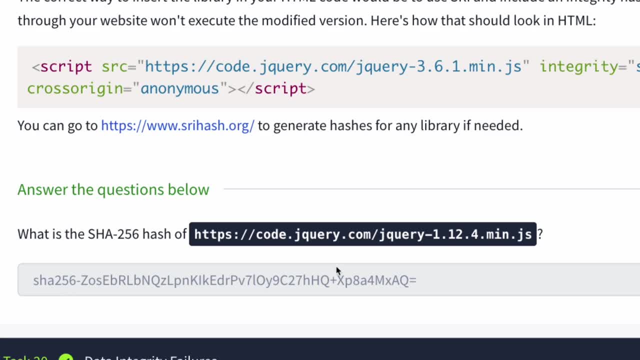 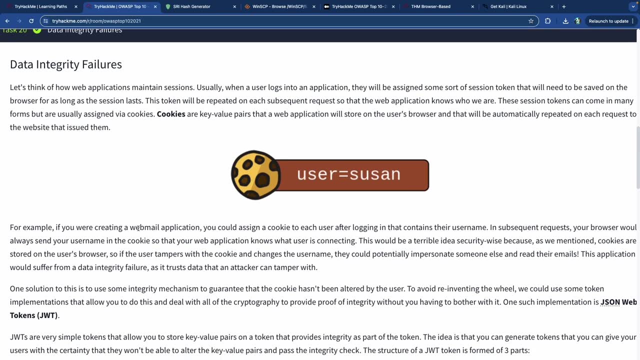 as well. So SHA-256 dash and then the rest of that and that is the full hash value that we got here. So that's software integrity. So let's look at data integrity in this case. All right, usually when a user logs into an application, they're going to be assigned. 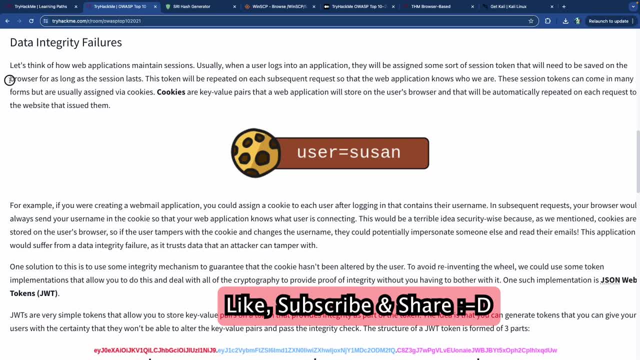 some kind of session token- We kind of talked about this already- and it's saved on the browser for as long as the session lasts, especially if you save your username and password. Then it's going to be assigned to the browser. So if you save your username and password, 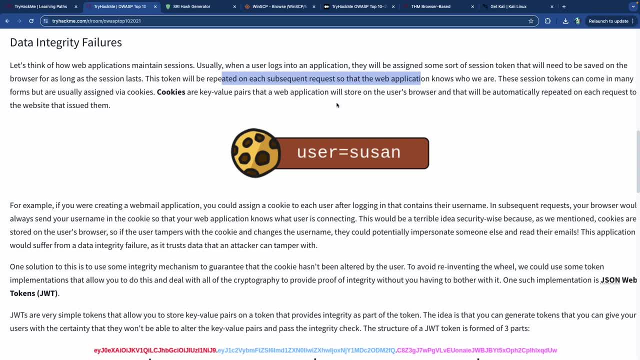 then it's going to be assigned to the browser. So if you save your username and password, then it's going to be repeated every single time that you access that application. And then they come in a lot of different forms, specifically as cookies. They're through. 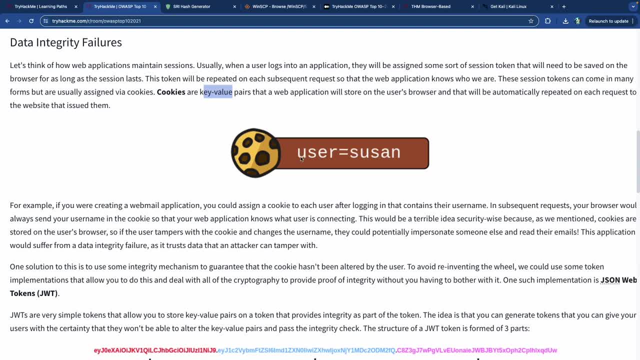 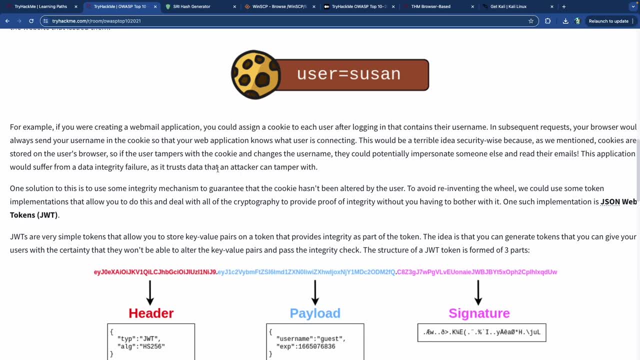 cookies And cookies are key value pairs. So the user Susan, the user is the key and the value is Susan in this example. And then there would be password equals yada yada yada. And so if you were creating a webmail application, you can assign a cookie to each. 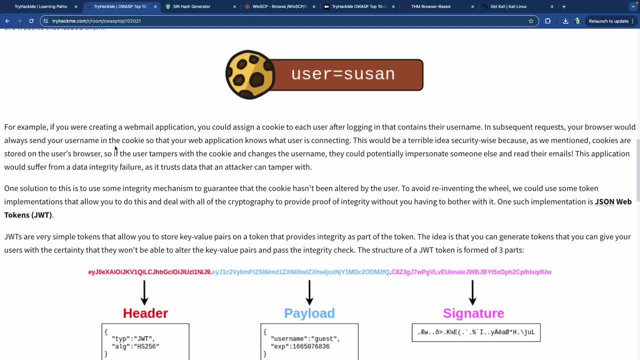 user after logging in And a subsequent requested browser would always send the user a cookie username and the cookie so that web application knows what's going on. And this would be a terrible idea security wise, because cookies are stored on the browser And if the user tampers with the 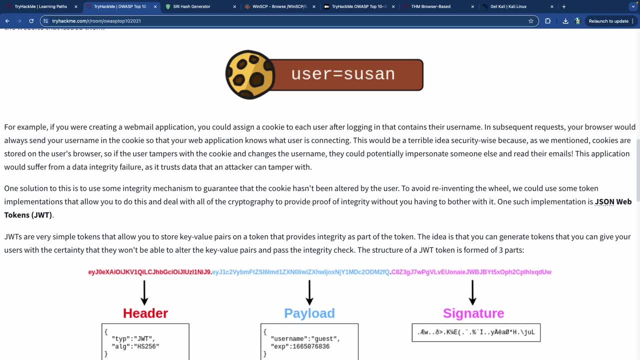 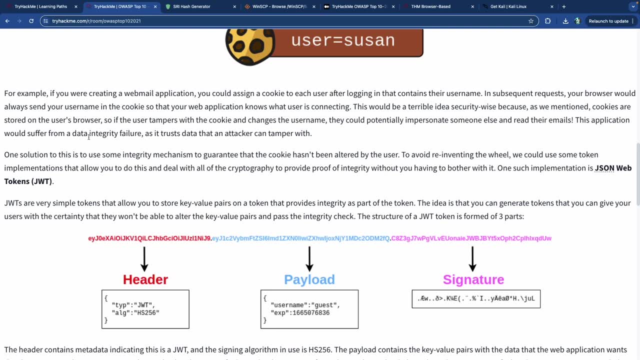 cookie and changes the username, or if a hacker tampers with the cookie and changes with the username, they could potentially impersonate someone else and read those emails. The application would suffer from a data integrity failure And if somebody wanted to hack into anybody's system, 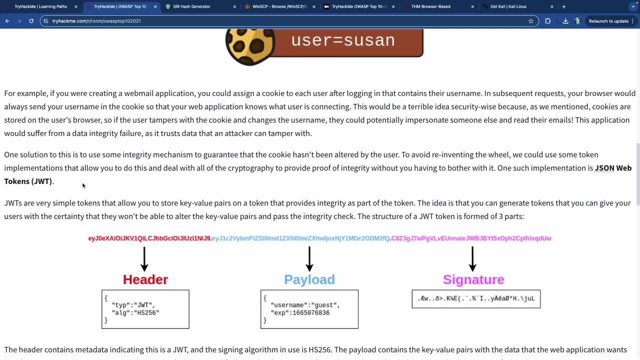 they could just sniff your traffic, And this is why they say: don't check your bank account or don't check your email when you're connected to a public Wi Fi at a coffee shop, something like that. And a lot of people do this, by the way, because if you do, do that, if you use the public, 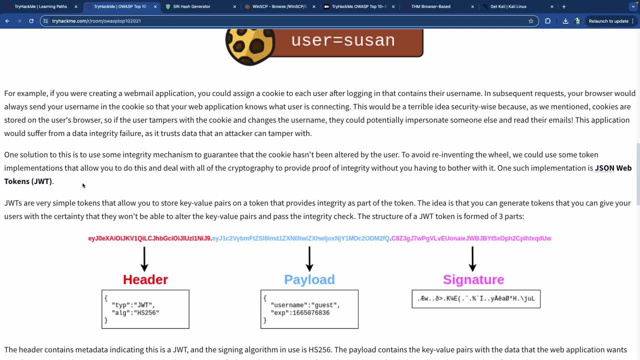 Wi Fi at a location like that. somebody could be sitting in that cafe And they're scanning the, they're sniffing the traffic using Wireshark or TCP dump And then they can capture that value from your cookies and then use that information to impersonate you and go into your 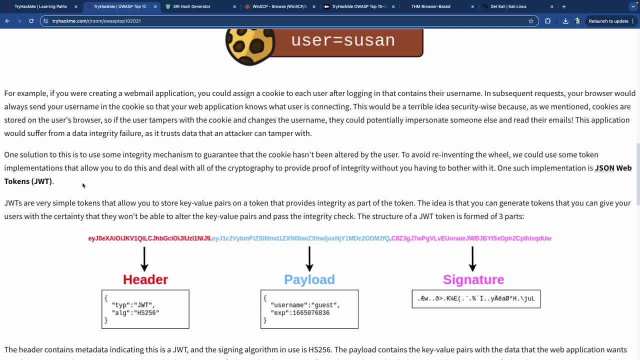 information. I've talked about this with a lot of my friends. one of my friends actually recently or, you know, a couple of months ago maybe- he got hacked and they got into his bank account and took money. It was crazy. There was like a really really crazy situation And he called me. 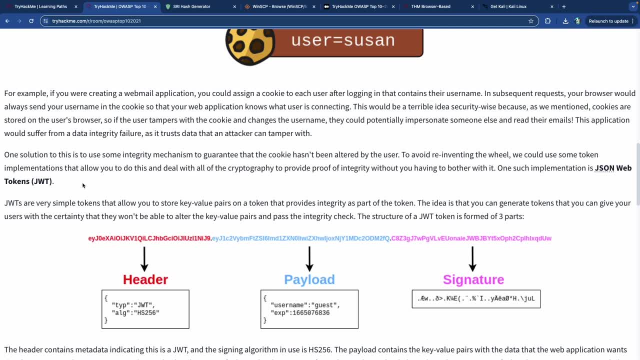 immediately. He's like Yo, what do I do? And I was like you need to immediately change your password, because I knew that he uses a bad password And he uses it on all of his stuff, on it on his email accounts, on his computer login. And I just knew I'm like bro, you can't. 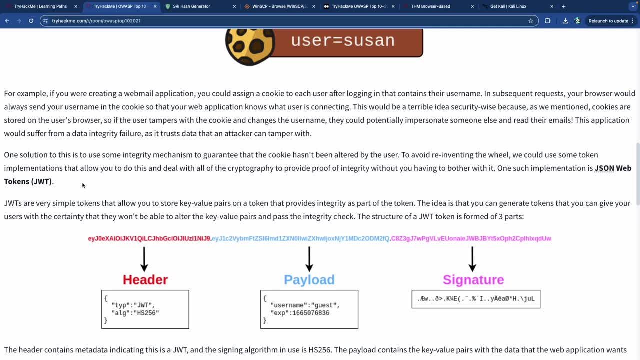 be using this And I told him multiple times prior to that And he still didn't listen to me until he finally got hacked. And that was the case where it's like, okay, well, you got to use strong passwords, man. This is like a, it's not. it's not even a question at this point. If you use a weak, 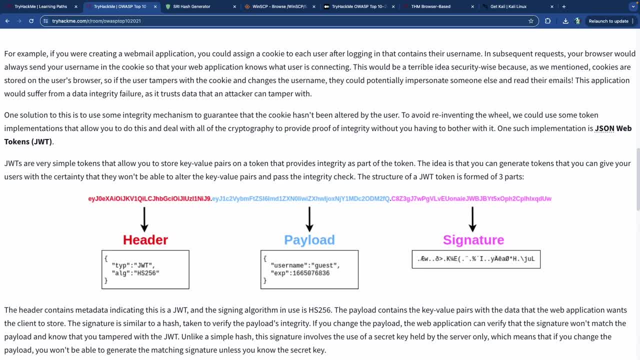 password. you're just asking for it. So a solution to this is an integrity mechanism to guarantee that the cookie hasn't been altered, And we could use some token implementations and cryptography to provide proof of integrity without you having to bother with it. 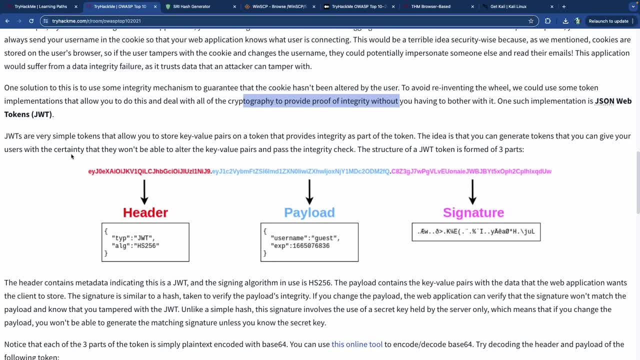 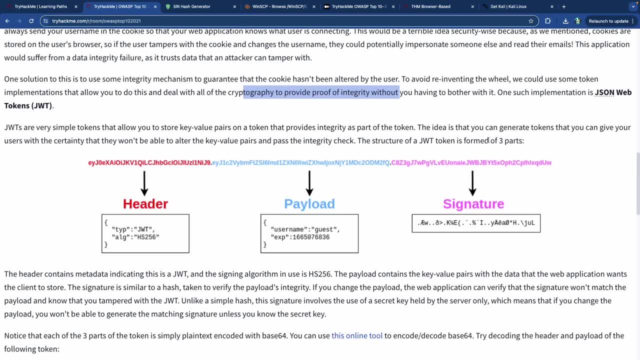 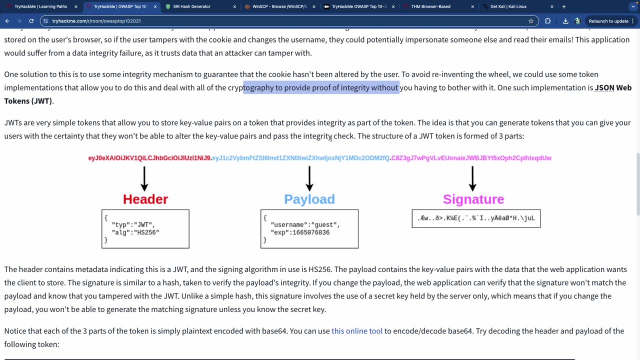 Something like that is called JSON web tokens. JWTs are simply tokens that allow you to store key value pairs and provide integrity as a part of that, And the idea is that you generate tokens that you give users with certainty that they won't be able to alter the value pairs and pass. 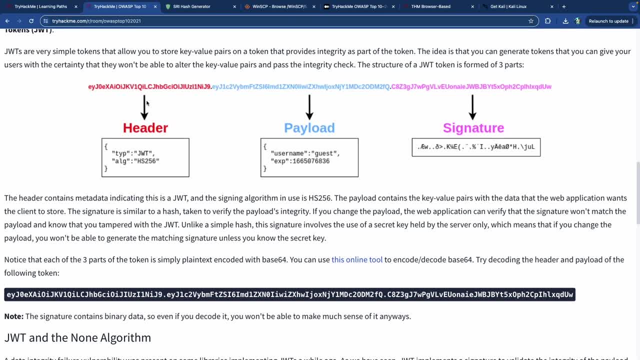 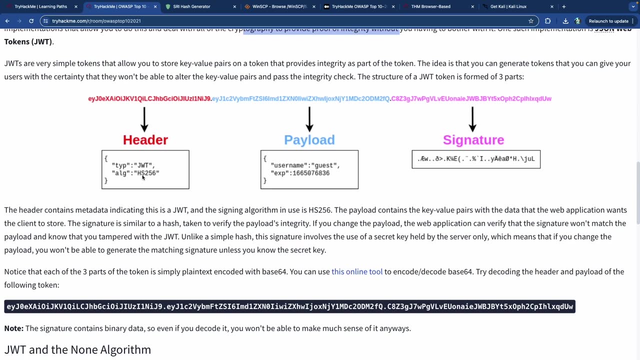 that integrity check And it comes in three parts. So you have the header, you have the payload itself and then the signature And the header is the JWT. So the type is J JWT, which is the JSON. JSON web token algorithm is going to be HS 256.. In this case, the payload, 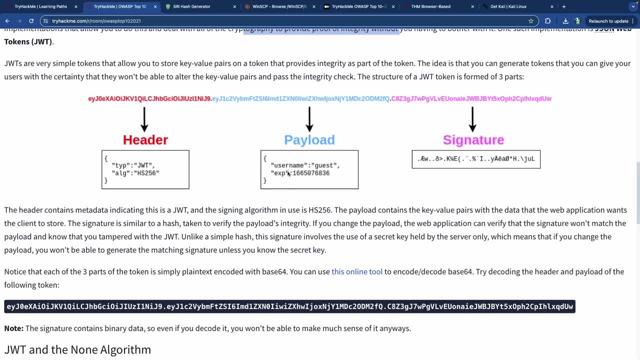 itself is the username and the password And, excuse me, I think the exp is the expiration, maybe for this- And then you have a signature that's been attached to this and it comes in three pairs, And so that's how you verify the integrity of it. The header contains metadata. 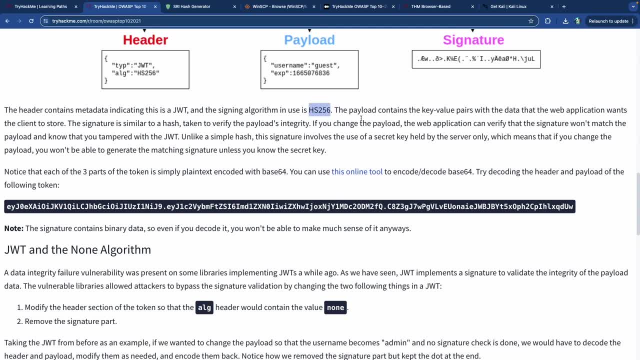 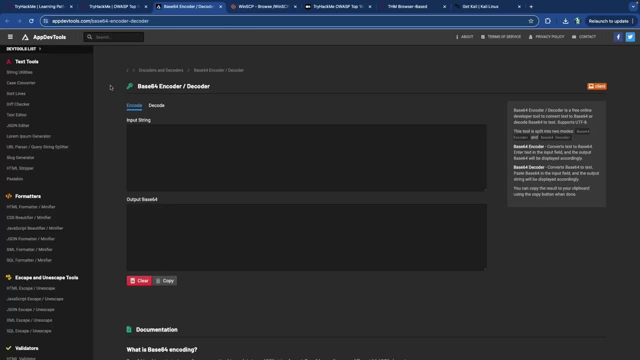 indicating it's a JWT, And HS 256 is the algorithm. the payload contains the data and then the signature is similar to a hash value to verify the integrity of that payload, And we can use this online tool that they gave us to go ahead and encode or decode Base64 and 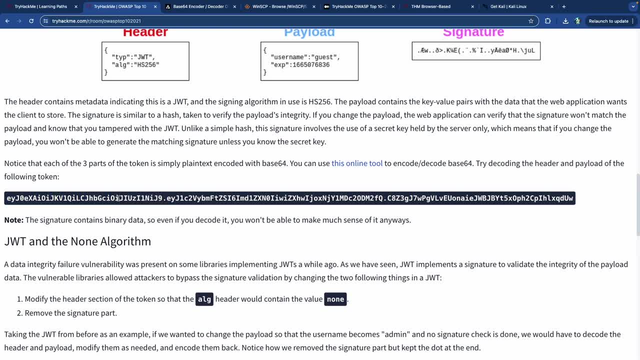 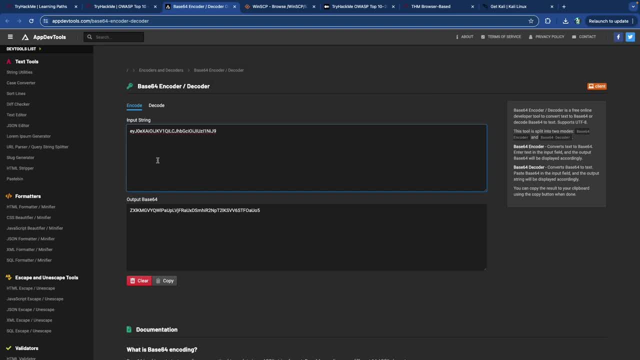 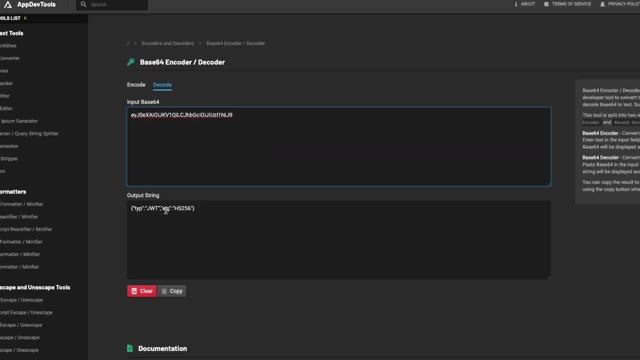 try encoding the header of the following token. So we're going to encode the header of this token, which is this piece, And so I go here and do this And the encoding would be this: So if I decoded it, it gives me that. So it's JWT algorithm HS 256.. So yeah, it's a decode, not encode. 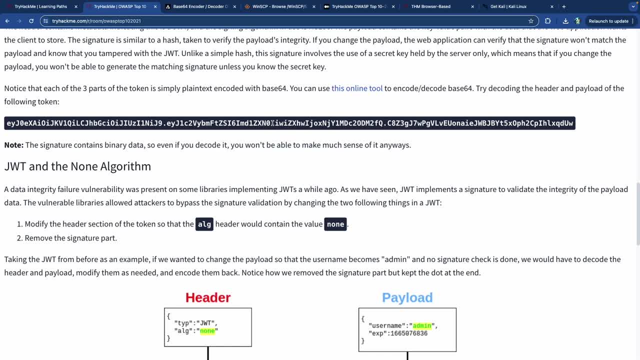 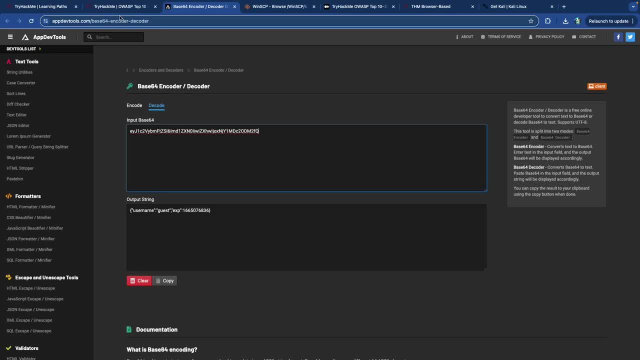 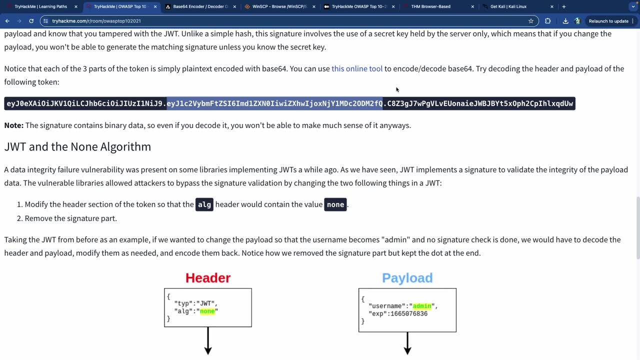 The signature contains binary data. So even if you decode it, you won't be able to make much sense of it. If we use the payload to decode, then you'll get username, guest, expiration, same thing. So there it is. So this is decoding the. That's so crazy. Decoding the Base64.. 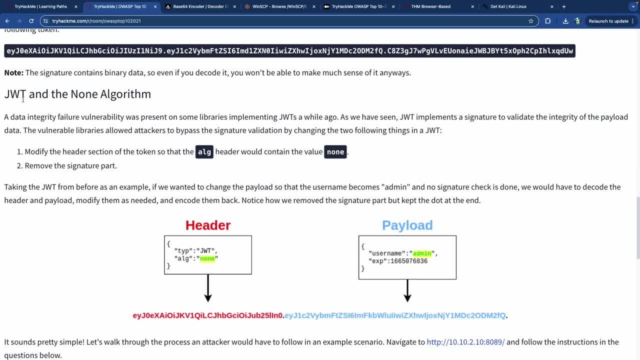 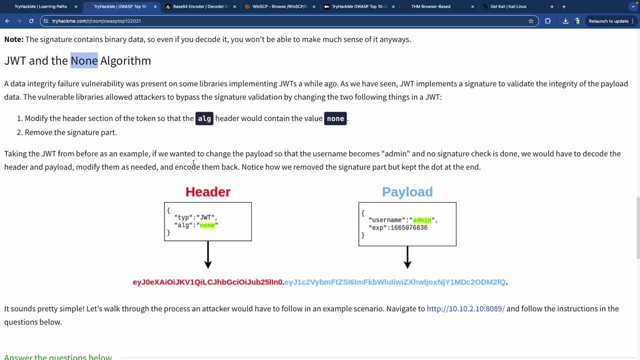 Information, So JWT and the non algorithm. So you just have a header and then you have a payload and there is no signature that's been attached to it And it's very similar to the other piece, It's just that there is no actual signature attached to this. So if we wanted to, 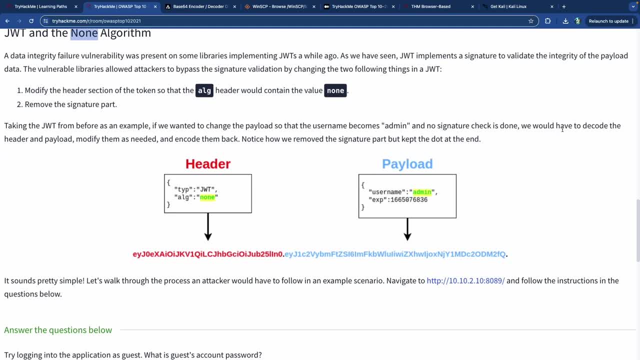 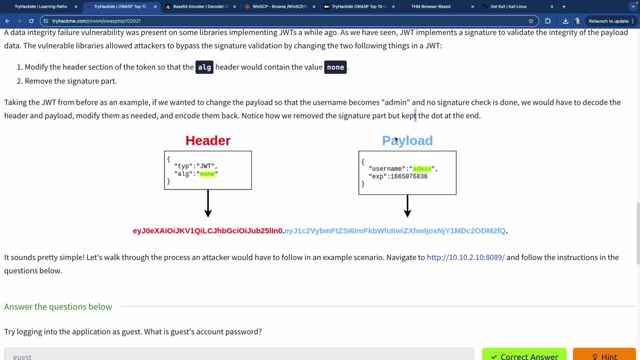 change the payload so that the username becomes admin and no signature check is done. we would have to decode the header and the payload, modify them and then encode them back, And then you remove the signature part but kept the dot at the end, this little piece at the very end of it. 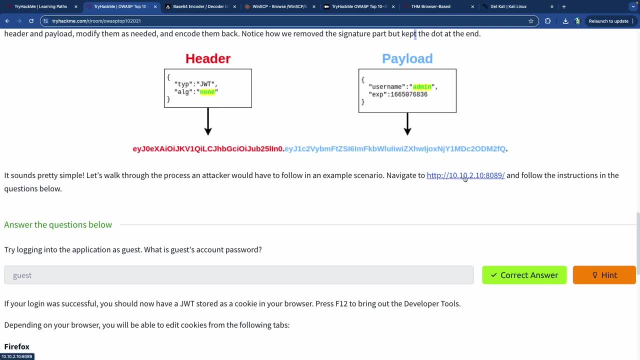 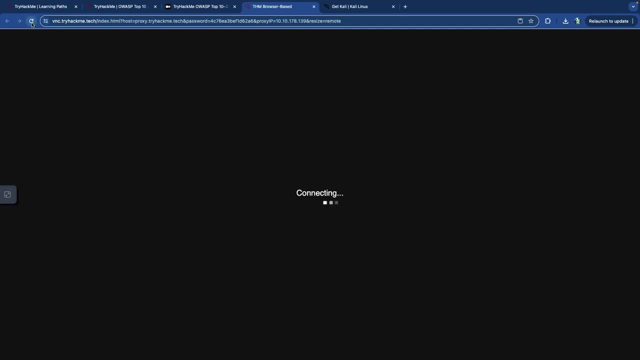 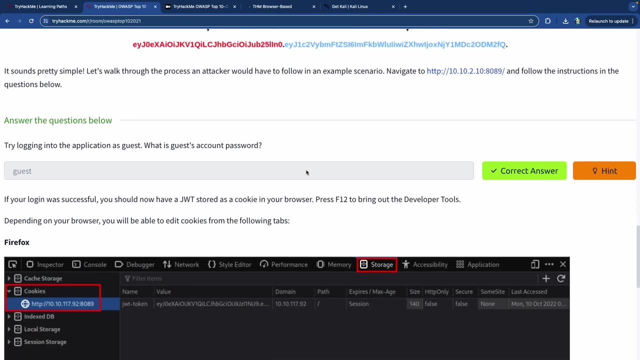 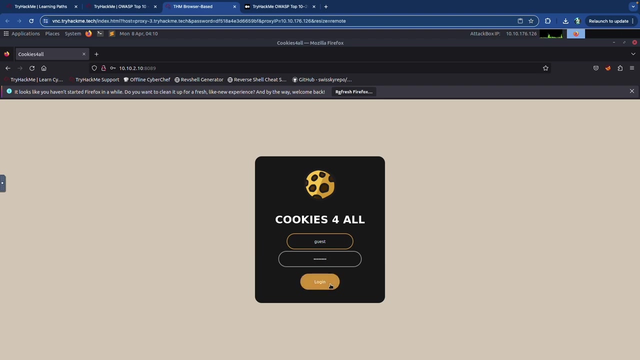 So it sounds simple. So let's go and actually do this on our web application here. So we're going to go to our portal right here and we're going to use the 8089 port and get some cool information here. All right, So here's our web portal here. So we're going to try to get. 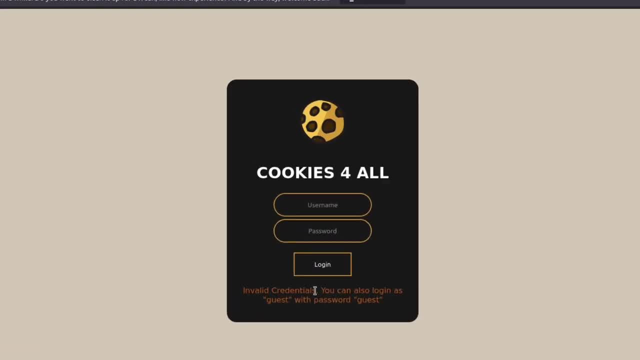 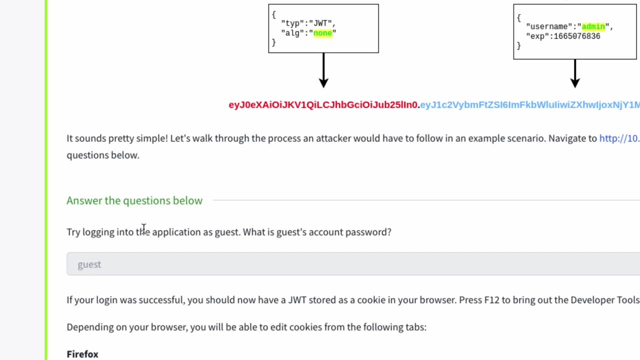 logged in as guest And so it says invalid credentials. You can also log in as guest with the password guest. So it already gave us the password for a guest. So application as guest. what's the account password? yada, yada, yada. So guest, guest. So now what we're going to do is: 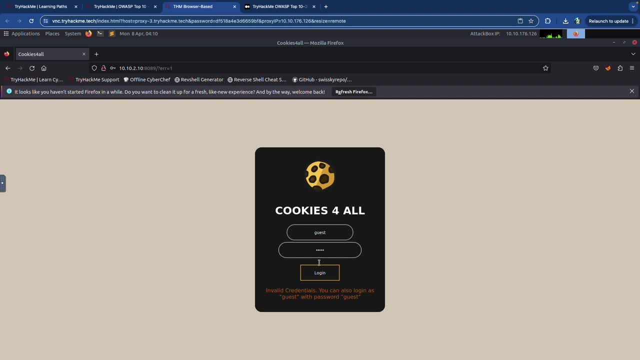 we're actually going to log in as guest, guest and save that And then so we're going to save ourselves. Hello, guest. Only the admin user is allowed to get the flag. So now what we want to do is we want to follow the rest of these. 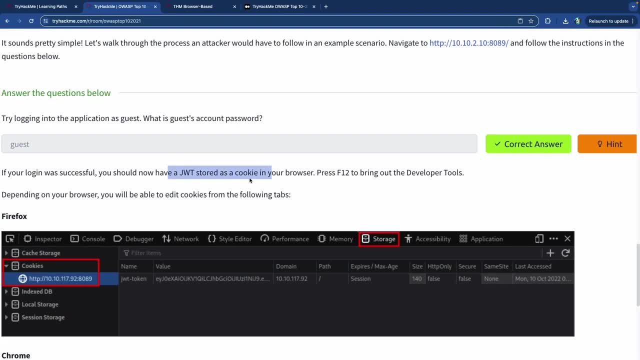 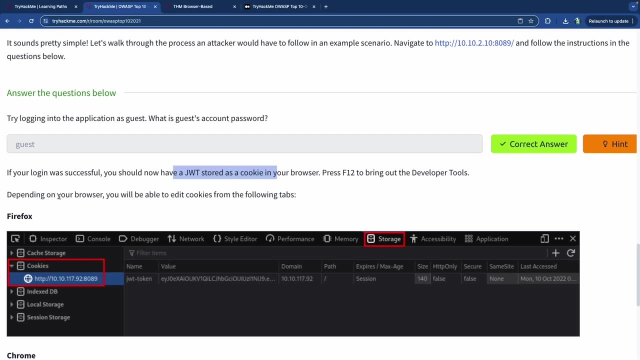 Instruction. So it says: if you're logged in, you should now have a JWT stored as the cookie in your browser So we can look at the developer tools. and we can also do that by clicking right click inspect, And then we'll be able to look at it either. if we're on Firefox, it's under storage. 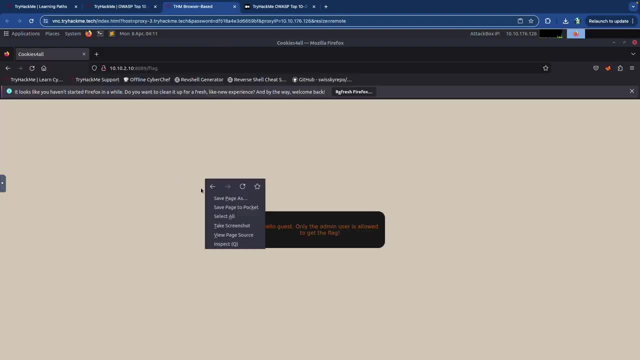 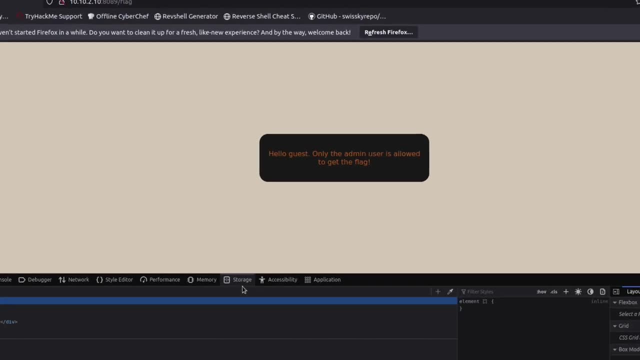 If you're on Chrome, it's under application. So in this case I am on Firefox, So I'm going to click on inspect and then it'll give this information for me here, And then, right here at the bottom, I'm going to click on storage. 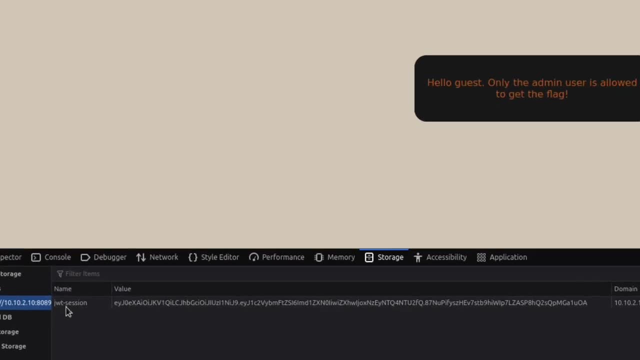 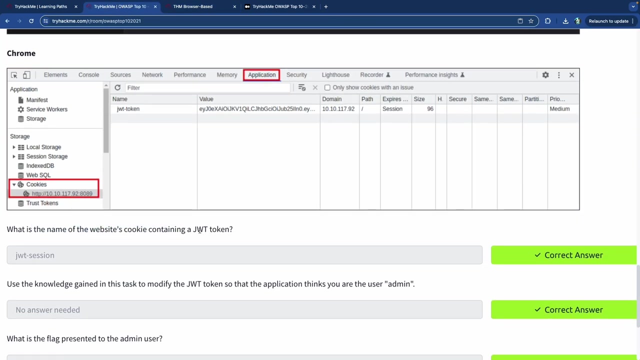 And then it has it saved right here. So the name for me is JWT session And this is the value that's been assigned to it, And notice how there's a dot here And then there's another dot here, right? So what we got here is the first question. It says what's the name of the website's cookie containing 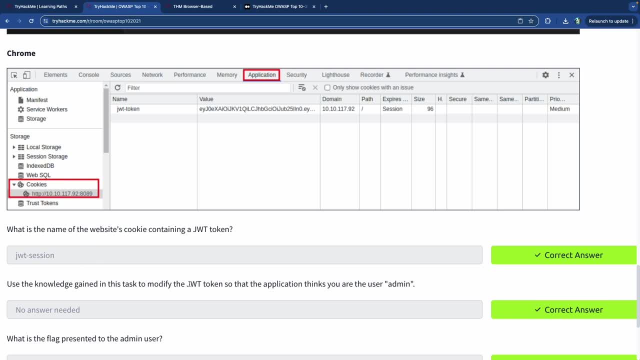 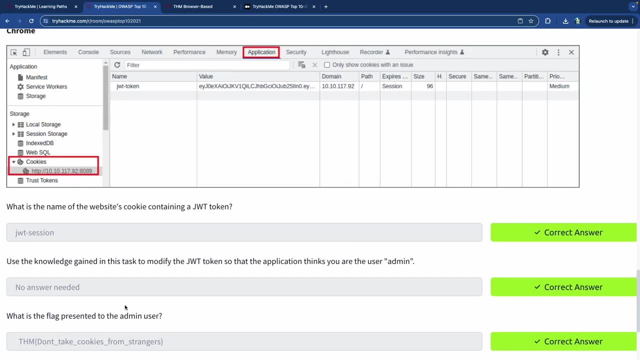 a Coke token is JWT session. So what we're going to do is we're going to modify the token, So the application thinks that we are the user admin and then presented- uh, get, the flag that's been Presented to us. So, uh, in this case, what I need to do is I need to get this information. 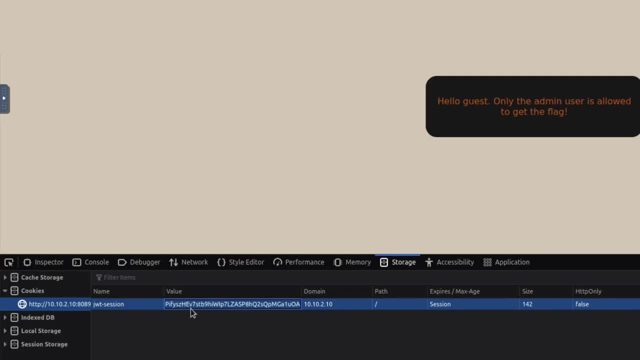 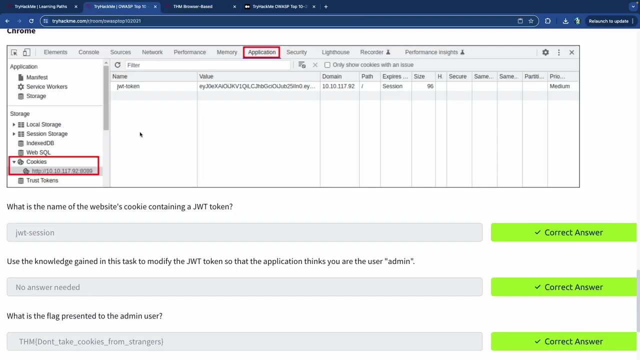 So if I click on this, I should be able to go in there. There we go. So I have this whole thing and I'm going to try to get the full thing. There you go, And I'm going to copy this and we're going to go on that one website. 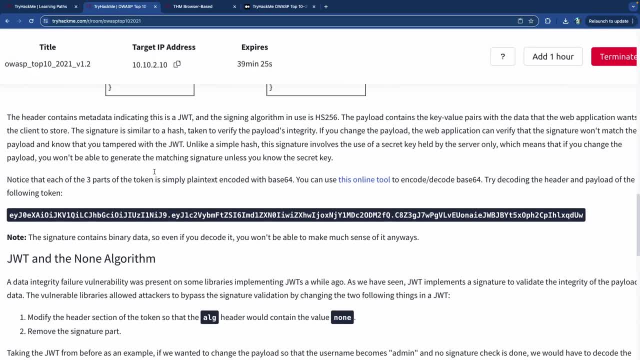 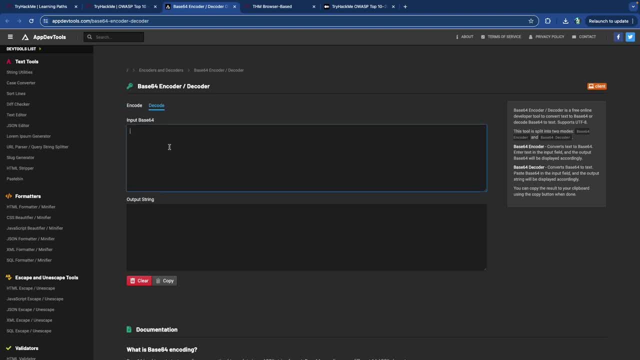 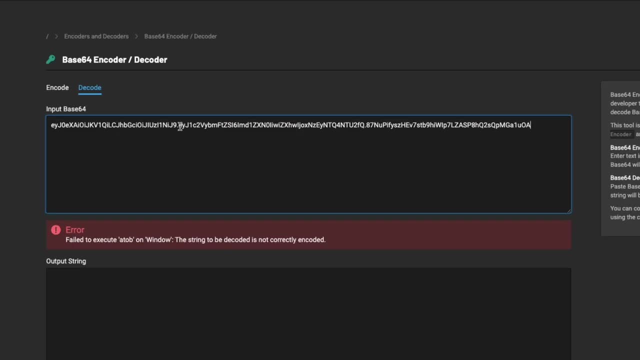 that they gave us here, which is, where is it, This tool? right here, So I can paste this. There we go. So this is the full thing that I copied. So what I'm going to do is I'm going to remove the first portion and I'm going to remove the last portion, And now we have username: guest. 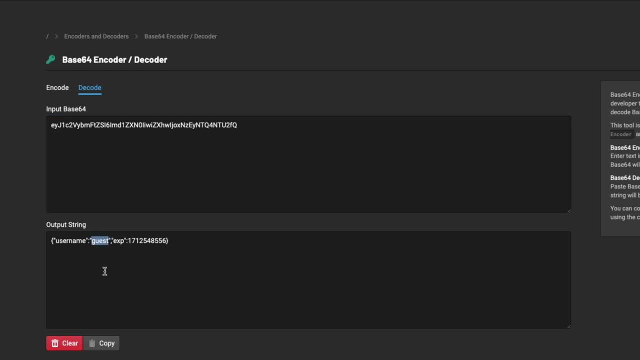 and that's it. So now I want to do is I want to change this username to admin, uh, the output string. So I'm going to copy this part And I'm going to go to encode and I'm going to paste it, And now I'm going to change it. 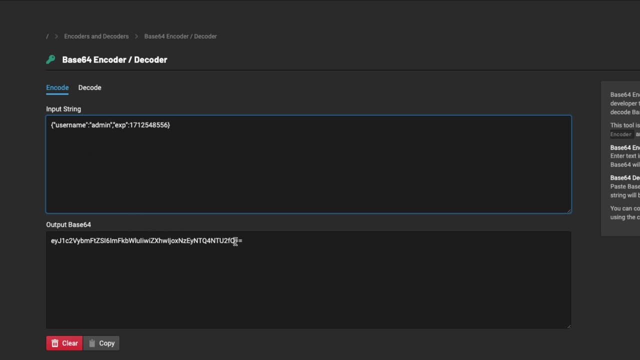 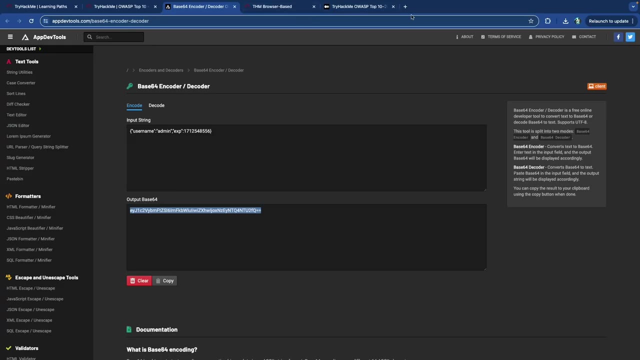 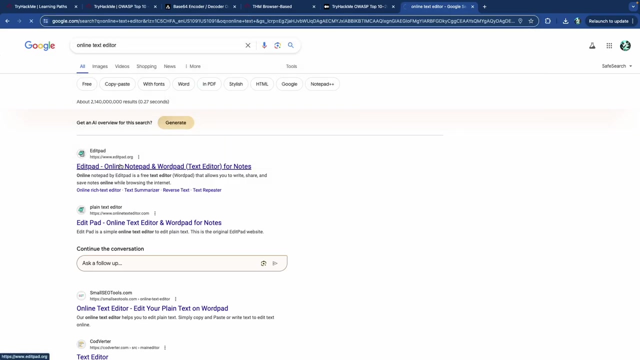 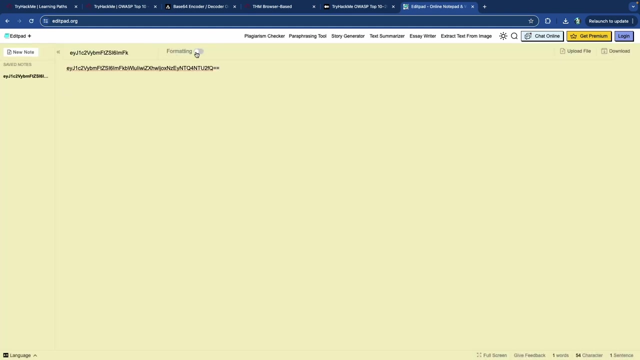 to username admin. So this is what's the base 64 version of that is going to look like. So we're going to copy this and I'm just going to use like an online text editor to make this happen. So, online text editor and we'll do edit pad here And there we go. So this is the new thing. 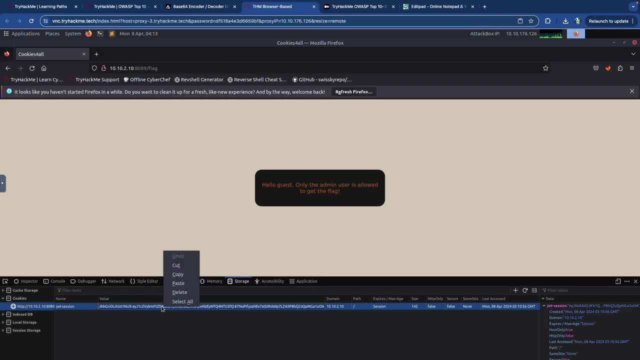 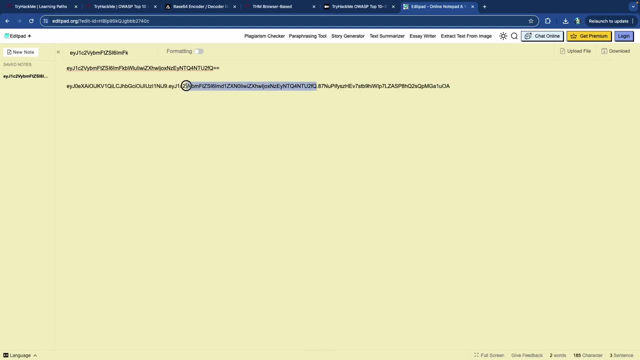 we got. so what I need is now this thing one more time: copy, go here, paste that. so now what we want to do is we want to replace this portion with the new info that we got. so we're going to copy this and we're going to paste it instead of. 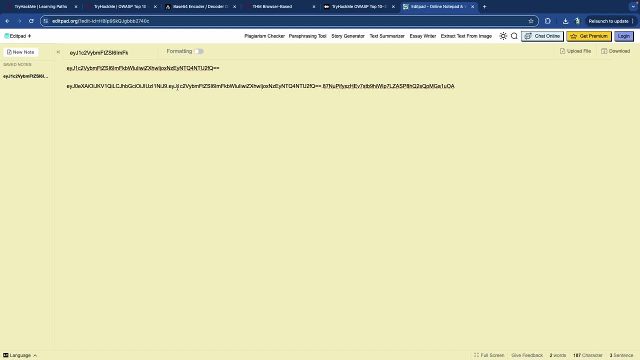 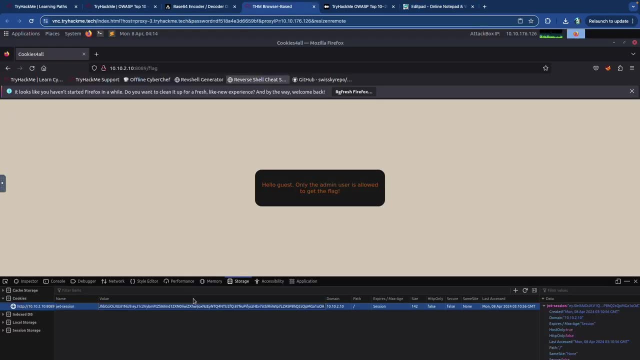 this portion right here. so this is basically between the two dots and now we have this. so now I'm going to go copy this whole thing and go inside of my browser and we're going to do control all to highlight that whole thing, and we're going to paste it in here and press enter. alright, so here's what we're. 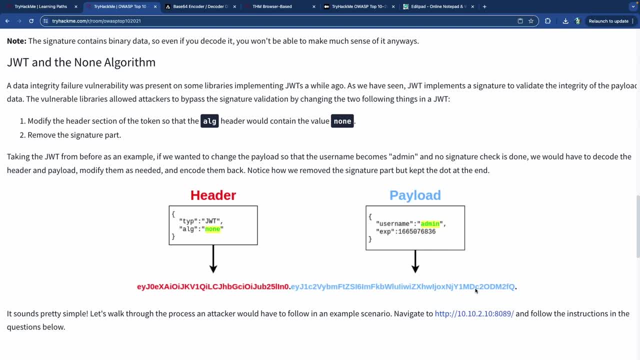 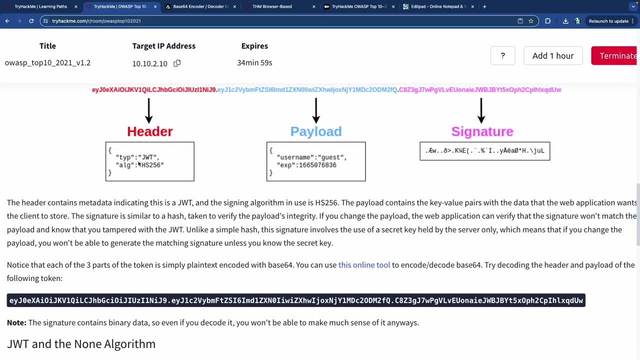 going to actually modify here. we're going to remove the signature because the error that I got is that either the token or the signature is invalid, and I know that I modified this part correctly. but the one part that I'm going to change now is change the algorithm from HS 256, which is what was over here. 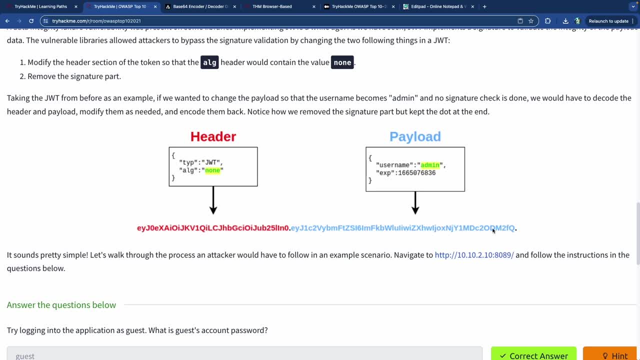 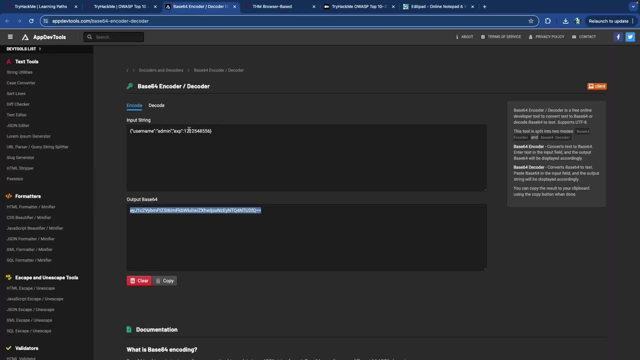 okay. so now we're going to go ahead and paste that in here and we're going to change it to none, and then we're going to just remove the signature at the very end of it. so we're going to go back to our encoder, decoder thing right here and 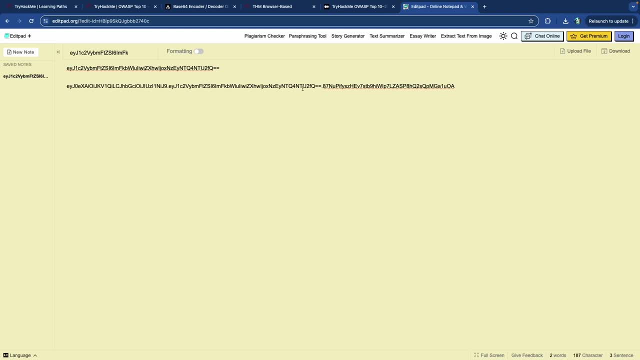 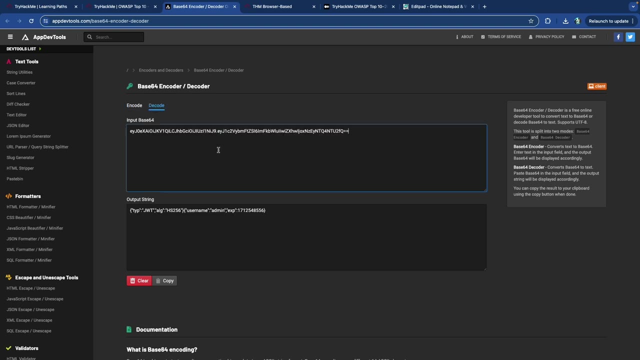 so this is what I had. so I'm going to take this piece. I'm just going to take that out all together. I'm going to keep this piece of information like this. I think I might be able to even do these in one line like so: oh, there you go. 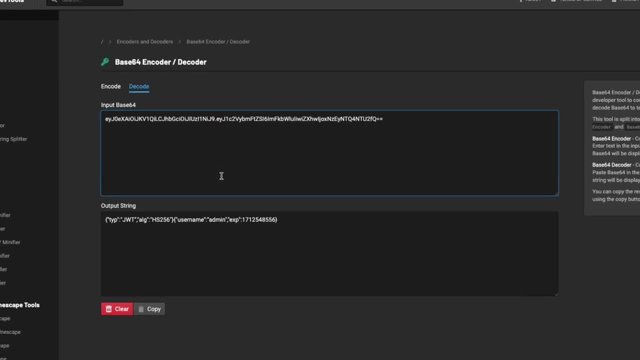 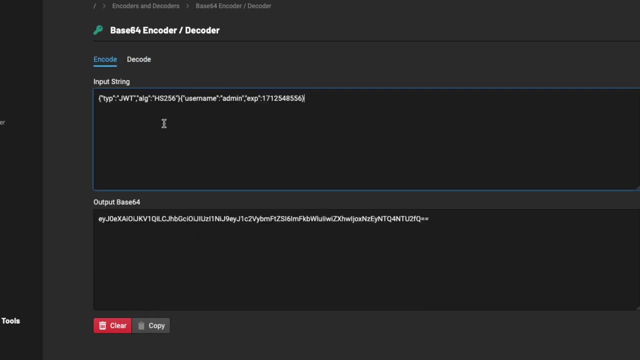 so I'm going to go ahead and paste that in here and paste that in here, and I'm going to just like that so I can change it in one line as such. so now what I'm going to do is I'm going to take this whole thing and copy this, go here, put that in here. 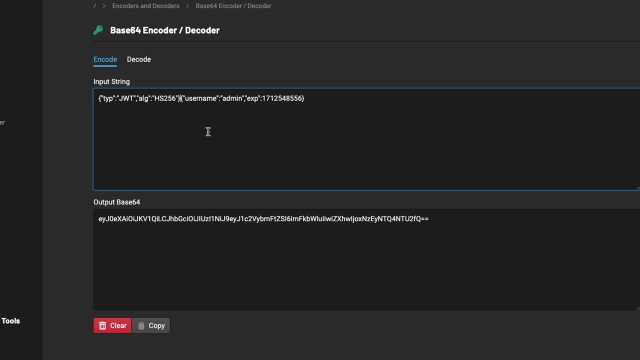 it should. it did not separate it by dot. so what if I put a dot here? no, so it's not gonna work like that. so we're gonna separate them by two lines? nope, it's not gonna work. so we're going to just remove this piece, because I already have this. 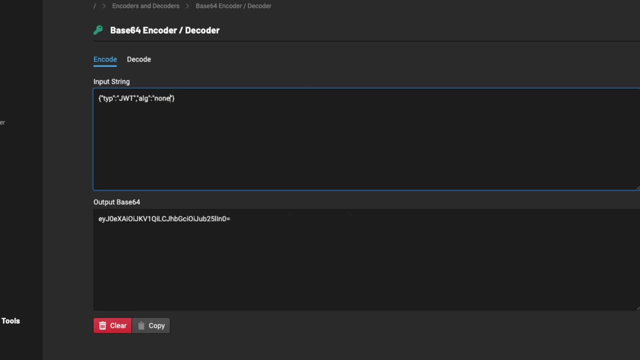 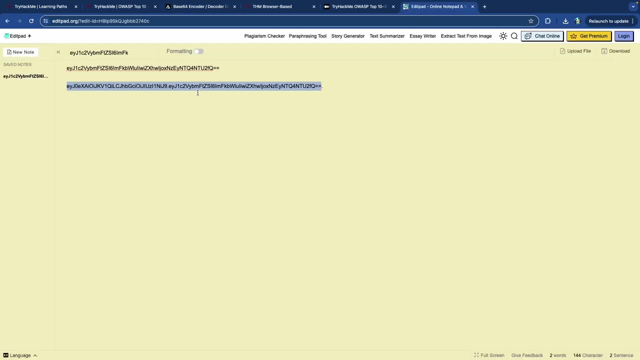 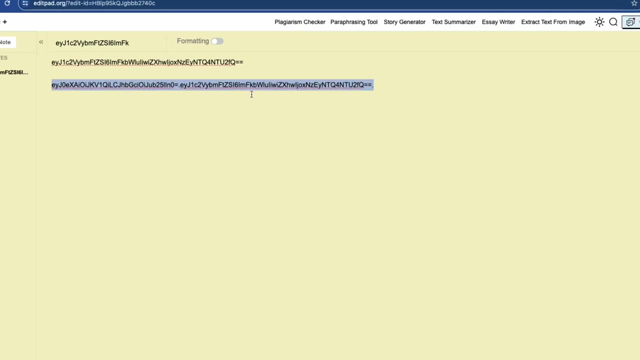 piece and I'm going to change this to none and this will be the new information. so I'm going to copy this and I'm gonna go to my notepad here and I'm going to paste it here and now I have new information, so we're going to keep that dot at the very 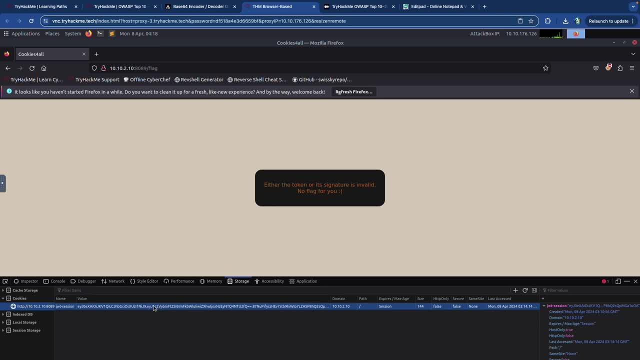 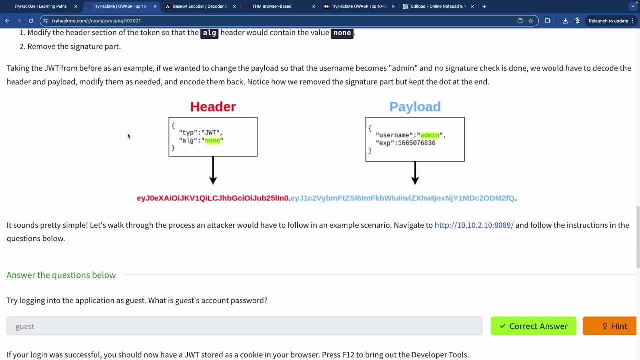 very end. I'm going to go back down here and we're going to change the value of this to our new value. press enter and here we go, fingers crossed, refresh the page. there you go. just like that it worked. thm: don't take the cookies from strangers. so essentially, what we did is: 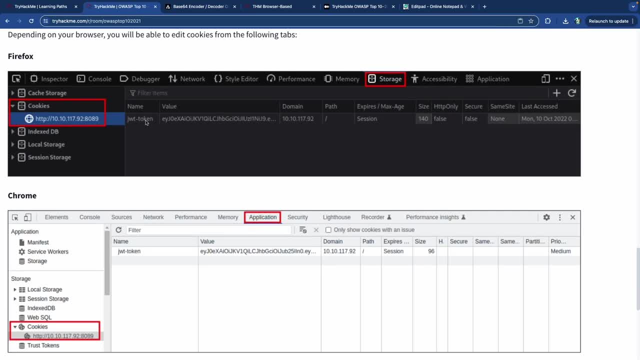 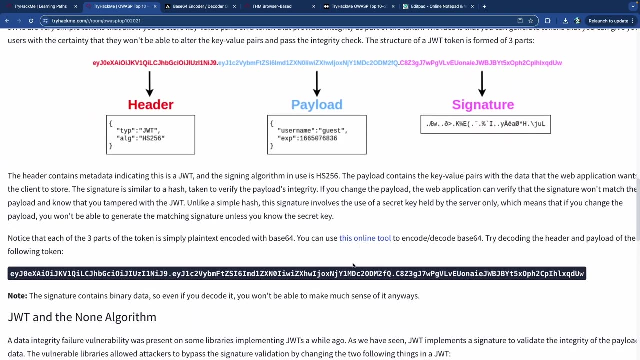 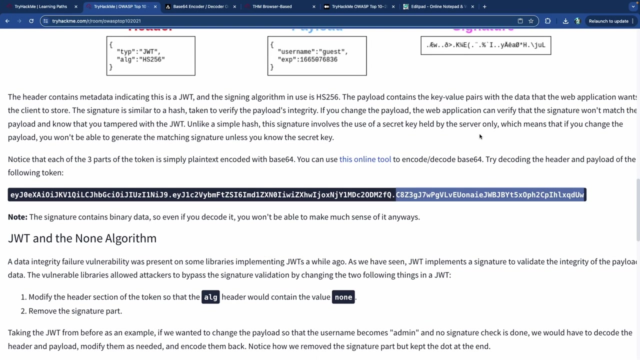 we went logged in as guest, we got the token. that's so crazy, how like. it's so scary, how easy this is. we got the the token value here and it came in three sections which it looked like this: it had three different sections separated by these dots. right, and so we removed the very last piece, which is the signature. 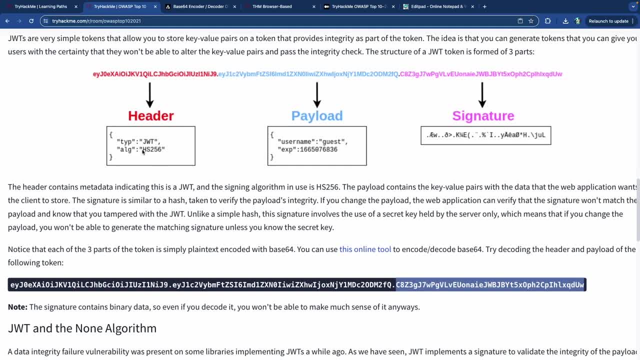 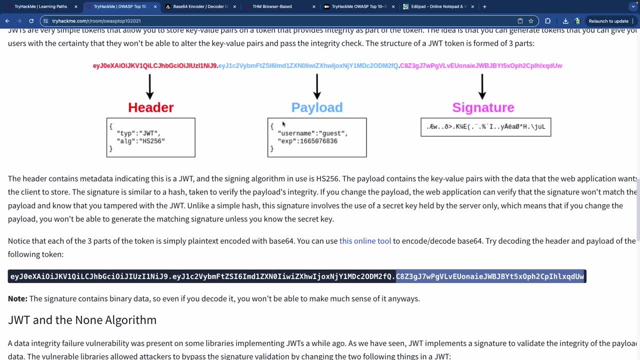 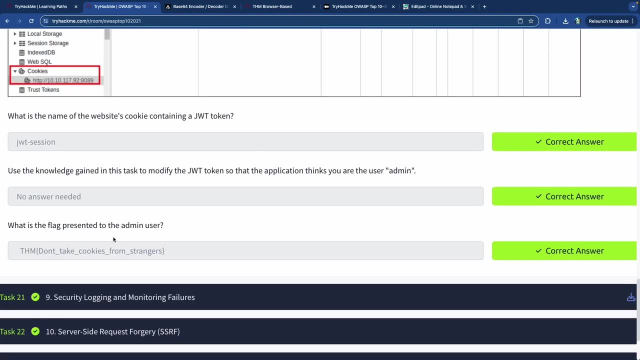 and then we changed the header from the algorithm HS 256 to none, and then we changed the username to admin and that's it. that's all we did. and then we pasted the new value after we encoded it with base 64, and we were able to get our 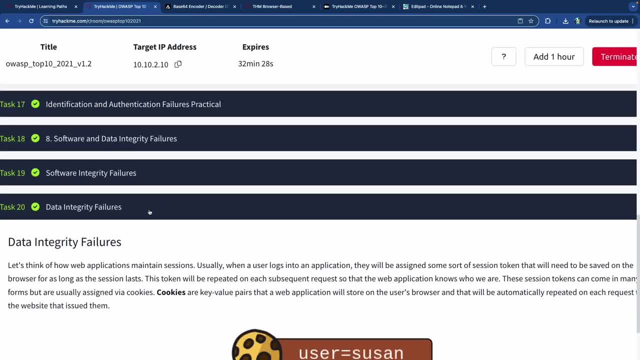 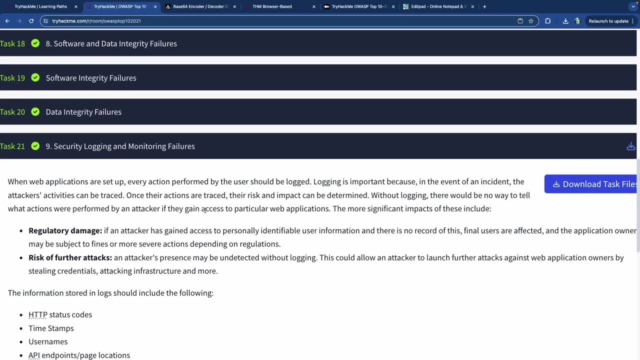 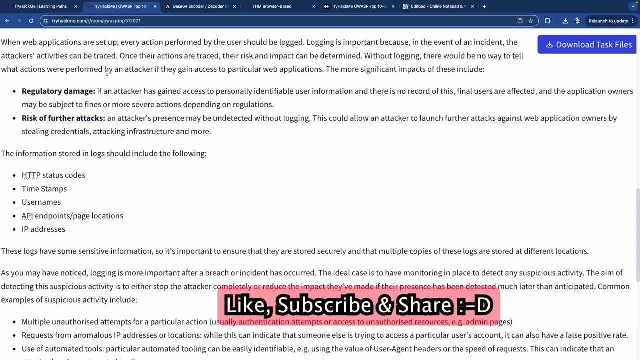 cookie. so that is that for data integrity failure. so let's go to security logging and monitoring failures. all right, so when applications are set up, everything needs to be logged. if not, I mean it has to be logged, and usually it is logged. we actually did a video. the last video that came out was on. 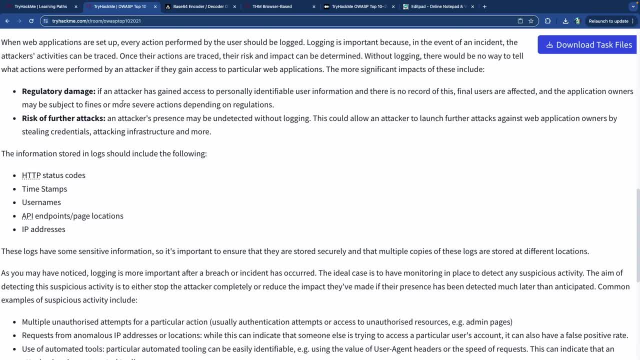 logging and auditing and all that. so logging keeps track of everything that has happened so that when you do an audit or when you're trying to do an incident response or trying to figure out what happened in any kind of situation, you just go review the logs to see what's going on, and usually there's. 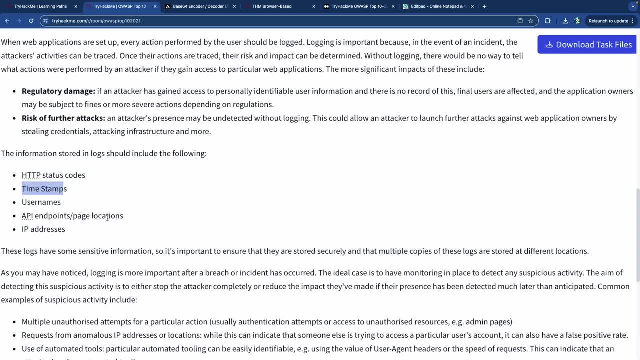 a status code that's attached to it. there's timestamps, usernames, API endpoints and page locations, IP addresses. all those things are inside of the log. each of the log items, like each line inside of a log, usually, especially for web pages, has this information. so what type of HTTP requests they were making, the timestamps, associated usernames. 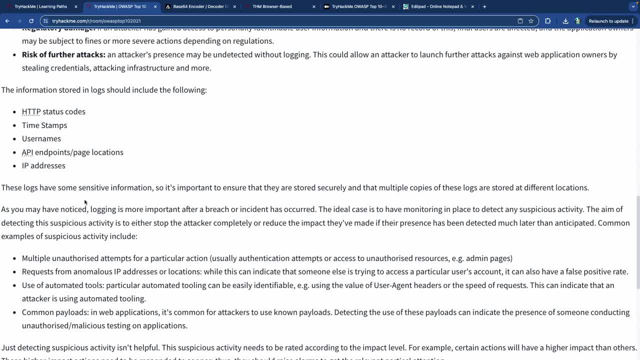 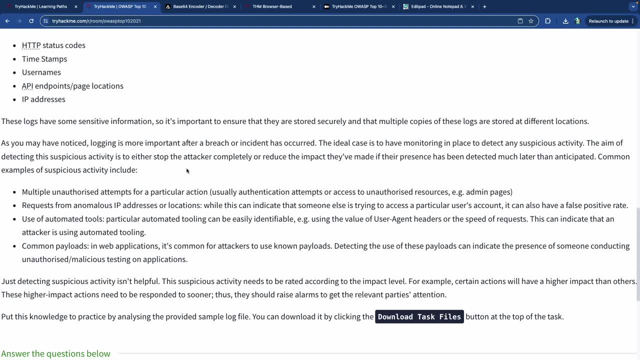 endpoints and the IP addresses- the source IP and the destination IP addresses. so all of that information is usually inside of the log and it's important to ensure that they are all stored and secured and multiple copies are stored in different locations, just in case somebody gets access to it or 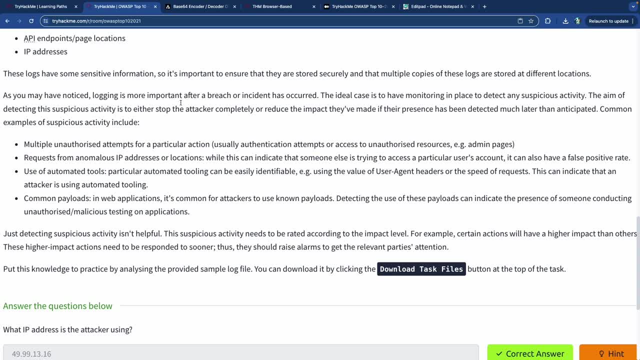 they wipe your systems. so after a breach or incident has occurred, you refer back to these things for incident response. if there are multiple unauthorized attempts for a particular action, then it's logged in: failed login or any kind of failed word that shows up inside of your logs. that's kind of a clue as to see what's going on requests. 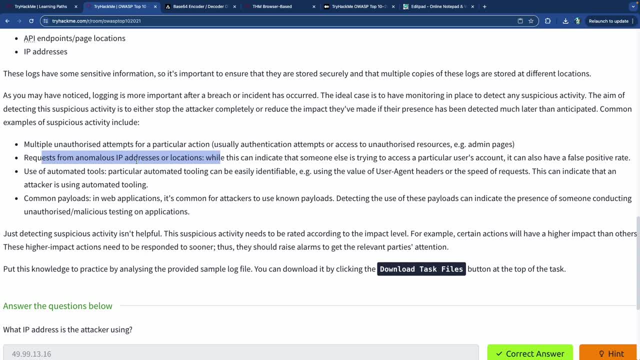 for anomalous IP addresses or locations. there's an entire directory and list of anomalous IP addresses and a lot of the IP addresses that are stored in the log are different. MITRE has them. there's another one that was really, really big. I forget the name of it right now, but there's a lot of websites that collect. 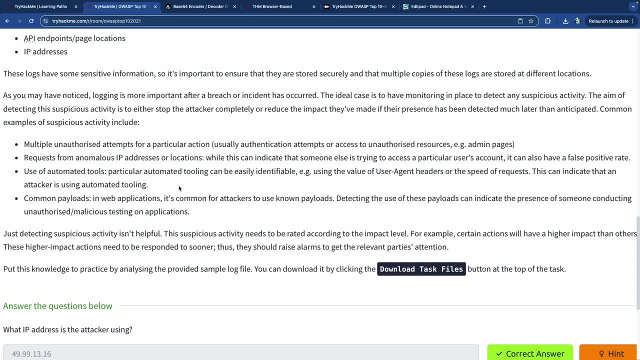 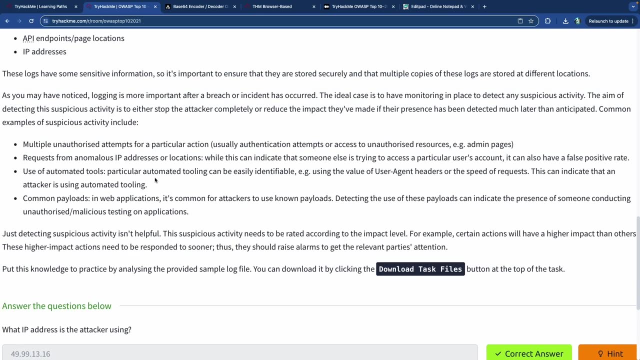 anomalous IP addresses. the FBI- Federal Bureau of Investigation- has anomalous IP addresses and it could be something that has been done to attack your system, so it can indicate that someone else is trying to access a particular account. it can also have a false positive rate, because somebody could be using somebody else's. 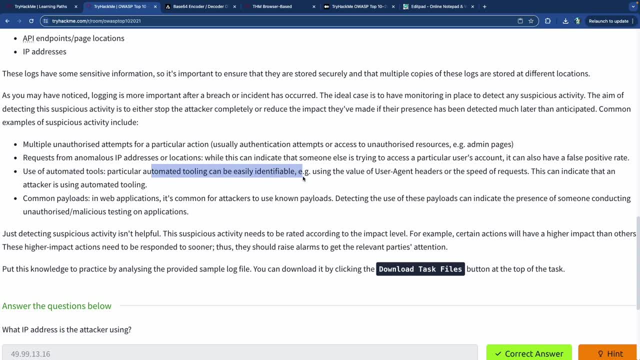 IP address to do this. automated tools: this particular automated tooling can be identifiable. so, using a user agent, header or speed of request, these can mean that there is an automated tool that's being used. it can indicate an attack is being obviously so. common payloads in web applications is common for attackers to use payloads and 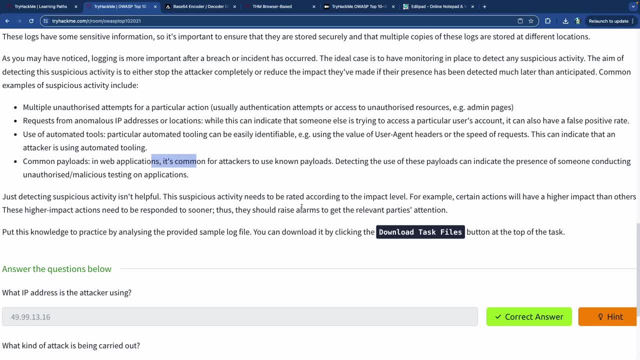 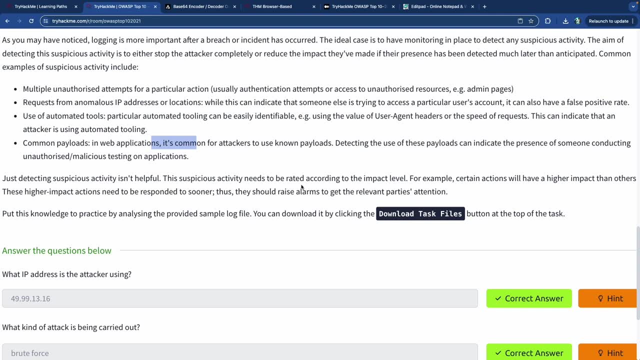 detecting the use of these payloads can indicate whether or not somebody's trying to do something shady. detecting suspicious activity is not helpful just by itself, so you got to have something to either rate the impact level or have some kind of remediation. so certain actions will have a higher impact than others and they need to be responded to sooner. so 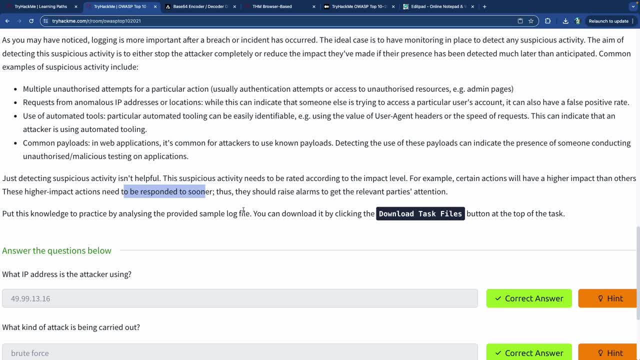 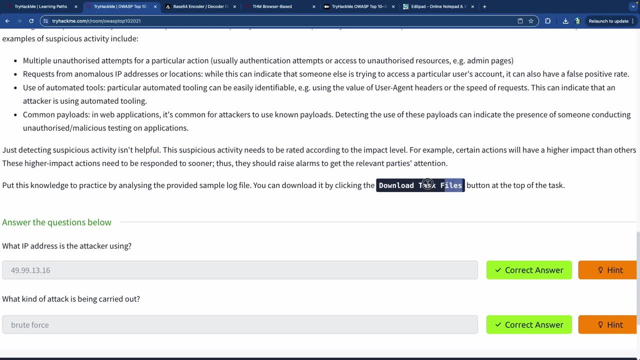 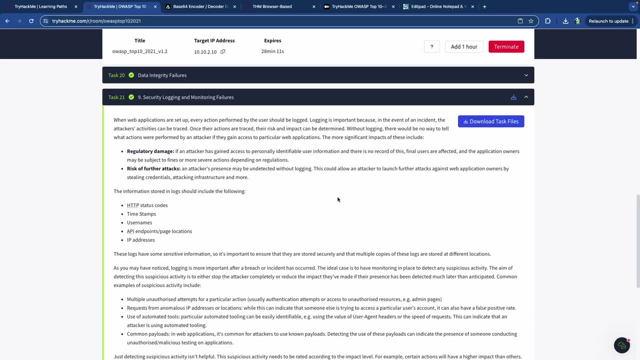 if it's more severe. you have to take care of that before you take care of the less severe ones. very, very basic. so what we're gonna do is analyze the provided sample log file, and it should be inside of this thing: download task files. hopefully it's already inside of the attack box that I'm in, otherwise I got. 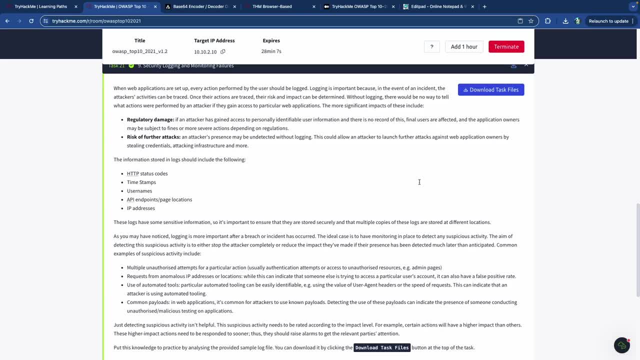 to find a way to transfer it. so let's see if I can find a way to transfer it. so let's see if I can find a way to transfer it. so let's see if I can find that. alright. so I downloaded the log file on my own computer and it's a 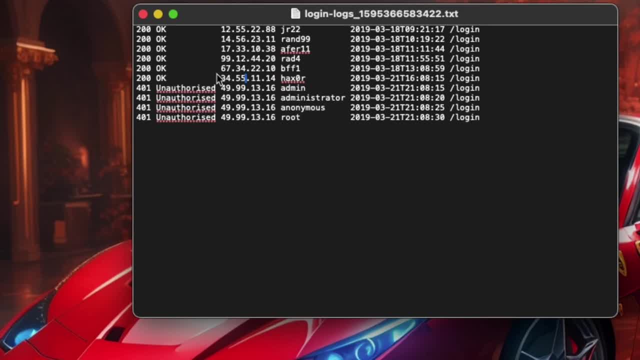 small one, thankfully. so what we can see is the status code, the specific flag that's been attached to it, the IP address and the username that's been attached to it and the timestamp, and then the page that they tried to visit. so you have the login page in all the cases. you have the username in all the 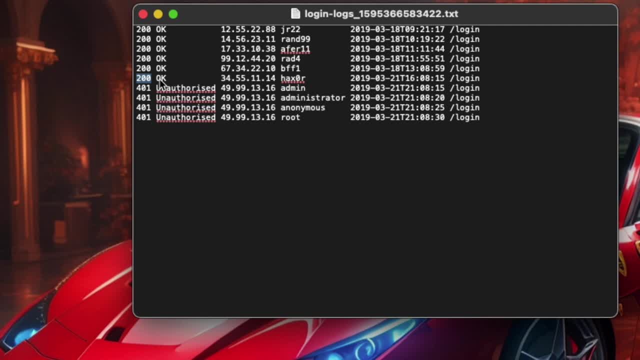 cases. 200 status code means that there were successful and it was all okay, and then this is the ip address that they used, right? so in this case you have 401, 401, 401, which means it was an error, it was not accepted and it was an unauthorized. 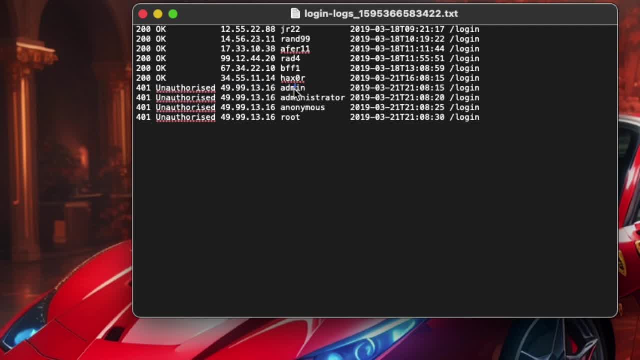 request by this specific ip address trying to do admin administrator, anonymous or root, and it all happened very, very quickly, right? so it all happened at this specific time, five seconds apart, so you can tell that they're doing some kind of a brute force attack using admin administrator. 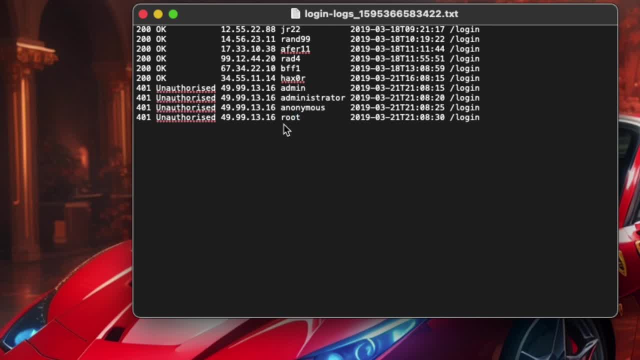 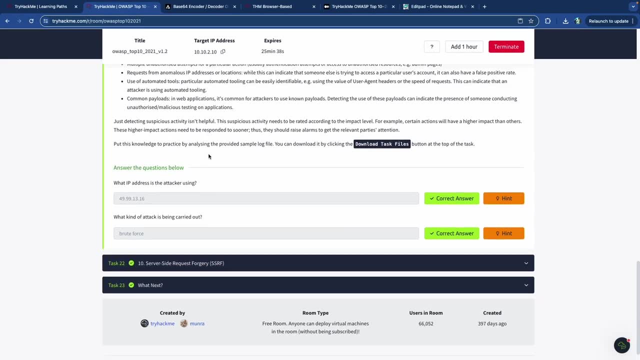 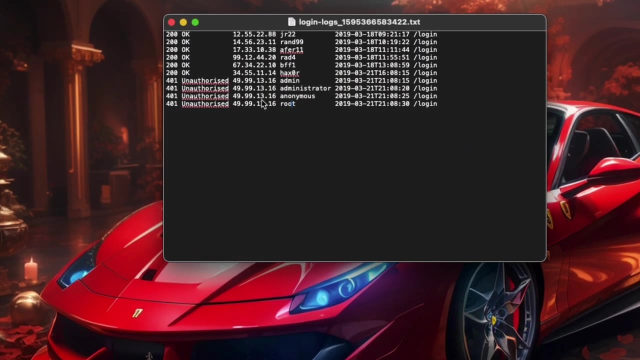 anonymous and root login ids here. so that's the, the log file that we're looking at. so now, in this case, if we go here, it says what's the ip address of the attack that the attacker is using, and that's the ip address that we already established right here, and what's the type of attack. it's a. 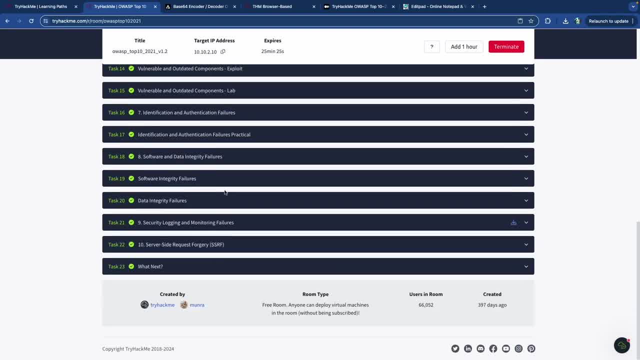 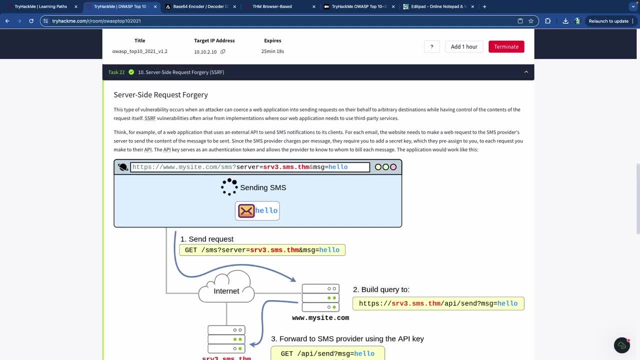 brute force attack, so that one is a brute force attack, so that one is pretty simple. and last but not least, we have server side request forgery, and this is a little bit of a complicated one. it took me a while to kind of grab this or to wrap my head around it. so 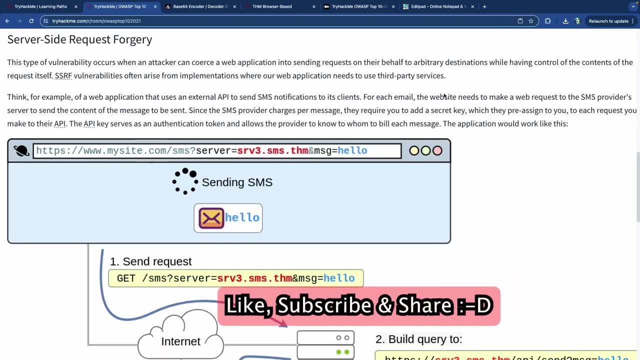 hopefully, this time around it'll be a little bit easier, and for this one i'm actually going to read through all of this instead of trying to paraphrase it. so this type of vulnerability occurs when an attacker can coerce a web application into sending requests on their 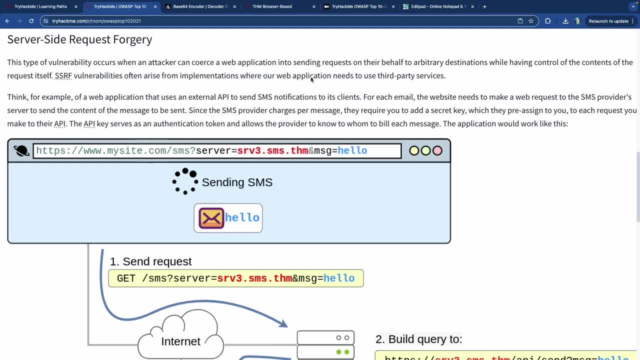 behalf to arbitrary destinations, while having control of the contents of the request itself. these vulnerabilities often arise from implementations where our web application needs to use third-party services. so, for example, if a web application uses an external api to send sms notifications, which texts to its clients for each email the website needs to make? 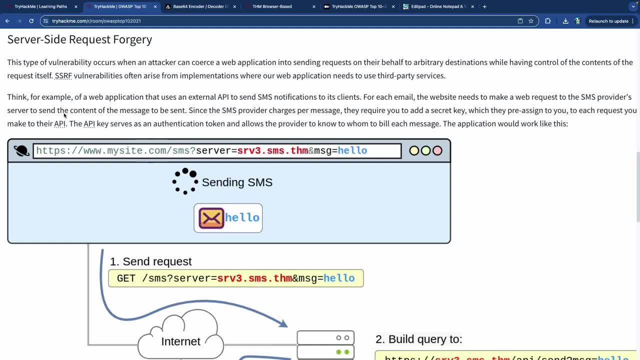 a web request to the providers server and then to send the content of the message to be sent. since the sms provider charges per message, they require you to add a secret key which they pre assign to you each request that you make to their API. The API key serves as an authentication token. 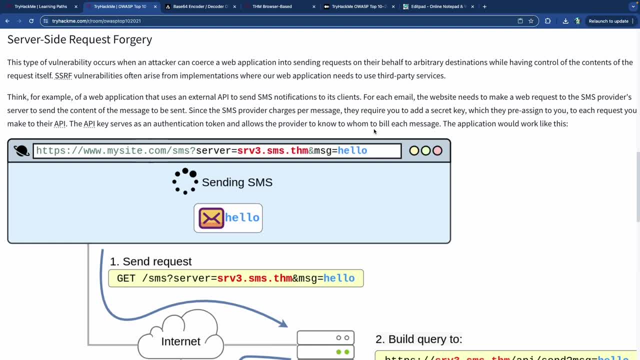 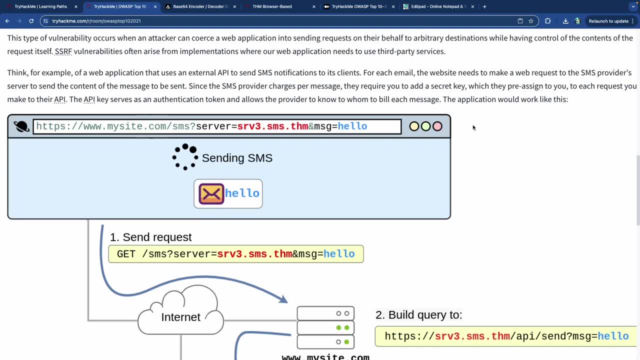 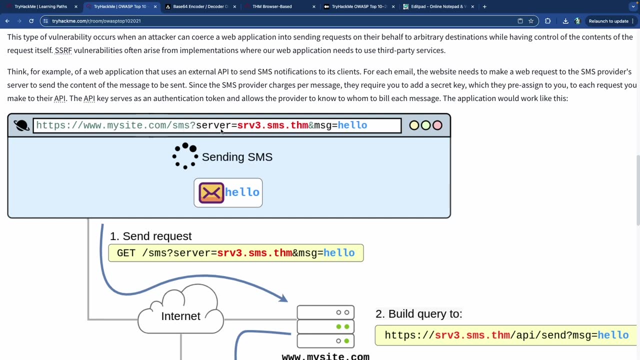 and allows the provider to know to whom the bill should be sent. So, basically, who do they need to charge? And the application looks like this. So you have the URL. Inside of the URL there's SMS, followed by the question mark and then the server, which is the name of the server. 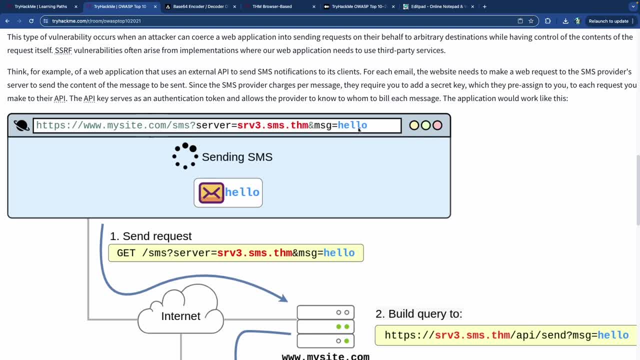 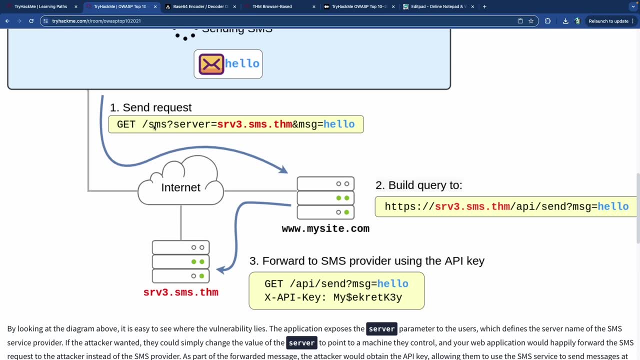 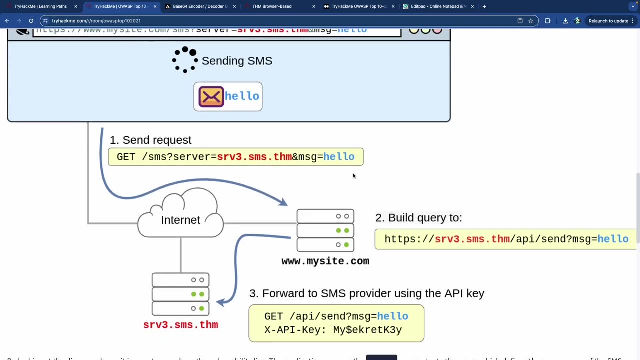 smsthm and the message is hello, And so it's gonna send the message hello and it first sends the request. So get the message, the full block. right after the forward slash, right here It sends a get request including that whole thing. 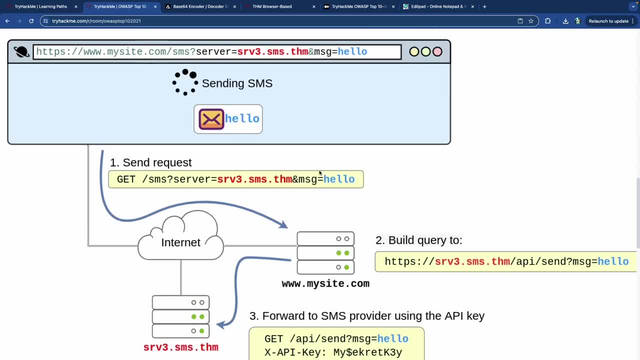 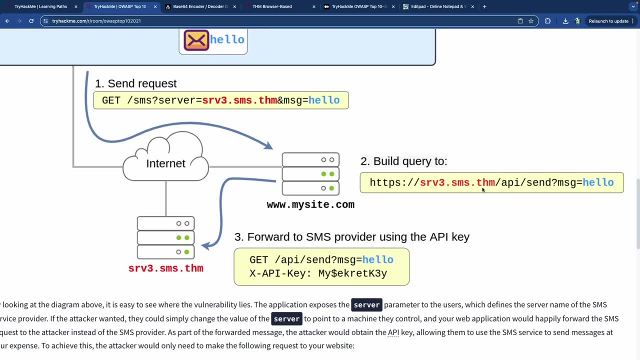 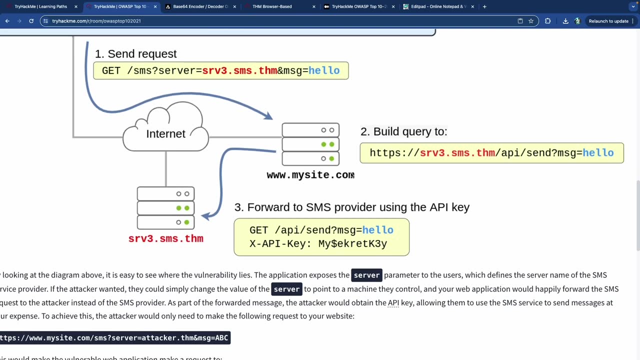 It gets sent to the mysitecom, which is the actual domain itself, and the query is built, And this is what the query would look like. So it's gonna be on the serversmsthm API send and then that's the message. 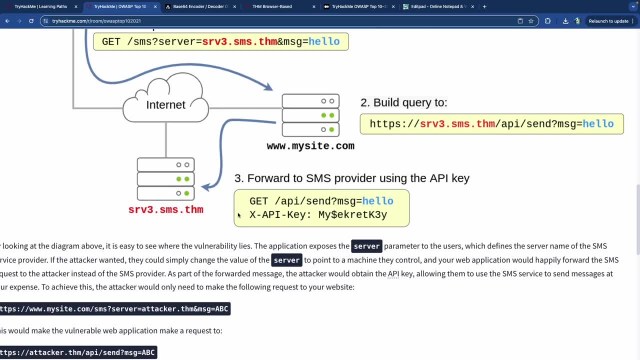 and then forward it to the SMS provider using their API key. So this is what that would look like. It's another get request and then API send. That's the message and this is their API key. And so, following all of this, 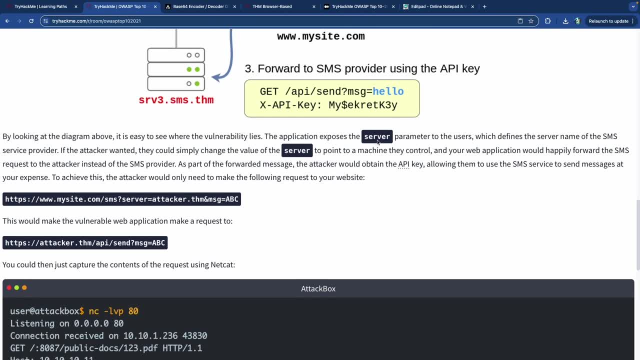 we can understand where the vulnerability itself lies, and it exposes the server parameter to the users which defines the server name or the SMS service provider, And if the attacker wanted, they could simply change the value of the server to points to a machine that they control. 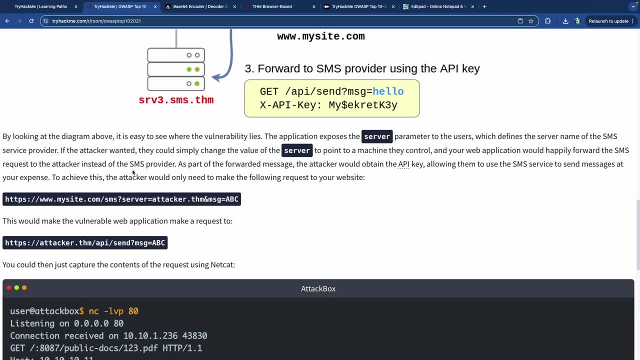 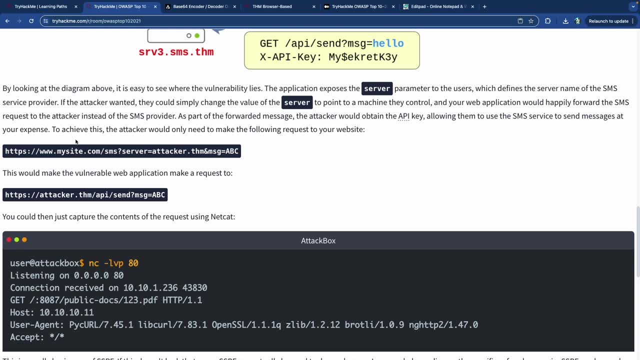 and the web application would happily forward that request to the attacker instead of the SMS provider. As a part of the forwarded message, the attacker would obtain the API key allowing them to use the SMS service to send messages at our expense, and they would need to make the following request. 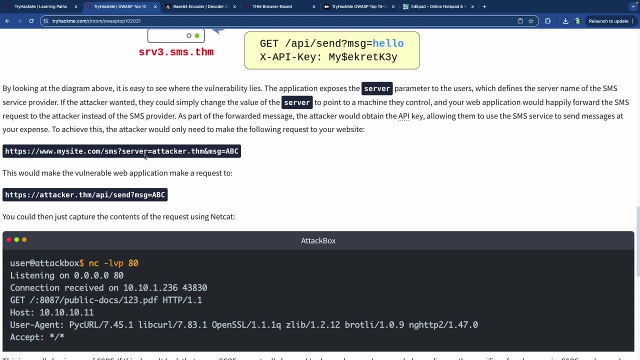 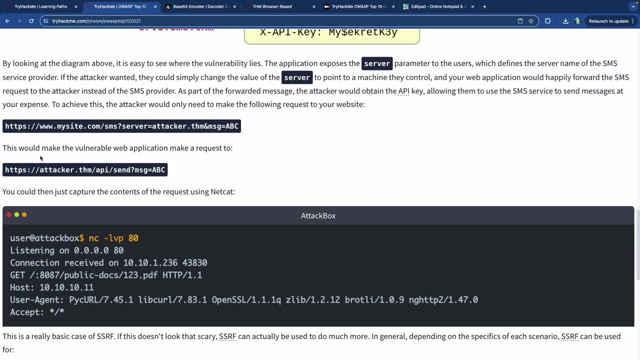 to the website. So first they go to the website. Server is going to be the attackerserverthm, Server is going to be the attackerserverthm, And then the message is whatever, And then it would make the request to attackerthm API. send the message. 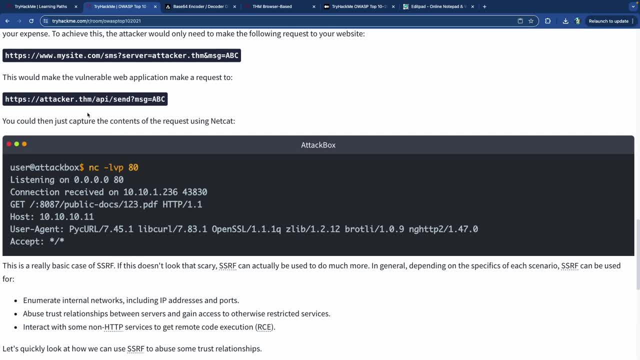 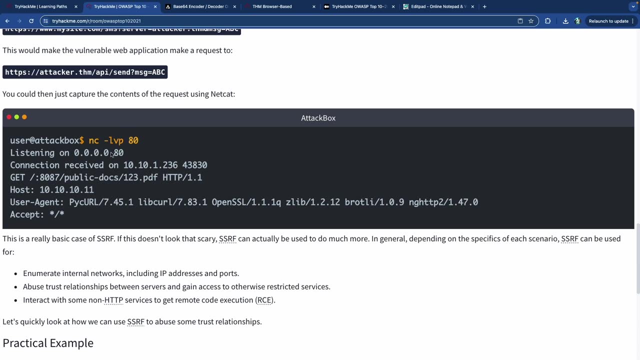 And then you can just capture the contents using netcat and whatever that. this would be their specific server, So attackerthm could be their IP address or anything of the sort, And if they have a netcat listener going on on their port, on their port 80, which is the HTTP port, 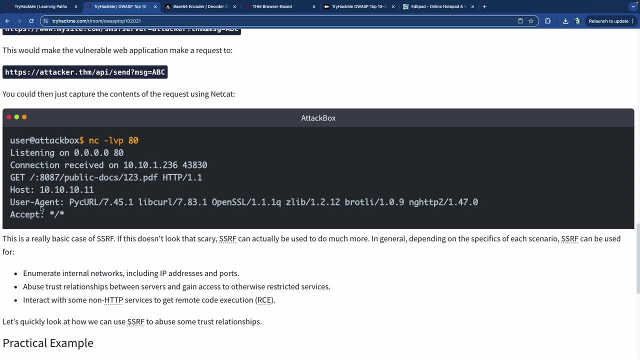 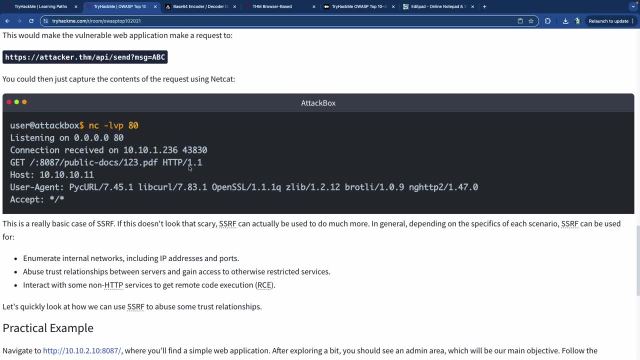 it would just receive that information, because that's where they're sending it to, And then this is the information that they get right. So the connection received: get request public docs. the host is this. the user agent is all this information. 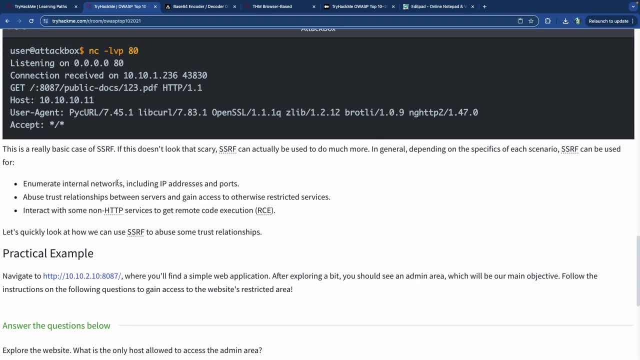 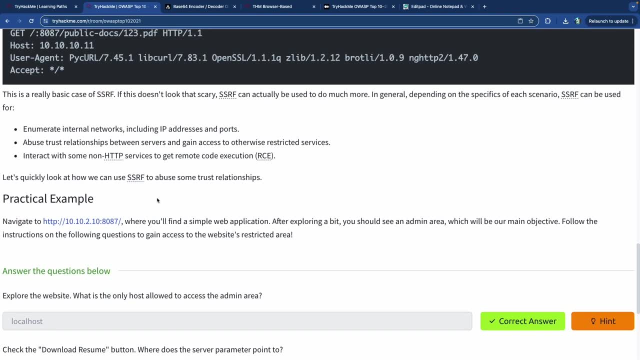 about the user agent, And it's very. this particular example is very basic, but it's essentially the concept is how this works. So what we're going to do is we're actually going to run this and hopefully, this time around it'll be a little bit easier for me to actually complete this. 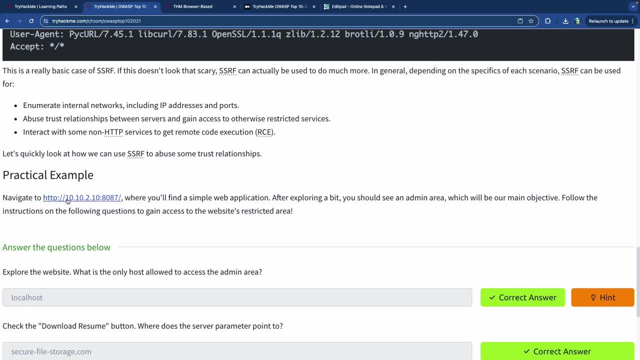 So we're going to run this And hopefully this time around it'll be a little bit easier for me to actually complete this. So what we're going to do is we're going to go to this web portal. We're going to find a simple web application. 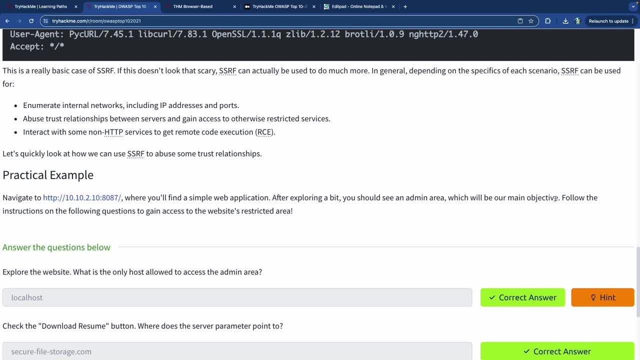 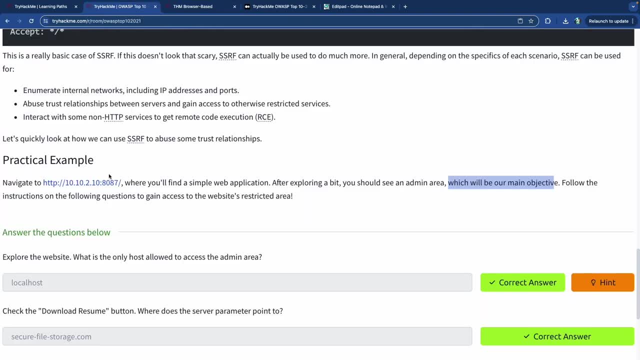 We'll see an admin area, and that's going to be our main objective. So follow the instructions to try to gain access to the restricted area. So I'm going to go to 8087 on our IP address And here's the website. 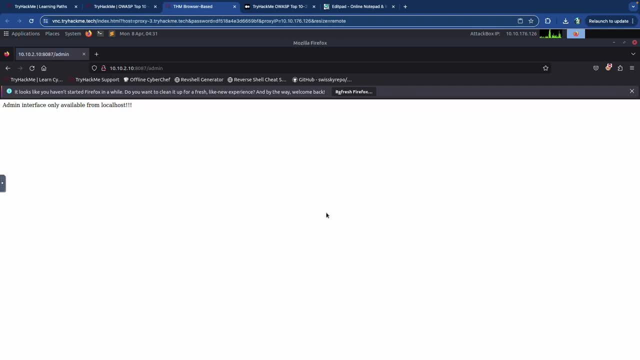 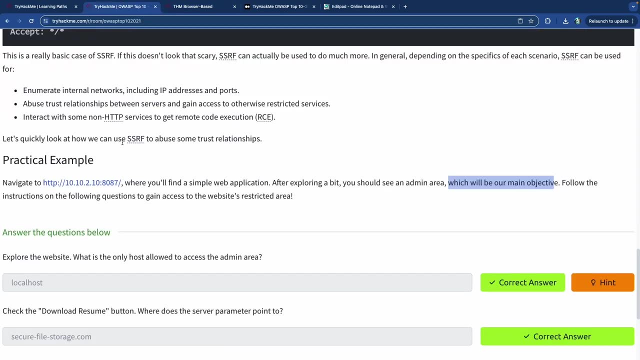 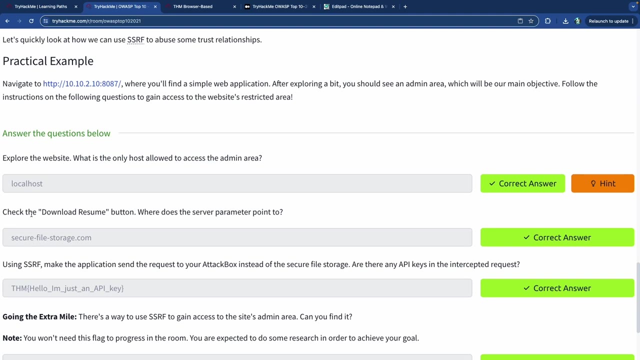 And so we're going to find the admin area in the menu admin interface only available from local host. Okay, So I explore the website. was the only host allowed to access this, which is local host? Check the download resume button. Where does the server point to? 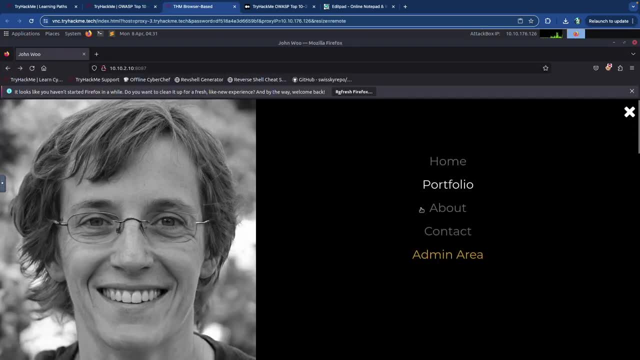 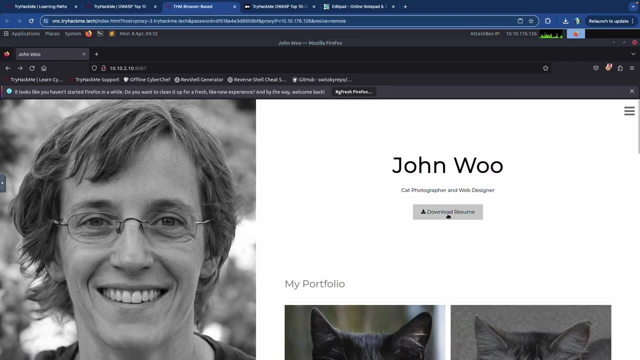 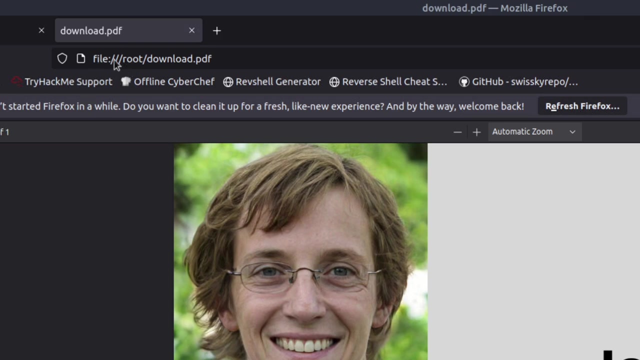 So let's go back to our previous portion And let's go to send the home page where we can do download resume. So if we click on download resume, it's going to point to file root Download PDF. So this is actually pointing to the local host, as it says. 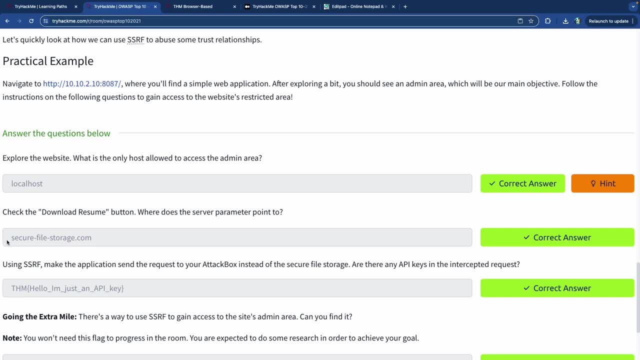 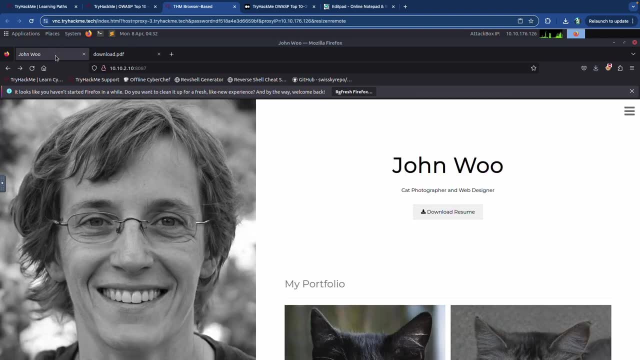 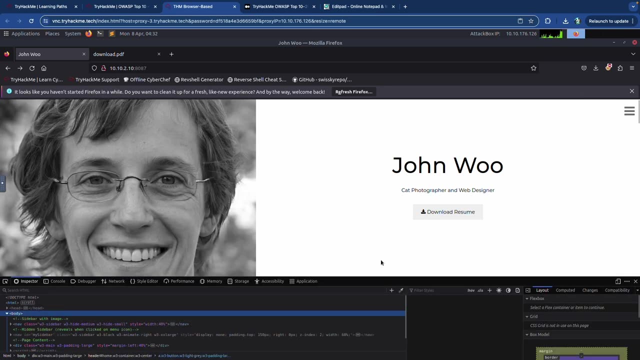 So where does the server parameter point? to secure file storagecom. Is that indeed the case? Oh, you know what? Instead of clicking actual download, I think I'm going to do this and let's see. We're going to do an inspect on that button and see where it goes. 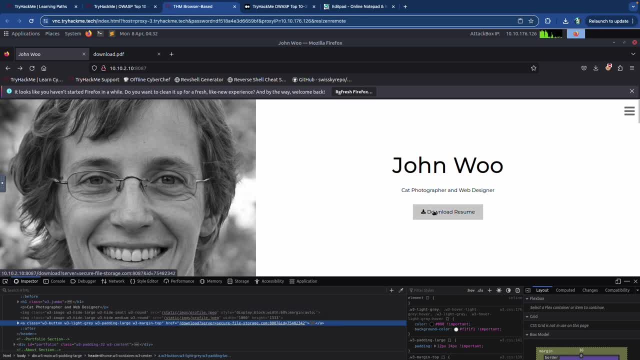 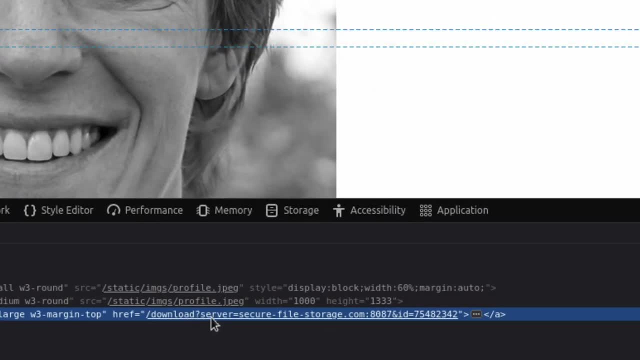 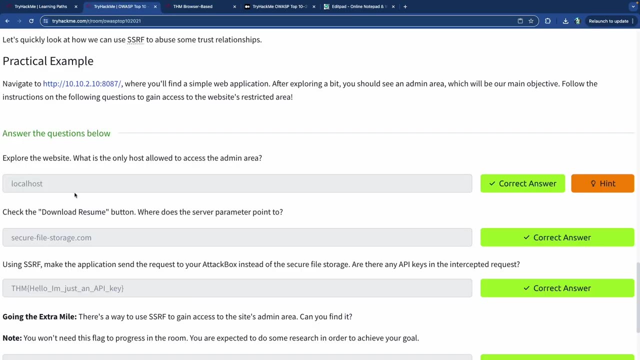 So there it is, And That's the button right here. So that's actually it right down here. So it points to download server, secure file, storagecom, et cetera. So that's where it's pointing to And so that's the answer right here. 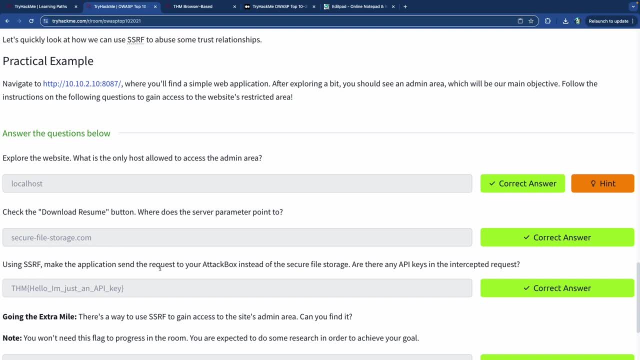 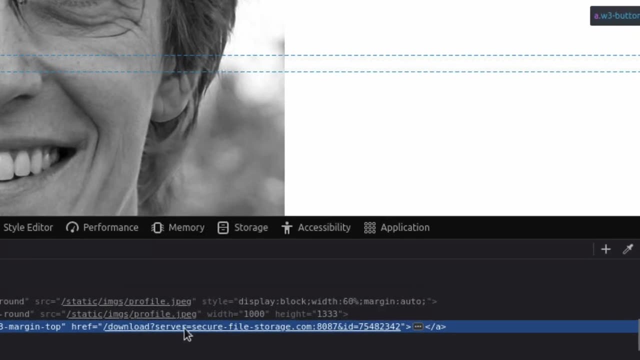 So now, using server-side request forgery, make the application, send the request to your attack box instead of the secure file storage. Are there any API keys in the intercepted request? So What we got to do here is we got to point this to our server. 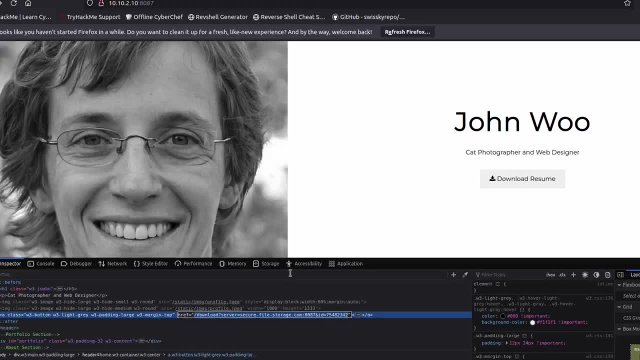 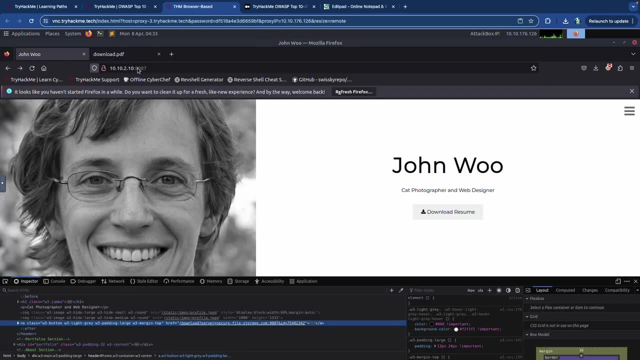 So I'm going to copy this value and I'm going to change it to my server And there it is, But I do need to put this portion at the beginning of it. So we do need to put the actual web page at the beginning of this whole thing. 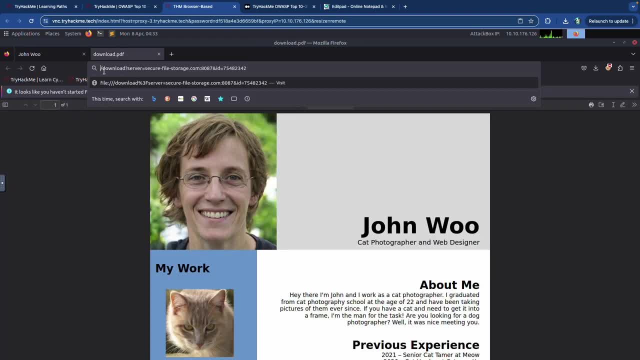 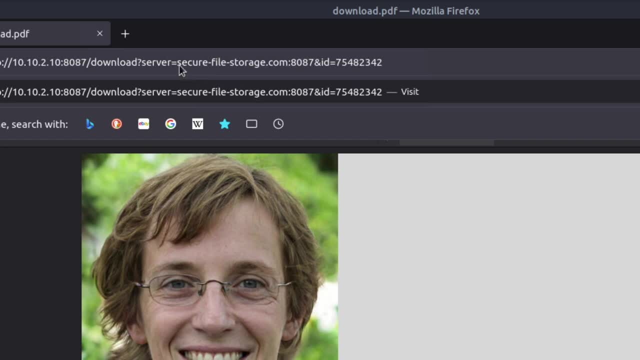 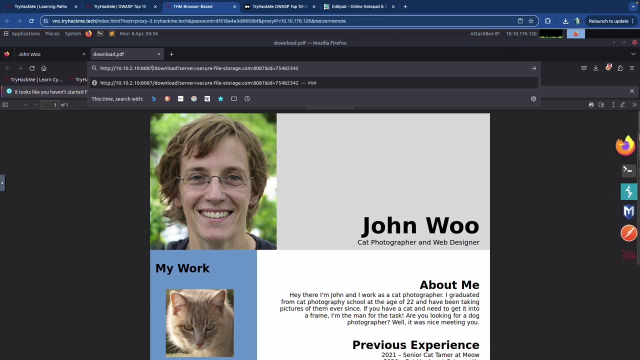 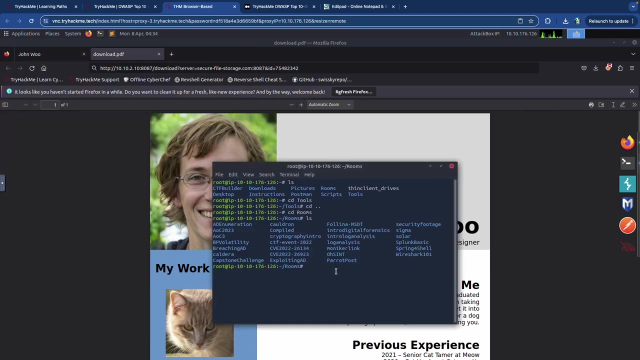 And We're going to put it at the very beginning right here: That's going to be the full link, And what we need to do is change the server. So from this it's going to actually point to my attack box, And so what I need to do first is I need to create a net cat listener, the way that we had it in the example that we got. 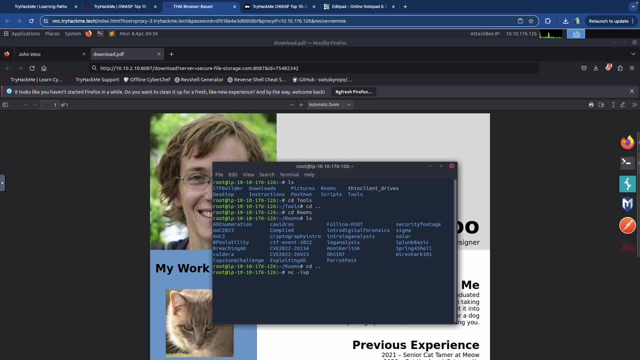 So we're just going to do net cat LVP and I'll do port What 80, will just do port 80.. So net cat LVP port area That's already in use. So I'll do net cat LVP, port 8087.. 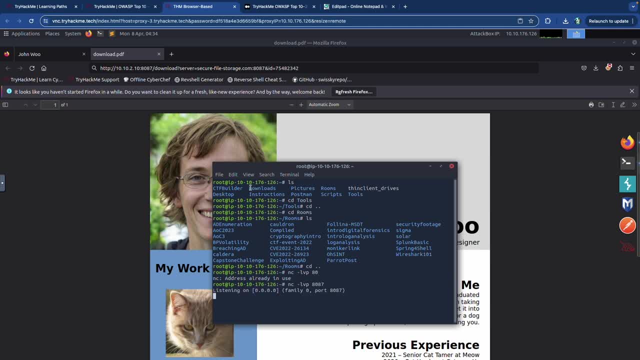 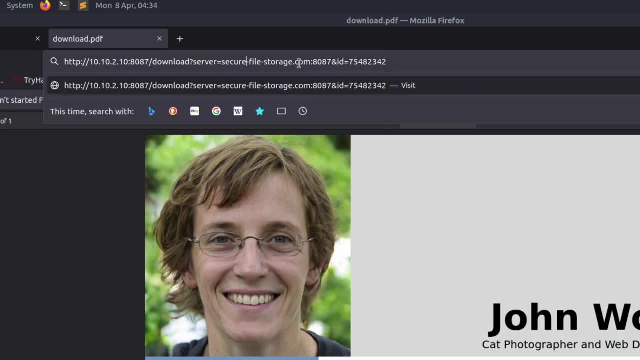 Is that already in use? No, that's fine. So 8087.. So that's already listening, And so now I got to do. I got to come up here and do 10, 10, 176, 126, as the actualcom right here. 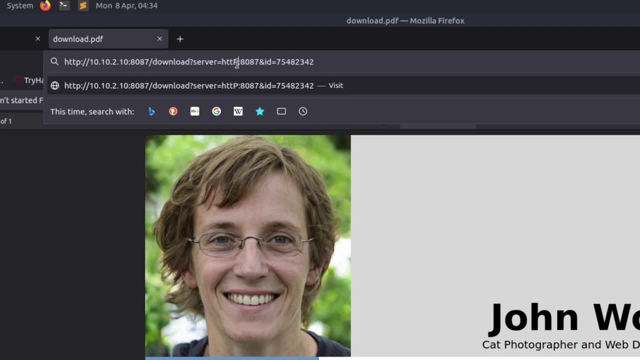 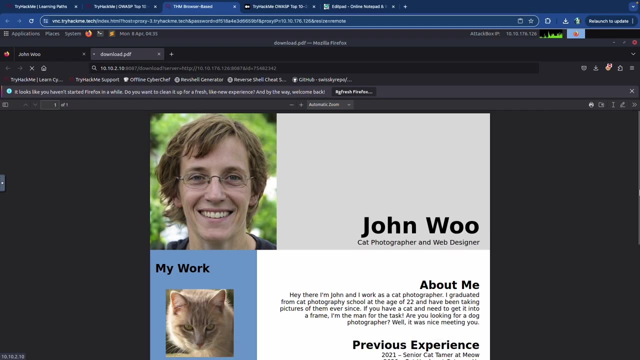 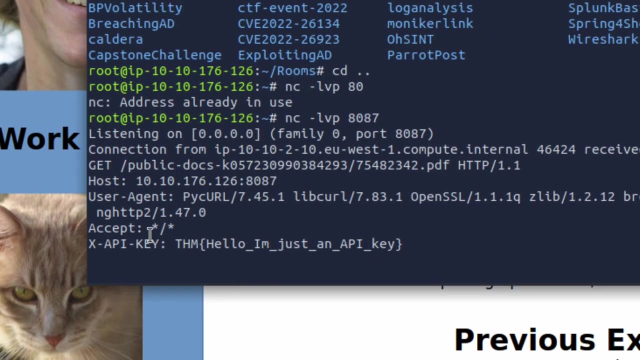 So HTTP 10, 10, 176.. What was it? 176.. 126, see, if that works, It worked. Look at that. Hey, it actually worked. Okay, that was not that bad. And there's our API key. 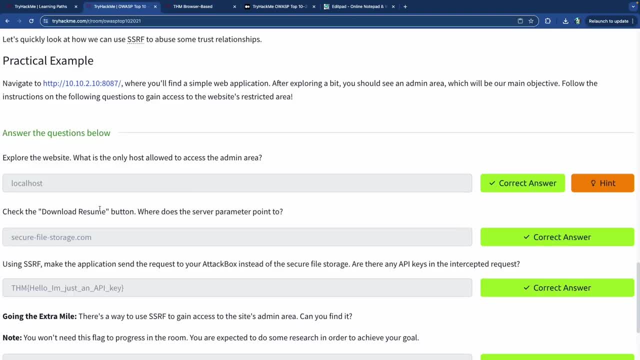 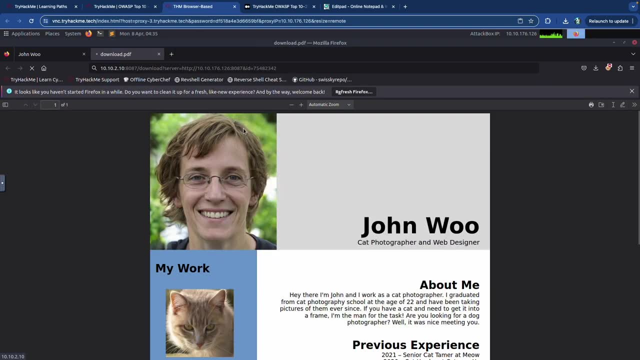 I'm just an API key And there it is. So this was not that bad. I don't know, Maybe it was just so far over my head last time that I had no idea what I was doing, But it seems to be. 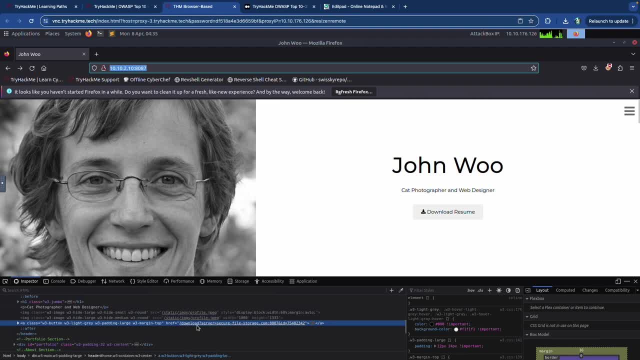 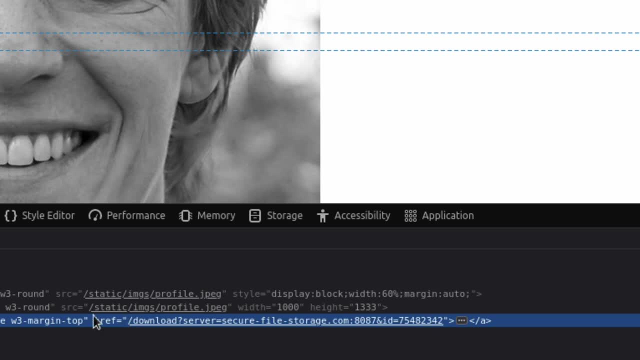 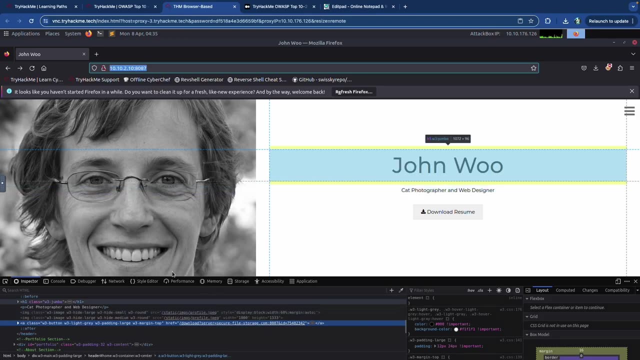 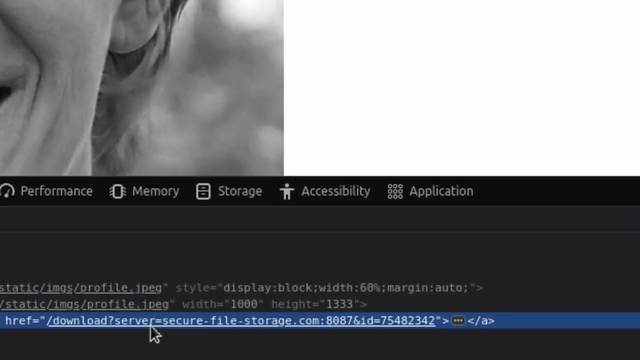 It seems to be way easier, way easier this time around, Right? So that is it. So you just make sure that you have that portion correctly configured, or you know, you just basically copy this entire value right here, You put it in front of the actual URL right here, and then you change the part where it's after the equal sign. you change equals to this entire piece right here. secure file. 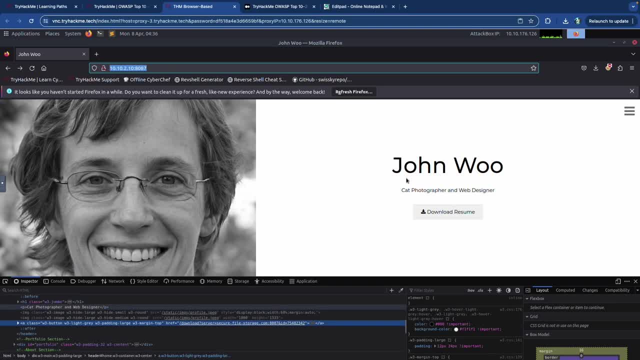 You take that whole thing and you turn it into your attack box IP address, which is this particular case, or your computer's IP address, at whatever port your netcat listener is running on, which is, in this case, port 8087, and just like that. 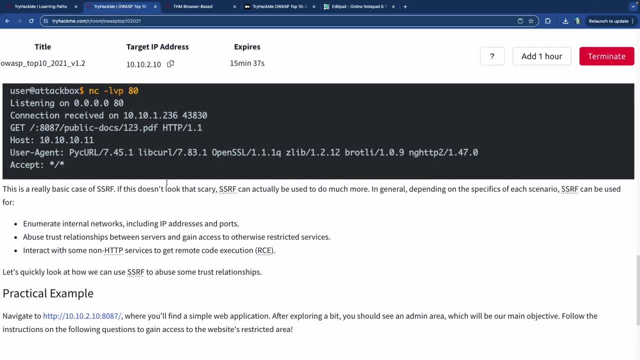 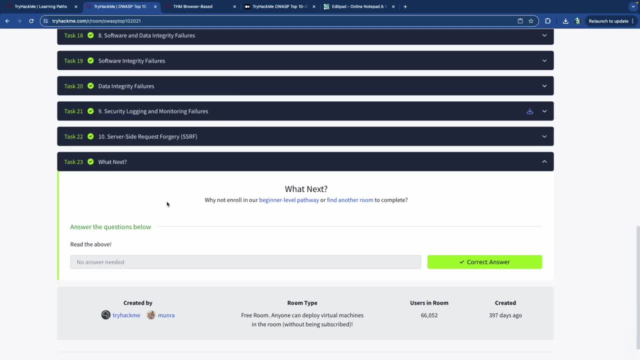 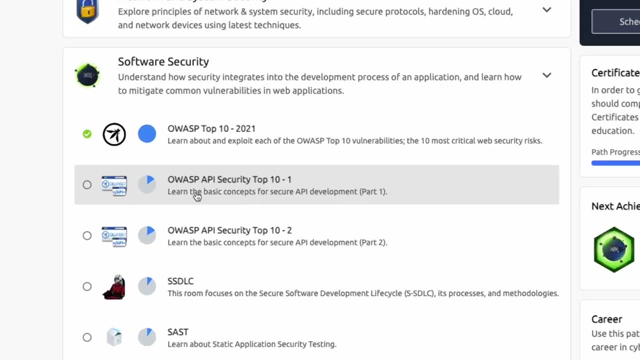 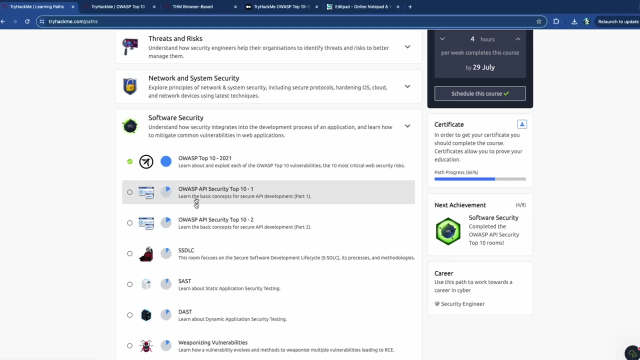 We got our flag and everything else was good, So very, very excited about this one. I'm very happy that that was actually done. So this was actually the beginner, So Kind of like an introductory to OWASP top 10.. We actually have two more rooms around OWASP top 10 API, security, top 10 1 and top 10 2.. 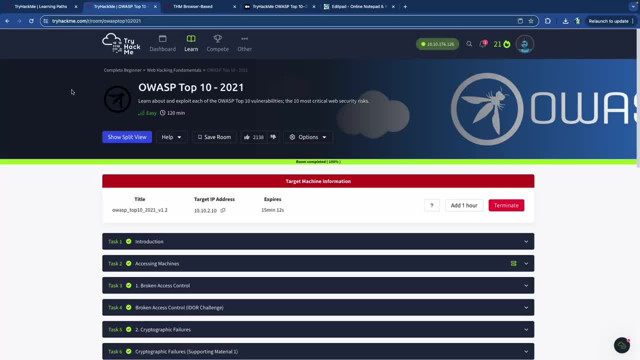 So we're going to do an entire other set of videos just around this concept, and it should be fun. Honestly very, very excited about it. 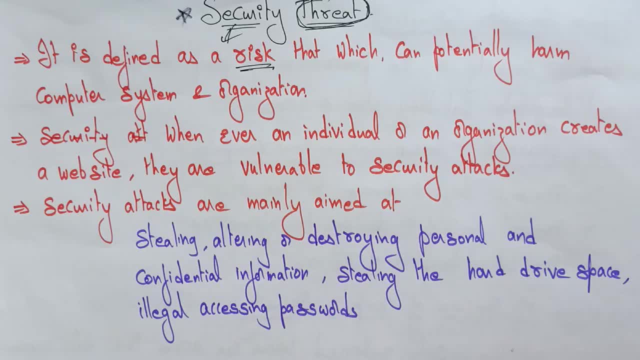 Hi students, welcome back. Coming to the next topic in this subject, web technologies, is a security threat. This security threat is one of the important concept in this web technologies, not only in the web technologies: in our daily life also, it is very important.